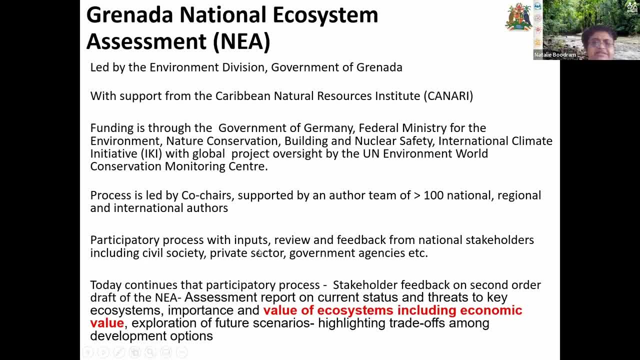 Our Grenada NEA is a very participatory process. So, as you all know, we've done lots of consultations, meetings and we are looking for both review and feedback and input from all national stakeholders for this initiative, And today what we're doing is that we are looking for stakeholder feedback. 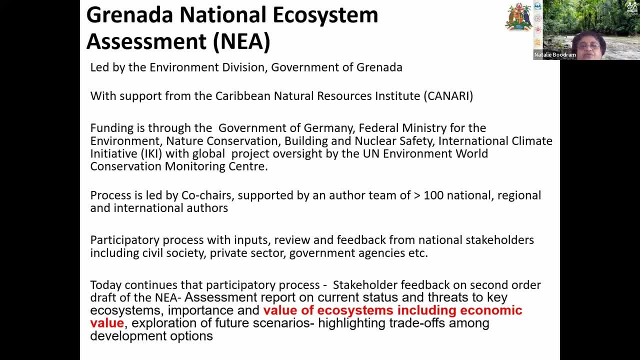 on what we call the second order draft And remember that the main product of the National Ecosystem Assessment is this assessment report, which looks at status and threats to key ecosystems and looks at the importance and tries to highlight the value of these ecosystems, including economic value, but not only economic value, And the idea is that, if we can, 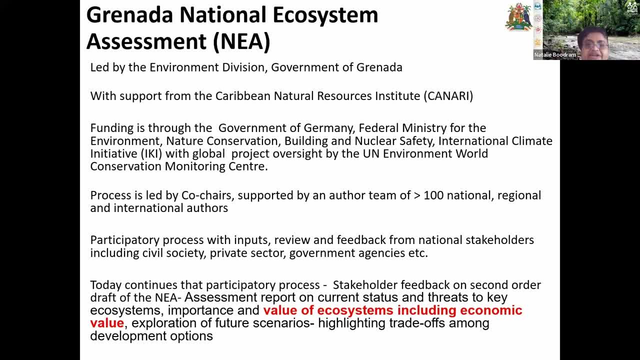 put some values, including monetary figures, to some of these resources, we can better try to advocate to protect these resources, And the report also looks at future scenarios. So what we try to do is present. if we do X to protect this mangrove, this might help us later on because it will protect. 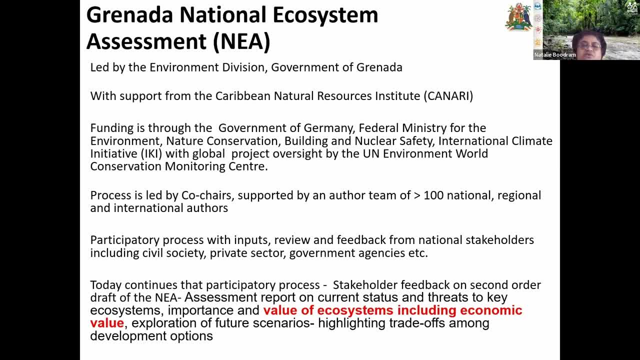 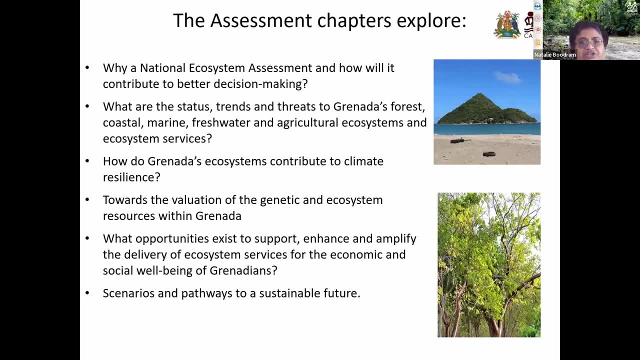 against hurricanes, to the value of, etc. So what we are doing- there are other products, of course, but today we are focusing on the second draft of the assessment report and we're looking for feedback on that. So the report has six chapters now and about a week ago or two weeks ago we looked at chapters. 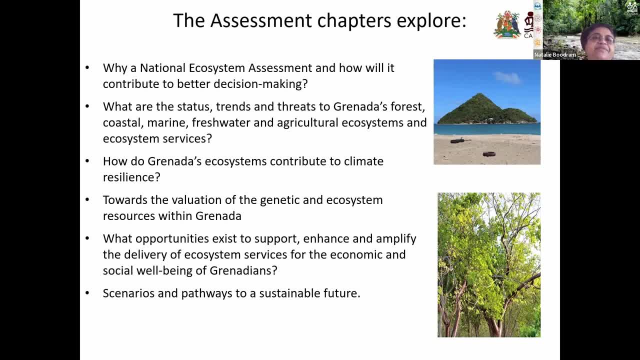 one and two, which explore the status and trends, and then the introduction to the whole NEA, and today we focusing on how the ecosystems contribute to climate resilience. that's chapter three, and then the valuation chapter, which includes both genetic and ecosystem level evaluation. We won't be looking at the last two. 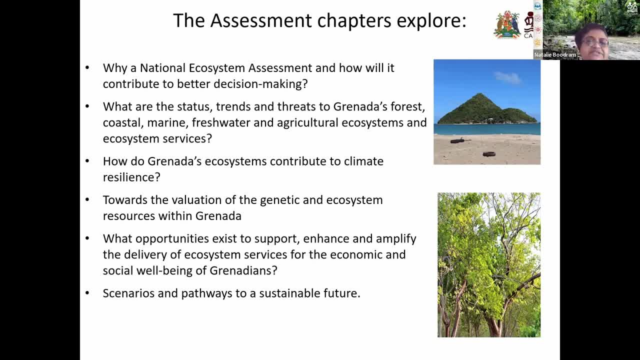 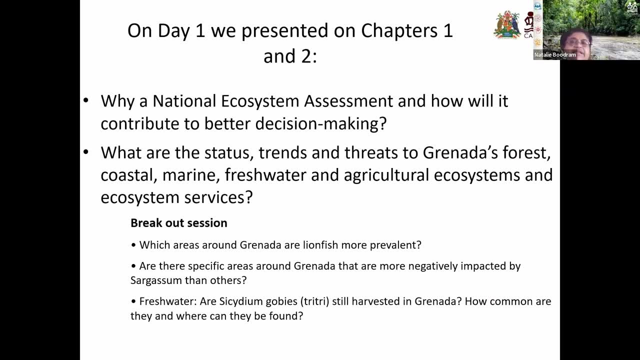 chapters right now. Those will be presented later on in the year or earlier next year. So just to recap, the last time we met we did look at chapters one and two and we explored what were the status, trends and threats to different types of ecosystems, And then we had some breakout. 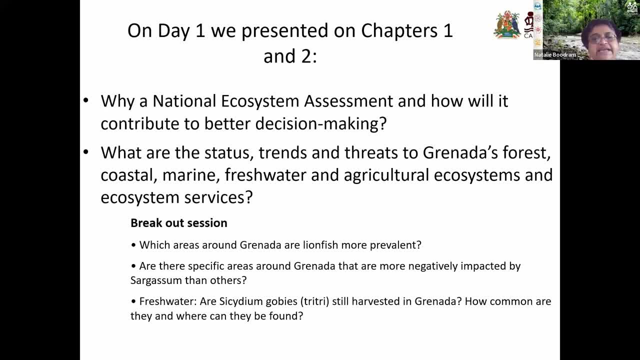 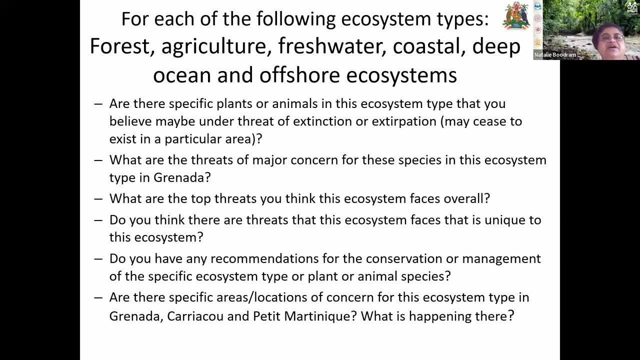 sessions, where some of you were- most of you are actually also here today as well- talked about and gave us input that we will be including in the report, talking about things like Lionfish and Sargassum and TreeTree in particular, And then we also got some input from you in terms of 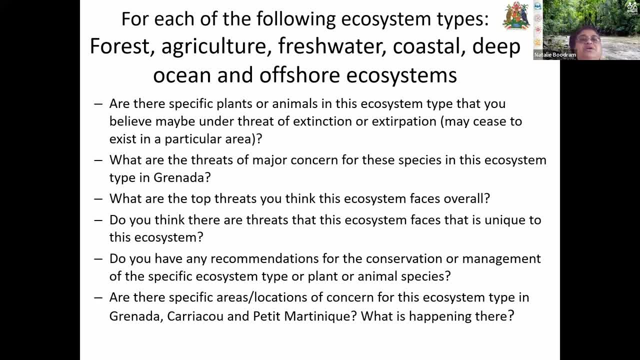 the different ecosystem types And if we were concerned about specific plants or animals within the stripe, what were the threats that were of main concern to you? you know all have any recommendations for the conservation and management of the type of ecosystem or the plant and animal species, and all of this was captured uh reported on in plenary and, as we've 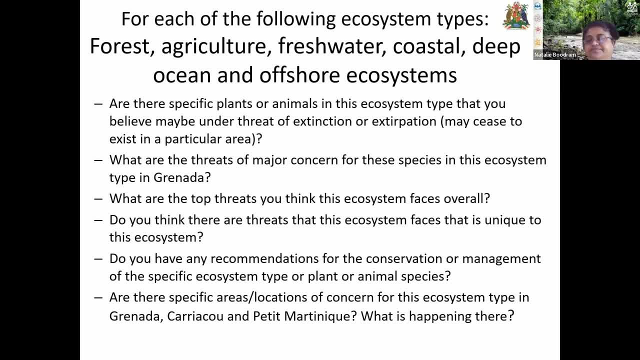 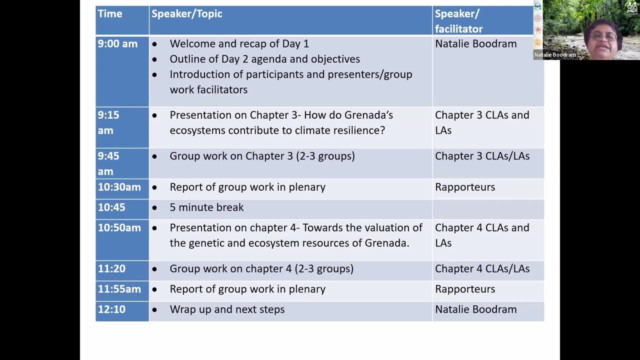 indicated, they will be documented within the chapter as well. okay, so today we will be moving on to chapter three, which is: how do grenada's ecosystems contribute to climate resilience? we'll be doing a little bit of group work on that. um, this chapter may not require as much time as 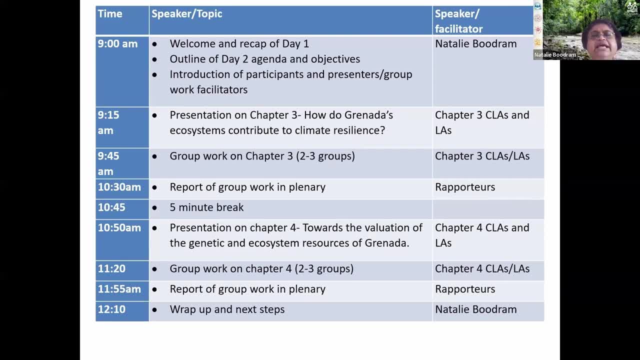 we've allotted. so we're going to do group work for about 30 minutes, then we're going to report on the group work in plenary, then we'll just have a little break present on chapter four, which is on the valuation aspects in particular. uh, do the group work on that and we've assigned the full 45 minutes. 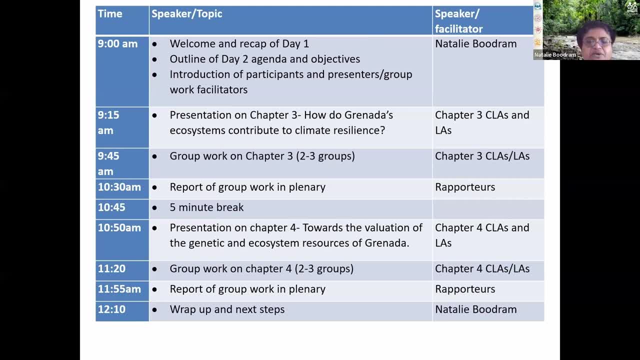 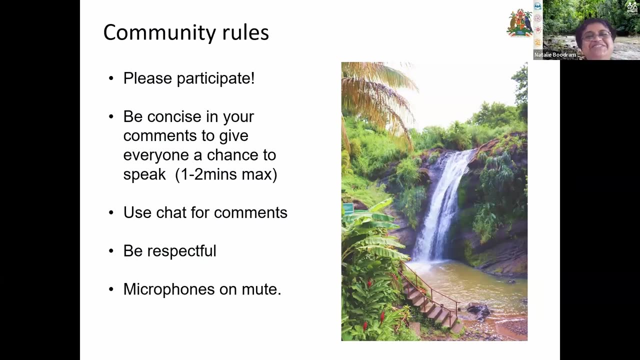 to that chapter because there are a number of questions that the authors would like us to go through. we do our quick report of that and then we do a wrap up, our next steps. so just for today, um, to repeat our usual community rules. of course, we want you all to participate as. 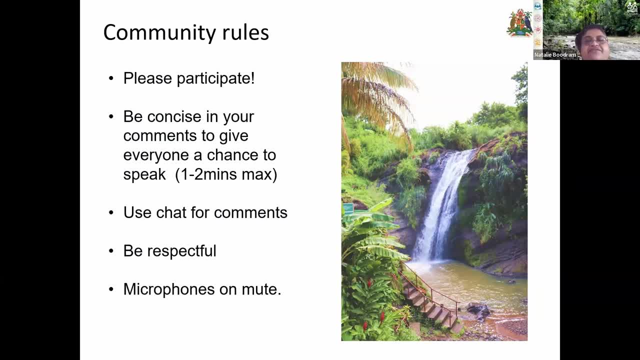 you all have noted, we're very informal, you know. raise your hand, give the comments. uh, just asking, though, that you be concise in your comments, just to make sure everybody has a chance. and if you don't get a chance to speak, um, please use the chat so we can still capture the information. 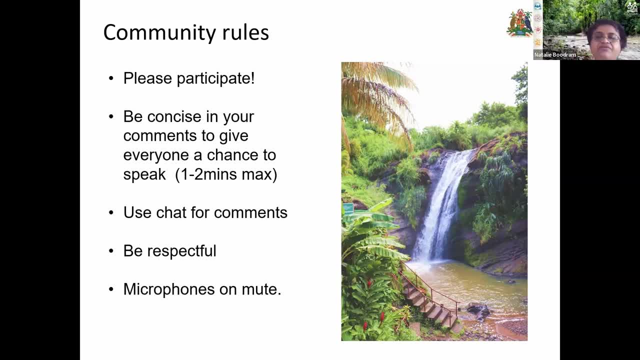 of course, please be respectful to others and keep your microphones on mute when you're not talking, and forgive us if we um mute you just to kind of reduce any kind of background noise. so just to say as well that while we're looking for feedback today, this is 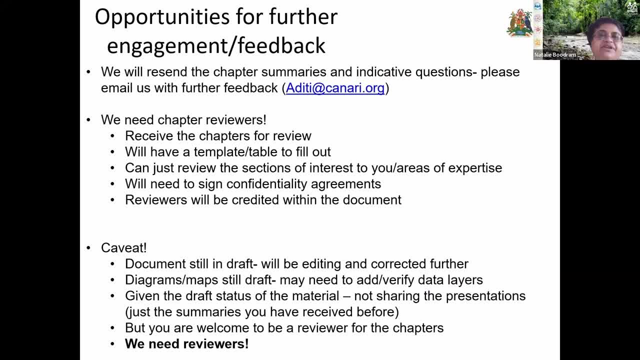 preliminary. uh, we have sent out the chapter summaries and the indicative questions. we will resend them again and then ask you all to please continue to provide feedback. uh, please send us any email feedback that you would like to hear from us, and we will be happy to answer any questions that you might have. 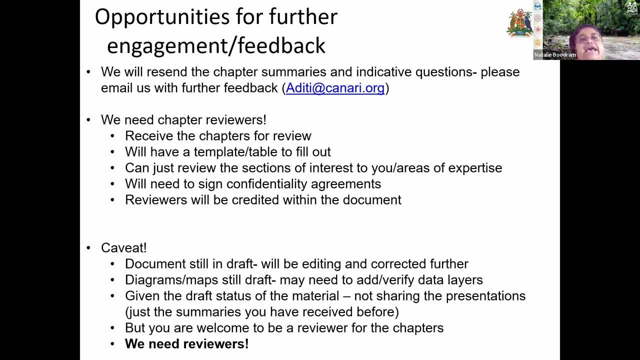 Thank you. So just to say that we are looking for chapter reviewers and thank you to those who have already signed up to be reviewers. So, while we're presenting summaries of the chapters today, uh, if you are a viewer, we will send the full draft chapter to you and there'll be like a little table for you to. 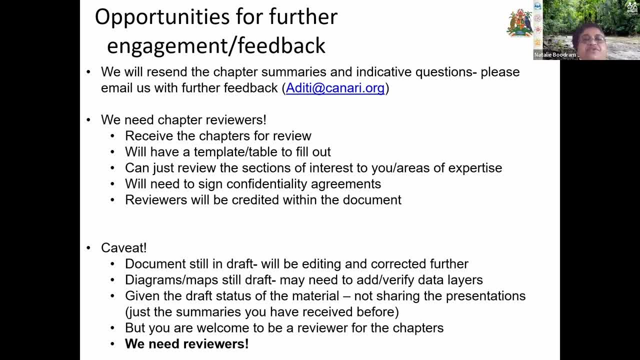 fill out to give specific comments and you don't have to review the entire chapter or all the chapters. you know you could tell us: hey, I'm interested in this particular ecosystem type, or I'm interested in this chapter, and you can do whatever makes sense for you based on your time. 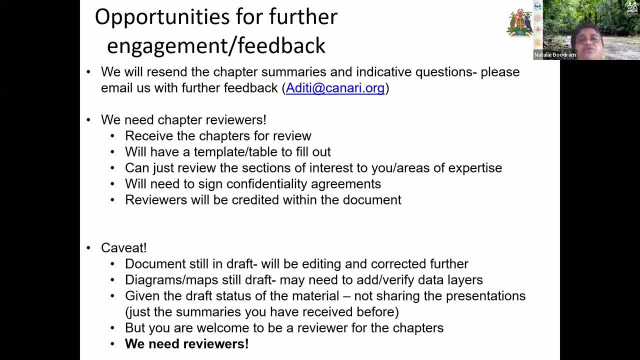 and areas of expertise. Just to say, though, that, if you are participating as a reviewer, we would be grateful if you sign confidentiality agreements just to make sure and protect the material until it is published, which will be, hopefully around March, between March to July. 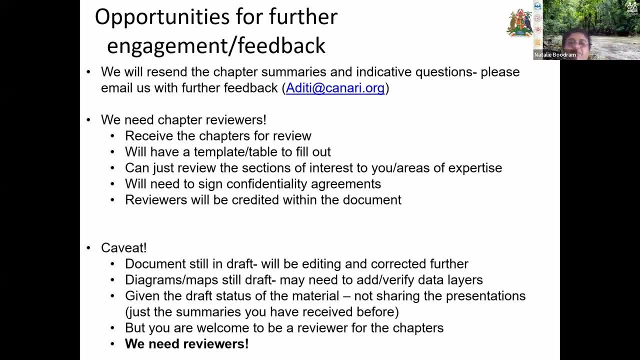 next year And if you are reviewing, please note, we will be crediting you as a reviewer within the document as well. Okay, the document is still draft and we will be relying on you as well to help refine it, including some of the maps. they still need some verification and a 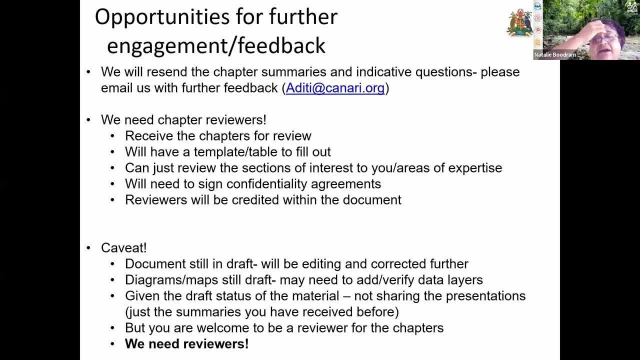 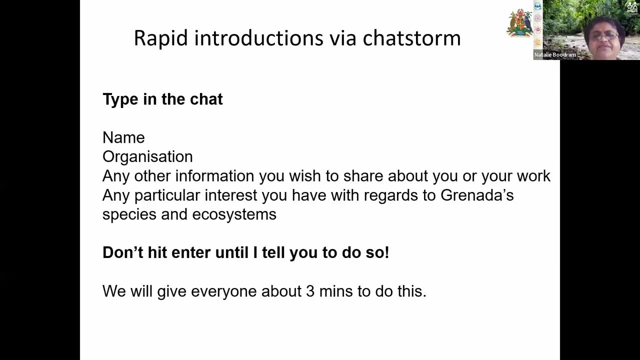 couple with regards to a couple of parameters, And today we are sharing the presentations and the summaries, but you are welcome to review the full chapters once you indicate that you're interested in the document. Okay, so we did a little bit of an informal chat for the people we were less familiar with on the 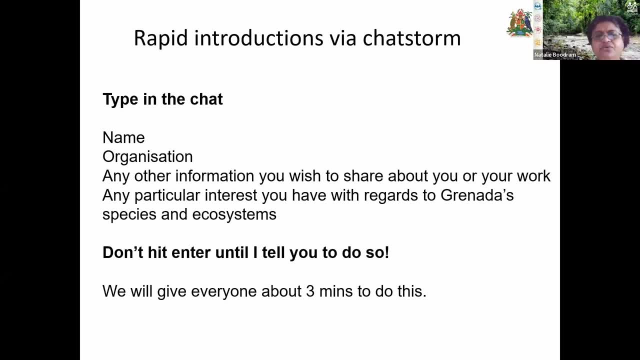 call, But just for people who are new and just give us a quick synopsis, I'll ask for another chat storm again. So if you all can just go to the chat, indicate your name, organization and if there's anything that you want to share about your work, please do so. 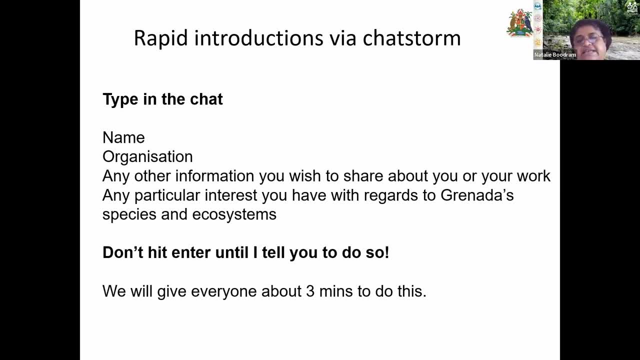 Okay, so if you guys want to do this, and then I'll give you all about a minute or two to do that, And then everybody hits enter And then we just see everybody who is on this workshop. So if you guys can go ahead and do that, 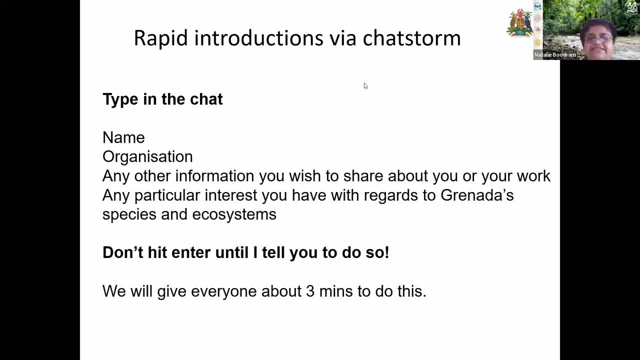 I don't know. just give you guys a little bit of time To do that, can I resolve? you guys go ahead and do that, tuna, So they can see which canary people are there. Alright, so you guys can go ahead and start hitting enter And we can see who's there. 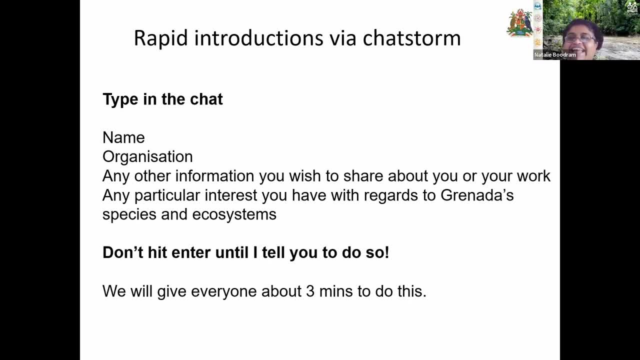 Oh, so we have someone from the solid waste group, Aiden Alright. some of our authors are introducing themselves. Brian Neff, for example, is one of our authors. Karim Anastasio Aaron from Canary Alright. Chris, of course, from St Patrick. 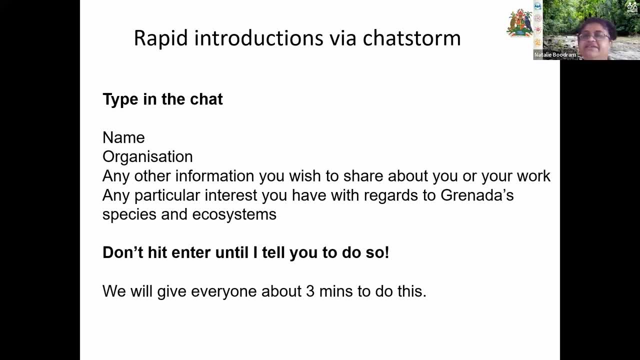 See if I missed anybody. Most of our authors have introduced, And then Ian Blakey from Grenada Green Group as well. Good, Thanks very much. Okay, guys, so we have an idea of the people on this workshop And you know you all can talk to each other. if you all want any contact for any particular group, we can help facilitate that as well. 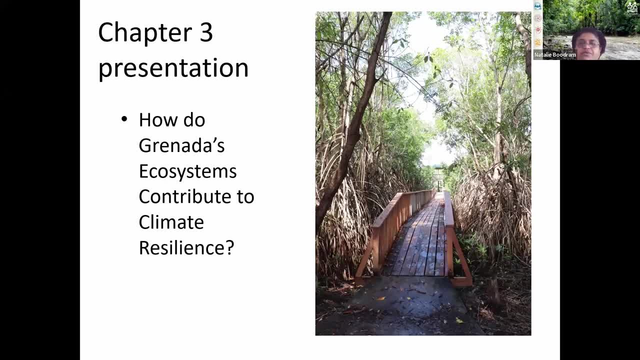 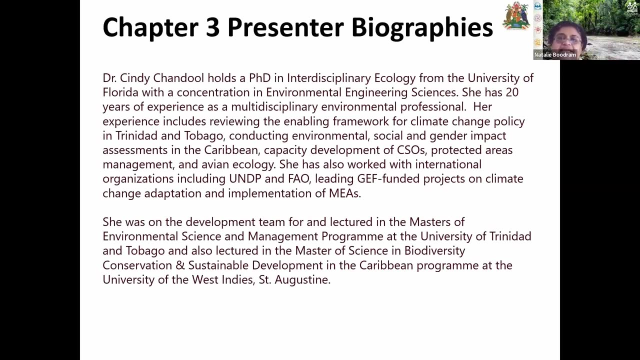 Okie dokes. Alright, so now We're going to go to the presentation of Chapter 3, which is on how Grenada's ecosystems contribute to climate resilience, And that's to indicate that we have one of our coordinating lead authors, Dr Cindy Chandu, who will be doing the presentation. 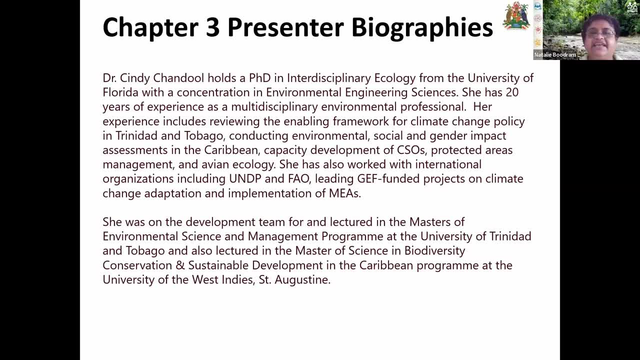 And Cindy like me. actually, Cindy and I did our PhDs together and we both have PhDs in interdisciplinary ecology from the University of Florida, And she has worked on a number of projects, including this one. And she has worked on a number of projects, including this one. 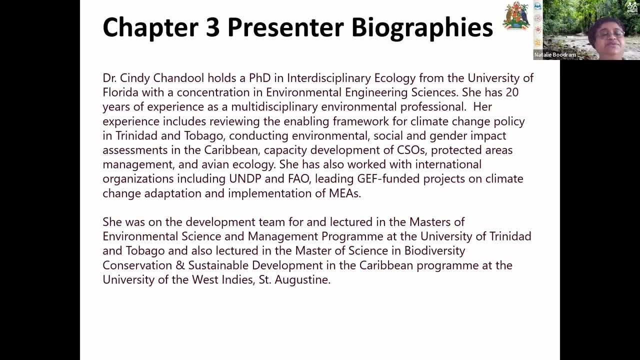 And she has worked on a number of projects, including this one, And she has worked at a multidisciplinary level, doing different kinds of work, including, for example, working on climate change with regards to policy aspects, And she has done a lot of work with regards to environmental, social and gender impact assessments and different projects related to climate change, climate adaptation and the implementation. 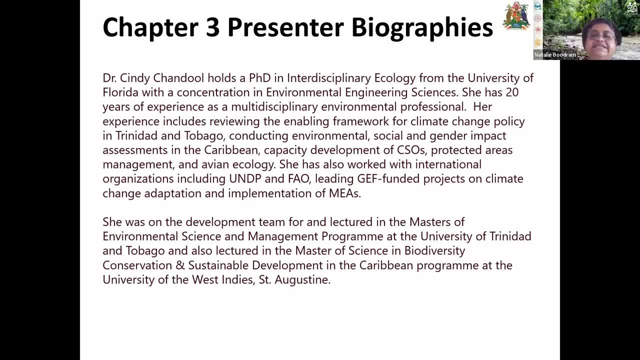 of multilateral environmental agreements, And she has lectured at both the University of Trinidad and Tobago and also in the School of Climate Change at the University of the West Indies. And with that I will turn over to Cindy to begin her. 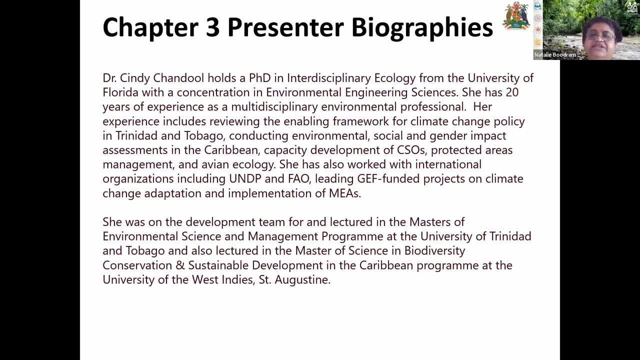 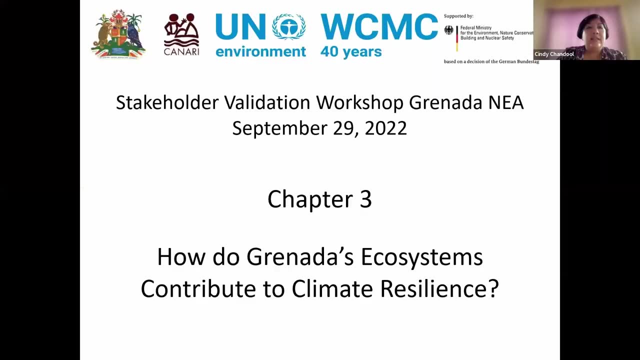 presentation. We will have a question and answer session in plenary before we go to the breakout groups as well. So, Erin, if you could share slides, and Cindy, if you can begin. Great Thanks everyone. Thanks, Natalie, and good morning everyone. I'm happy to be here to present on behalf of our 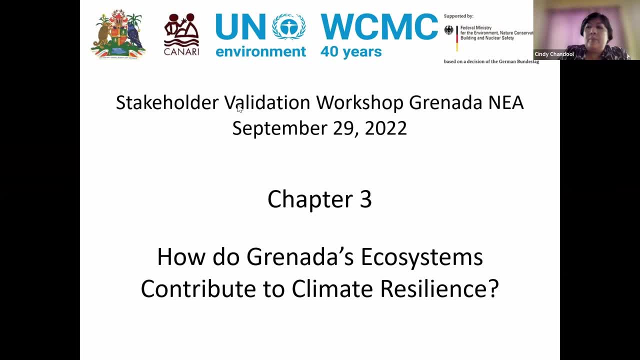 chapter, which has been a lot of work done by all of our lead authors and contributing authors, as well as our fellows. What we looked at in this chapter is how Grenada's ecosystems will contribute, or do contribute, to climate resilience. Next slide. So the first thing we want to do is go. 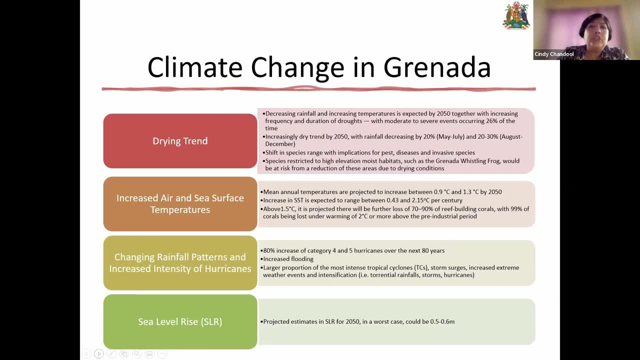 through what climate change in Grenada looks like and is expected To look like in terms of projections. So one of the first things we've read about, and especially in our latest IPCC report, is that there is a drying trend And a lot of these projections deal. 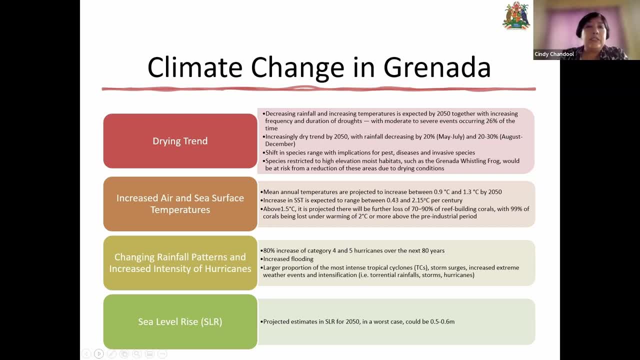 with either the entire Caribbean and, more specifically, the Eastern Caribbean. So we are expecting decreasing rainfall and increasing temperatures by 2050.. This, of course, will lead to increasing frequency and duration, So we are expecting increasing rainfall and increasing precipitation of droughts. We're expecting that there may be moderate to severe events occurring. 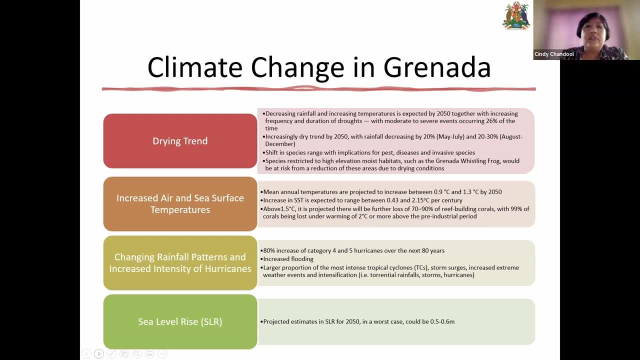 26% of the time, and varying levels of decreasing rainfall over the year, throughout the year. We also expect that there's maybe as much as, depending on the range of increase in temperature, as much as a 60% increase in the number of people who will experience severe water resource stress. 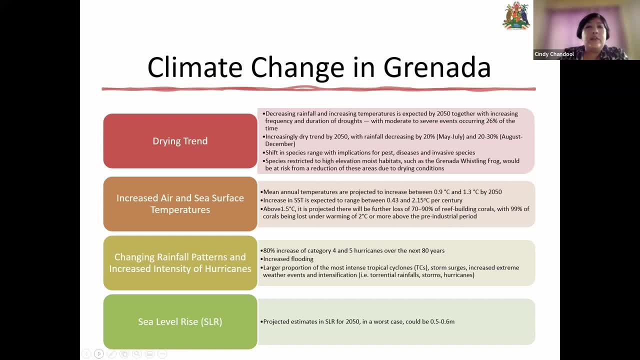 From the range of time between 2043 to 2071 or so. This, of course, brings with it an increased risk of wildfires, something that we in the Caribbean already deal with. So wildfires may, of course, impact ecosystems, reducing our zones of rainforests, migrating species to higher elevations. 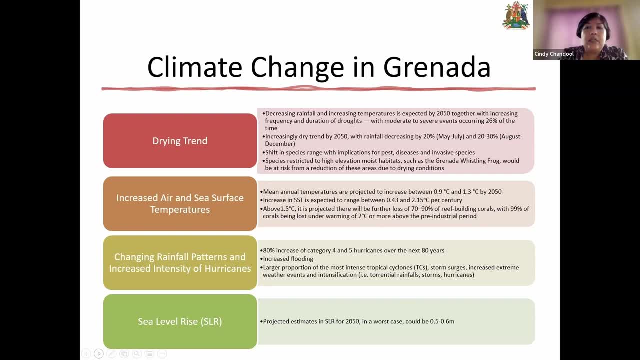 leading to increased soil erosion. Of course, pollinators are a serious concern. Wild pollinators may be affected as well, So we're expecting that there's going to be an increase in the number of of wildfires maybe affected as well, And our already stressed freshwater systems will continue. 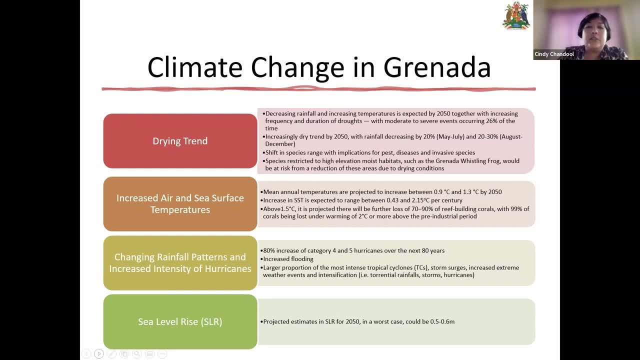 to face additional stresses. We already have water stress because of pressure from normal human activities being population growth, expansion in our tourism sectors, And so we will expect with these droughts, there will, of course, be reduced groundwater recharge, our flows in our rivers will be lower, may even go lead to increased siltation in dams and so forth. 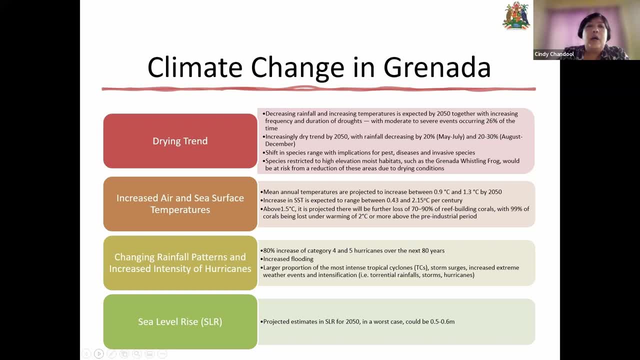 So this is of serious concern. Our species, especially species such as the Grenada whistling frog, could be at risk because their habitat area will reduce due to drying conditions. We will talk about that when I speak about some of the terrestrial effects. 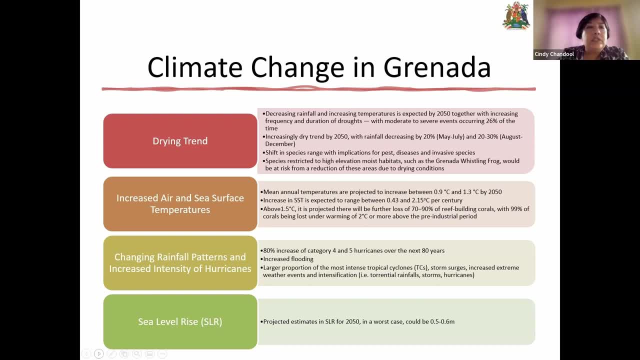 We're also expecting increased both air, as I talked about before, and sea surface temperatures, And so we're expecting between, for the Caribbean, between 0.9 and 1.3 degrees Celsius by 2050.. Sea surface temperature is expected to increase anywhere between 0.43 and 2.15 degrees Celsius. 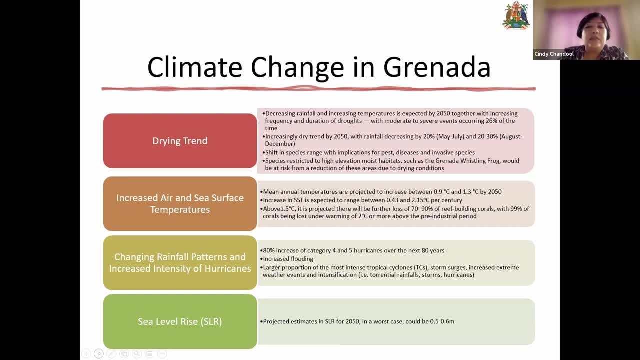 per century, Past sea surface temperatures have been: from 1981 to 2019, we've seen about 0.17 degrees Celsius per decade within the Caribbean. If we continue to see these kinds of temperature increases, we are expecting organisms such as 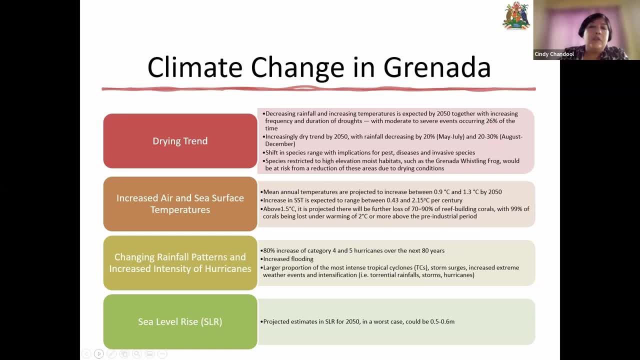 corals. we will have loss of reef building corals in particular and potentially a loss of 99% of corals In general. we are expecting and we've seen some of this. we're seeing the effects, of course, the devastating effects of Hurricane Ian right now in Florida. We are expecting in 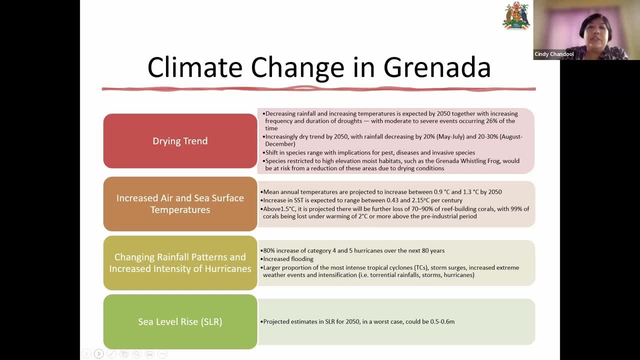 the Caribbean as well. changing patterns, increased intensity, increases in intensity of the number of category four and category five hurricanes that will be over the next 80 years or so. Increased flooding is, of course, a serious concern. We are already seeing increased flood risk. when we expand for urbanization, We are removing 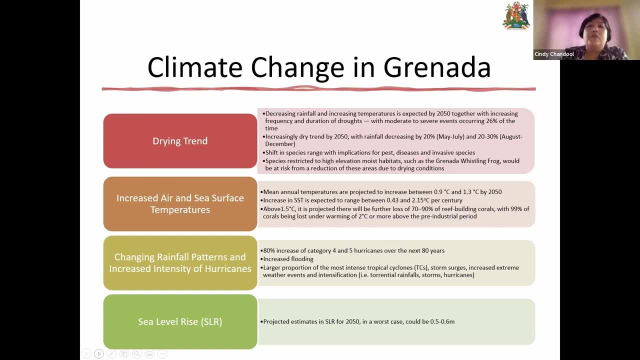 you know, if we remove forests and vegetation of cover and of course we're increasing concrete surfaces, the impermeable surfaces, so we're reducing infiltration into the soil, So a lot more surface runoff and so on. Again speaking about hurricanes, when we looked at after Hurricane Ivan, there was a lot of damage. 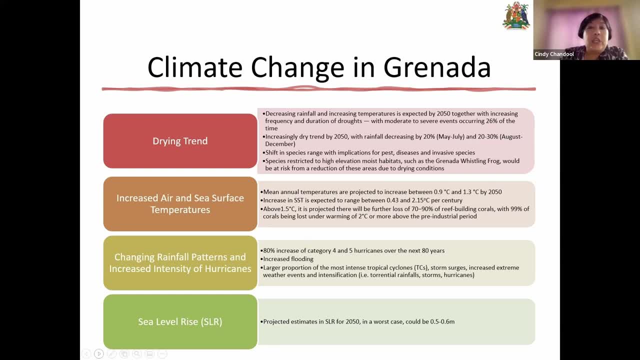 to the vegetation areas. the watersheds were severely affected. We, you know, there's a lot of agriculture, and so that was affected. Estimates for the damage to Grenada from this hurricane was a little more than 1 billion US dollars, which is, of course, quite significant. 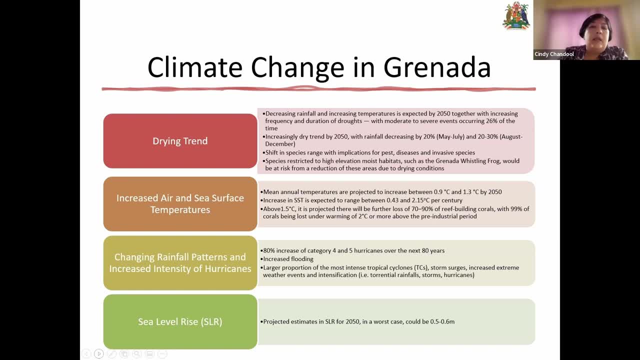 Sea level rise is also expected. Projected estimates, again- and this is a worst case scenario- could be between 0.5 to 0.6 meters. As much as that. Besides our natural ecosystems, we also have to be aware of our built areas, where. 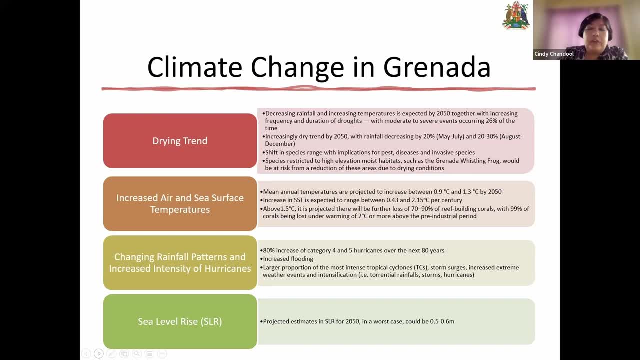 resorts, our housing areas in low-lying areas and so on will be affected. If we have as much as a one meter sea level rise in the Caribbean, it's expected at about 29 percent of resorts- sorry, as well as you know- would be affected. We would have damage, et cetera, et cetera. 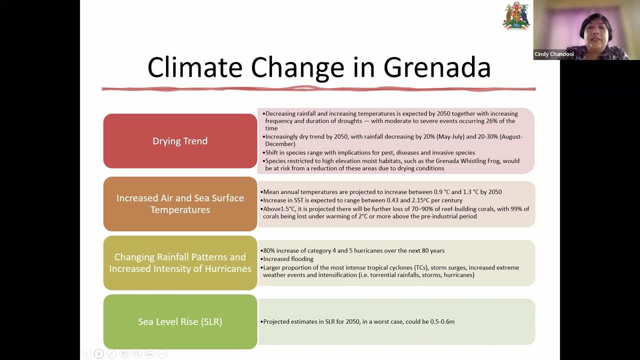 For Grenada specifically, at such a high sea level rise, if we have as much as one meter, we could have something like one percent of total land, three percent of agricultural land, eight percent of total nesting sites. So these are some of the figures that you know. 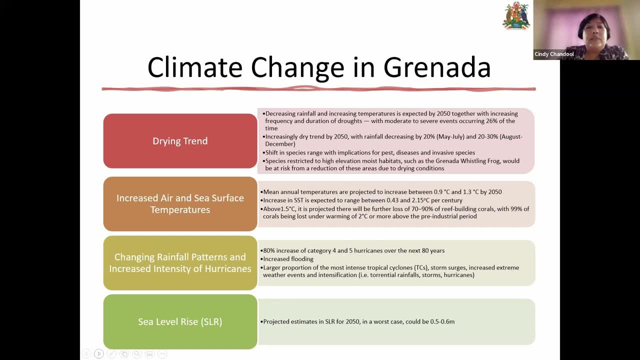 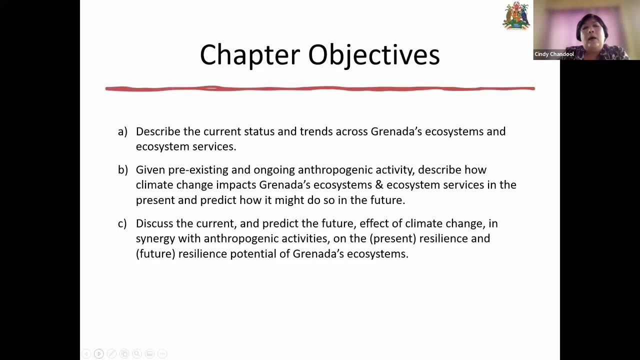 just to summarize some of what's in our chapter. this is the kinds of effects we're looking at. So, being that we are expecting serious repercussions from climate change and serious impacts of climate change. Next slide, Tans, We are looking for our chapter. what we're. 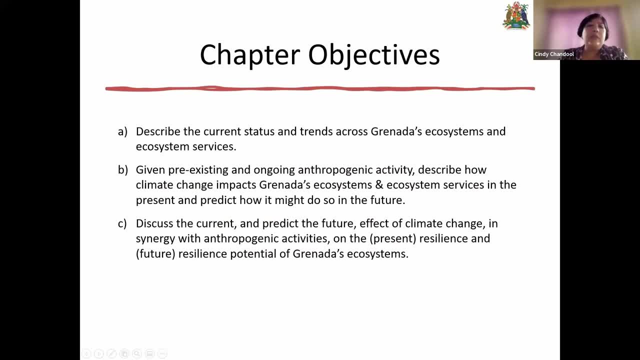 trying to do is describe these trends, describe the status and the current status of these ecosystems. We are looking for what these will be turning into in the British Columbia- Clean and Sustainable Planилли, here near tiger이다, and we are also looking what impacts will we have with relative 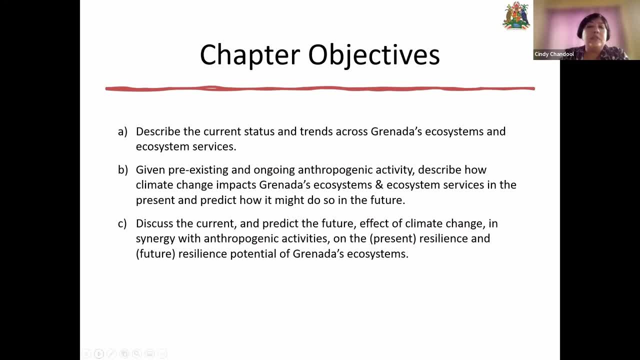 to those risks And then what we can build upon that will be the kinds of impacts that, In addition to that, given that we already have human activity, human impacts, how would these climate change impacts continue to affect Grenada's ecosystems and services? and ecosystem services. how will they, how they're affecting it now, And especially variety, to predict what may happen in the future and also to discuss the current and, of course, predict the future effect of climate change. but but to it, also discuss the current and, of course, predict the future effect of climate change, but also measure the range of efect ofiska or environmental activity, or social worker, możCP, or Looking at the context of climate online as well, as we're beginning to base in, I think, new family infrastructure, When the last five chapters in field space time covered. our studies are currently 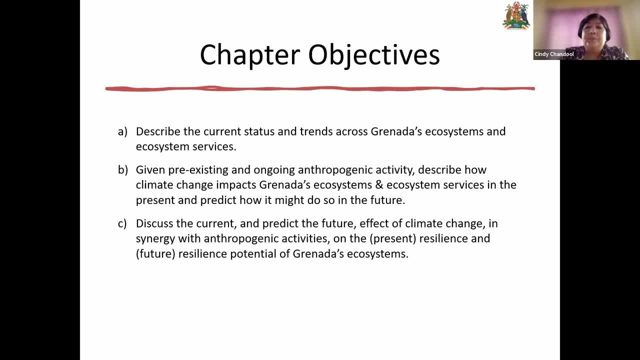 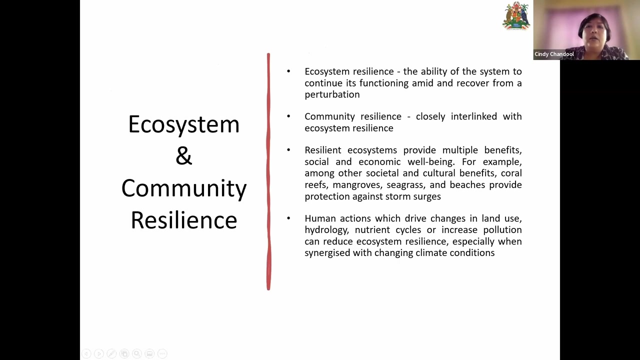 change. but we're looking at resilience, the effects on the resilience of our Veneta's ecosystems, and what are the future. look at the future resilience of the ecosystems as we may proceed. So what is resilience? We talk a lot about ecosystem and community resilience throughout these discussions, So let's set the context in. 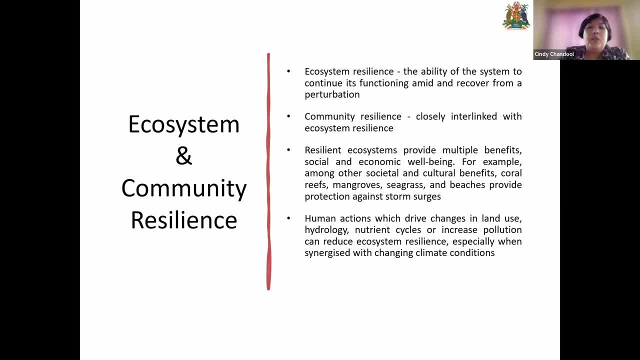 terms of what are we talking about? So the ecosystem resilience. when we refer to this particular aspect, we're talking about the ability of these systems to function in the face of perturbation. Basically for this, and specifically in this case, we're looking at it in the face of 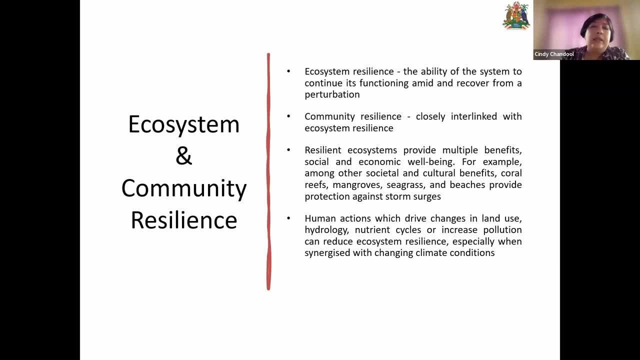 climate change. So how will, in layman's terms, how will these ecosystems bounce back, How will they recover if they're affected? And this term resilience is used for all effects, but, as I said, we're looking specifically today at the resilience to climate change In terms of community. 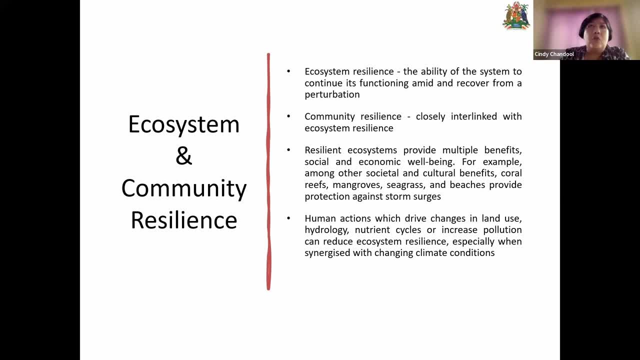 resilience we look at. of course, our communities are very dependent on ecosystems and their services, and our friends in the evaluation chapter are very dependent on them. So we're looking at resilience to climate change. So we're looking specifically today at the resilience to climate. 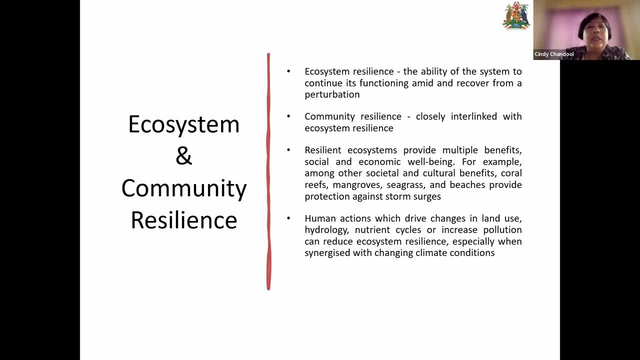 change And our friends in the evaluation chapter will point these out and the we need the community will be affected by the system. So community resilience is closely tied to our community resilience. Resilient ecosystem, resilient ecosystems- we all of our multiple benefits that we went. 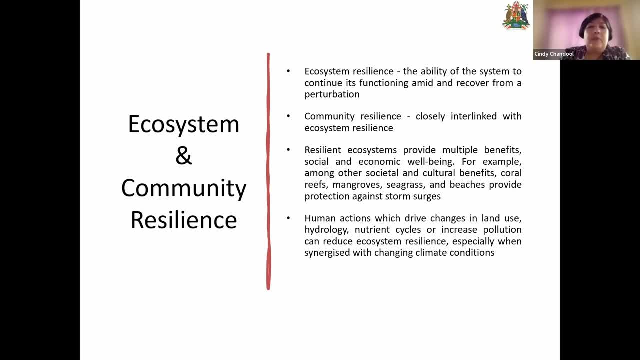 through in our previous workshop. For example, you know coral reefs, mangroves, seagrass- all of these provide protection against storm surges. This is just one example of how our ecosystem, we example of how these ecosystems will improve our- will assist our resilience to climate change. 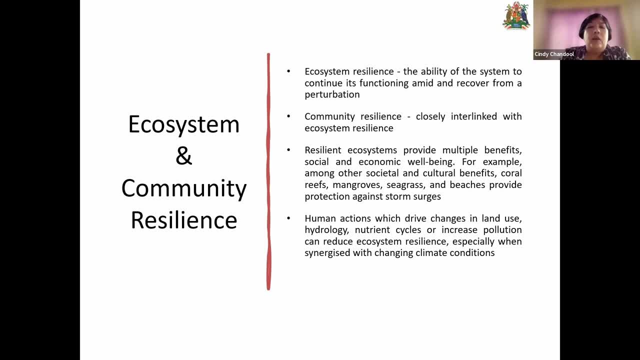 impacts. There are many, many more. of course. We already face a lot of changes due to our human activity. We're already seeing changes in land use, pollution, etc. We have. these may already be reducing our ecosystem resilience and we need to be aware of that With changing climate. 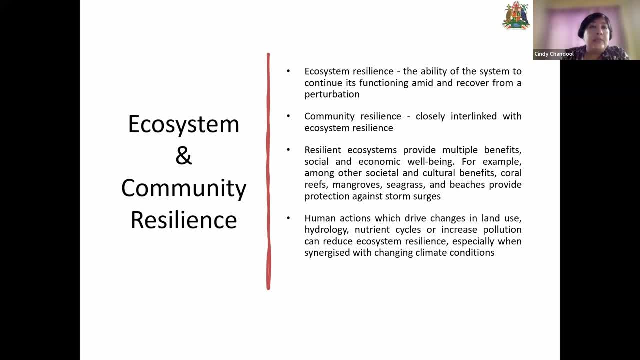 conditions, these effects can be exacerbated. So we want to enhance our ecosystem resilience and build our ecosystems to a point where- and continue to protect them- where they will continue to provide ecosystem services And, as I said, one example is storm surges- continue to. 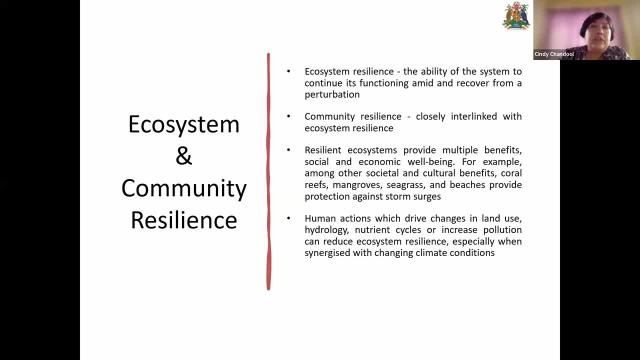 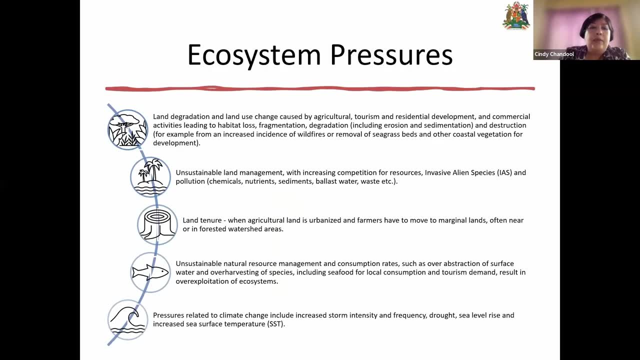 give us some level of resilience and protection against climate change. Next slide: So when we looked at ecosystem pressures, we- this is a summary of each. it was analyzed for each chapter sorry and for each ecosystem, not each chapter sorry for each ecosystem. So we looked. 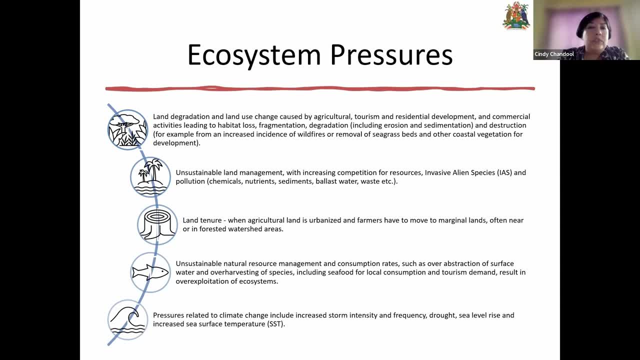 at terrestrial, agricultural, marine, coastal, freshwater, And this is a summary of all of the various pressures that were found that affect our Renata's ecosystems. So one important one is land use and land degradation. So we spoke about that, that we are changing our land for various reasons: agriculture, tourism, residential, commercial. 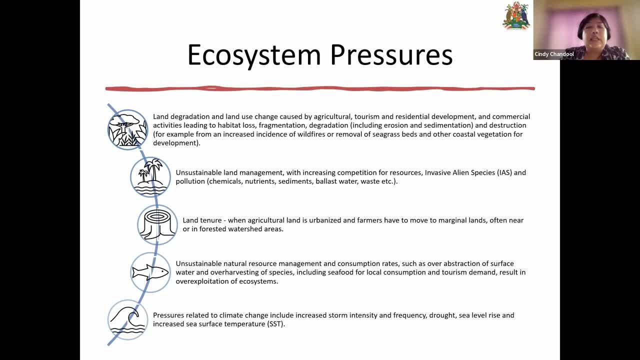 All of these leads to, of course, erosion, things like erosion degradation. one of the concerns, of course, is fragmentation of our habitats and loss of habitats. Another important pressure is unsustainable land management, which may lead to issues such as invasive species. 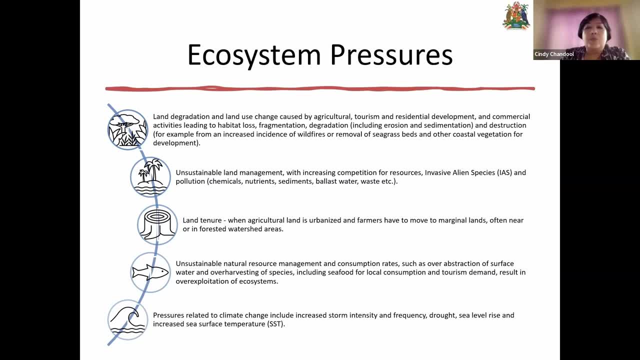 pollution from chemicals, nutrients, ballast water, et cetera. Land tenure is a pressure because when we have agricultural land being used for urbanization, farmers may move to more marginal lands, affecting watershed areas, et cetera. Unsustainable natural resource management is important as a pressure, as well as our consumption of resources. 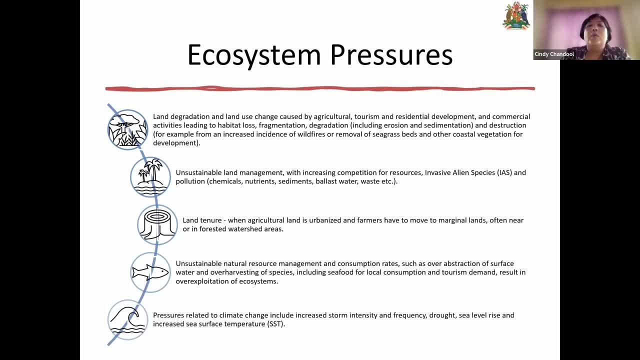 So we may have issues such as over-abstraction of water. We know there's over-harvesting of species such as seafood, So generally over-exploitation of our ecosystems and, of course, the pressures that I've spoken about, those climate change impacts that we will be experiencing. 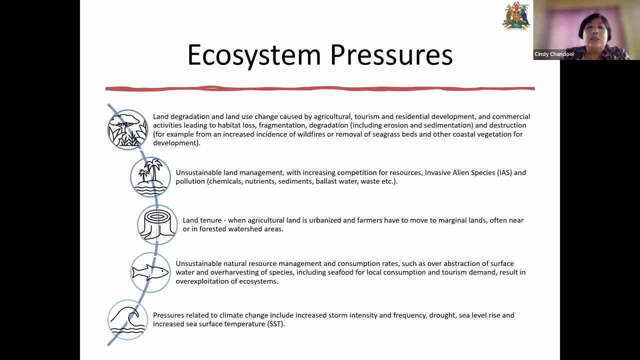 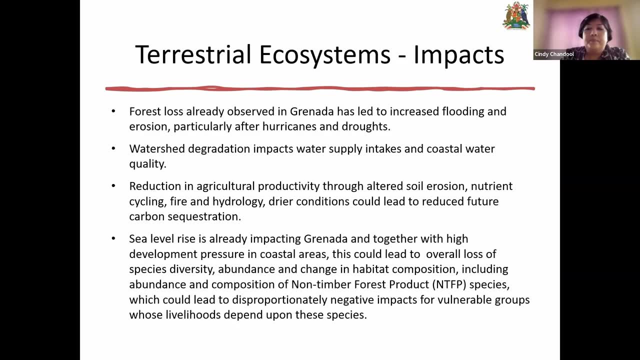 So things like storm intensity, drought, et cetera, Are considered pressures that we will be facing as well Next slide. So we've gone through each of these ecosystems, as I said, and in the face of these pressures, we've looked at what may be the impacts on each of the systems. 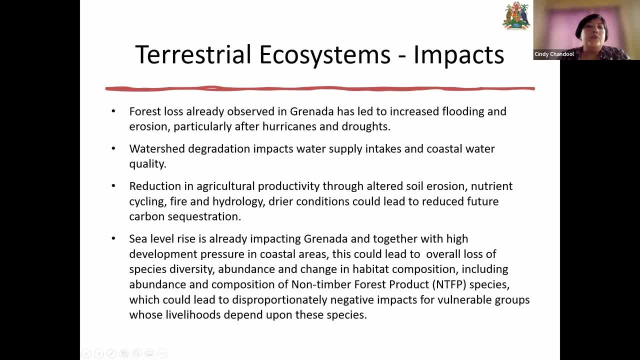 So in terms of terrestrial ecosystems. so including, you know, all of our different types of forests: dry forests, rain forests, et cetera, et cetera. forest loss has already been observed And we know this, Both from issues such as the hurricanes, of course, as well as human intervention. 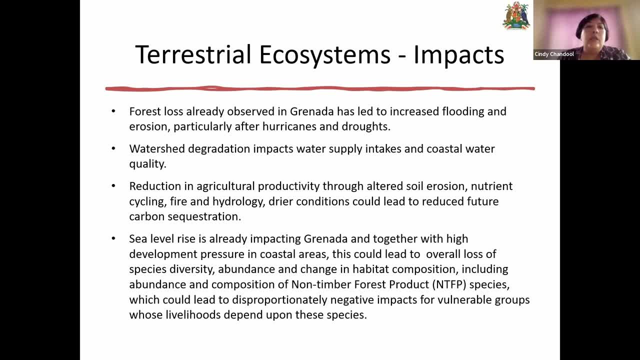 We've already experienced increased flooding erosion, and we're only going to see more of this in the face of potential increases in hurricanes and droughts. The watersheds themselves are facing degradation and we are going to be faced with increasing requirements for water resources. 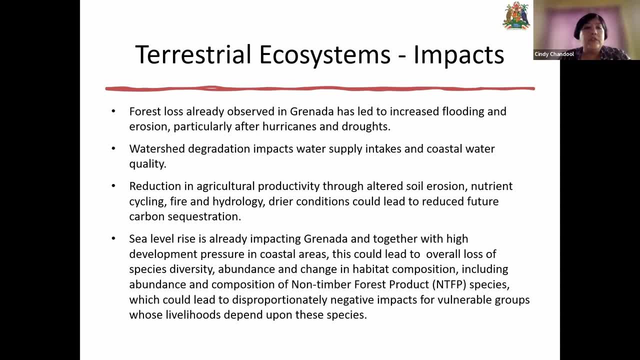 Coastal water, of course, is also an issue. the quality of such water, which is also very important, of course, for our tourism product, Agricultural productivity, is going to be affected. We may see issues such as soil erosion leading to- sorry, the chat is just popping up on me- leading to dry conditions, nutrient cycling, fire, etc. 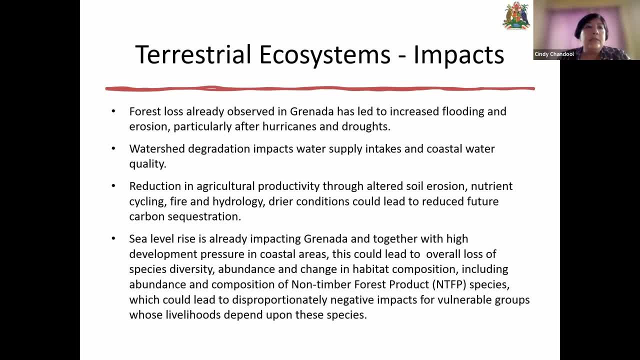 Sea level rise. as I mentioned before when we looked at the impacts, the general changes due to climate change, we will see. you know there's going to continue to be pressure on our coastal areas where a lot of our tourism products are going to be affected, So we may see issues such as: 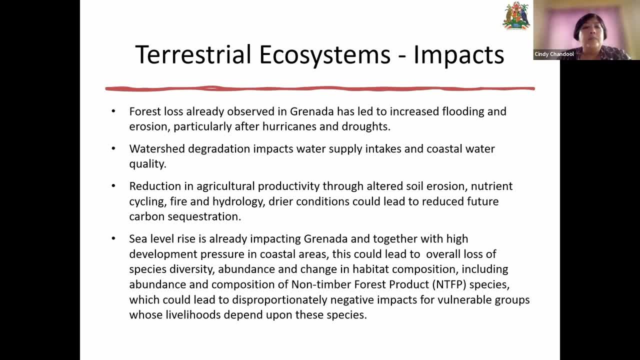 and development is occurring, Things like species diversity, our actual composition of our habitats. you know, even some of our non-timber forest species will be affected, So you know things used for horticultural products, our herbal medicines and so on, Always being aware that. 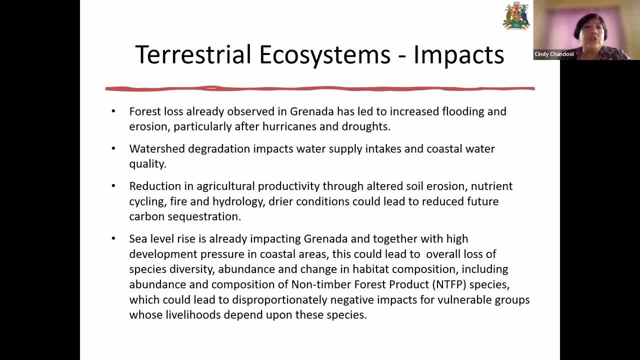 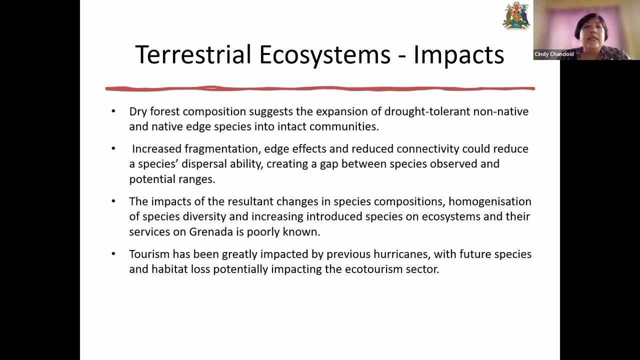 many of these impacts may be disproportionate, affecting our vulnerable groups, And this is something we need to always be aware of as we look at impacts and possible solutions and interventions. Next slide: So we talked about fragmentation. We may be seeing more drought-tolerant species. 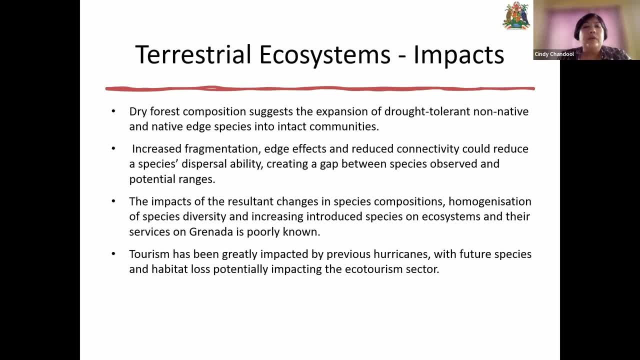 taking over our, our terrestrial ecosystems. We're We're looking at homogenization of our species, as I said, when these types of species take over. So I know of course we have to consider that our ecotourism product may be impacted. 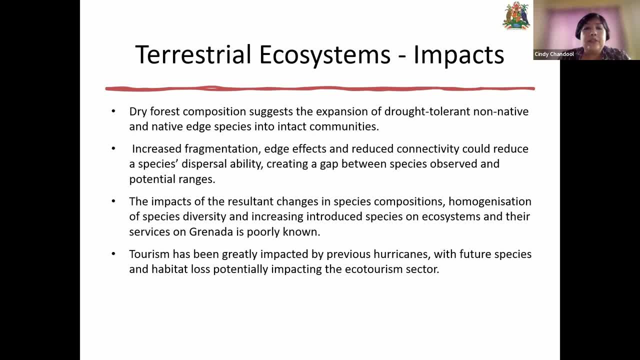 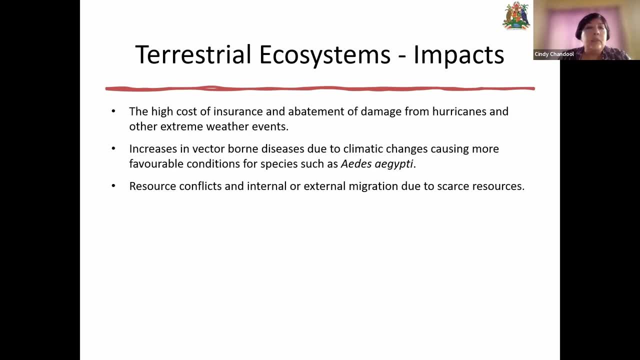 due from past impacts and perhaps future potential habitat changes as well. Next slide: One of the human impacts we are seeing is that the high cost of insurance and damage from hurricanes and extreme weather events. Any increases in these types of weather events, of course, will provide a further burden on 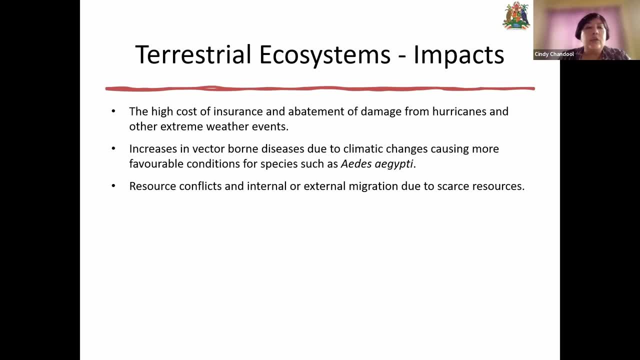 citizens and the costs and economics of that. Vector-borne diseases are a concern and, of course, species such as Aedes aegypti- other things that we Impacts that we know We need to consider potentially internal or external migration of our human resource. 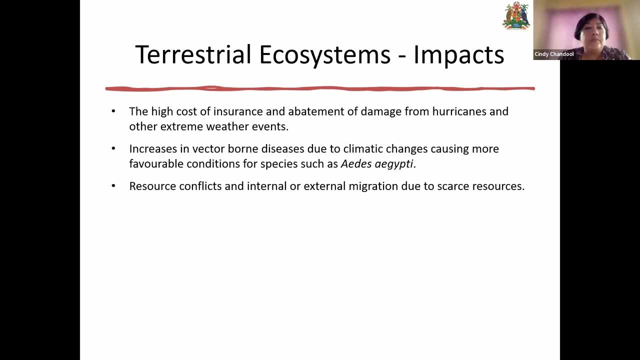 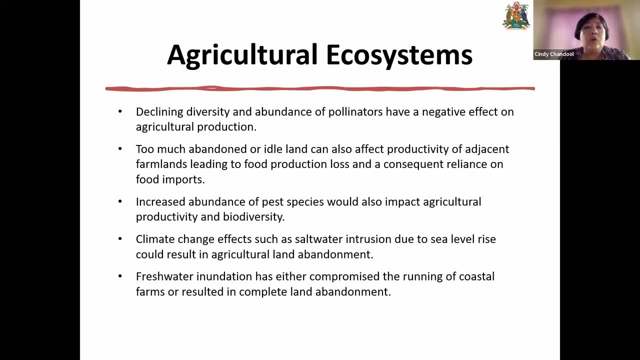 and our people due to scarce resources. So we're looking at changes in- That's okay, You can go ahead- Changes in ecosystems, but also, of course, we have to always consider the impacts on our people as well. Agricultural ecosystems: we talked about pollinators early on, so we have to consider that there. 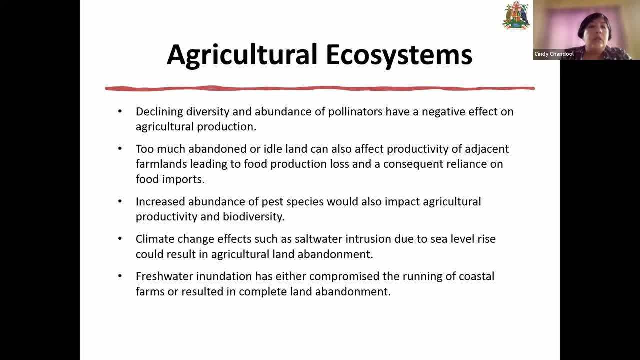 may be a serious effect on our production. If we see land being abandoned due to changes in productivity, we will have an effect on food production. Pest species may increase, changing again our biodiversity as well as our productivity within the agricultural sector. 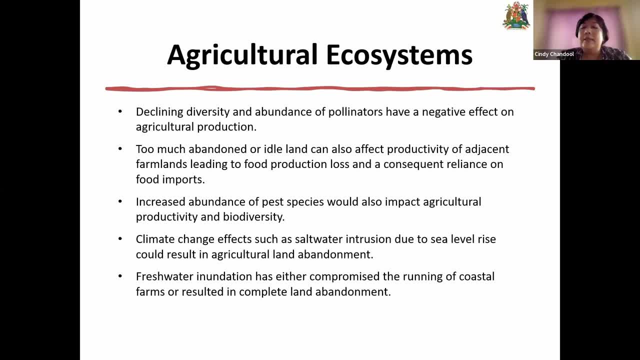 Saltwater intrusion may Will be a concern as, again, due to sea level rise, We may We may see land being abandoned as saltwater continues to intrude. Freshwater inundation due to flooding may also compromise our coastal farms and, again, 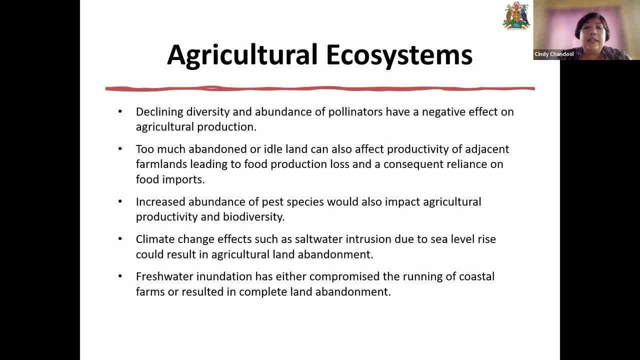 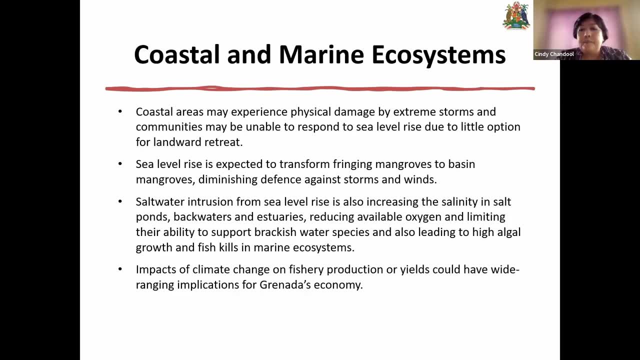 may result in completely leaving the land because you just It just isn't going to be functional or productive anymore. Next slide, So coastal marine ecosystems. This is a major concern to our small islands within the Caribbean Coastal areas. physical damage is, of course, the first thing you think about, because these 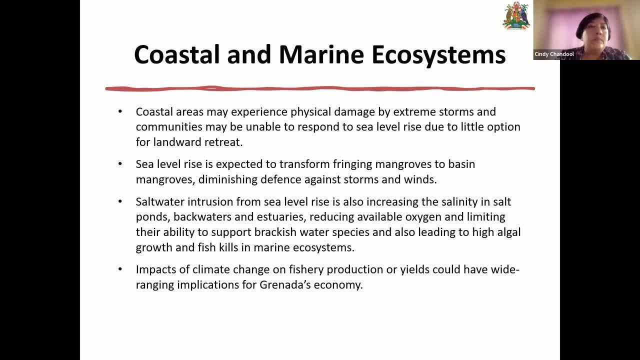 storms et cetera. sea level rise: there's not much land space where we're going to go, so little option for moving inward, little option for migrating, sometimes within the island. Sea level rise will also affect mangroves. We've got to be careful. 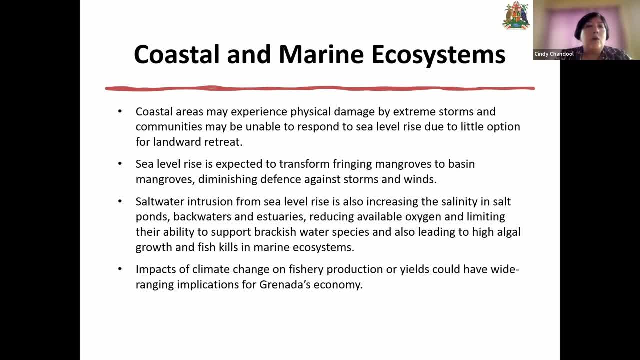 We've got to be careful. We've got to be careful, And we spoke about how important these are to protect us against storms and winds. Saltwater intrusion is a serious concern. We talked about its effect on agricultural systems, but it will also affect our existing. 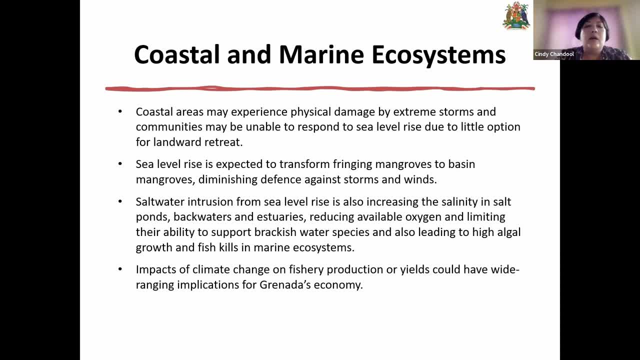 species within the coastal, marine, Coastal areas, reducing ability of oxygen, increasing the salinity of all of our other ecosystems within the area: Estuary, Estuary sorry And salt ponds, et cetera. It may even lead to fish kills in some cases. 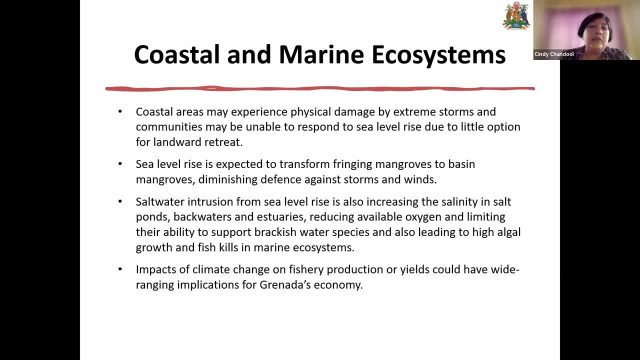 Anything that affects these fish. the fish will affect, of course, our fishery production yields And, as I said, we always have to think about, in addition to the ecosystems, how is this also going to affect people and the economy, and these would have wide-ranging implications. 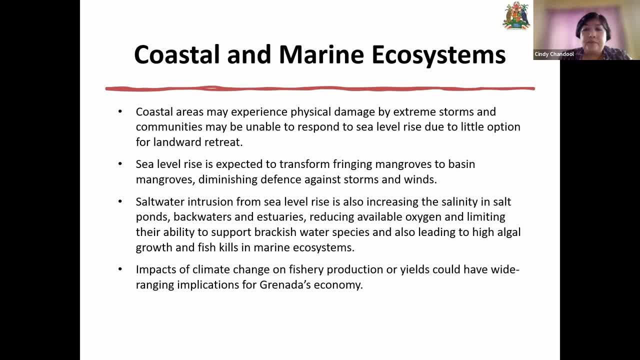 for the Grenadian economy as well. Thank you, Thank you. Thank you for your wonderful question. Thank you, Thank you, Thank you, And I'll keep talking about that in the next session. We'll see about that in a few minutes or two, but we'll take a look at it as well. 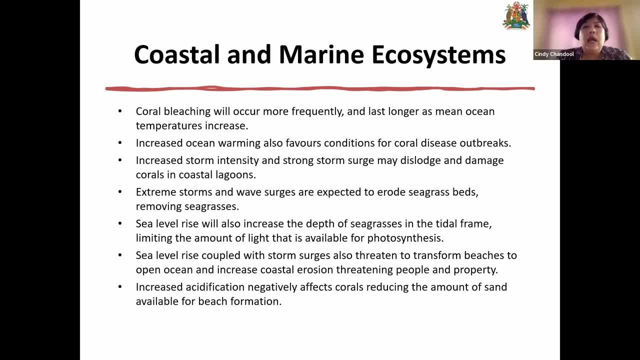 So in terms of corals, the Caribbean reefs in general have been warmed by about 0.18 degrees Celsius per decade since about 1988 or so, so the Eastern Caribbean has even been higher. It's expected that we may have additional warming of about 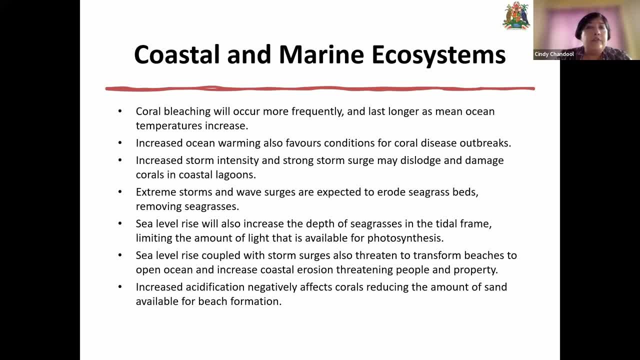 Over 10,000.. coral ecosystems by about 1.5 degrees Celsius on average by 2100.. This, of course, will also lead to coral disease. We are seeing incidences of increased frequency of coral bleaching and even the increase in storms. actually, you know, physically damage our corals. 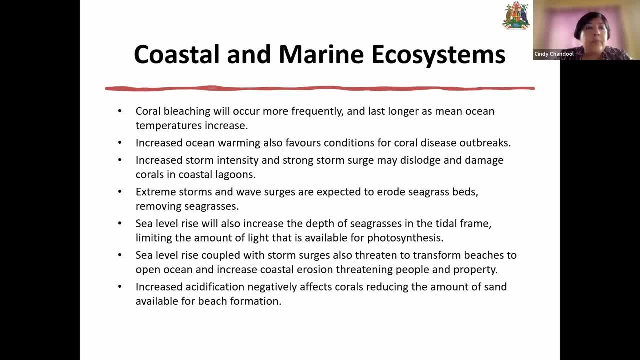 It also may erode seagrass beds And with sea level rise, we also have the additional issue of increasing the depth of seagrasses, which require, of course, a certain amount of light for photosynthesis. When we increase those levels, they will not be able to photosynthesize properly. 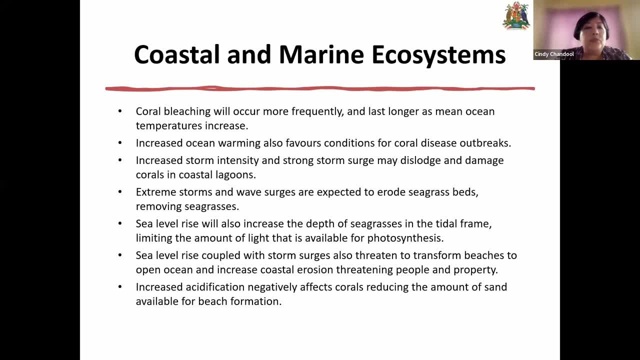 effectively, sorry. So both of these issues- storm surges, sea level rise- will also have a negative impact on our corals. And so you know we are seeing. you know we are also seeing that the sea level rise in the west and it will also affect our coastal systems. 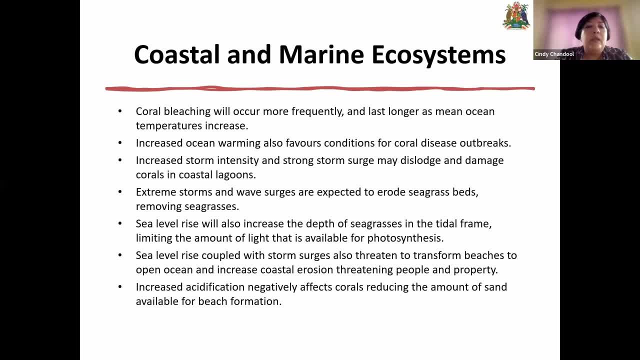 leading to coastal erosion, threatening people and property, And we talked about acidification affecting corals and effect of a lead-on effect of the corals being reduced themselves also affects beach formation because of course, the corals produce the sands- in Grenada a large amount of it, So this also affects. our beach formation, And so this is also a sign of, of course, the sea level rise in the west, And so this is also a sign of, of course, the sea level rise in the west, And so this is also a sign of, of course. 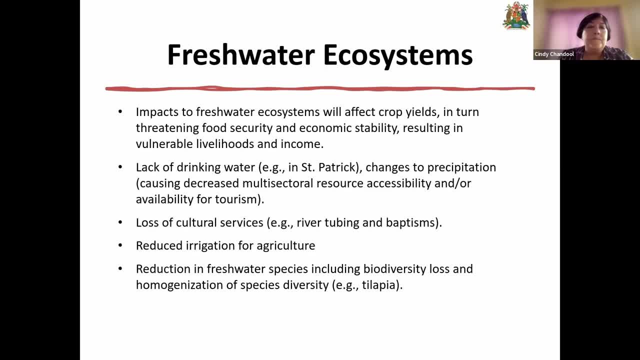 beach formation, In terms of freshwater ecosystems, our impacts are expected to affect our crop yields. we talked about, I spoke about earlier, the, basically the fact that you know we'll either: we'll have flooding, yes, but we will also have drought. So our 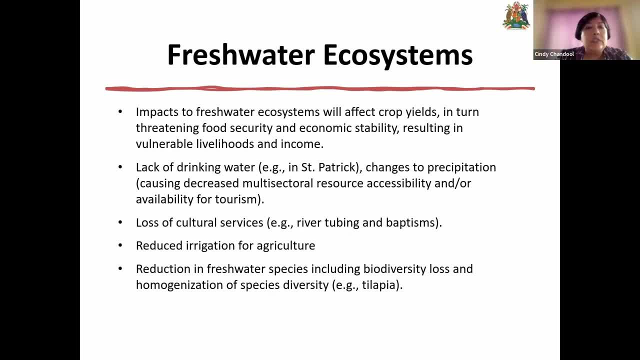 freshwater ecosystems are going to be affected And, of course, this in turn affects crop yields and, very particularly, food security, and leading to a lot of impacts on our livelihood, the livelihoods and incomes of farmers. in Grenada, Lack of drinking water is a primary concern. changes in 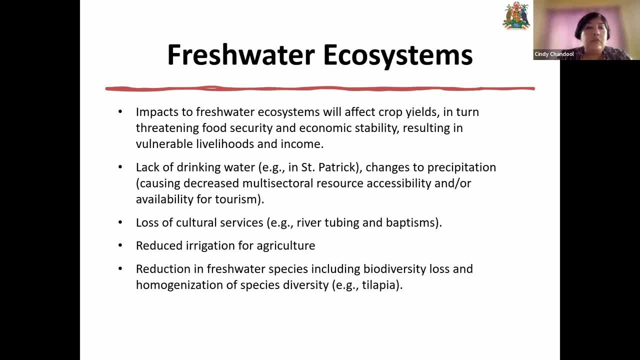 precipitation, variable amounts of rainfall, etc. will continue To have serious repercussions, And already there is. of course, you have to remember, there's a tourism demand and the tourism demand is going to most likely increase, So we will have a 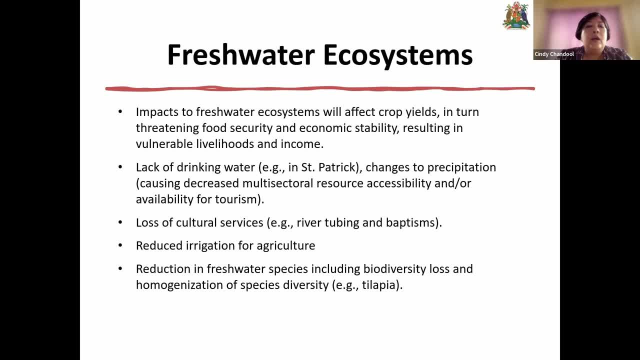 challenge for accessing sufficient drinking water, We have to consider our cultural services as well. Water is very much tied into the Caribbean way of life, both for recreation and for religious and cultural activity, So these are concerns when our freshwater ecosystems are affected. We talked about 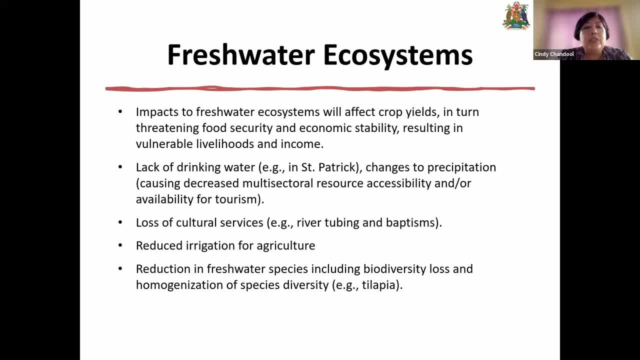 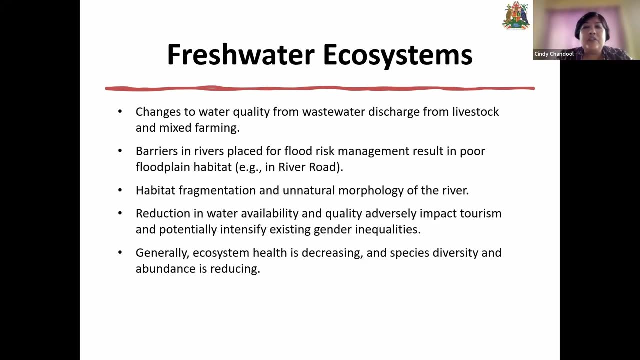 agriculture already, and the primary concern of biodiversity loss, leading to homogenizing and also homogenization of diversity. Any of our- you can go ahead. Any of our- these degradations of our systems, our terrestrial, freshwater, marine systems, continues to amplify our already vulnerable. 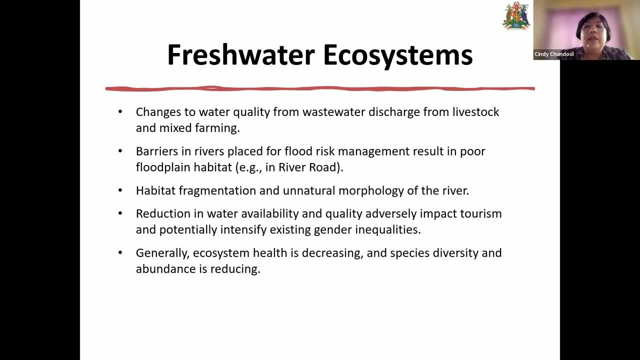 population, Our already vulnerable islands and our people. So you know, any degradation in our ecosystems that continues to affect these resources that we rely on will continue to impact our settlements, our infrastructure, our food, our water security, our health, culture, migration and economies, Other systems, other impacts. 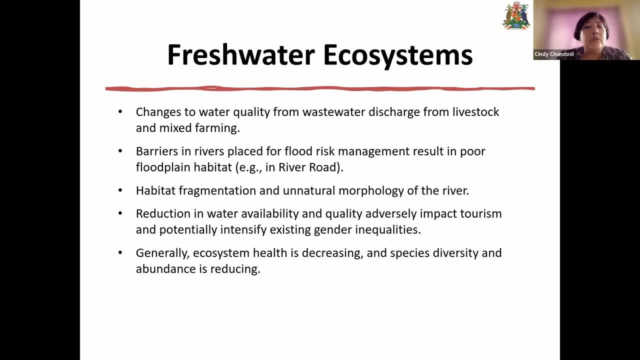 sorry- are changing the water quality, So when we have wastewater, discharge from livestock and so forth, changing our water quality. physical barriers, when you place them for flood risk management, may also result in affecting the habitats within the flood plains, So that changes the morphology of the. 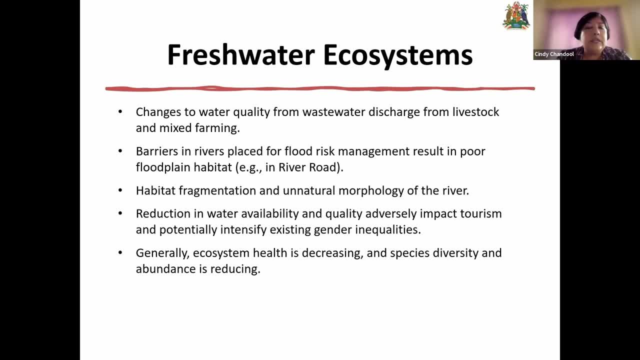 river and you know leads to fragmentation of that particular habitat. We talked about water availability already And so, generally to sum it up, you know the ecosystem, you know health of the freshwater systems is already decreasing and species diversity and abundance will tend to reduce as well. Next one, So 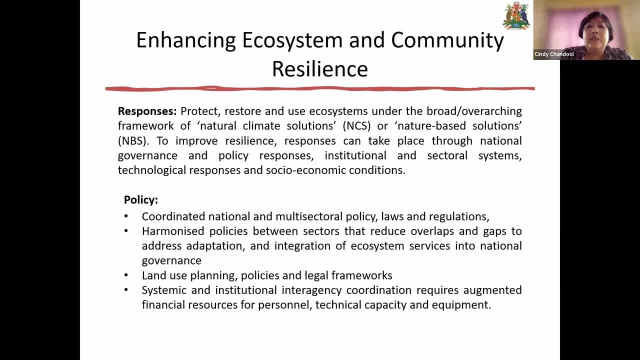 given these- and I know it sounds a little grim, but given these, these impacts, we are looking towards enhancing our ecosystem and community resilience. To do so, we need to protect, restore and use ecosystems in a manner that we're looking at. you'll see different. 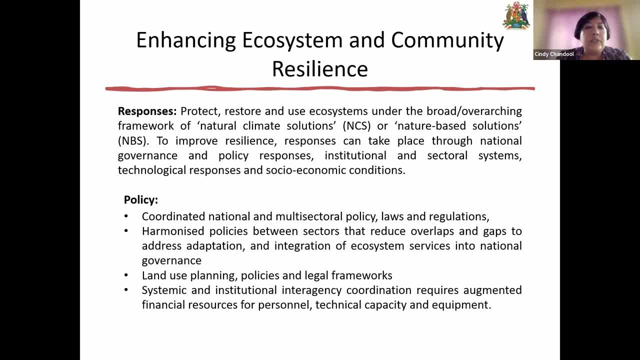 terms: natural climate solutions, nature-based solutions- you'll see these kinds of terms coming up And we can initiate responses, implement responses that are done through policy, that are done through institutional and sectoral systems. we can have technological responses, changes in socioeconomic conditions. So 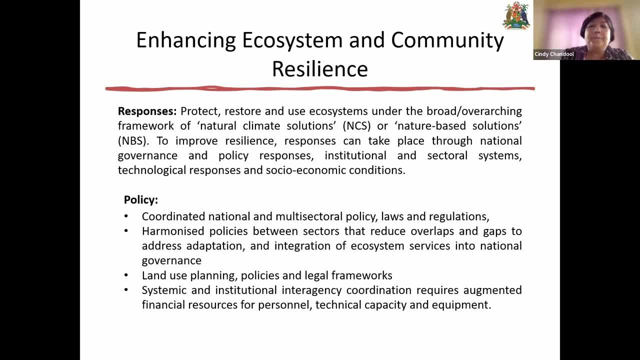 we'll go through some of these responses And we'll look at what has been done and we'd hope, in our breakout sessions to find out further information in terms of your ideas and what you've seen, perhaps in terms of examples of these. So when we 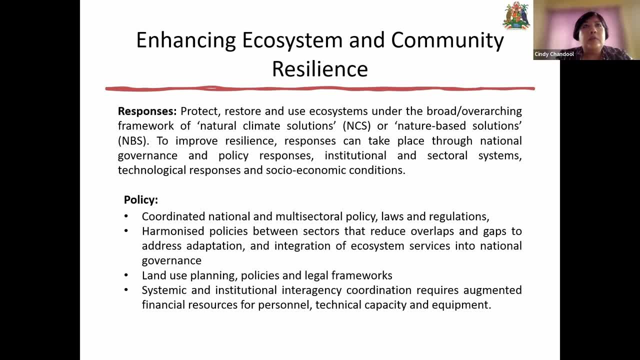 look at policy. we can look at better coordination of all of our policies: national, multi-sectoral, harmonizing policies between sectors, ensuring that, you know, adaptation, ecosystem, services- all of these policies are in place. And then we can look at what has been. 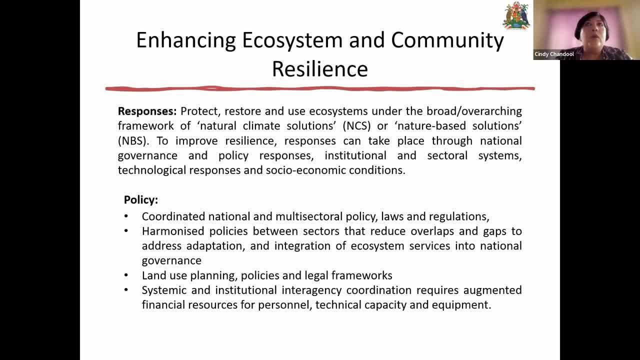 done and we'd hope in our breakout sessions, to find out further information in terms of these policies: national, multi-sectoral, harmonizing policies between sectors, ensuring that, you know, adaptation, ecosystem services- all of these policies are fully integrated into national governance We look at 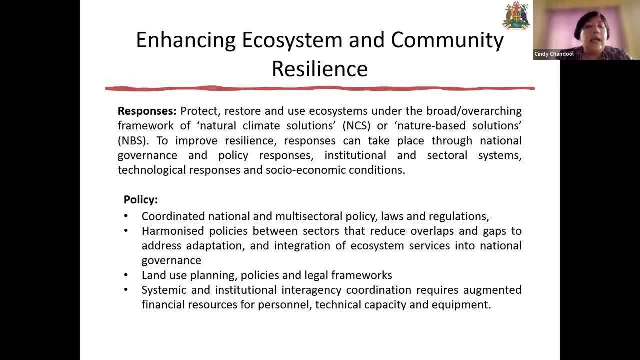 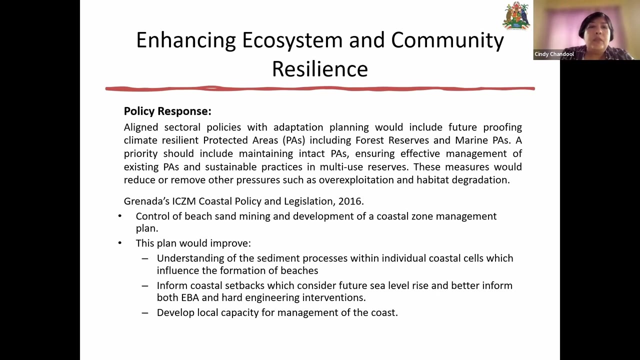 land use planning policies frameworks and institutional coordination, So coordinating among agencies. of course, this requires a financial input as well as capacity development, from both a technical standpoint as well as physical equipment that may be required. So, when we look at one of the key initiatives that we would like to see, 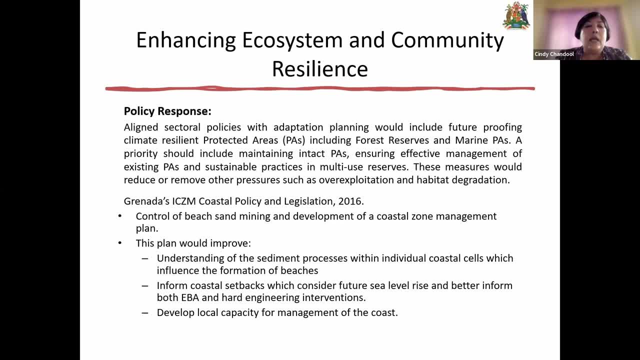 in terms of producing climate resilience is leading to increasing our protected areas resilience, So things like both forest reserves and marine protected areas, of course, should be a priority. So I think it's important to look at the Sustainable practices, because we recognize that some of these reserves 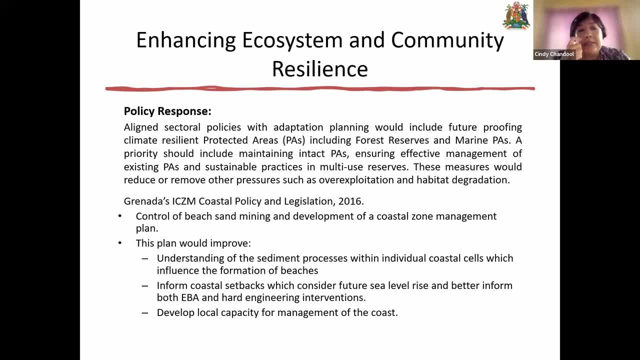 will need to be multi-use reserves, So to look at removing the pressures or using the pressures that are leading to habitat degradation. So you know, one of the policies that was adopted by the was looked at in terms of its potential is the ICCM policy. that was done in 2016.. So 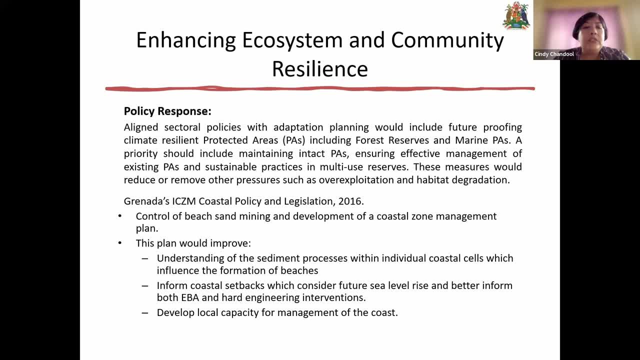 the ICCM will control beach sand mining and it makes provision for a coastal zone management plan. This type of initiative will help us both understand the sediment processes, inform coastal setbacks, look at ecosystem based adaptation as well as hard engineering interventions, and these plans will look at development. 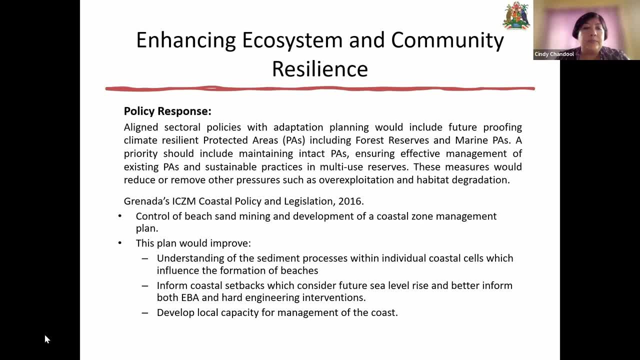 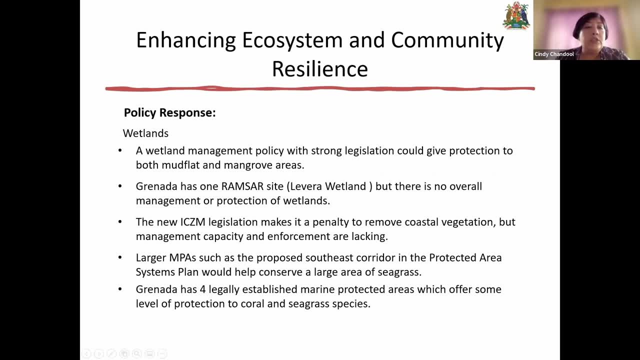 ofArtest. that is truly essential for the development of catfish science. that's going to be developing capacity for management of the coast. Next slide, In terms of wetlands, one suggested policy response. we all there's already: the Ramsar side, the Levera wetland. 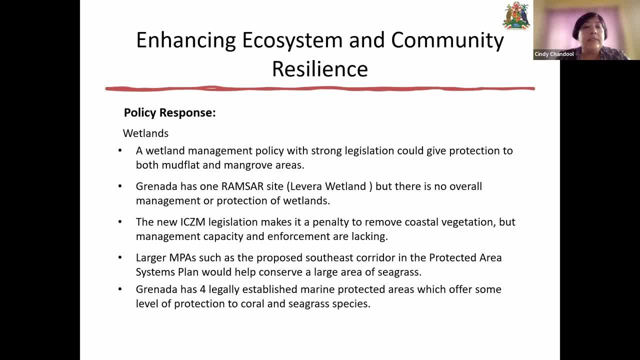 but we want there needs to be more overall management protection of wetlands, suggested in a wetland management policy with strong legislation to give protection to these areas. Although the ICZM makes introduces a penalty for coastal vegetation, we know that capacity needs to be built. 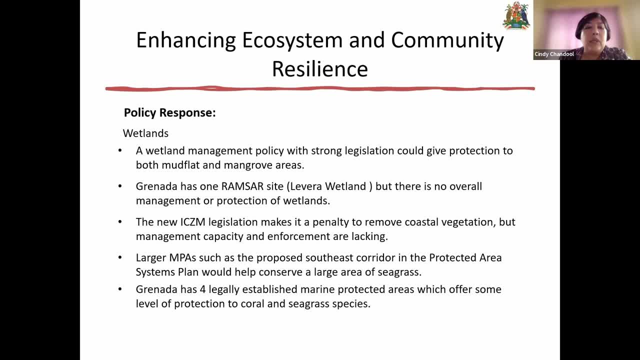 It's you know. there's just needs to be more management personnel and so on. One of the suggestions that may work in terms of a policy intervention is larger marine protected areas, such as the already proposed Southeast Corridor in the protected area systems plan. 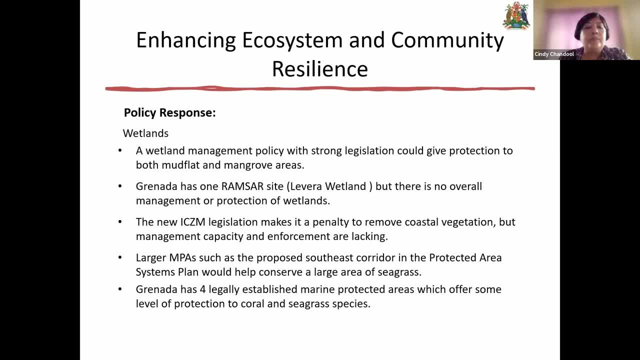 that will protect large areas of seagrass right And of course, there's already four marine protected areas, which does offer protection to the coral and seagrass species. Incentives: these have not and I would love to hear if there are examples of this. 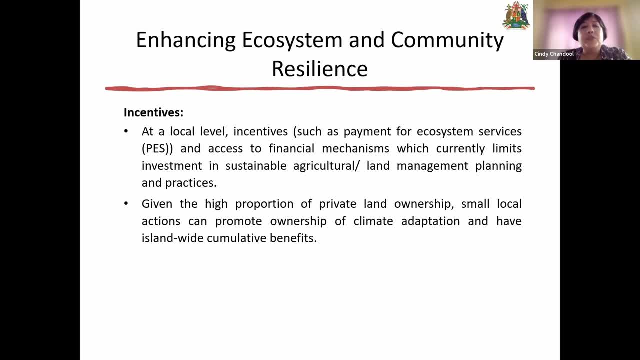 or any proposed measures. the incentives such as payment for ecosystem services, other access to finance. we know we need a lot. there's a lot of capacity that can be built. Issues such as sustainable agricultural and land management- very important that this capacity is built as well. 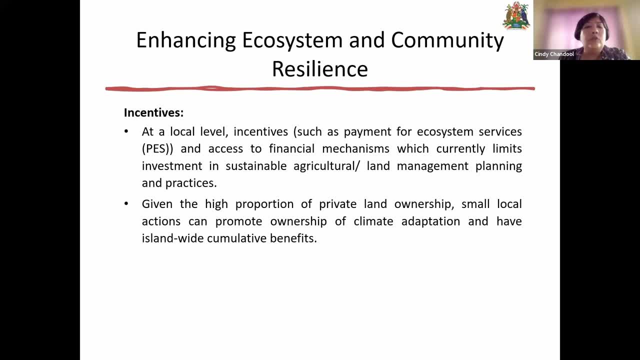 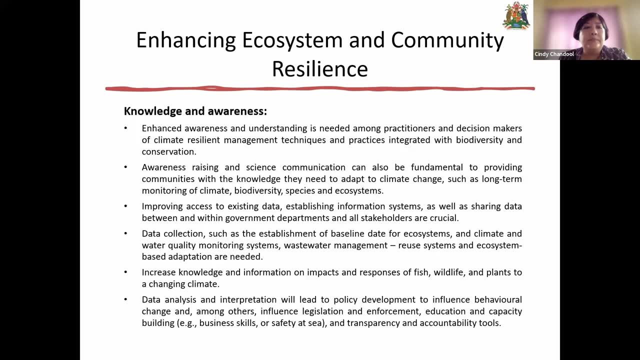 So small. you know, local actions can also lead to resilience measures and adaptation measures. Next slide, Knowledge and awareness, is quite a big one. I'll just go through some of these very quickly. I'm sure most of this you know already. 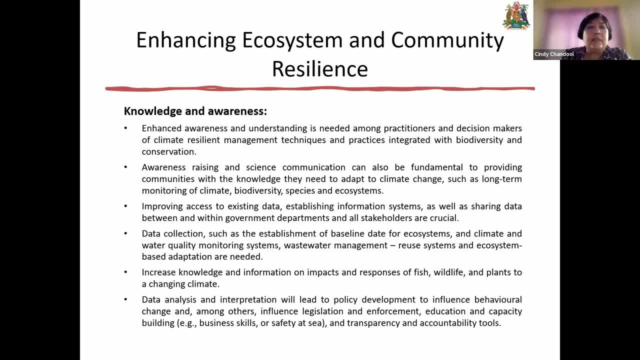 The data. access to data is very important. We need to know what opportunities are available to us, what we're protecting, so having this baseline data is important. as well as monitoring, we need to see what are the effects. what are the effects of climate, what are the effects of changes and 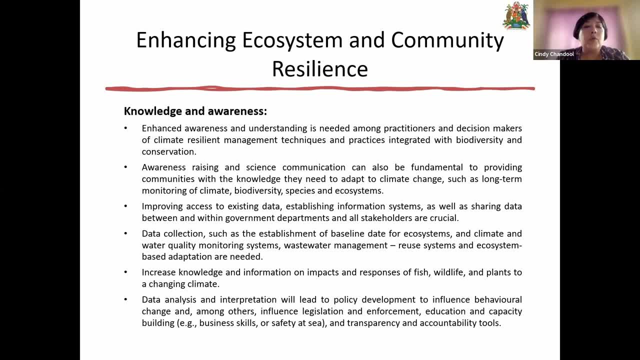 what you know, what are, what is the water quality like now, and make sure to monitor how it, how it changes in the future, wastewater management, and so on. coupled with this, we also need to raise awareness and understanding, both among practitioners and decision makers, which i know is always a challenge in terms of: you know, what are the management techniques, what are needed, what. 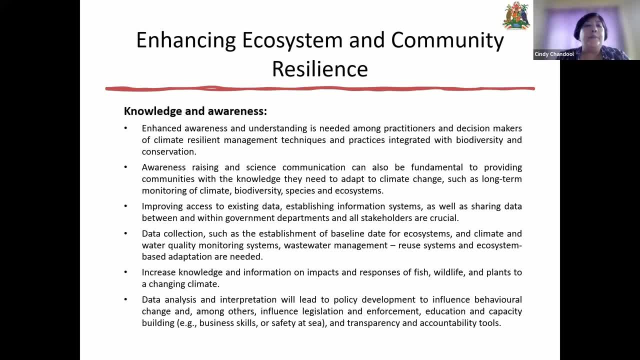 practices are needed for biodiversity and conservation, um and also our communities. communities need to be armed with the knowledge of what they need to do to adapt to climate change. data analysis and interpretation to actually feed into policy development. and, of course, changing that behavior is always one of. 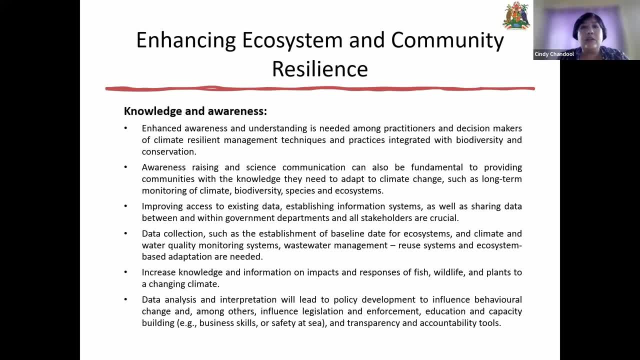 the biggest challenges in our communities when it comes to climate funds. So, as I said, of the key challenges that we face in the conservation arena and actually changing people's fundamental behaviors, And, of course, the interpretation is needed to then affect legislation enforcement. 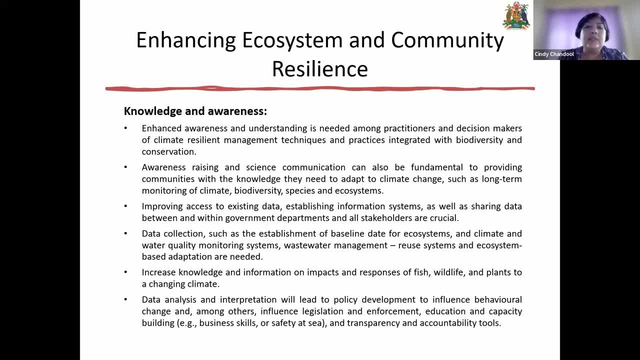 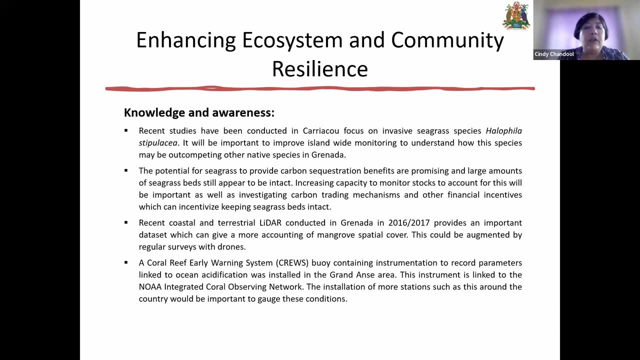 all of the types of capacities, such as safety at sea, business skills and so on, that will be needed as we move forward to facing climate change. So some of the examples of data and measures that have been already implemented that can be used to increase our ecosystems. 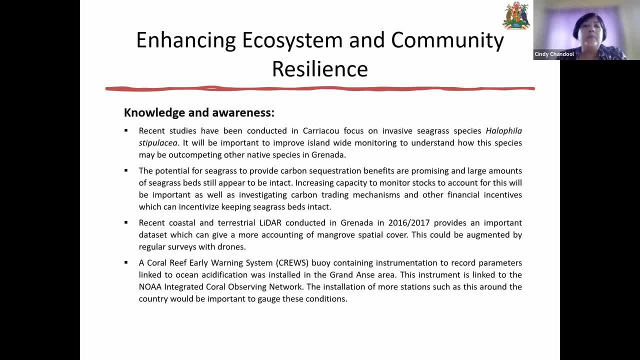 climate resilience Kariakou, for example, there was studies on the invasive seagrass species and it's important to monitor in terms of how these may be out-competing native species. Carbon sequestration benefits of seagrass are also important. 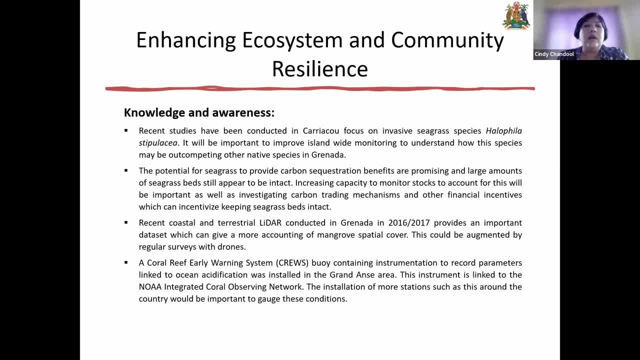 One of the issues we face is that a lot of the carbon sequestration studies have been done on terrestrial ecosystems, So it's important to look at the marine ecosystem as a valuable resource for both carbon sequestration and other climate resilience measures. There's also been studies on LIDAR conducted. 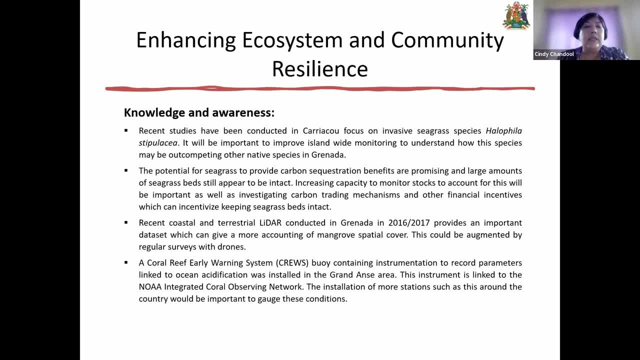 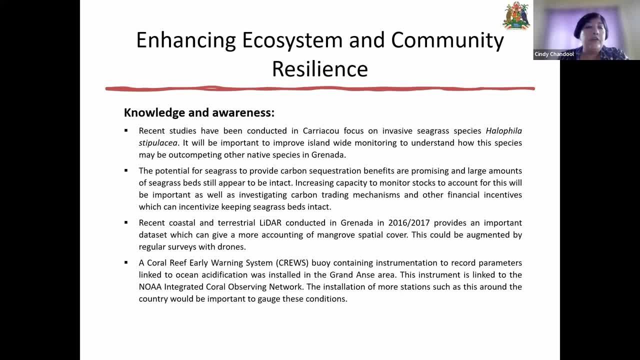 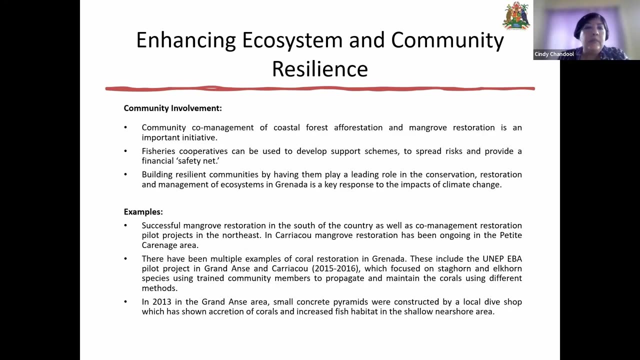 that can be used for mangrove is used for mangrove spatial cover and the coral reef early warning system and stolen ground ants area is also another example of data being used for enhancing ecosystem resilience. Next slide: Communities. So we spoke about communities and the importance of community resilience. 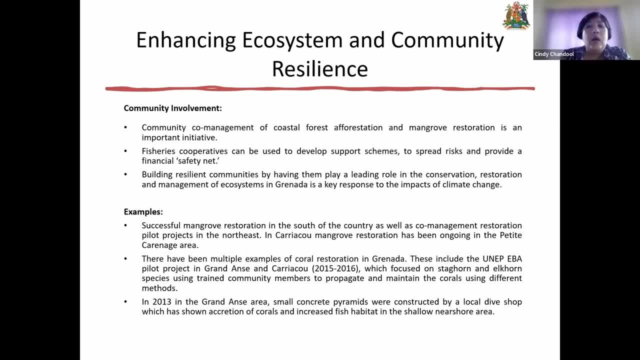 and not just ecosystem resilience, and how very much these two are interconnected. So community co-management is very important in terms of having this climate resilience, enhancing this climate resilience, Fisheries cooperatives, for example, having that safety net in terms of finances and so on developing that type of scheme. 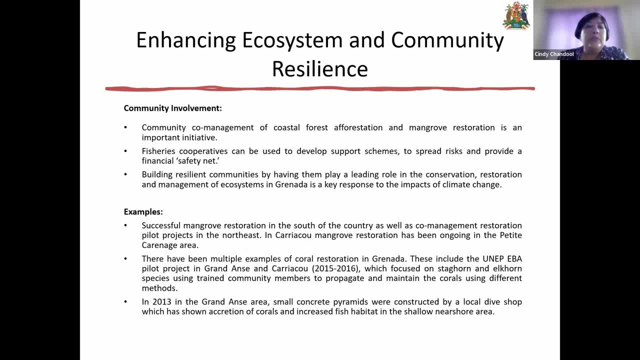 risk management schemes, building resilient communities by having this co-management approach to conservation, management, restoration. So there are already many good examples of this. in Grenada, There was successful mangrove restoration as well in the South region, as well as co-management pilot projects in the Northeast. 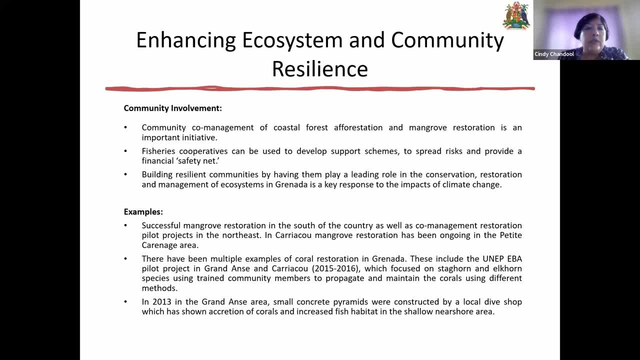 in terms of mangrove restoration And, of course, continued mangrove restoration initiatives in Carriacou, Multiple. there's also coral restoration, Grand Anse. in Carriacou There's been many some restoration activities in terms of staghorn and elkhorn species particularly. 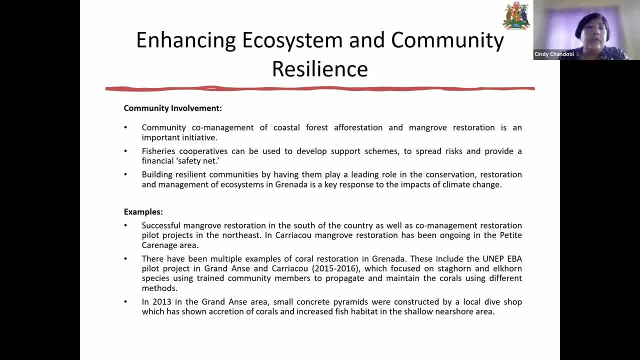 And there are many, many options and available initiatives that we can look at for training community members to continue restoring these ecosystems. Right and when we talked about small initiatives by local businesses, there was the local dive shop where we installed concrete structures to propagate corals. 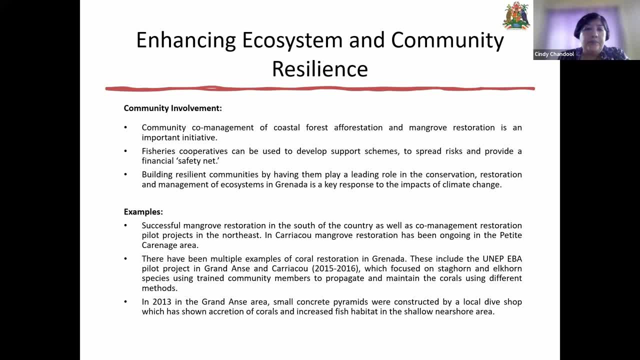 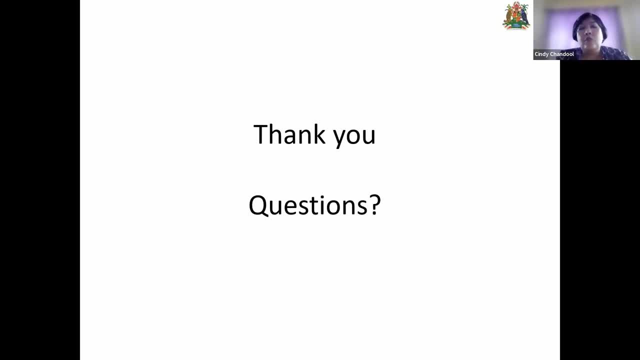 and, of course, increase fish habitat as well. Right, so to wrap up these kinds of co-management initiatives and technologies is important to continuing to implement these kinds of interventions, build local capacity and, as we move along, reducing the non-climate stresses. 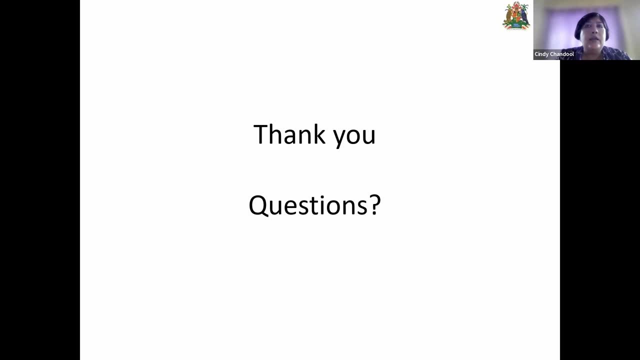 that we talked about. I can see somebody put in the chat about pressure from land changes and agricultural changes due to agriculture and so on. So if we continue to reduce these non-climate stresses, we will help that resilience of our fish wildlife plants. 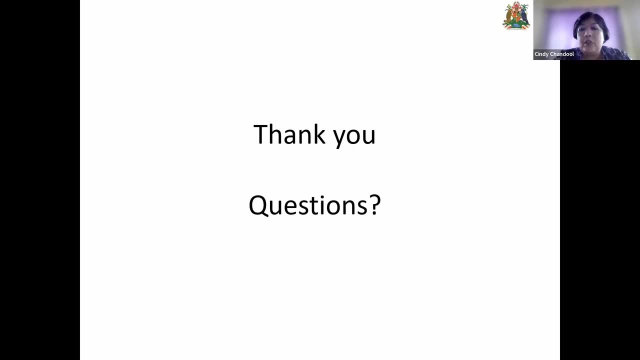 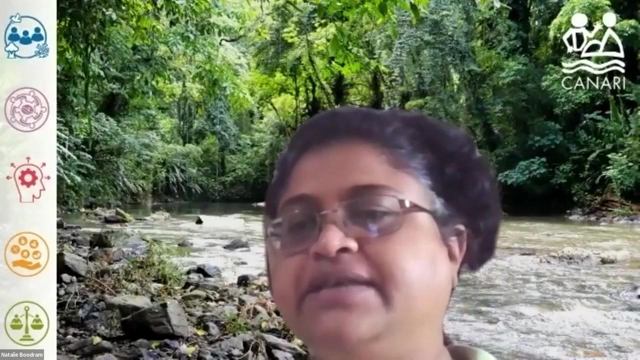 all of our ecosystems in adapting to climate change. So thank you very much for your attention. That was just a summary of our very long chapter And, of course, I'm available for questions, Natalie. So we do have breakout groups, but we can open up the floor for some questions and comments. 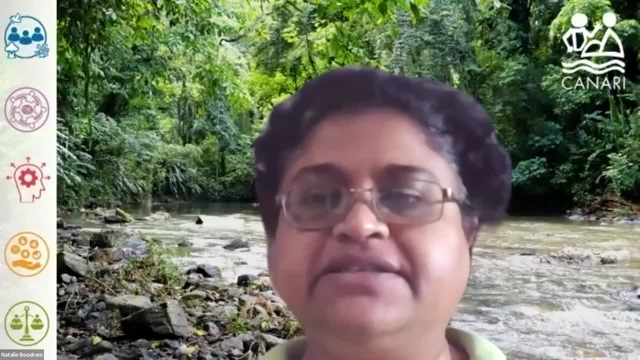 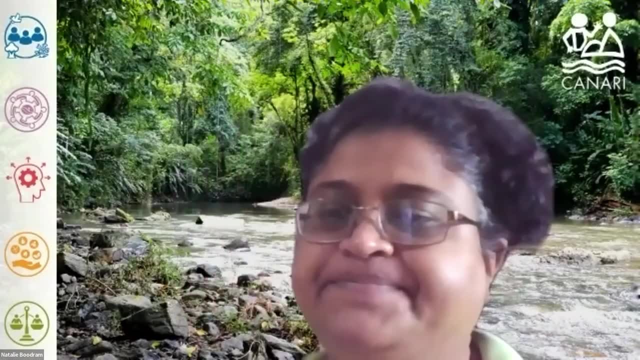 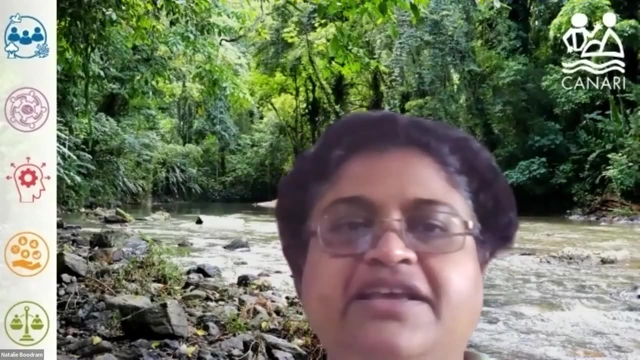 now for a couple of minutes, for five to 10 minutes, before we go into the breakout groups. So the floor is open. If anybody wants to say anything or ask a question, Okay, All right. well, I'll go to the people who'd like to speak. 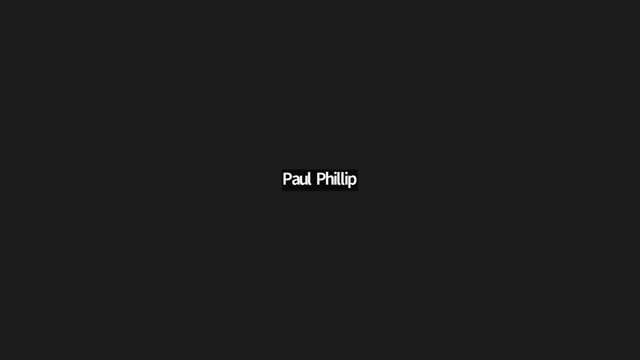 but then I'll also read out a few of the chat comments. Go ahead, Paul. Good morning, Very good presentation. Thank you very much for that. It brought out a lot of things that I was going to speak about, but I'm still going to make a few comments. 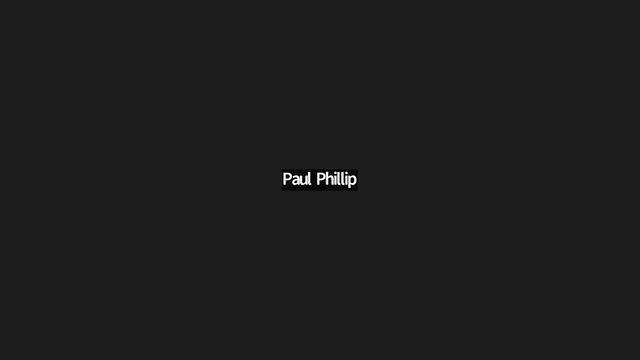 And, as a marine biologist, I'm going to look basically at the question of coastal zone in Grenada. We have a situation in Grenada where we're looking at climate change and trying to build our resilience to climate change Now in Grenada, one of the first areas where we're going to be affected. 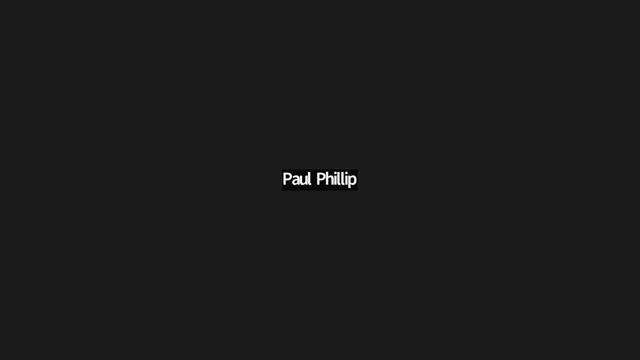 from climate change is through sea level rise. And if we're looking at sea level rise and we're looking at resilience of sea level rise, we have to look at our coasts, not only for the to combat the whole question of climate change, but because we also marketing Grenada as 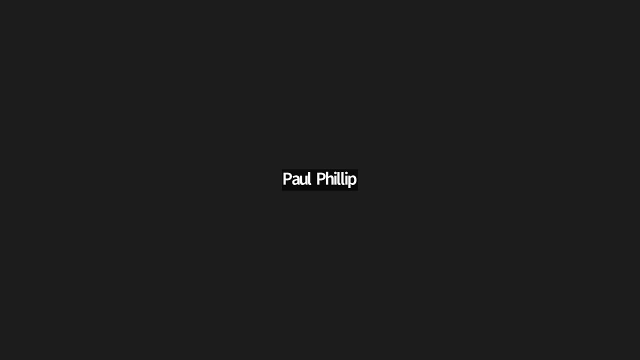 a tourist destination and one of the products that we have is our coast, so there is a need for us to protect that. however, in the Grenadian context, what you find happen is that, over the years, we have basically removed most of our coastal areas. people might argue and say: okay, 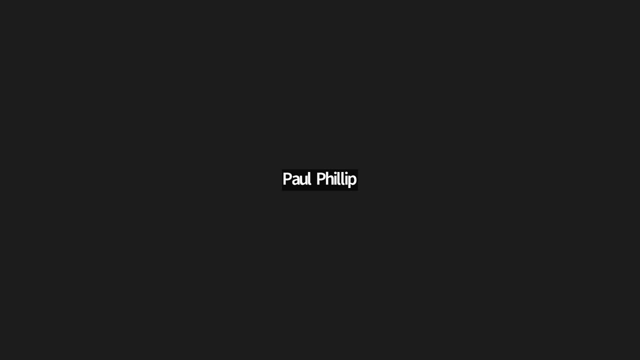 we are losing our coastal beaches through to erosion. I would argue differently. I would say that we're not losing it to erosion. we are losing it to construction, because one of the things that you find happening in Grenada is that used to happen and still happening is that most of our 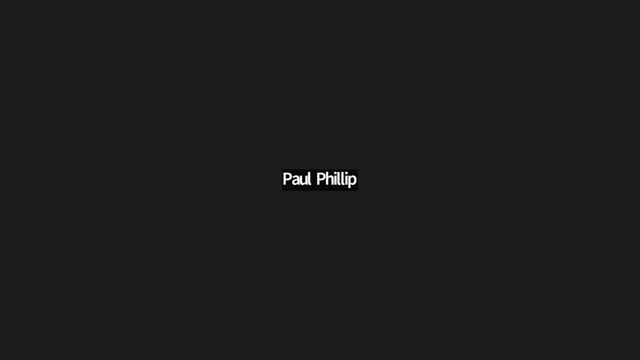 people. they think they have the god-given right to remove sand from the beaches whenever they want to, and so we have the east coast examples. we have the east coast, we have Garby beach in the, in the, in the St David's area, and more recently we have 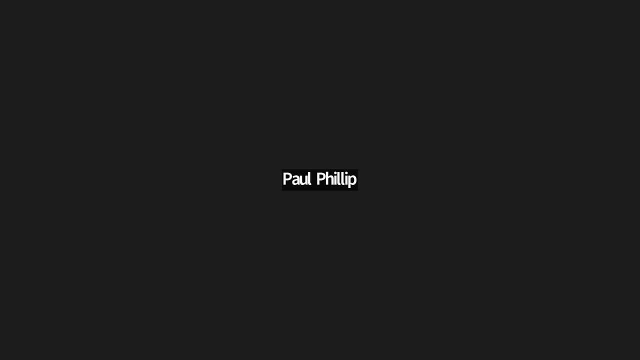 St Patrick's area where we have quite a lot of erosion going on now, and most of that is due to human activity. but my point, the point I'm trying to make this morning, is that I'm, I would like to see the this process that we do in true going through here, looking at the ecosystem. 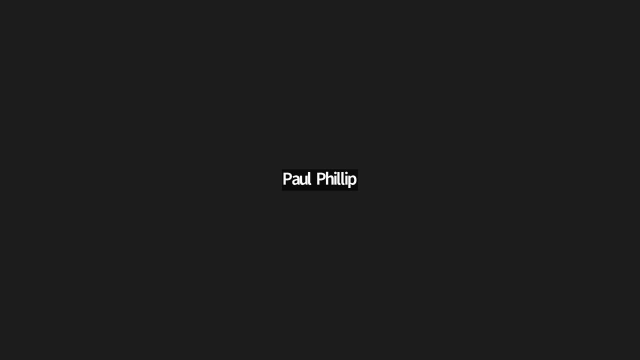 assessment. I would like to see coming out of of this a number of recommendations that will assist us to do better in the future, because in my tenure in the in the government process there has been an integrated coastal management policy was developed and an integrated coastal zone act management act has been passed. 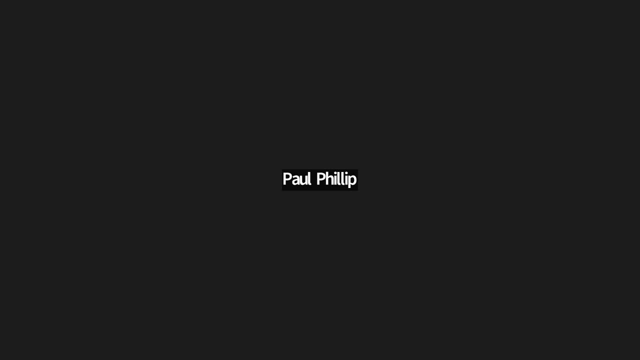 and yet still we we not seen any of these things being implemented on the ground. we also have in granada, i think, is a coastal zone management task force, um, one of the things that were mentioned. um, that's a few. in a few areas we have had efforts to improve the. 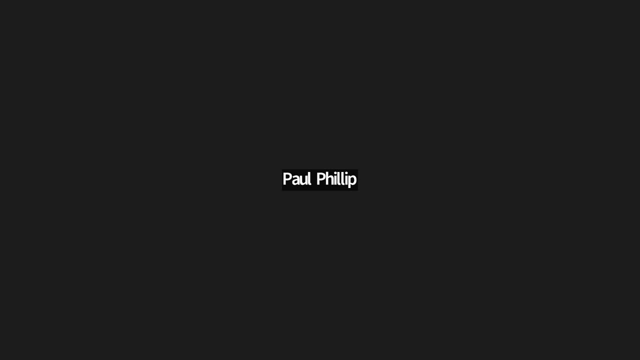 the resuscitation of coral reefs. yes, that is, that is correct. that is very correct. we have seen the resuscitation of car risk in some areas, but on the other hand, we have seen the demise of a marine protected area system. we we said some years ago that um. 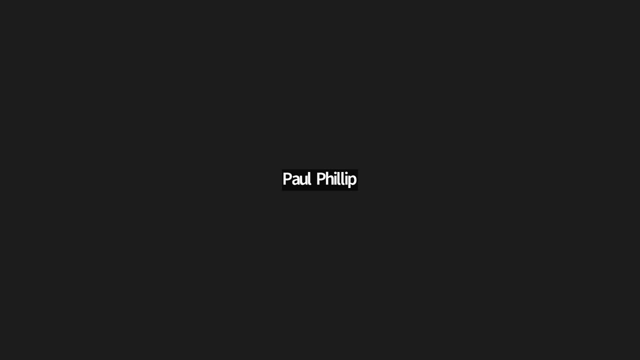 we are going to try to protect 20- 20 percent of our coastal marine resources by 2020, but we are in 2022 and um that has not been coming forth. so what i would like to see- i'm saying again, what i would like to see is that this assessment- not only do an assessment, but come up. 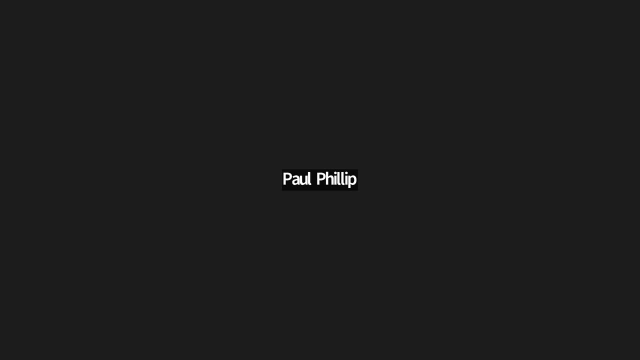 with recommendations where things can be done to improve our coastal resilience, because it's very important to us not only as a country to protect our coastal territories, our landmass, but also to assist in improving our tourism industry and also our fisheries industry- fishing industry. thank you very much. 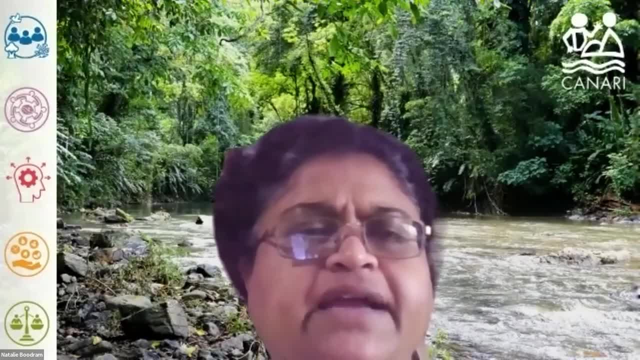 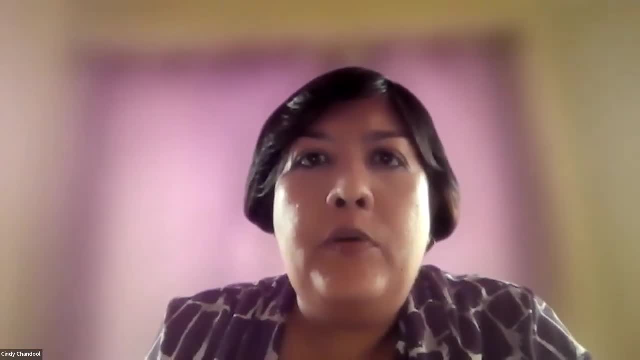 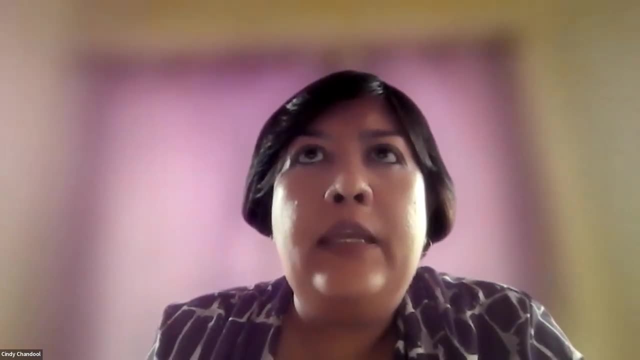 okay, thanks, cindy, if you want to um react, and then i have some questions that i'd like to make as well. those are excellent points. i i completely agree with you and i take your points. we definitely will be looking at um recommending and i will try to make the you know. 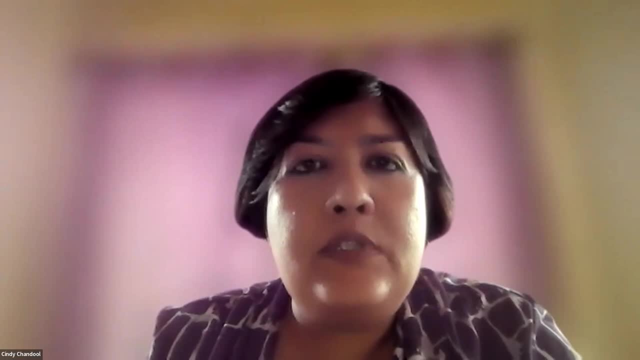 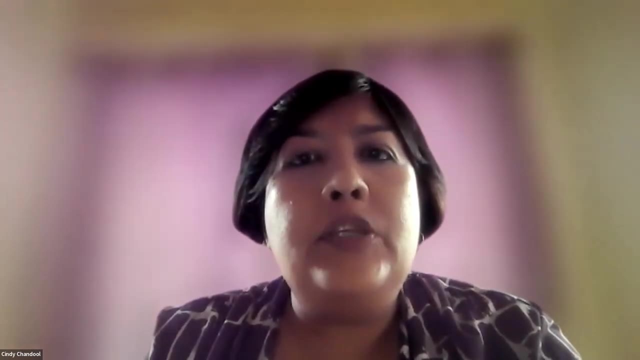 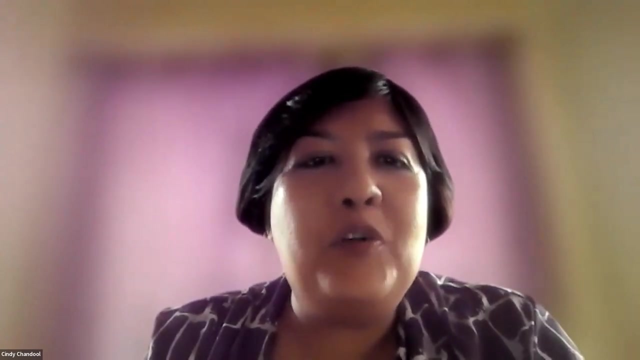 recommendations more specific. we do have some in there. as i said, this was just the summary, but we def. we will definitely look at some of the responses in terms of um- underground recommendations that we can implement and um. i definitely appreciate the information that you've and there's some information there that i'd like to take on board. so thanks very much for your. 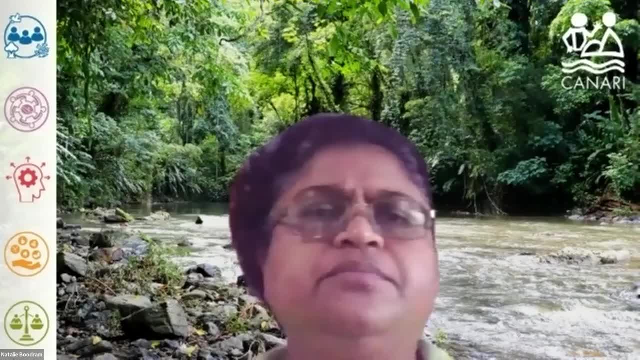 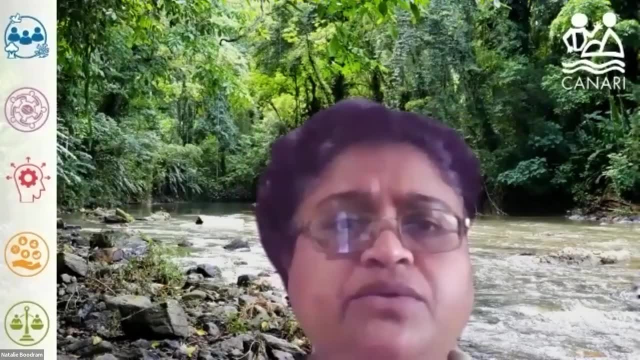 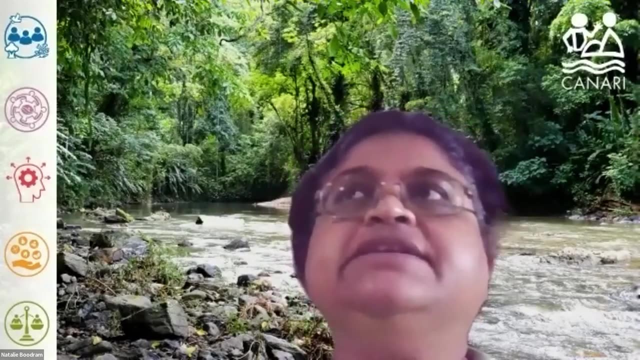 comments. yeah, all right um, paul. so in the breakout group we're actually looking for any specific recommendations or stakeholders have um to include one within this chapter, but one of our chapters that we'll be dealing with and taking to the public um later in this year, early next year. 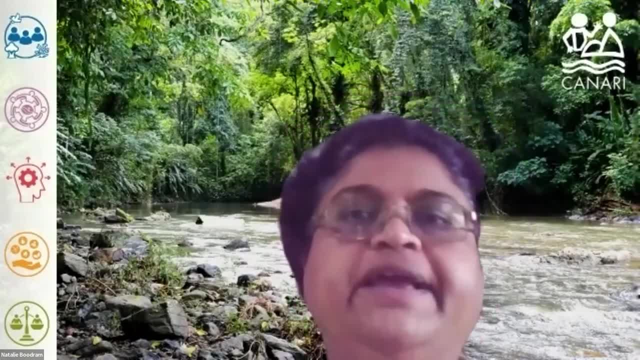 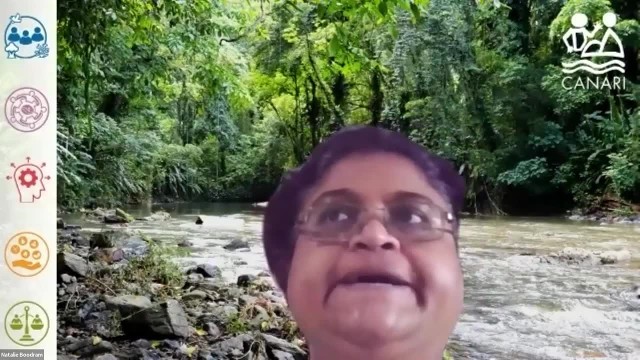 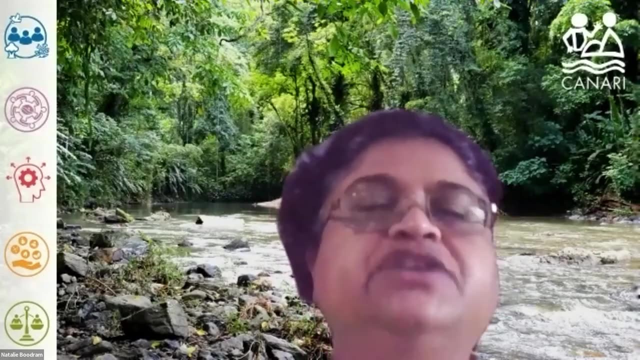 is a policy chapter, um, where we are hoping to make some more concrete recommendations, pulling in stuff that's coming out from the other um chapters as well. uh, as we keep saying, though, at the end of the day, um, it still is just recommendations and stuff that's in a report. 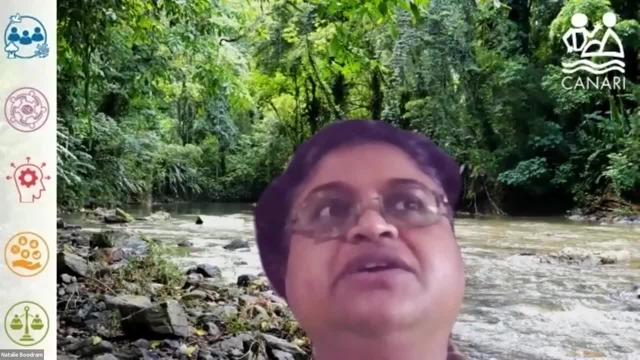 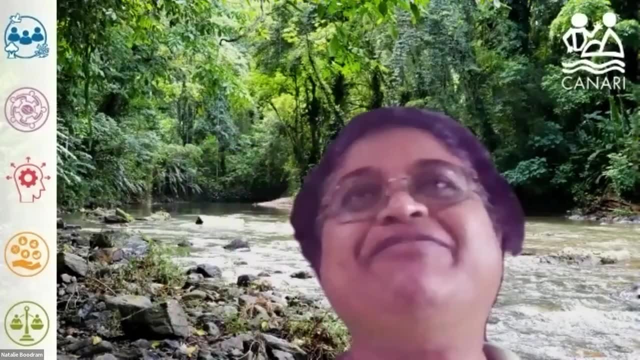 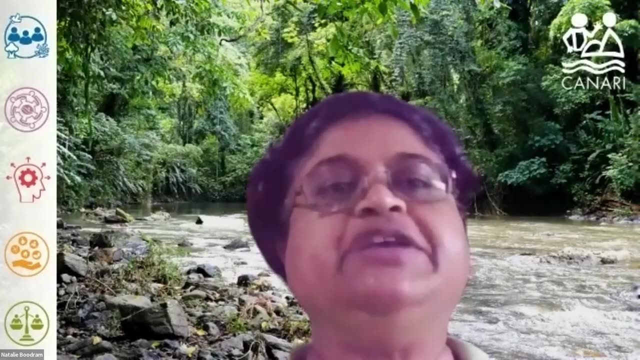 and one of the things canary is trying to do is to try and elevate it out of that box. so we are of course doing- sorry, i know i keep saying to referring to this. we're doing a citizen's as well. so, and we're also also doing a communication of information on the NEA material, which actually will be starting in. 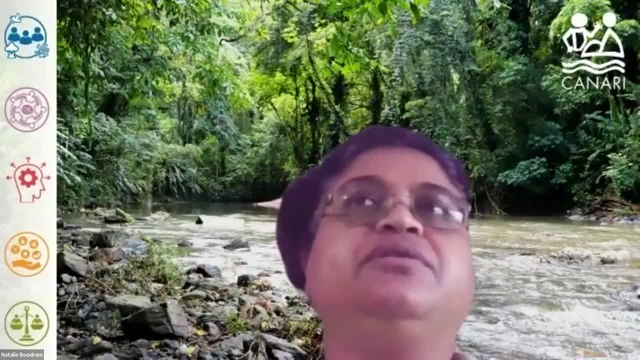 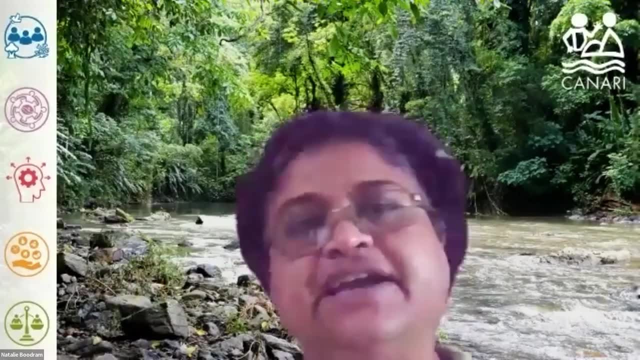 a couple of weeks. So, apart from there just being material put into this document and supporting documents, what we're hoping is that everybody here and anybody else can actually take that information and go to a meeting and, you know, talk about the issues and reference. okay, this. 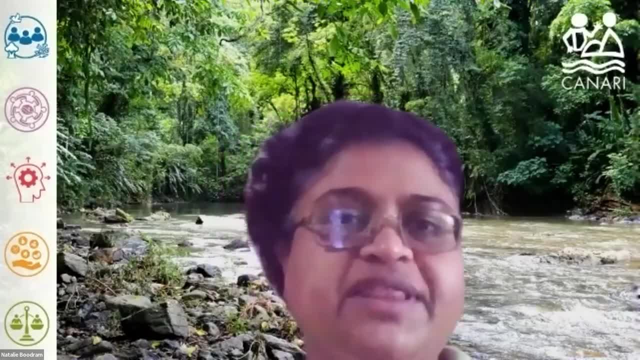 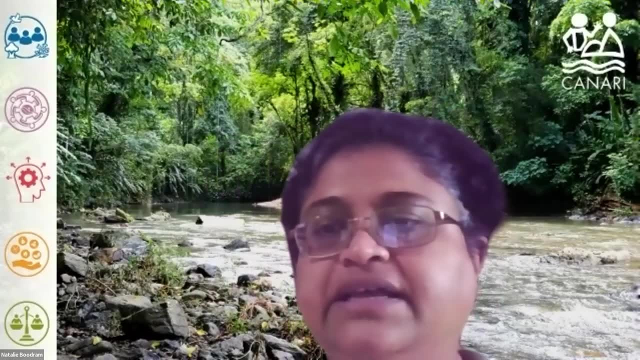 is. you know we're losing money to this amount, et cetera. So we think that is equally as important, other than, you know, just putting in the recommendations. So yeah, in terms of, let me okay, Joseph, I just want to read out a few of the chats which are relevant. So there, 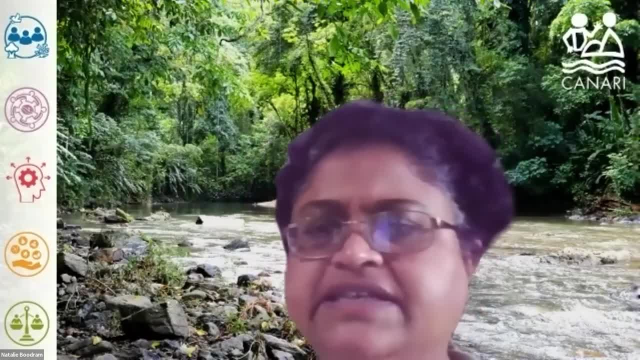 was a fair amount of discussion on the different data sources, but I think we answered some of those questions. unless Cindy has anything else to add to that, Just a point: I think you all did a very good job. thank you of addressing those questions. 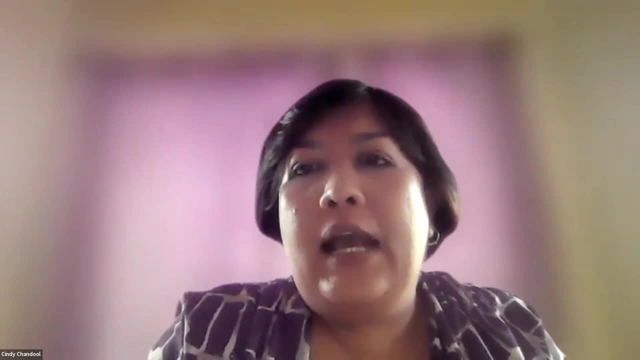 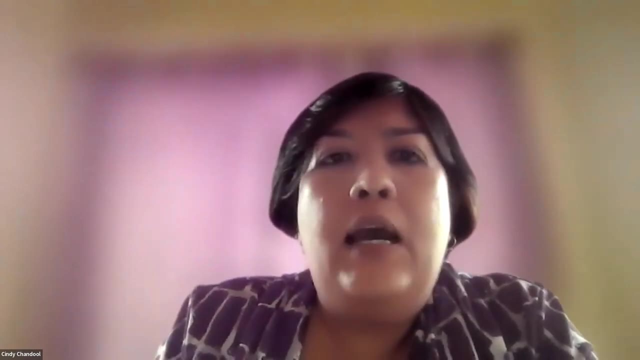 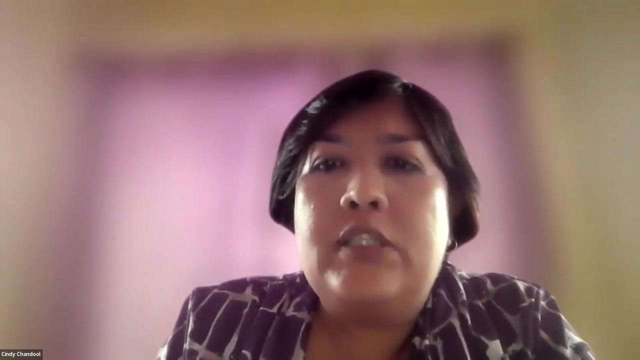 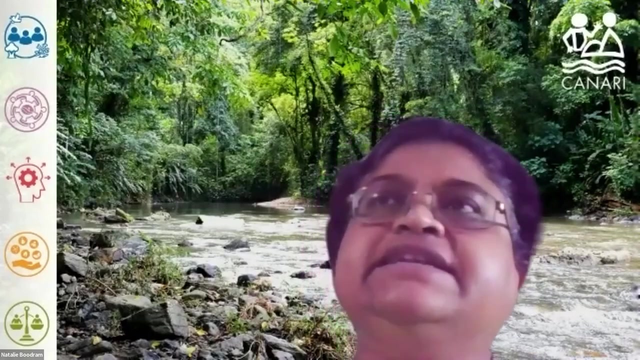 Yes, we did. We did look at AR6, and there will be potentially further information included. but Aria, I think, ably, answered the question about the projections. But yes, we are considering AR6 and some of it that's already integrated. Okay, great. And then Terrence noted that the other factors that in 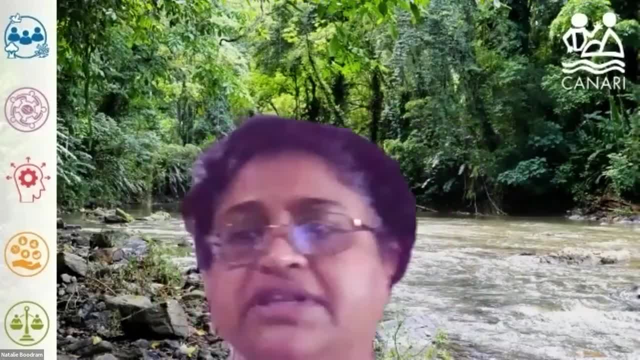 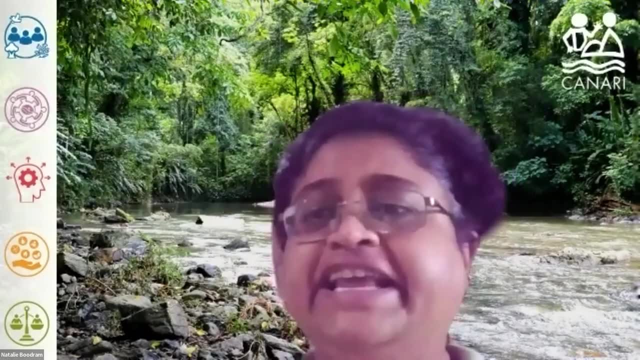 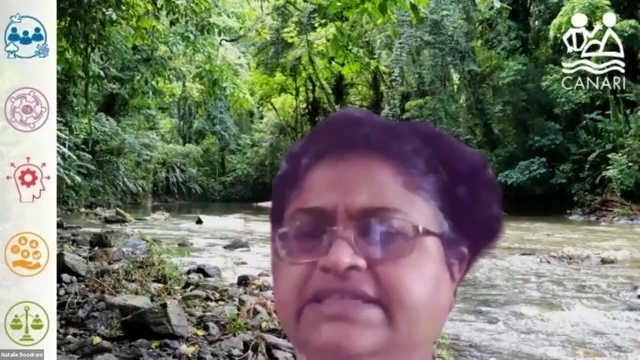 addition to climate change, that are stressors, including water quality issues with regards to waste Water and so forth. So thanks for noting that. Brian well indicated that he was impressed, but he did actually have a question that we've discussed: impacts in terms of qualitative impacts. 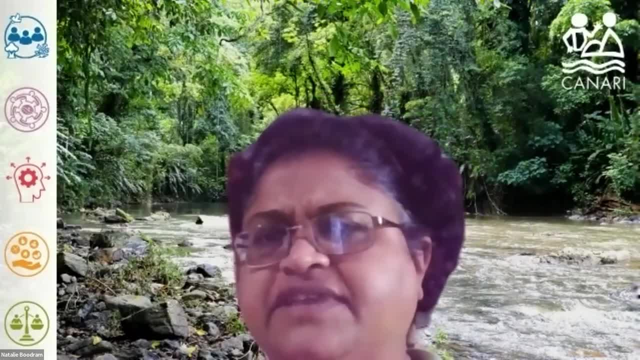 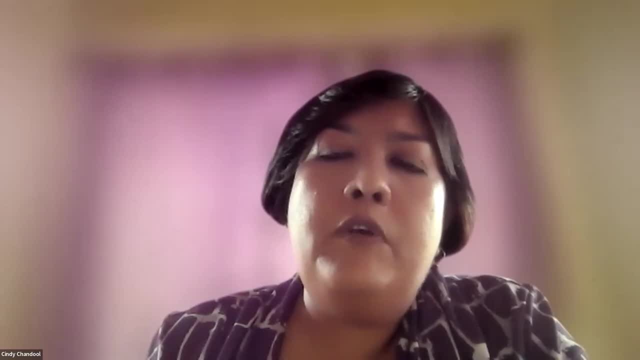 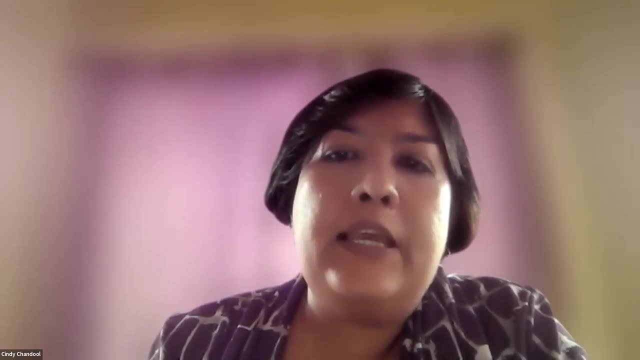 we cannot quantify impacts if the information isn't there And unfortunately we don't have the scope to do modeling, as you know, and so on. So we are relying on the impacts that are available and that we can refer to literature, grey literature, you know, published information. So this has been. 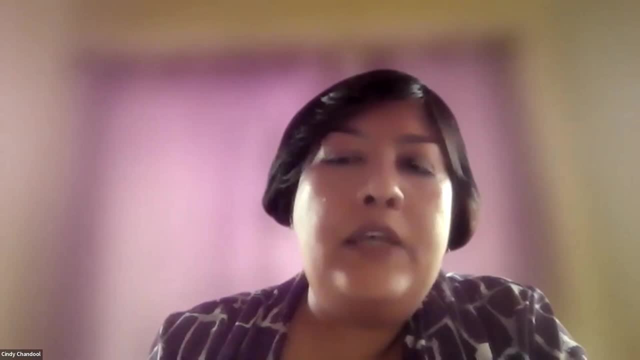 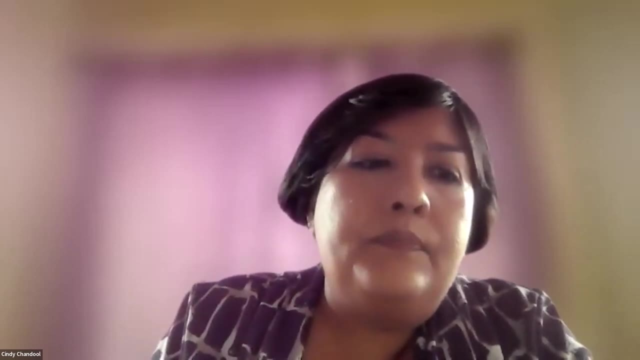 a limitation that, because of the way- as you would have said, Natalie- that these assessments are done, we have to rely on what's available. So you know, we can't, you know, we can't, you know what's already published. Yeah, so just to reiterate, I mean I mentioned it at the last. 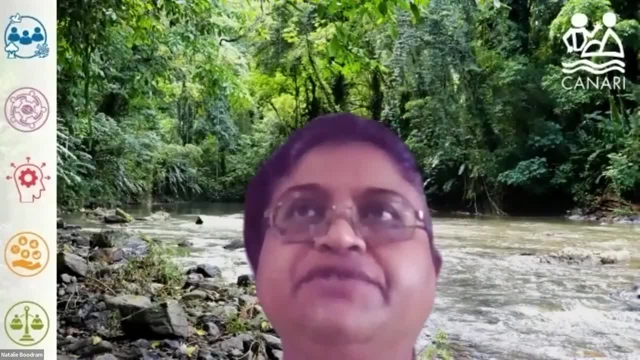 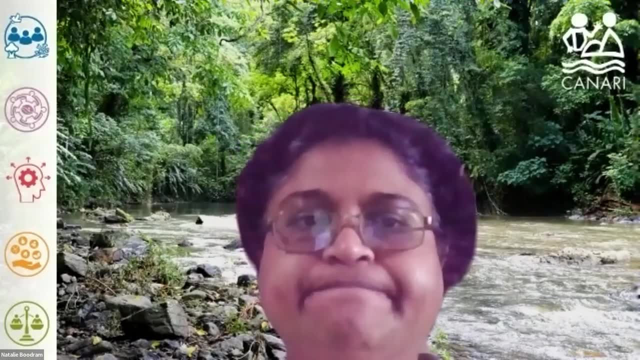 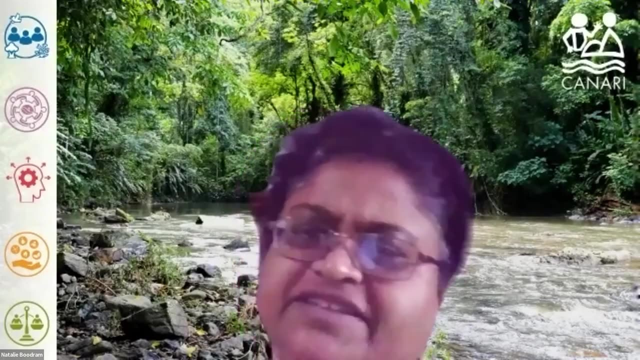 meeting. unfortunately, the methodology largely relies on literature. We are trying to expand and incorporate local knowledge and doing interviews and so forth, But this is what we have to work with. So Hayden made the point about competing priorities. Well, not quite related to this. 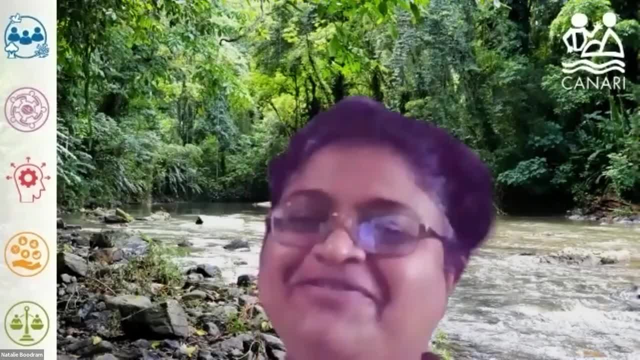 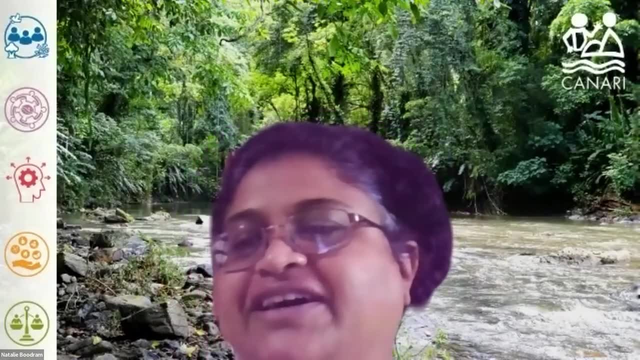 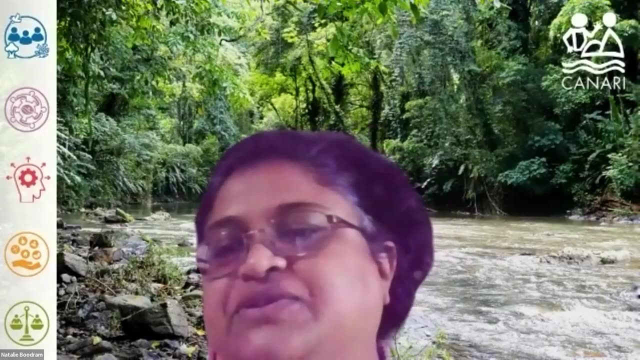 chapter, but all noted, Hayden. well, I mean related, but you're making a lot of sense. So I'll make a comment more on the environmental impacts and which actually are causing which sectors actually leading to some of the degradation. So you know, interesting to note whether it's more. 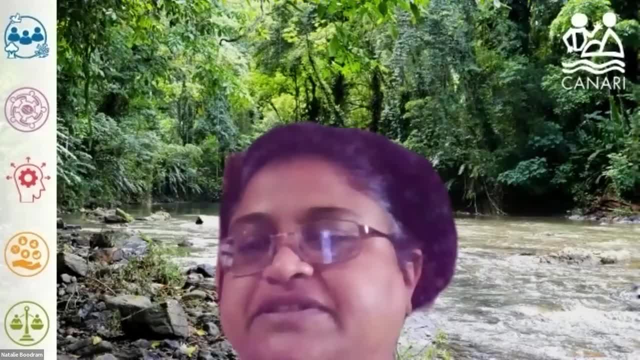 the yachting or the other types of tourism and so forth. Happy to see enforcement mentioned. Yes, So as much as possible, both in this chapter but more importantly in the policy chapter. we will be trying to speak to that. But. 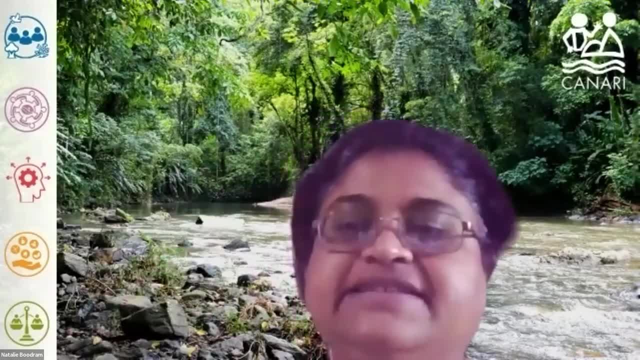 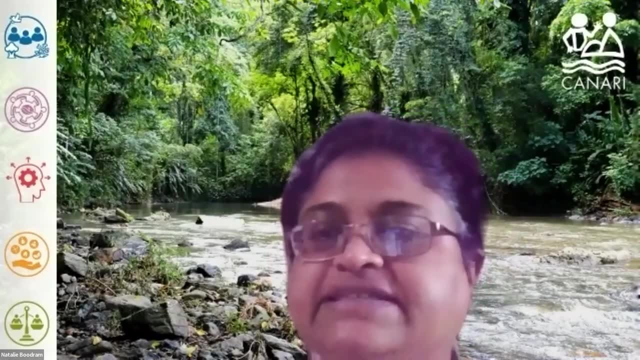 Again, what we're hoping and our method to try and get this information and implement it is for you all to take it and use it. So Chris Hayden mentioned, yes, the 20 by 20 challenge And Terrence, then noted: okay, using stronger and less diplomatic language. 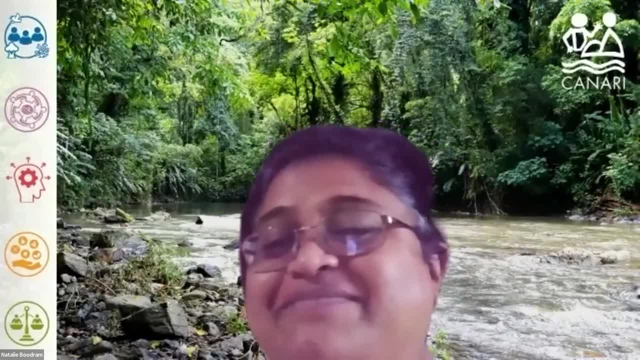 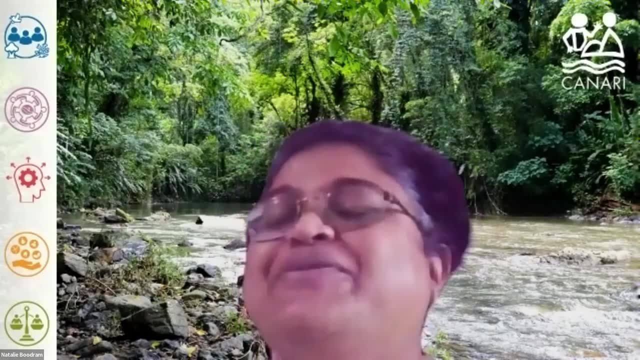 Actually, Terrence, we have to be a little careful And honestly, what I'm saying in terms of the language. you all take the information and use the strong language. We have to try to be a little neutral, but we will put all the information there for you all to use. 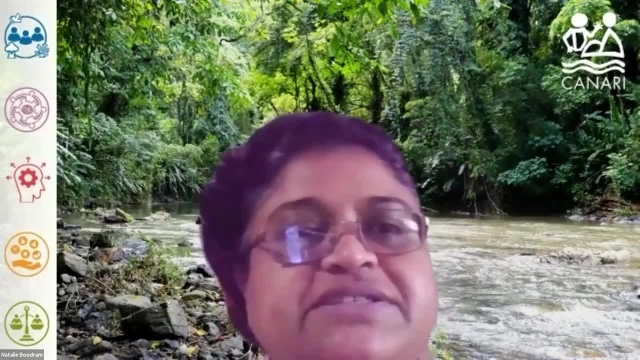 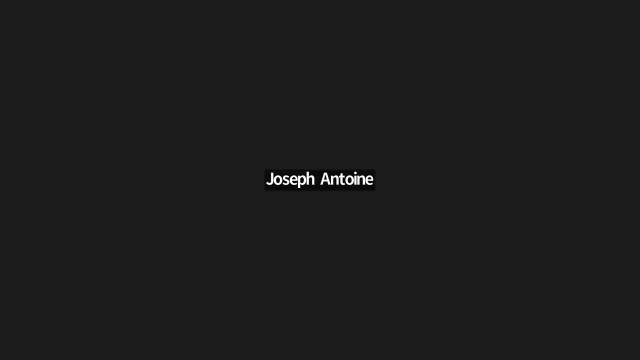 Okay, so I think those are all the chat comments, Joseph. we'll take your comment and then we'll move to the breakout groups. Go ahead, Joseph. When I came in, I heard the issue of coastal protection and that we have marine systems. 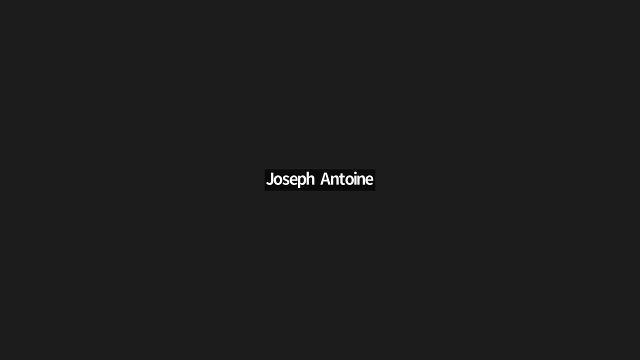 And so when I asked myself marine protective systems, I asked myself- maybe with the exception of carrier crew- where do those come from? Do those exist in Grenada? And also to say that, while the work you folks have been doing is very commendable in terms of bringing all this information and studies together to make sense, 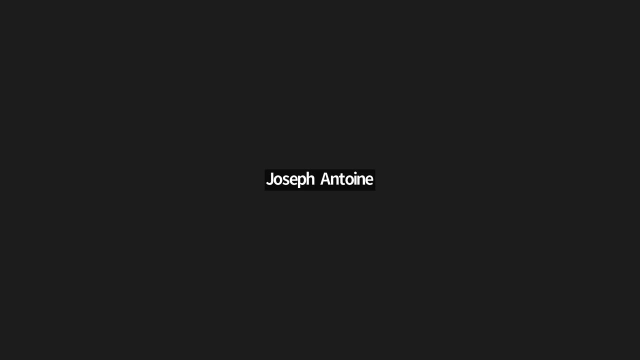 I'm afraid, by the time this is completed, there might be no thing to be concerned about. And the question I want to ask Natalie and the new policy makers: are they aware of the work that you are doing? I'm not saying that they have to intervene, but are they aware? 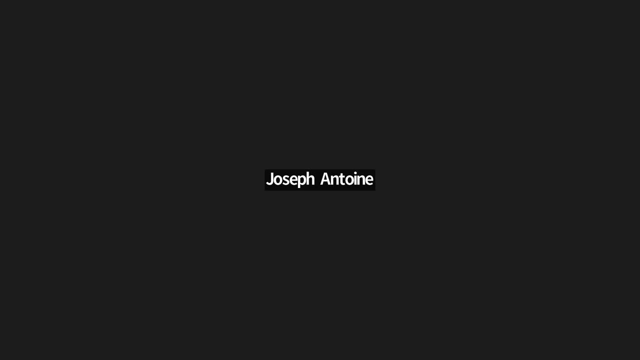 Because to me they're contradicting what you're doing, both the past and the current ones. So unless we send a halt to the ecological destruction, which I think is ecological crimes, we'll be just having intellectual exercise. Sorry, I'm sorry. 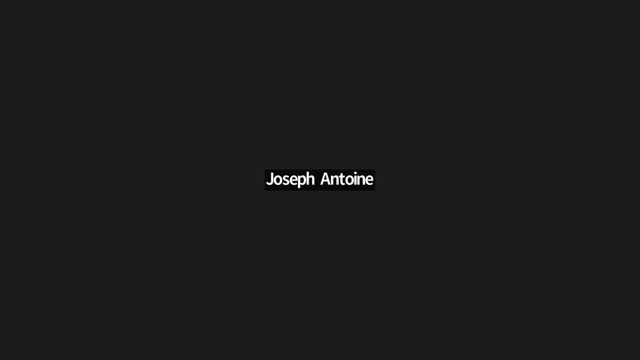 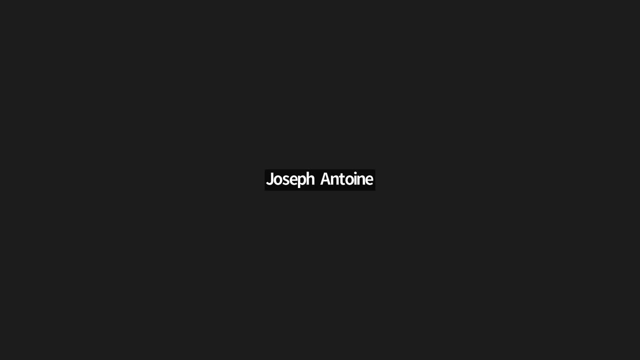 Thank you, I can go on, but I just felt that after me, that's it, man, And maybe, maybe, Natalie, you probably need to get to the new policy makers, So I'll go ahead with that, All right. 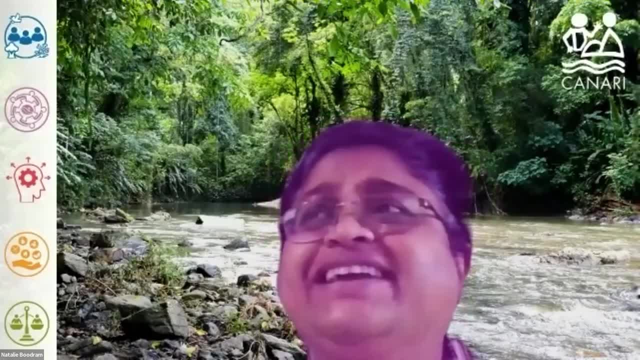 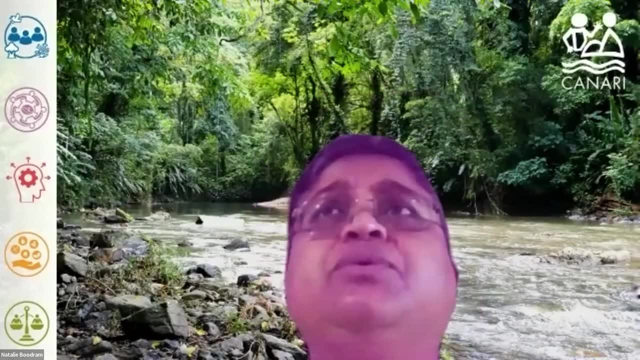 So, Joseph, you know I've been, You know I've been talking to you, Chris, the others, for a long time. We know that this is going on. We know that we were wary when we started this project because, yes, it is mostly a report and documentation and so forth. 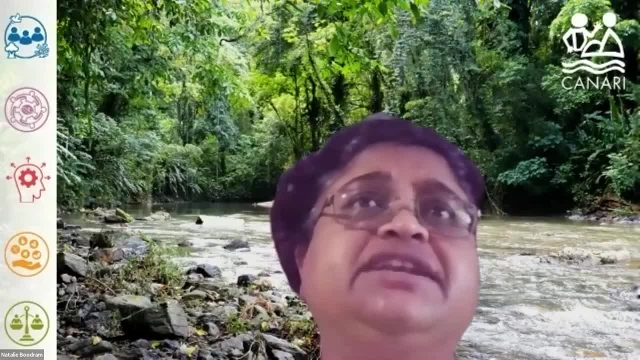 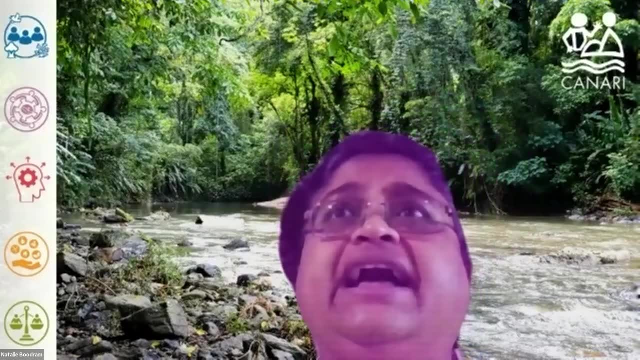 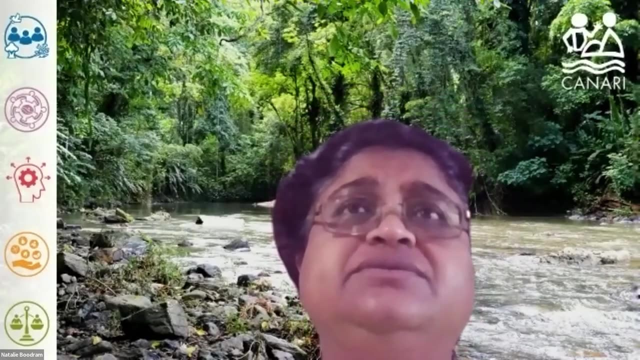 We are really hoping, because we're doing the evaluation aspect, to try to use a little bit more of that information in terms of communicating. I can't promise anything. You know that We are just trying. I would say that what we are trying to do, separate and apart from past things, is to try to help others communicate this information. 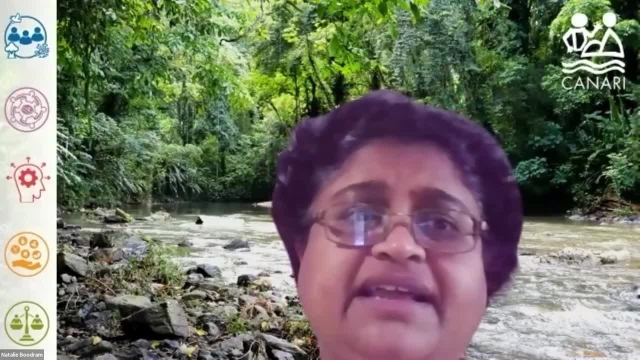 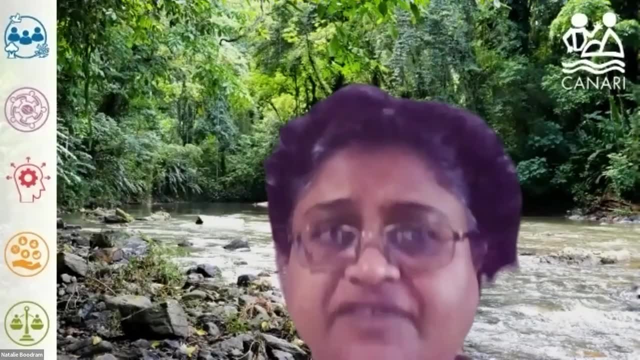 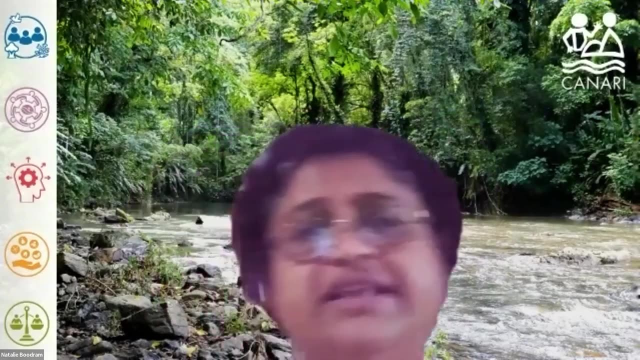 Yeah, I don't have an easy answer for you, but what I will tell you is that part of this process and this workshop is to capture stakeholder feedback. So we will have a section where we have stakeholder. we have that expression of comments and sentiments. 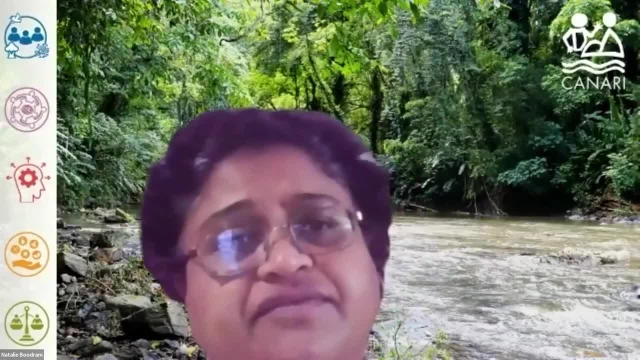 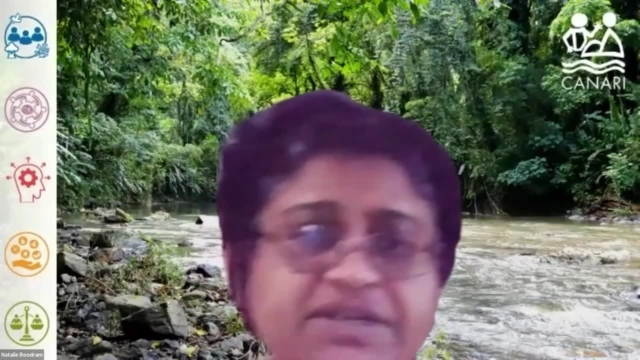 And we will be highlighting that stakeholders are wary of of you know what's going on and are concerned about the destruction of the mangroves, et cetera. So this is just the other. the other question: This is a government of. we need a project that canary is executing. 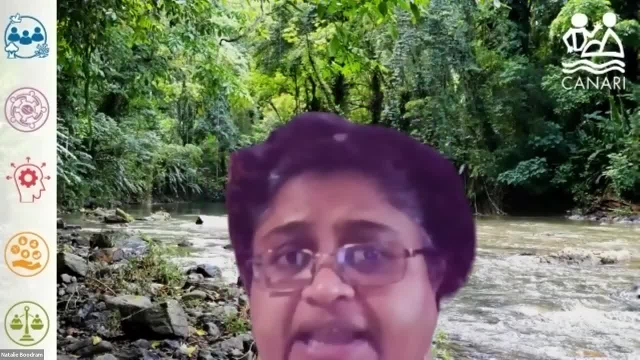 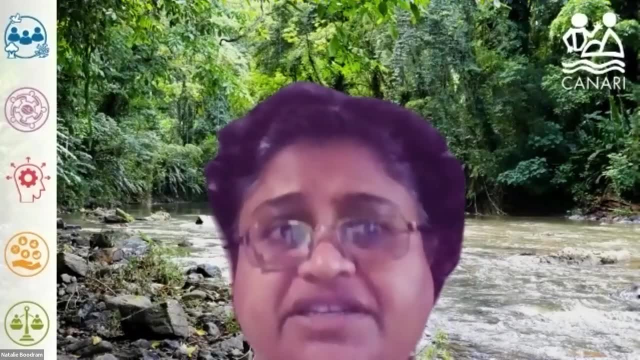 So, yes, they are aware. I know that there has been a change in the government and we have not engaged fully as yet with the new regime. We need to do more, We need to be more aware of that, And certainly we will. 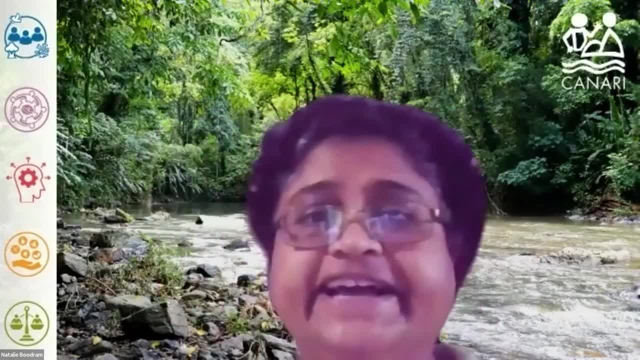 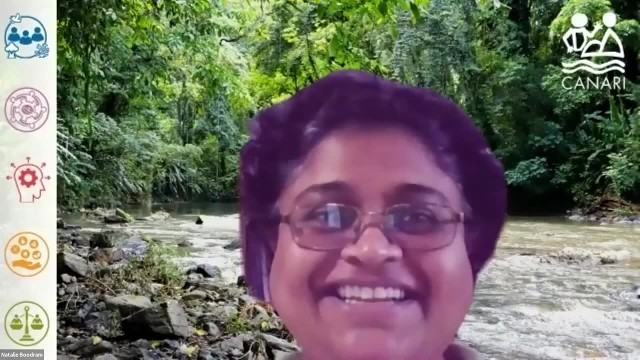 So, and of course, they are very aware of the project And I actually have some budget information I'm supposed to send which I haven't done as yet. But yes, it's, it's there, All right. So I hear you. 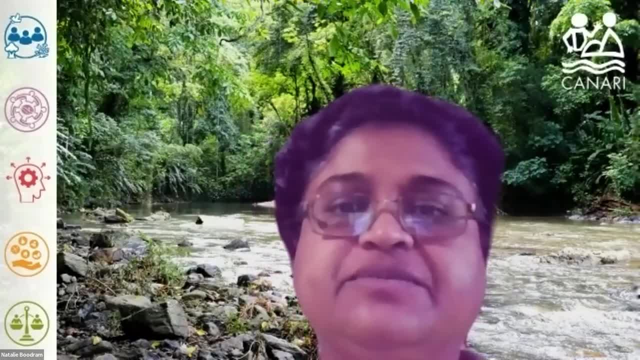 I don't have an easy answer, But we are trying and we're trying a slightly different mechanism which is focusing. To me, the reports and stuff is just step one. The bigger part of it which we've gone and got, got an extra. 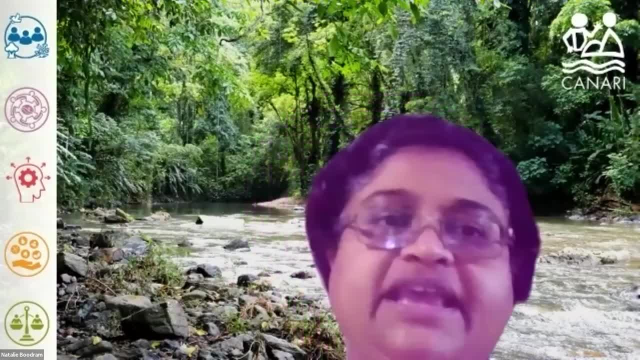 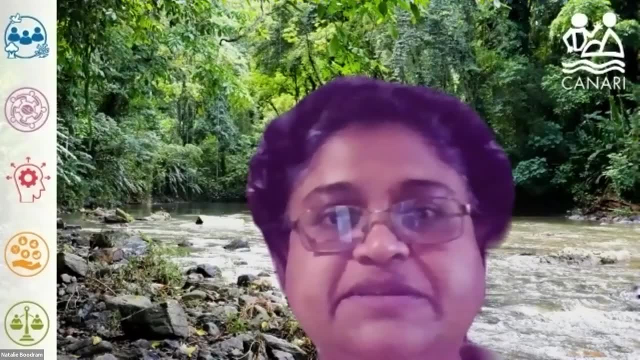 Yeah, We've got a lot of money for et cetera is to try to help communicate this information and make it out there. So all of you maybe have added fuel to be able to have these discussions, But I hear you. 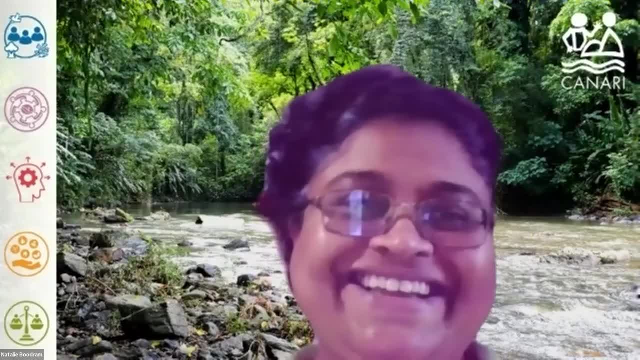 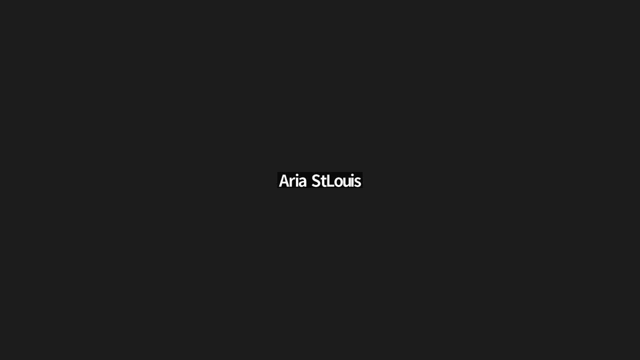 And it's not an easy answer. I don't have an answer. Yeah, Okay, Natalie. if you will permit me, I just want to highlight that, as part of the project, capacity building is also being conducted, And this was an important part of why we worked with. 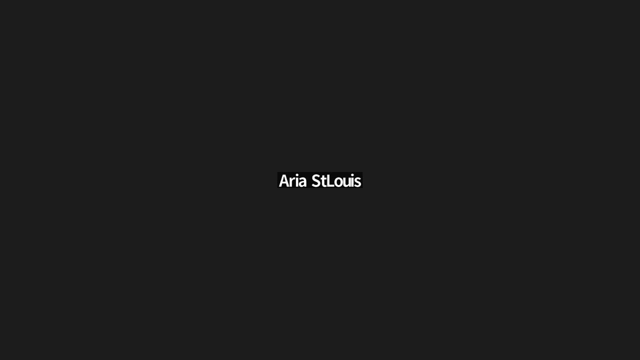 Canary, rather than picking a typical university that may not have had that feel for how participatory work could be carried out to help to empower community representatives to convey key messages to the community. So the capacity building that has taken place already in understanding and being able to value ecosystems and value species within ecosystems is another key part that hasn't been tried before. 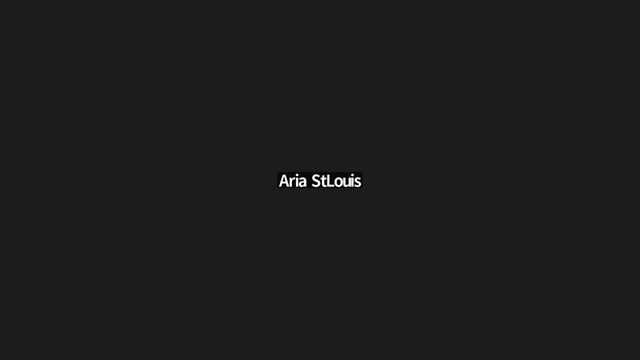 I think that that needs to be recognized And the efforts that Canary has made in order to even. I have to thank Canary again because they found additional monies. They will be conducting an advocacy workshop- an advocacy workshop, Not this, A separate workshop. that will help to understand how the results of this can be used for advocacy at the community level. 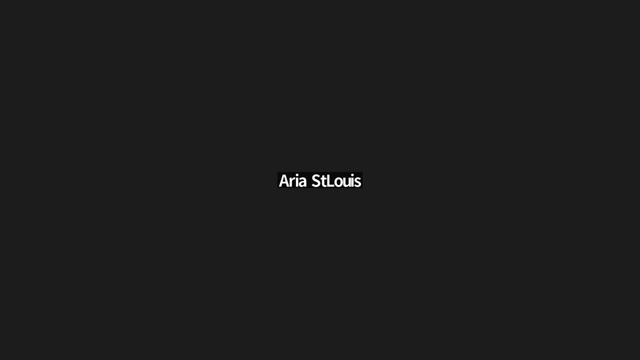 And that's distinct and separate from the monies that they got to produce the citizens guide. So, in addition to that, That is being done And all thrust internationally to raise the awareness on things like the value of our species, the value of our ecosystems, which perhaps through multilateral environmental agreements- which is what environment is responsible for at this time- and bringing that into 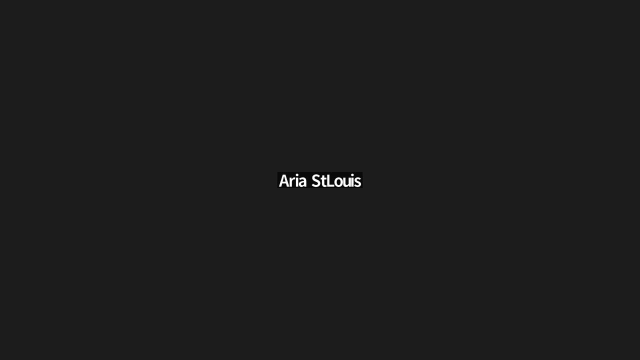 domestic action can actually put some pressure. but also because it's Canary, we have benefited already from- and these things are available on the Canary website- recorded sessions that build capacity and hospitality, And I think that's really important, And so the whole thing of building capacity and how to do things like valuation. 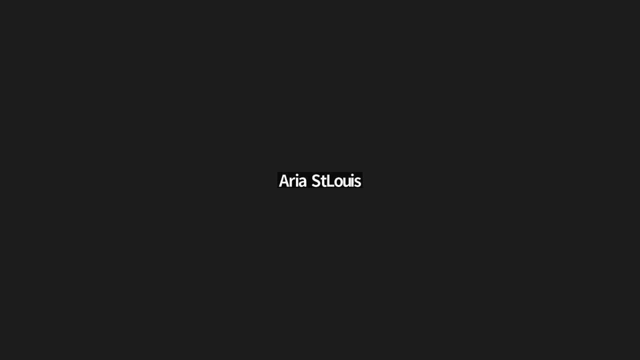 Thank you, Natalie. All right, Thanks very much. If I, if I may, I think that some of these, This workshop, that we talking about value in the ecosystems, We should try to get some of our policymakers involved in the economics of ecosystems and biodiversity, because that's a very, very important tool. 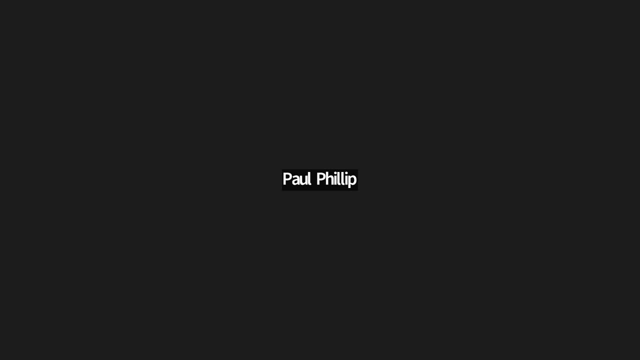 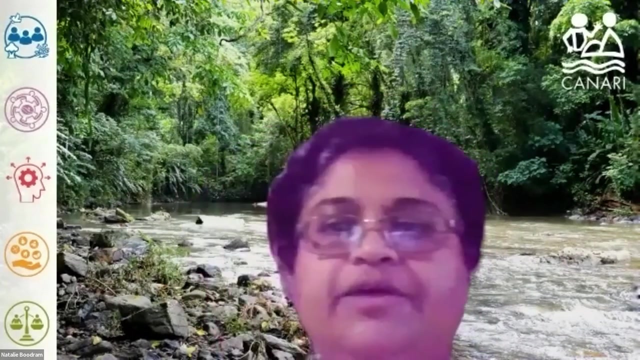 first we can use because, um, some of them, they see things only in dollars and cents and team would assist them to, you know, make sense of what is going on with with things like that, with projects like that. okay, okay, okay, okay, guys. so we're gonna go to our breakout groups right now. um, we're 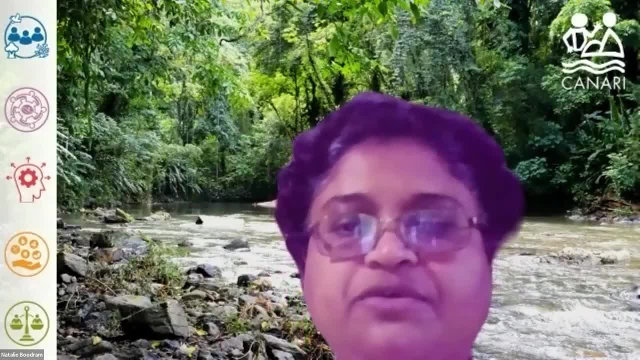 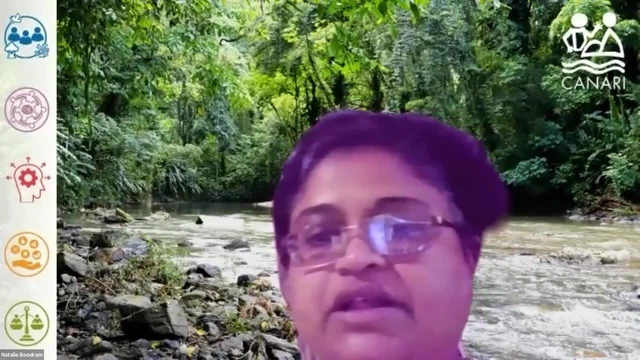 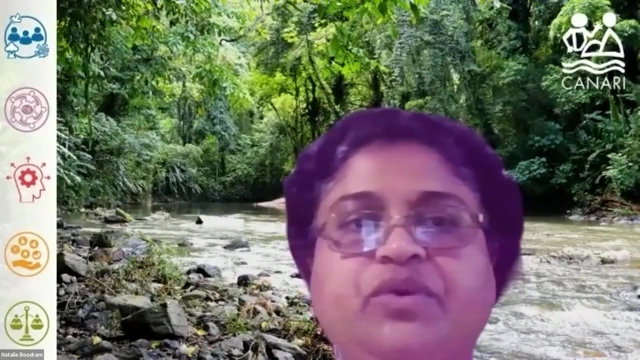 assigning people randomly, but please know that all the groups are doing the same questions. we have 30 minutes for the breakout group and then we will come back in plenary and we have three rapporteurs who will report on the breakout group um questions and session. okay, so we're going. 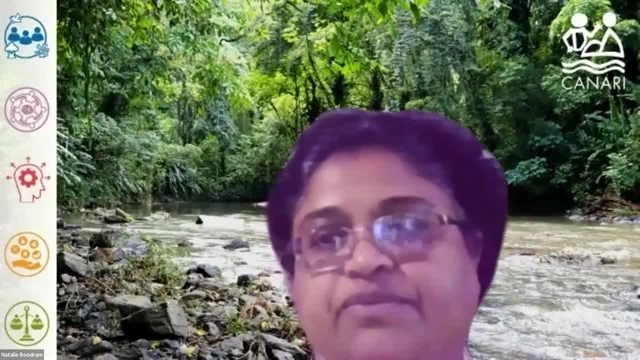 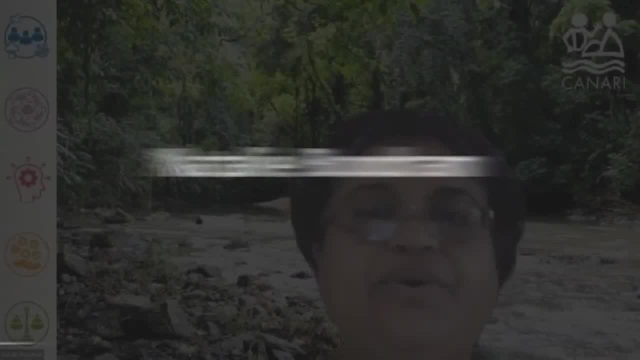 to go to breakout and after we report back we're going to take a short break. so, um, colleagues, anastasia, aaron, if you guys want to send us into the breakout groups, okay. so we're just going to go to the group work report in plenary and we're going to go to the breakout group and we're going. 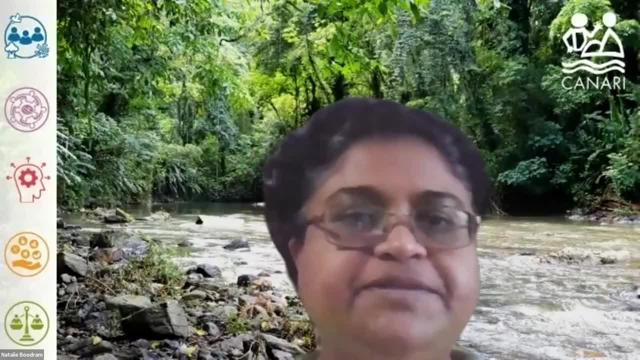 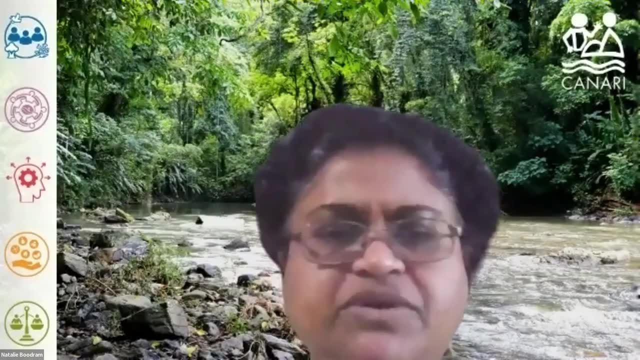 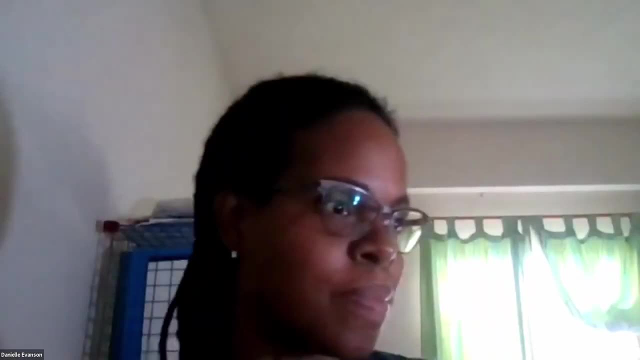 to take a short break and then we'll take a break. so each rapporteur has up to five minutes, uh, to just talk about what um the group spoke about. um, who wants to start? um, danielle, you were rapporteuring for one of the other groups, right? if can you go ahead, great, thank you um. hey, money everybody, uh, so 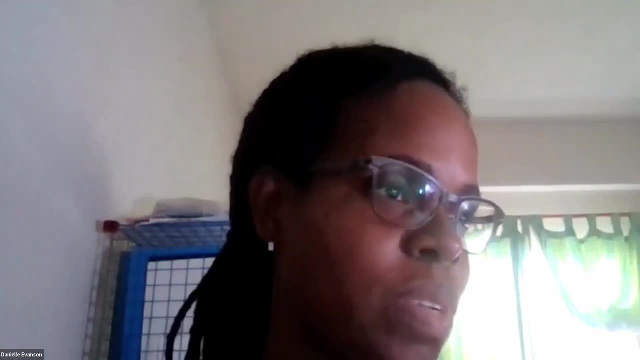 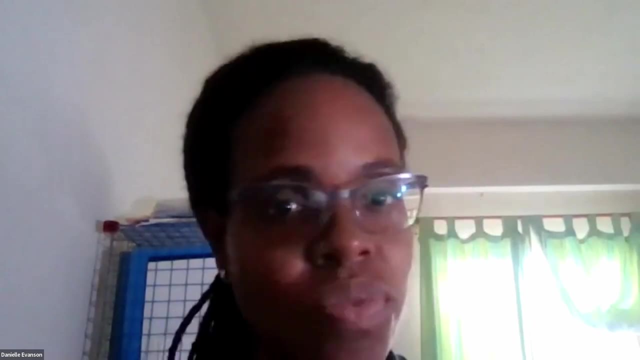 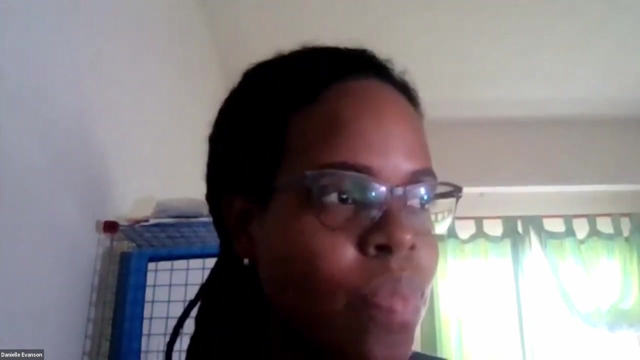 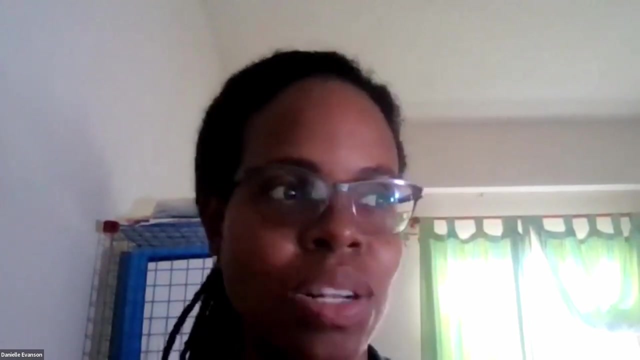 um, some of the things that we we discussed were: um, well, one, the. the group talked about the, the actual structure of the, the nea report, and how it's very, it's very, science-heavy. so, um, because the data and the cabinet, decision-makers and policy makers don't necessarily understand all those terms, um, we need them to be able to so that 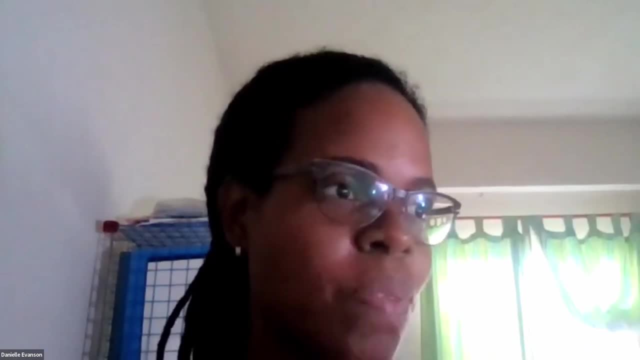 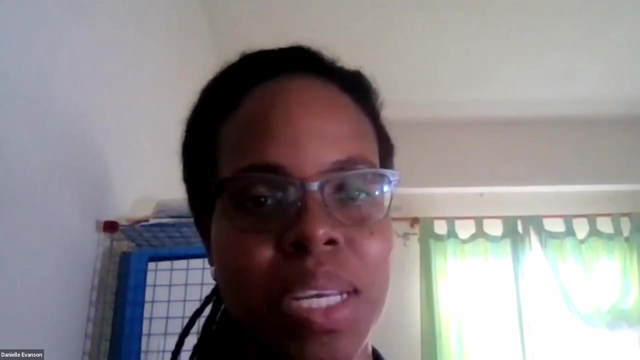 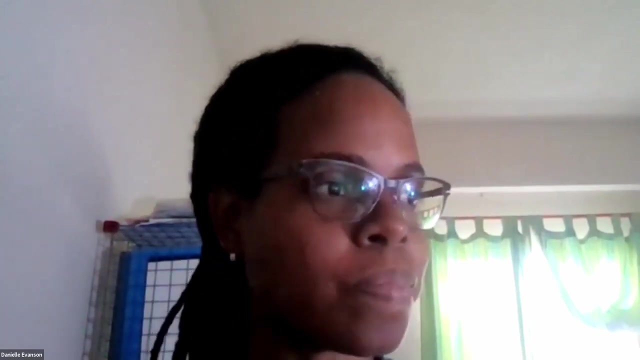 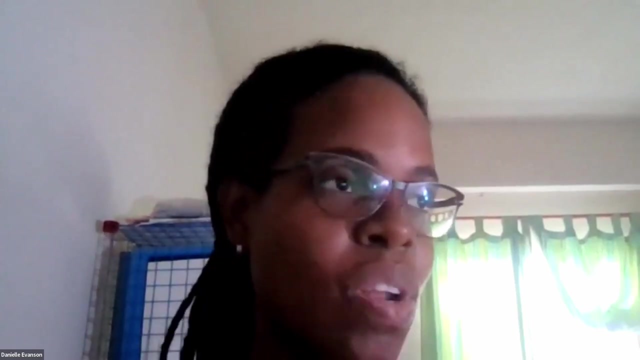 they can make more climate-resilient decisions and we need to frame the data for groups, um. but um, cindy mentioned that canary will be preparing the summary for the policy makers and the citizens guide, um, which should help to address those issues. um touched on the issue of having lots of consultancies, being signatory to lots of meas, having lots of. 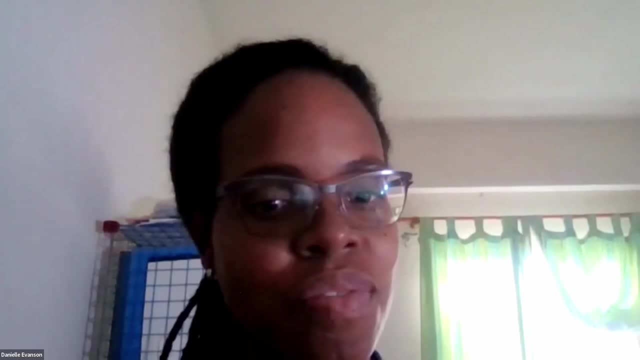 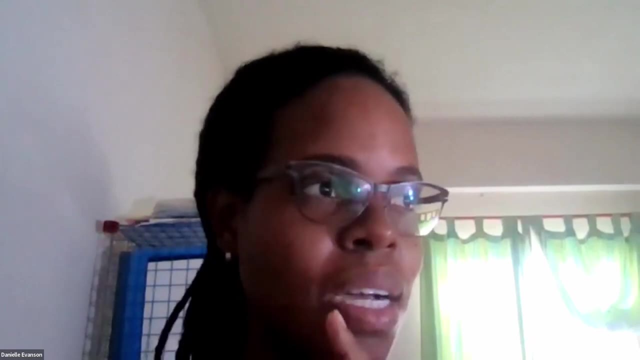 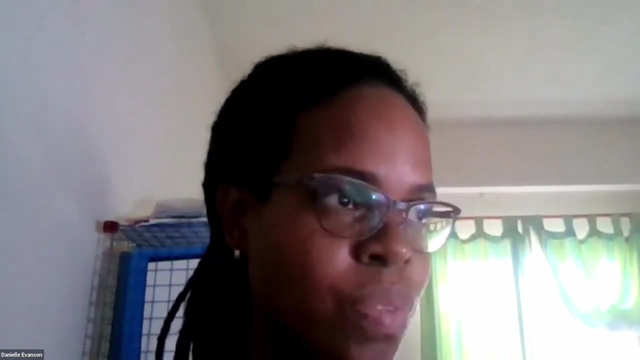 laws and funding and so on, but lacking enforcement of of these various things um, and there was also a comment that the government is um not just people in cabinet, but everybody um, including the, the public officers, uh, who are not necessarily um doing their jobs effectively. um in these spaces, um there was concern about um only 20 percent of of um the marine space. 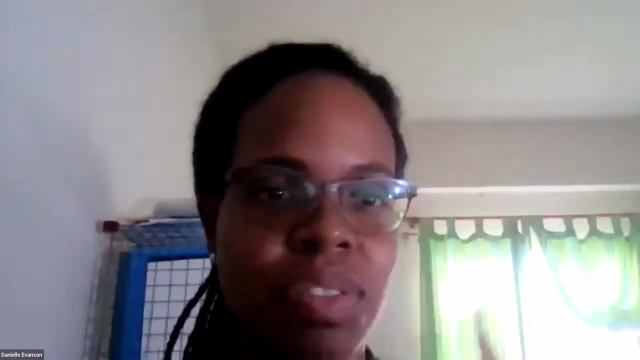 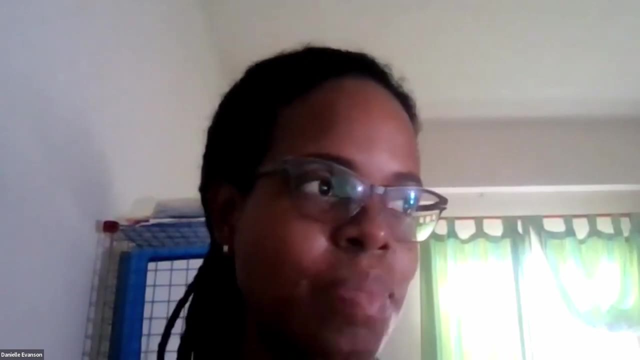 being protected, which of course leaves 80 percent up to the vagaries of of everything that happens um. and even in that protection it doesn't. it can't combat um sea level rise and and surface temperature raise um- and hayden did mention that very few bcci countries. 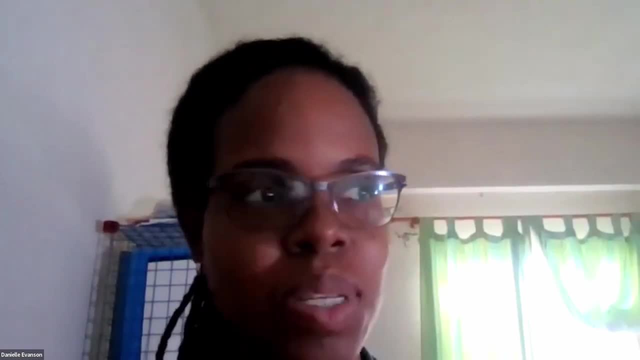 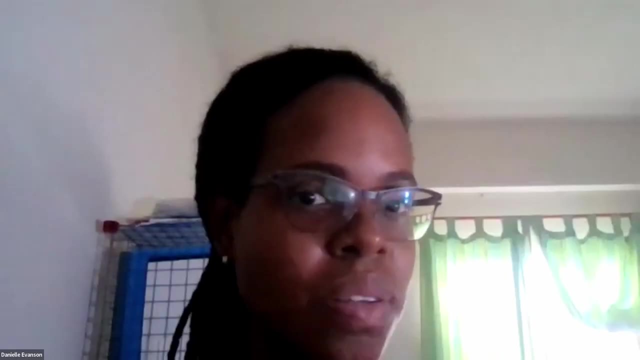 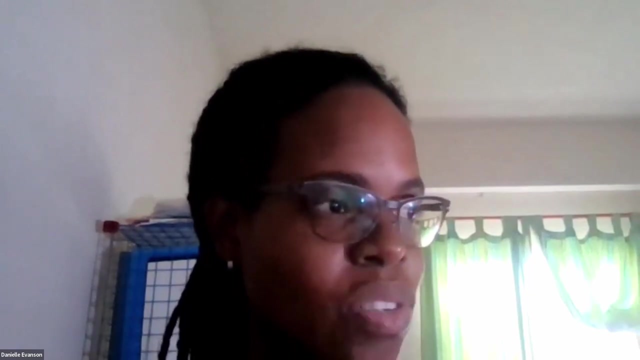 reached this 20 percent um figure and that it was missile. there was evidence that it was not much more than it being on paper. it's that contribute to ecosystem degradation, including the bushing programs that expose the soil um, the erosion and siltation and flooding and so on. how culture is used, an excuse for continuing unsustainable. 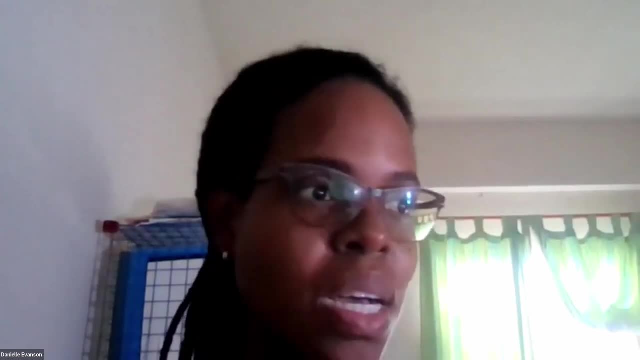 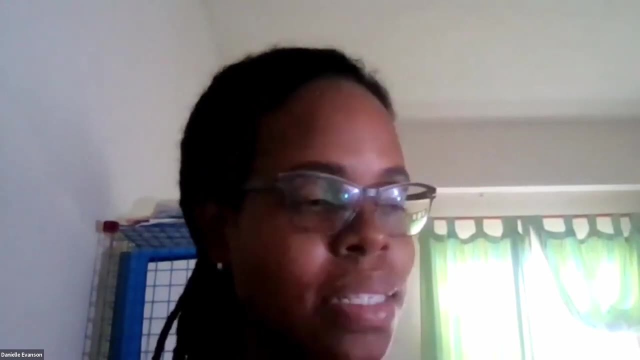 um so continuing to fish the overfish species, because that's what we do and that's part of our culture, so we'll continue to do it. um, and there's a potential double extinction of wilks and hermit crabs that are, that is, um looming, but people are continuing to to harvest, and um harvesting. 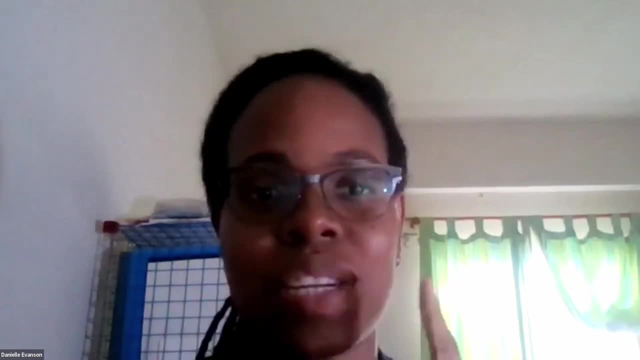 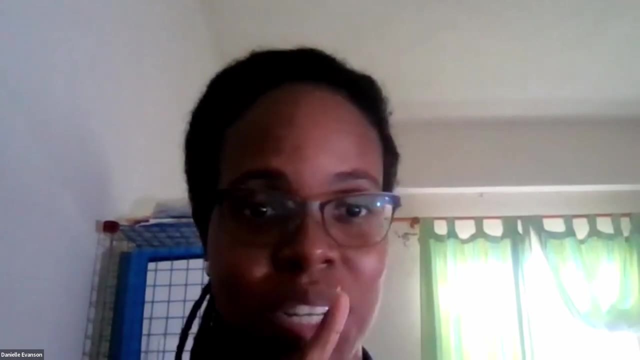 juvenile species, but calling it a different, saying that it's a different species, so that they can, um, the legal part of not being able to to fish juveniles, um, so they're calling it something else. so they're calling a cornish lobster, they're calling it some other name so that they can. 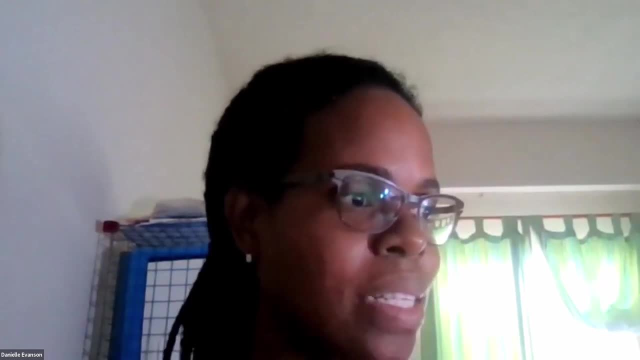 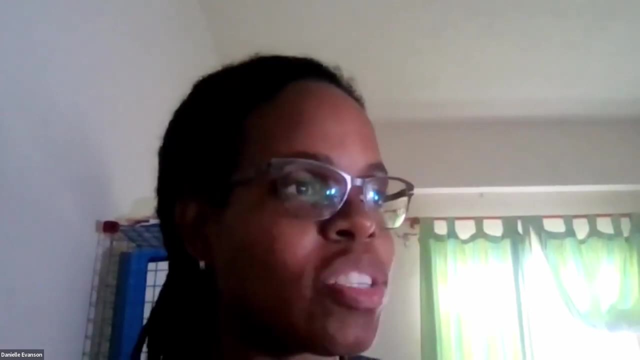 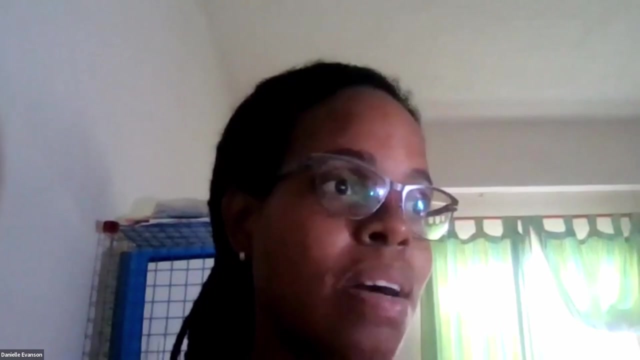 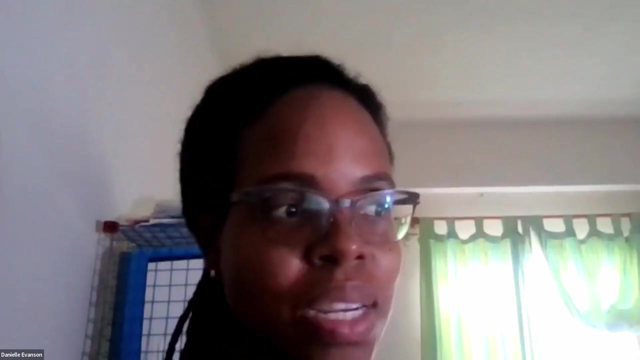 continue to fish it um, and there was a lot of discussion about public education, um how there's there's not much investment in it. um the only people who seem to be concerned and seem to be supportive are foreigners and um locals. um essentially, um actually disrespect the activists and um perceive them as outliers and complainers, and 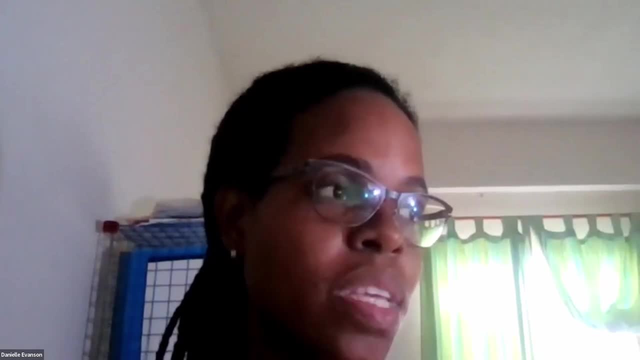 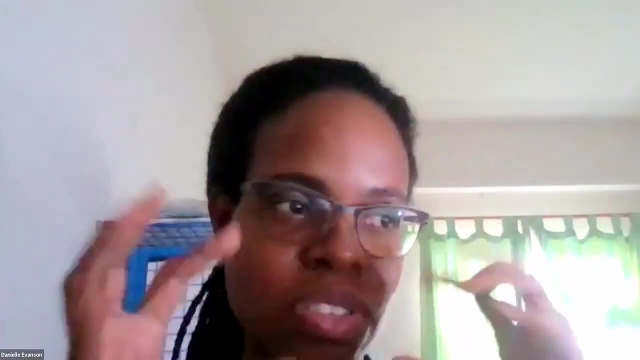 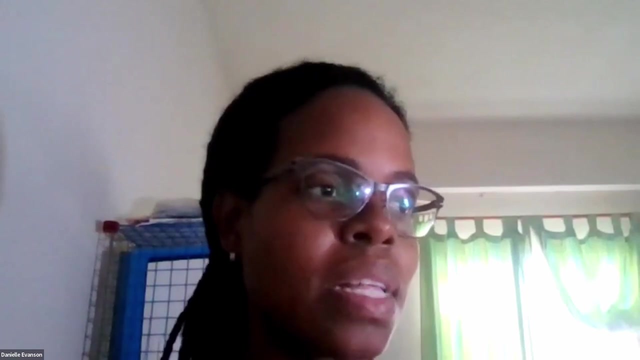 and disrupting um. so, of the recommendations, um, there's a need for the different environmental groups that are have, that have their little separate actions, to come together to to create um one big campaign and decide on the important messages and be able to that the activists become the, the focal, the spokespersons and and the, the champion. 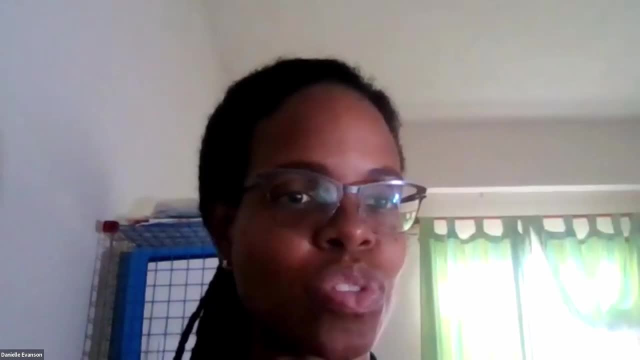 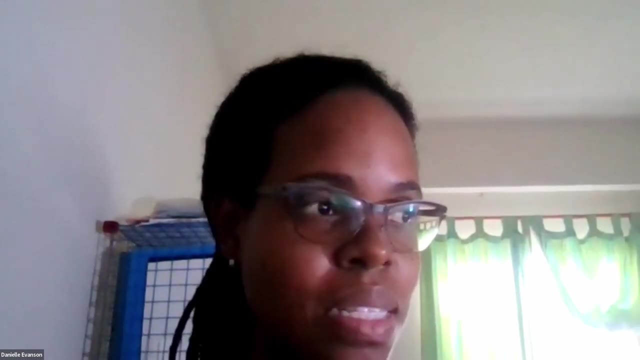 of the independenting of the kaoka and the, the middle class and theirceuple and theirsepties. um, in the while the people are fighting that, uh, the those expressions, that the people's, that they were showing up for and that they were saying that you know, if we don't, uh, we can't do this. 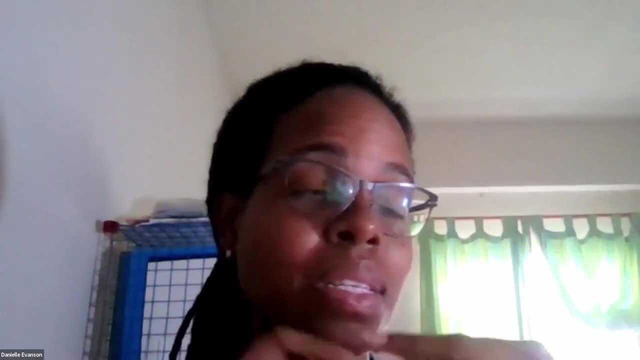 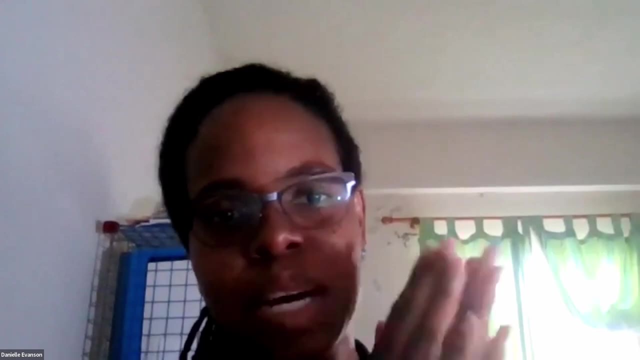 then they're just gonna let us down, um. so i think it's really important, for i think we're going to bring up some of the issues um because, once again, as a comment, i've been on the radio from two and a half years ago and there's um a lot of questions about the? um, the, the, the um, the. 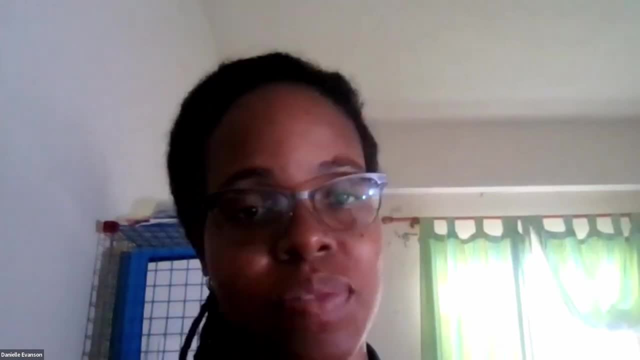 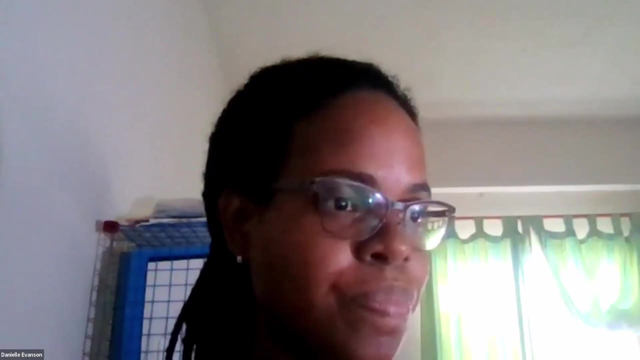 um, the, the, the of the, the the of the um, the, the of the um, the um, the um, the of the um, the, the um, the um. so, without the penalties, the system will eventually collapse and it will not be of any value if, if there's no willingness to enforce um, the, the regulations that are put in place. 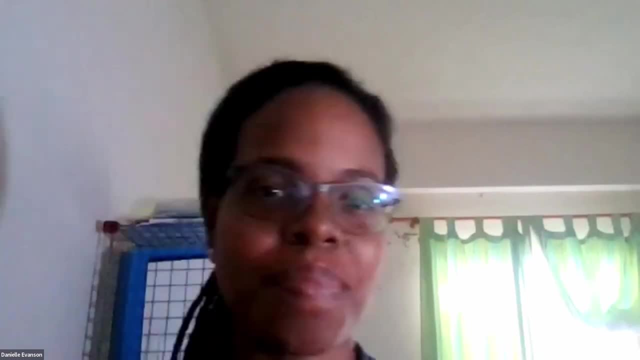 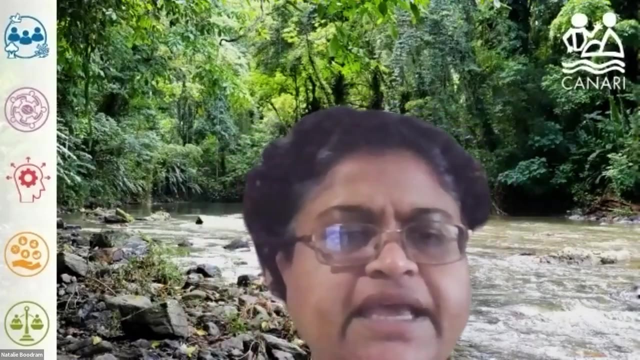 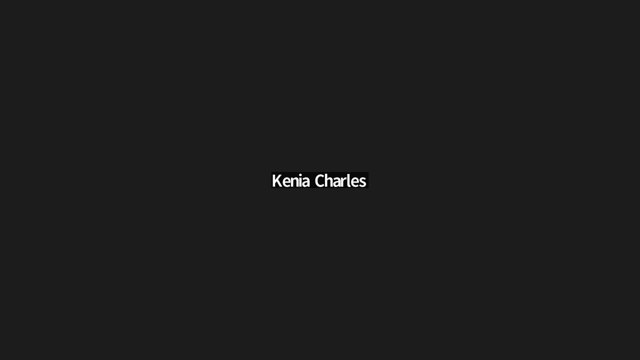 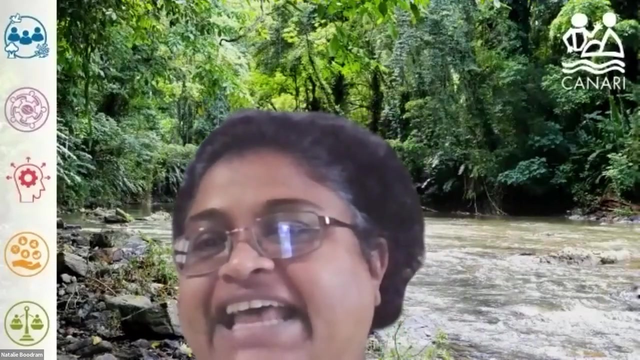 um, i think i'll stop there. yeah, okay, great, thank you very much, danielle. um, i will just ask for any feedback on what danielle said. kenya, no, i was just clapping. oh, sorry, okay, that was a clap that i had up. okay, um, and then uh, paul. 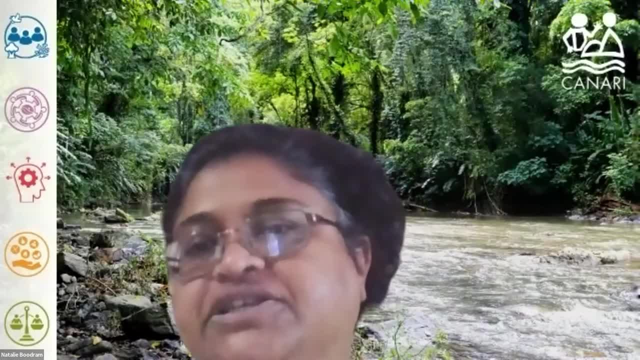 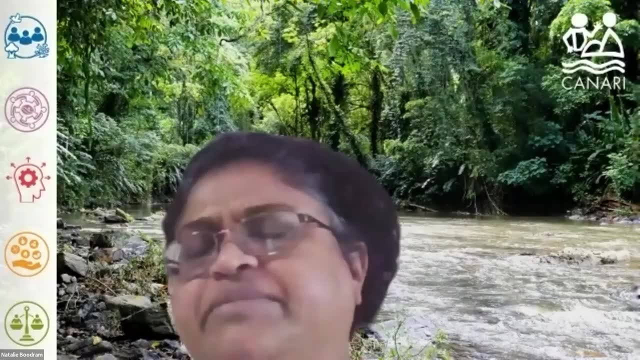 is talking about finding a method to expand, in general sense, entire knowledge of our policymakers, really economics, of ecosystems and biodiversity. all right, i'm not sure. i'm sure. what if i got that right? so i'm not sure if i got that right. so i'm not sure. i'm not sure if i got. 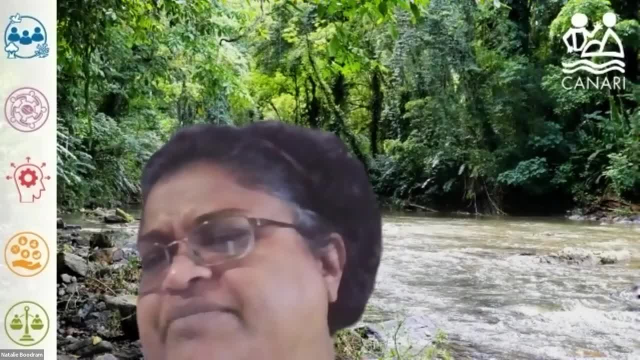 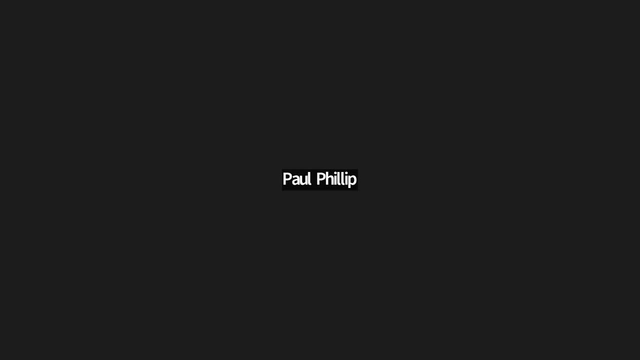 correctly, um, but basically i'm assuming you mean just trying to to make sure they understand the economics of it. so, um, could i please? yeah, um, i put up that um thing about the economics of ecosystems and um biodiversity. now it is important that people understand not only the economics but 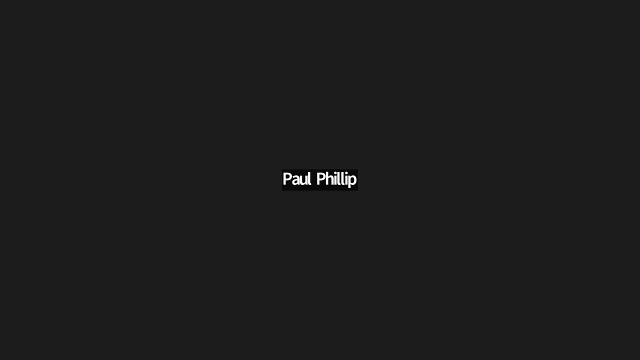 the importance of, of, um biodiversity, um and um. and if you don't, if you don't understand that because, for example, the, the, the we we have, we have had examples of um these people looking at destroying mangos to build hotels, but, in the end of it, if we have um a storm and there is a strong storm surge, 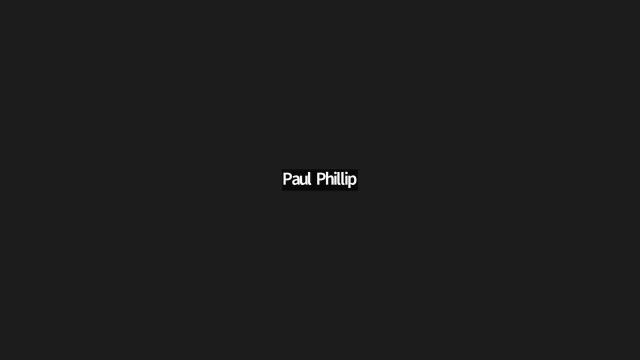 there would be, there wouldn't be any mangos there to protect their hotel. so what are we doing? you know exactly, exactly and um, just to comment on the, the first report. now i, i, i noticed that a lot of the um comments that were made in that group had to do with the 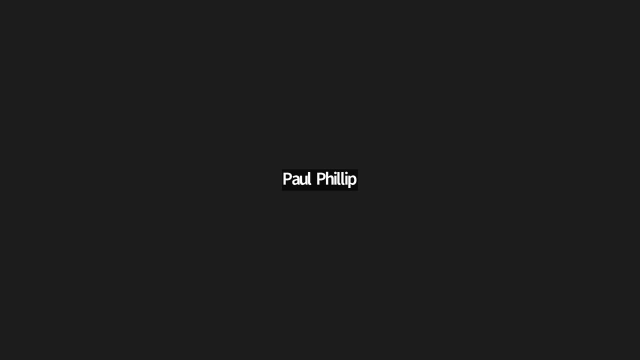 the, the marine ecosystem, and one of the problems that we have in grenada now is that the marine ecosystems fall under the management orbit of the fisheries division and, um up to this point, the, the fisheries division is not manned, um, there isn't even a chief fisheries officer. there are no officers in the fisheries division. 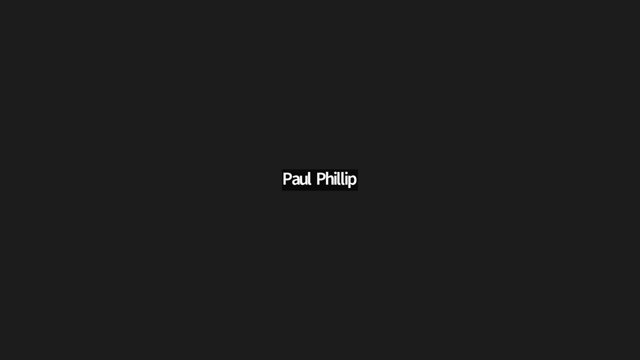 so there is and there is nobody to actually manage the marine environment. so that is a huge problem is there is a huge deficit that we have, and that is something that has to be. that is something that has to be corrected, um, sooner rather than later. okay, so that's. that's important to. 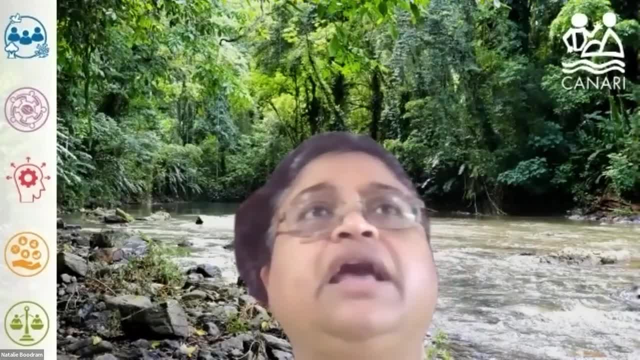 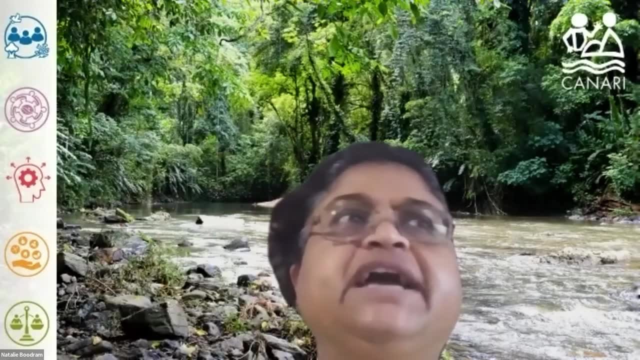 note. what i'm noting, though, is that a lot of these comments um are not climate specific, which is fine, so just saying: don't look necessarily for this comment in this chapter. i think we might reorganize some of the feedback. a lot of what we're hearing um is pertinent to the 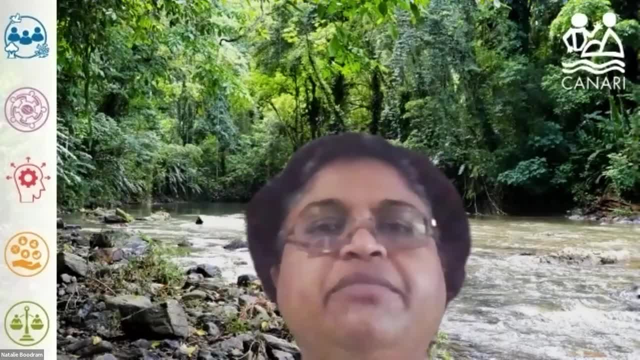 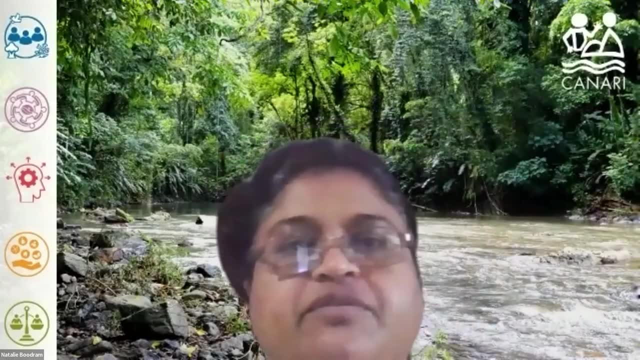 and the recommendations chapter. so, um, we may be putting that within that chapter, um, because it's more appropriate there. so just flagging that, um, the information will be removed as needed. okay, i see a thumbs up from hayden. alexander, do you want to try now? 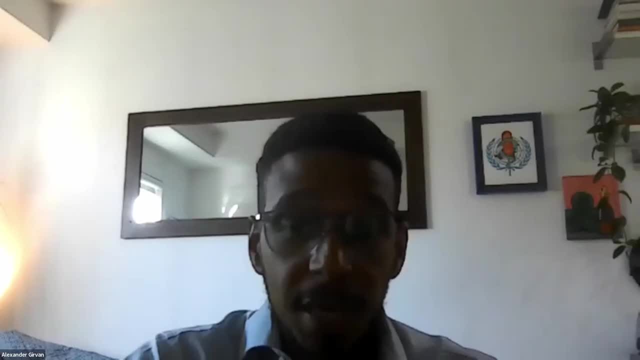 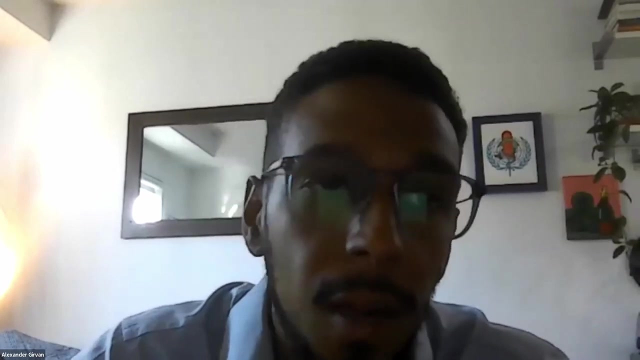 yeah, can you guys hear me? yes, okay, great, so i'm just gonna go through. um, sorry, let me minimize so i could see both, uh, my notes on the screen. so i'm just gonna go through the main points. um, from our group. um, natalie, please step in if i'm not doing this accurately, because i think you 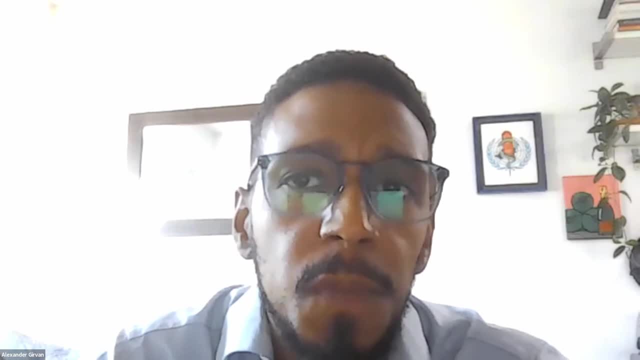 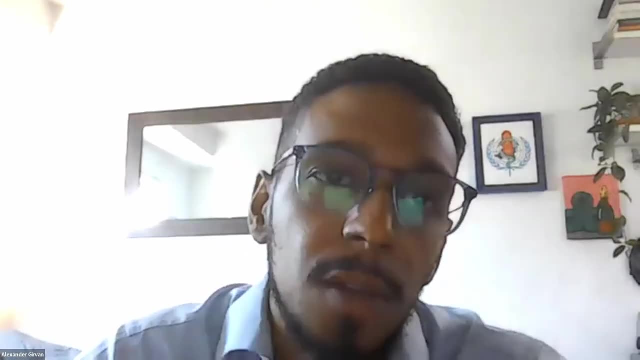 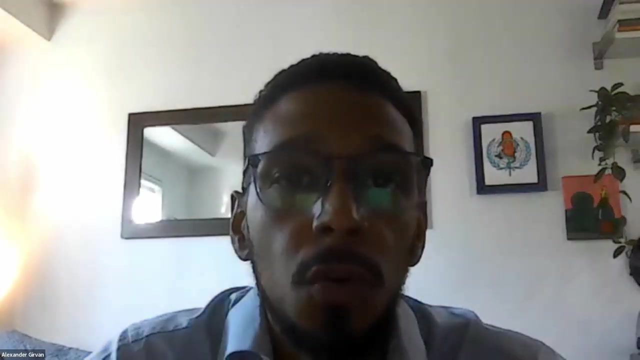 were really good at summarizing everybody's point afterwards. um, so when i came back, there were some concerns being expressed about the relationship between freshwater resources and climate impacts. so, um, someone noted that a lot of the impacts are driven by changes in the hydrology. um, you know, they said, uh, particularly due to changes in rainfall and worsening dry season flows. 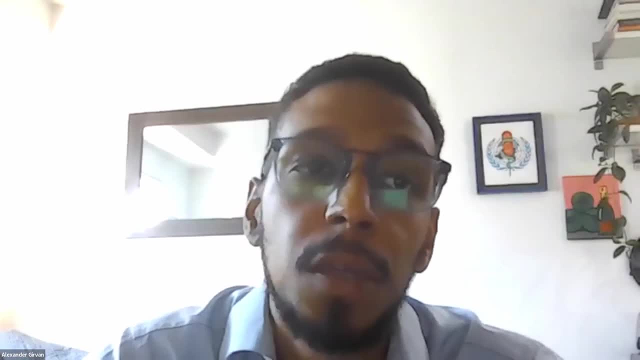 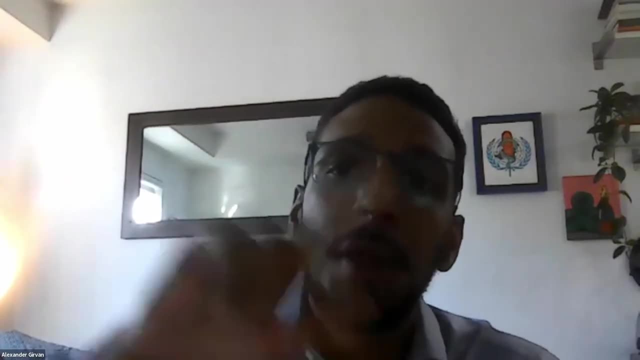 you know, flooding will also become more intense. but also important, it's important to note that there'll be changes in the vegetation um which were, you know, the third impact that was mentioned, which may also have a negative feedback loop. so you have lower dry flows, which may have a negative 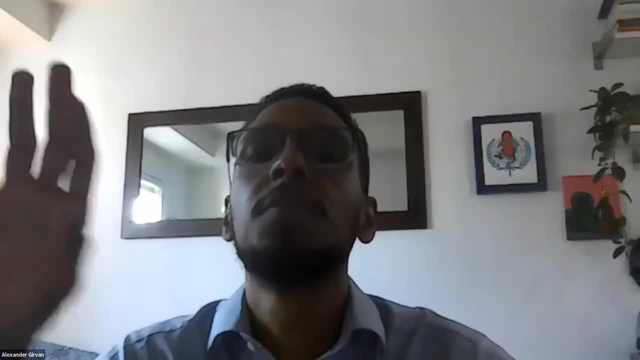 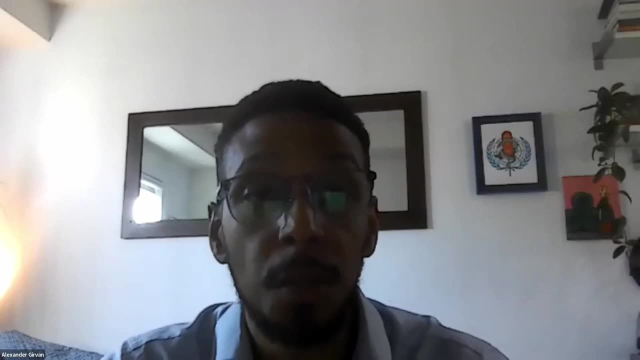 effect on the health of vegetative ecosystems, and it may also then affect rainfall and a kind of feedback loop. um, it was noted that rivers have disappeared in some parts of the caribbean. um, and there's a risk, of course, of rivers being lost in grenada, and somebody was noting that maybe these three points could be. 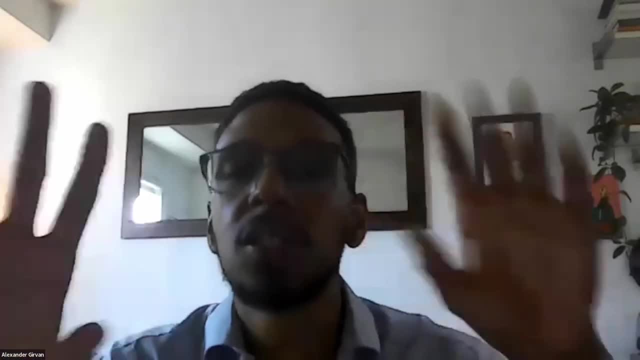 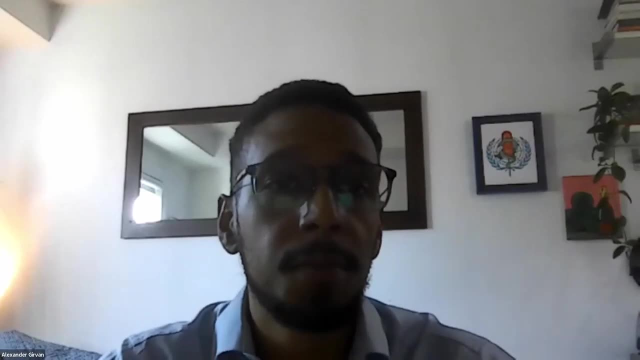 reinforced throughout this section, um to make sure that these risks are kind of highlighted, of these changes in hydrology and kind of the feedback loops between them um people. i think chris started by saying that this residential is extremely impressive, um, but brought up again the point. 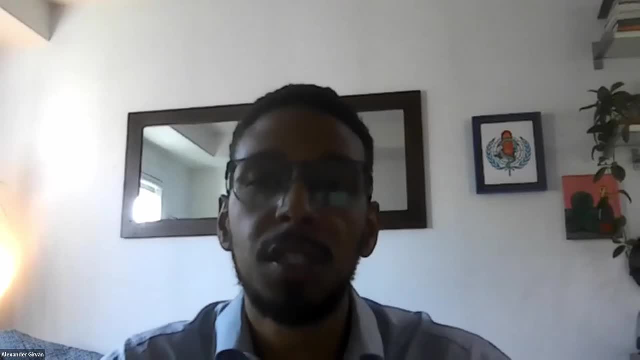 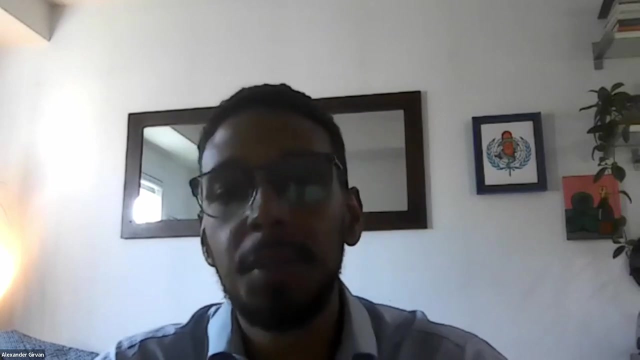 of us potentially being a bit diplomatic and actually, of course, explain um that because it's produced by the government, with the government, we have to be a little bit diplomatic, but also we're providing you with tools to then use this afterwards um the. i think chris noted that we were potentially being a little diplomatic. 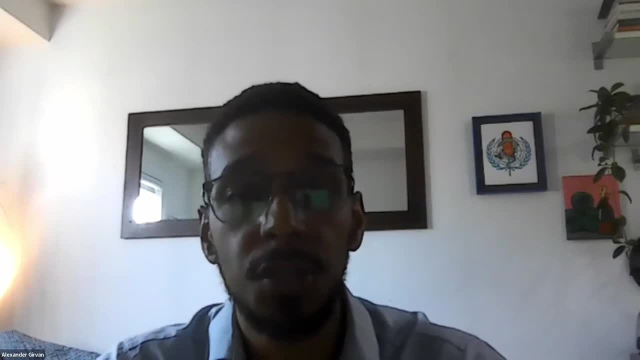 particularly about changes along the coast. um, from sauters, i think, was mentioned. um, and it was asked: you know, how do we describe these human impacts in the report and these human impacts interacting with climate change impacts? to make things worse, um, it was one of that. sand mining is. 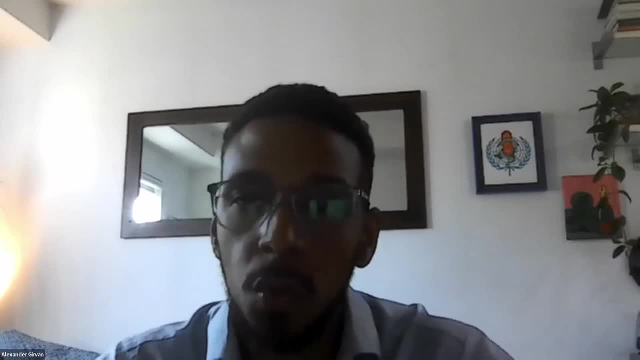 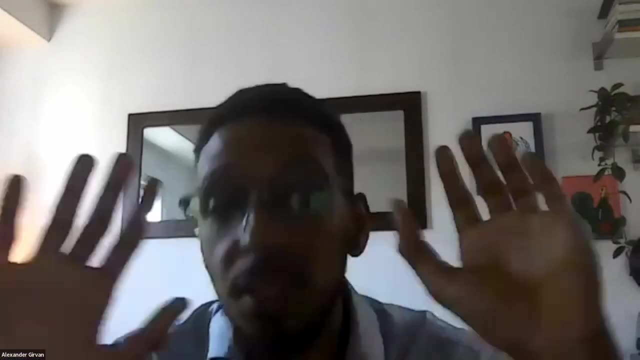 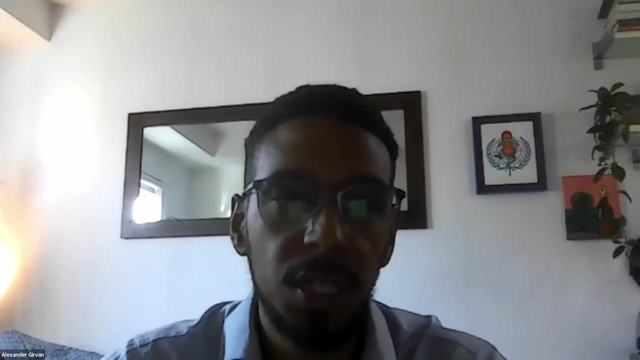 happening on certain beaches. so i'm not so sure of the chapter. just wants to note these, these interactions between human action and climate risks. uh, maybe something to reinforce throughout this section. um, just based on these comments. um, so, yeah, somebody also noted that human practices are co-stresses along climate change and, as well, it was noted, um, with reference to. 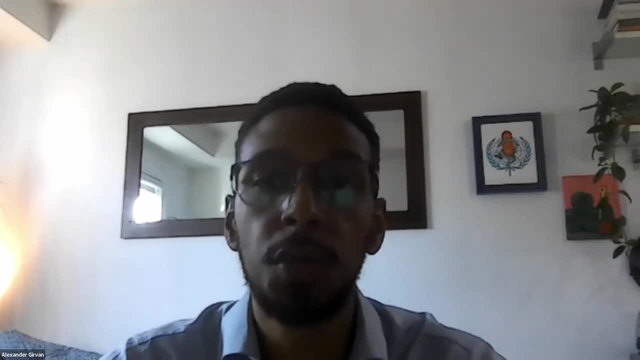 mangroves and i think somebody- just you know- mentioned this point. mangroves are truly important as a nature-based solution to to climate change issues and very important for climate change. so it was just kind of this idea of these co-stresses um- someone noted that- um sea level. 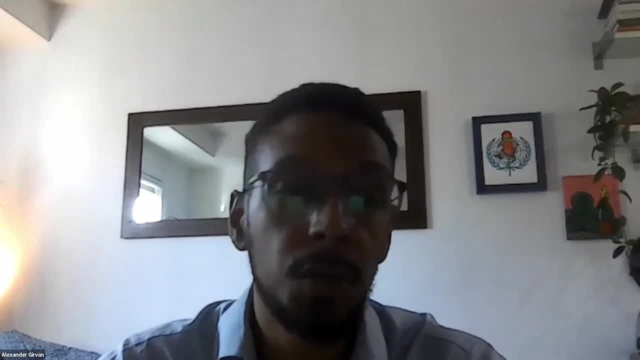 rise and coastal erosion and lava. that was really, you know, strongly noted as being eroded by meters and somebody said it's possibly the fastest coastal erosion in the region, um, and it also poses severe risks to inland transportation and to roads. so it was a severe risk to a very important. 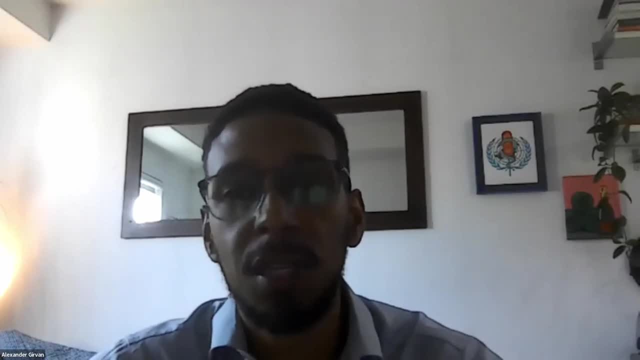 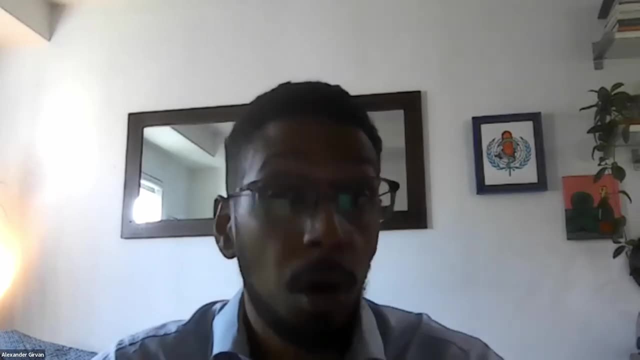 coastal infrastructure and transportation and i think aria noted that um some of the some routes, some new routes may have to be found because of losses of these coastal roads, which of course, are quite severe impacts. um, from the agricultural perspective, i think someone noted that we must also consider soil health and soil microbes, not just the effects of inorganic 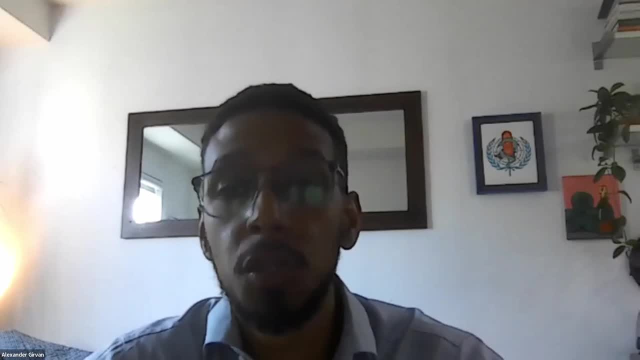 fertilizers. somebody said soil development is key to kind of food security and resilience, so i don't know if something can be added. a line maybe about the risk of climate change to soil health and so on. microbes- so leave it up to the traps to decide. natalie also mentioned the 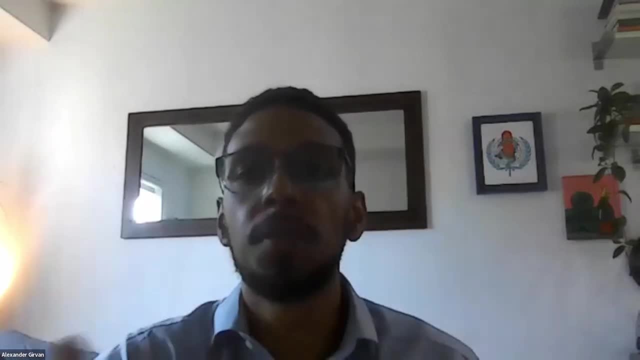 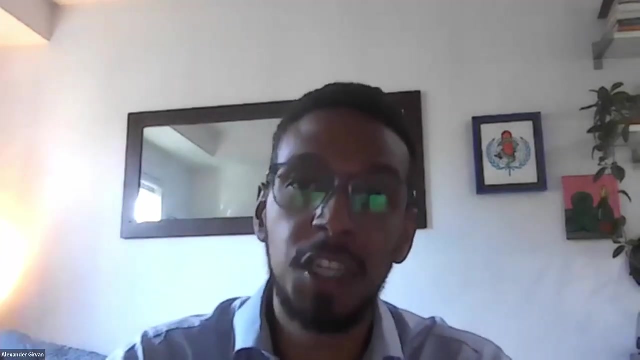 next slide: um, um. so i just want to very briefly refer to this finds um the, the issue of climate protection in the caitlin and roland carrier crew as a key part to climate resilience, and this conversation about mangroves and other ecosystems being very important for 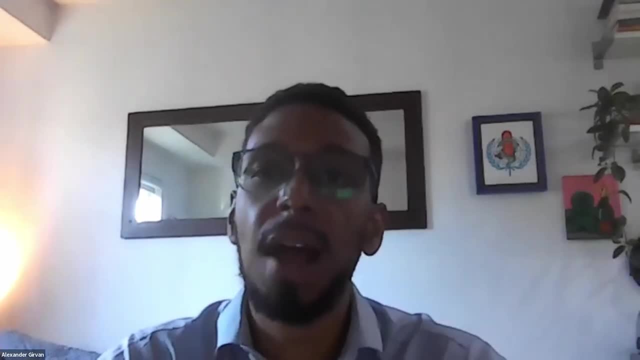 um being resilient particularly to extreme events, and um somebody finally closed it off by noting that um this feedback loop again of cutting down vegetation for agriculture, cutting down vegetation for other types of development having a negative effect on rainfall. so basically saying that rainfall is under pressure from climate change, but all these other human activities are placing a very significant impact on our climate and on other economic activities. 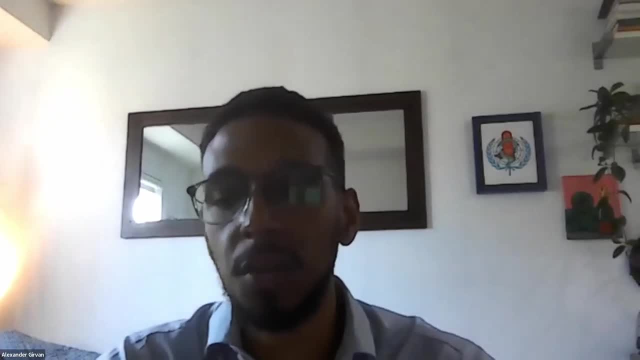 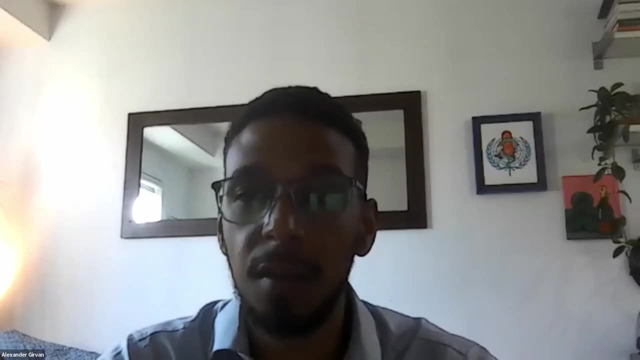 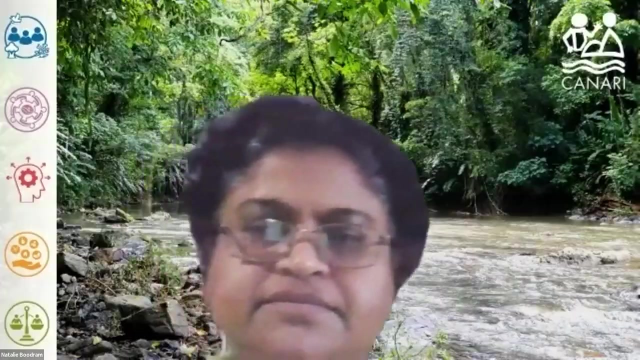 stress on rainfall, on the water cycle in Grenada, which of course presents significant risks into the future. So these are the main points I have. Nathalie, I'm not sure if you want to swing in and do any. No, that's fine. Thanks very much, Alex Rhea. Hello everyone, Can you all hear me? 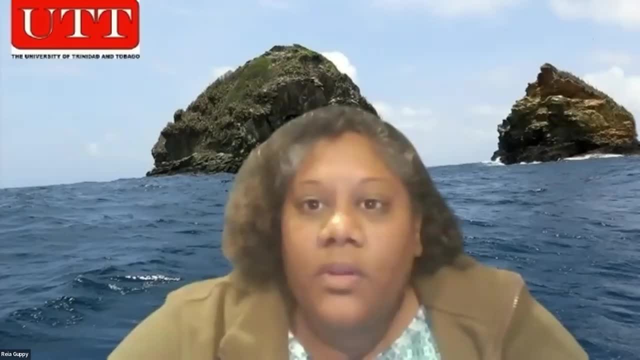 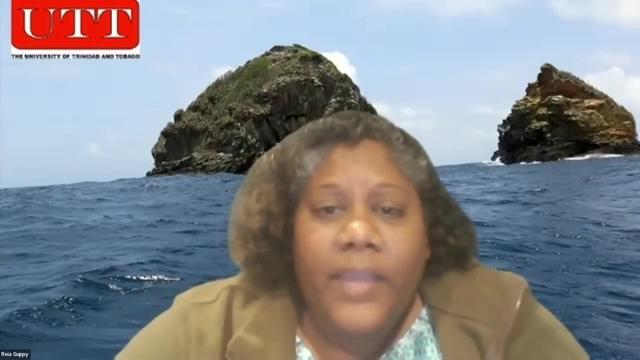 Yes, loud and clear. Rhea, Okay, lovely. So I was rapporteuring for Group 3, and, generally speaking, it's quite interesting that the groups touched on so many different things, because our group, while they generally had, and they started off a little bit shy. 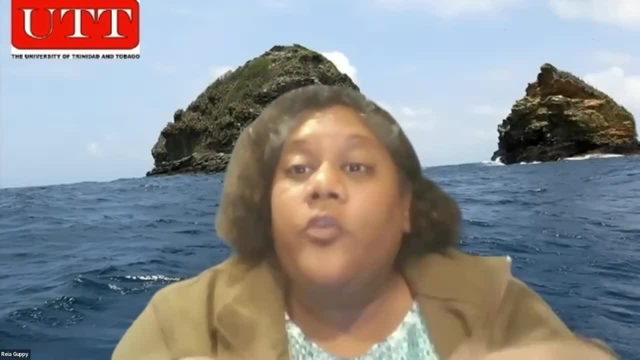 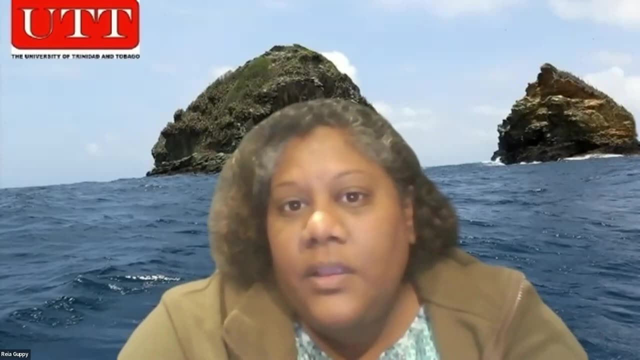 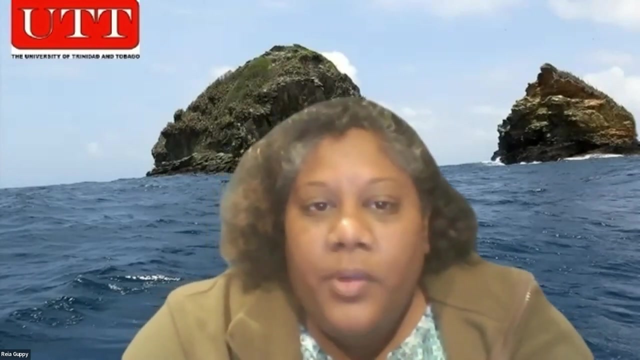 and we started off with basically how much they agreed with the presentation and they were very happy especially to hear the importance of mangroves and Dallas accent the reefs. But they noted that the presentation kind of focused more on the natural causes and or 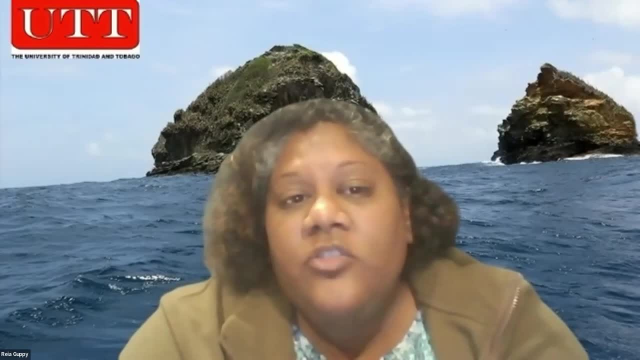 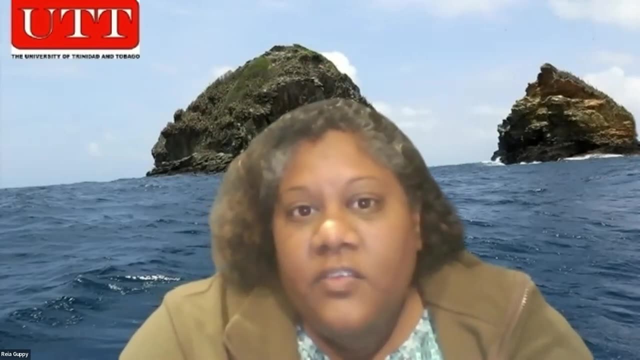 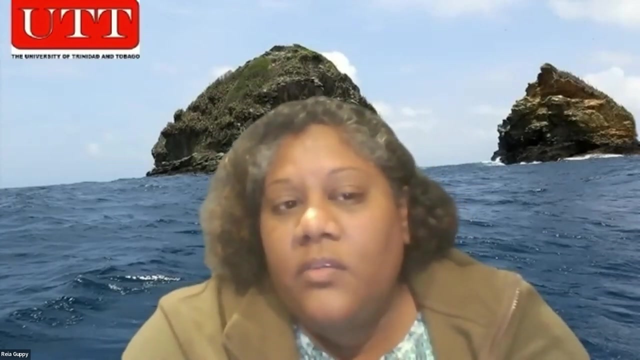 impacts as it related to resilience and climate change. What they would like to see if it's not, there is an emphasis on the impacts that anthropogenic activities are having on the specific ecosystems And, a lot of the time, the works that they do involve the reefs, looking at the physical, natural, scientific and social impacts. That's the concept, And they also started to focus on the effects of climate change on the social and economic impact of highways and small-scale legislations. They wanted to create a space that exacerbates climate change impacts. They just want to make that connection a little bit stronger, And the example that was provided by this was a coral reef example where for a lot of their reefs they're being destroyed by lbs pollution- land based sources of pollution- and with the reefs being destroyed, therefore any sort of climate change impacts would be that much greater. So they kind of just want to see how this works. 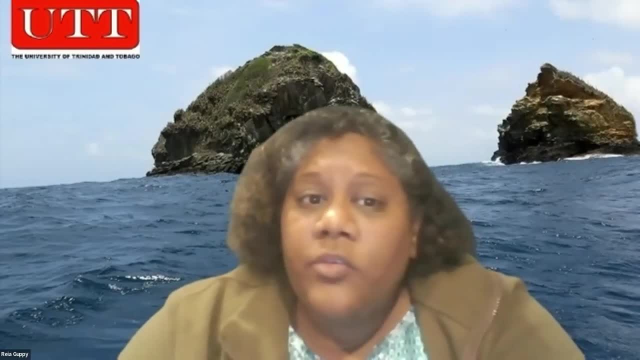 So how can it be that this is a whole range of examples of things that they can be familiar with and that they're working with be that much greater? So they kind of just wanted to make that a much stronger linkage to come out a little bit more. Mangroves and coral reefs featured quite a lot in this particular group. 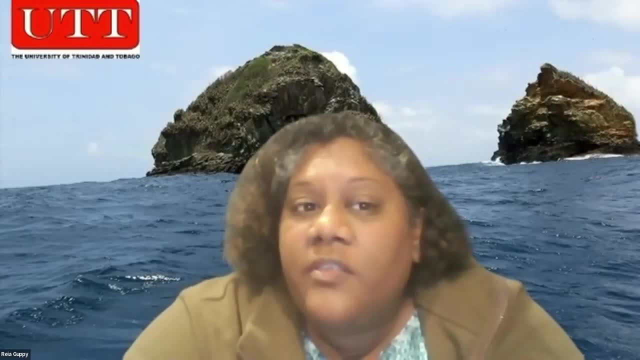 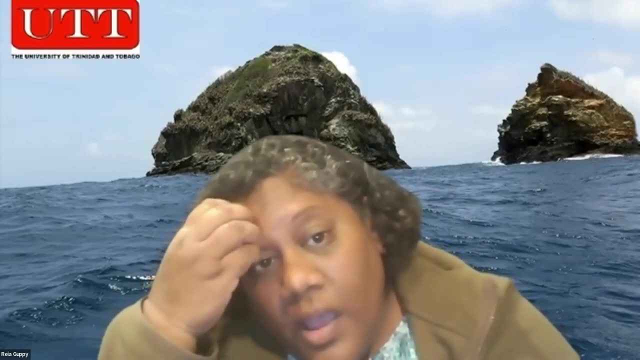 and these were some of the main ecosystems that were of concern. However, from further discussion, coastal agriculture was specifically highlighted and the examples. there were a couple examples that were used on the east coast of Grenada. They have a lot of cash crops and subsistence farming. 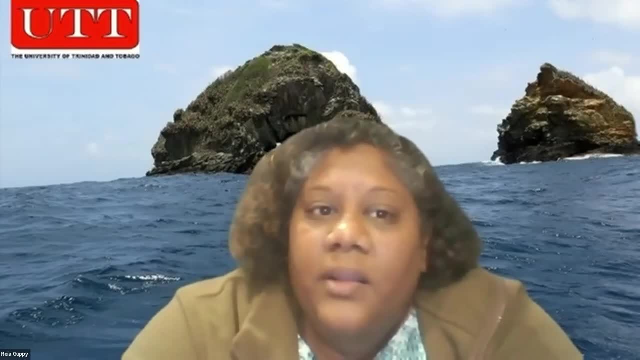 that is typically done, but they are already being impacted by sea level rise and salt water intrusion, and they had noted, of course, that a lot of coastal areas are being degraded, partly from developments- and I might get the name wrong: Lavera developments and some of the gold. 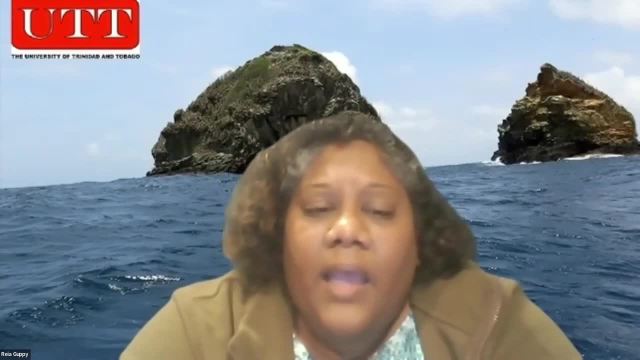 courses that are being developed there, And so, even though some of these developments may not have come to fruition, the removal of vegetation for such developments had already occurred, and they are already seeing greater impacts, as it relates to erosion, on those sides Exactly, Especially since on the east coast of the island there's generally less rainfall anyway, and so, with 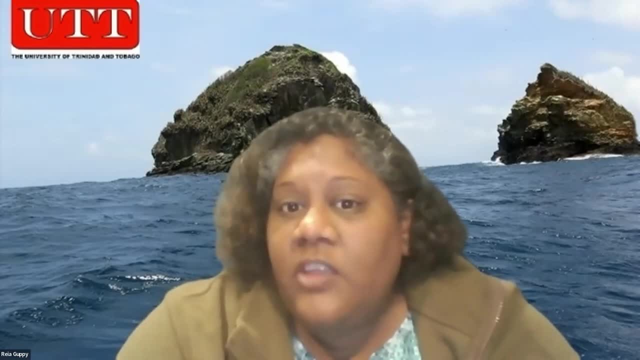 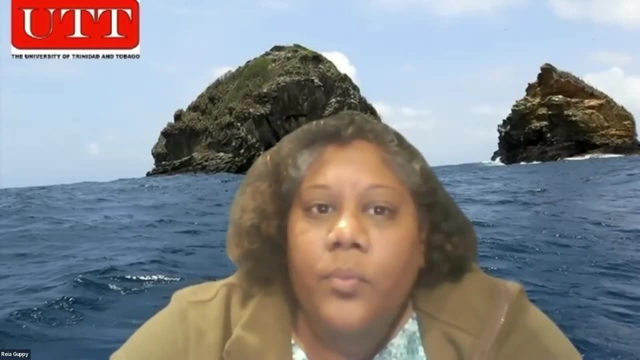 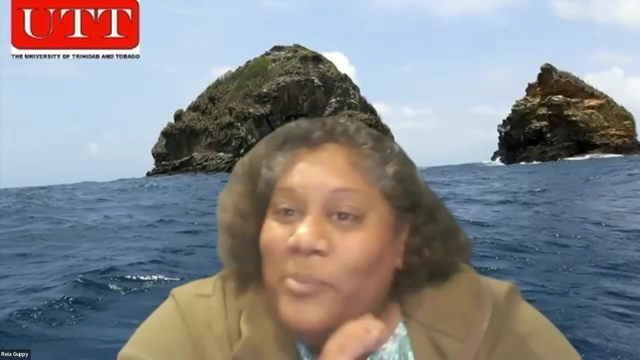 the reduced rainfall and removal of vegetation. there's been a lot of soil erosion that's occurring. Then we went on and moved on to some of the examples and, hey, I got very excited. I know I'm not supposed to, but I got very excited because we got some. 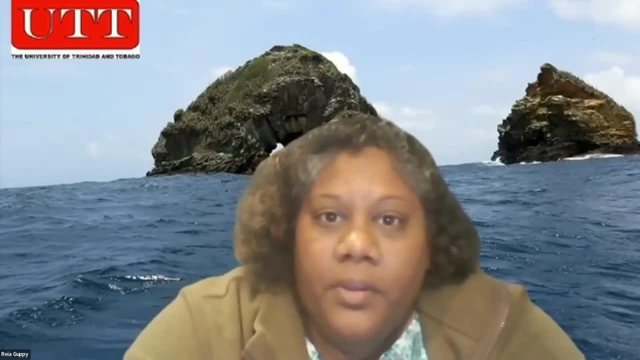 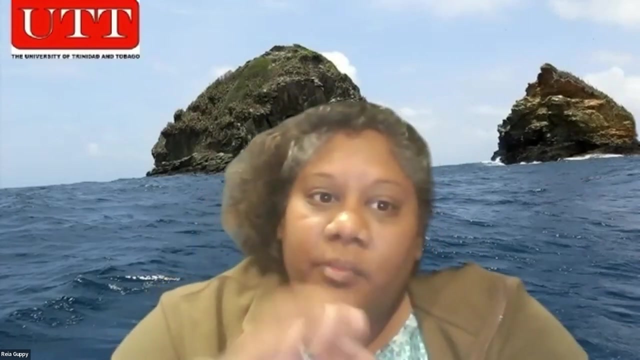 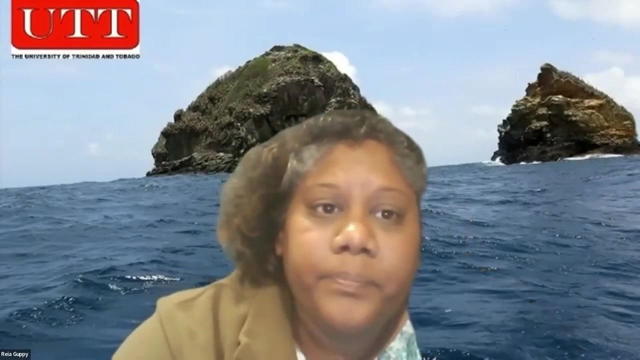 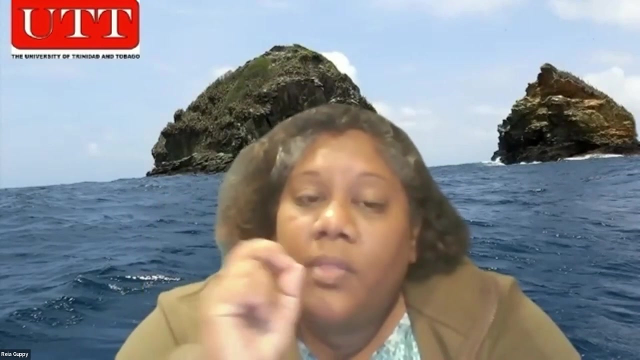 very good intel from a couple of the group members that you know two examples of how we can do some very low cost but very important changes to improve climate resilience. We had a group- and I have names within the report that are two different examples- examples of the same thing- where they would have um transplanted sea urchins on reef areas, um. 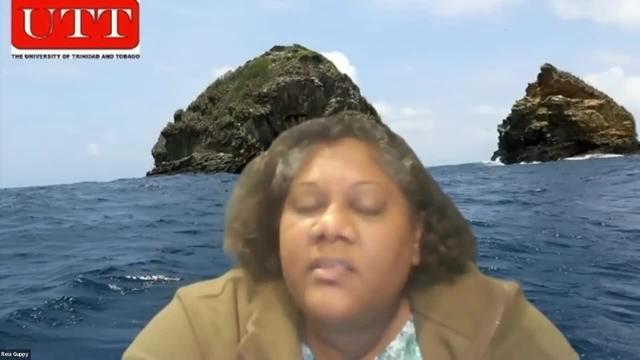 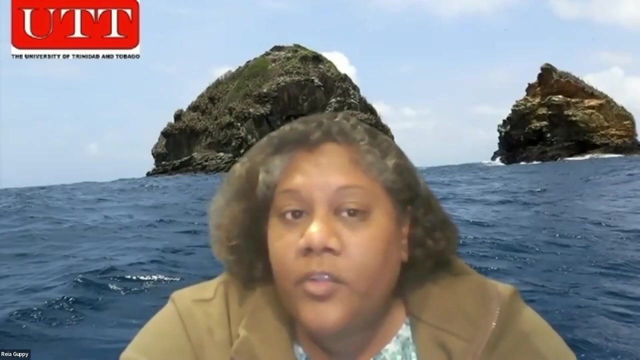 within and or right outside the mpa areas and they saw a marked improvement um in terms of coral health. so we have specific data, videos, photos that can be made available um to the chapter um that will show examples of how. so the in the information we got was, for example, they moved. 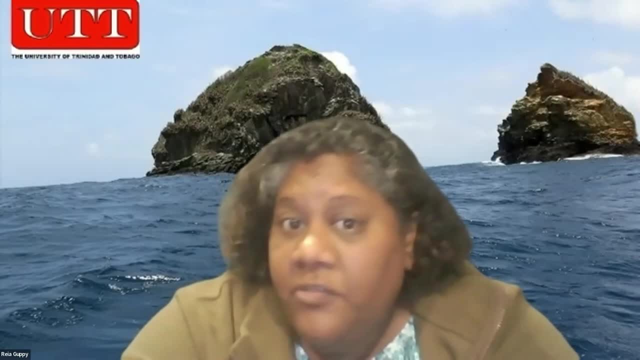 5 000 urchins to um five different dive sites outside of the caracoo um mpa, and within four months they saw an improvement. and this has been going on, i believe, either within the last eight years or the the effort was within the last eight years, and then there was a second example, similarly 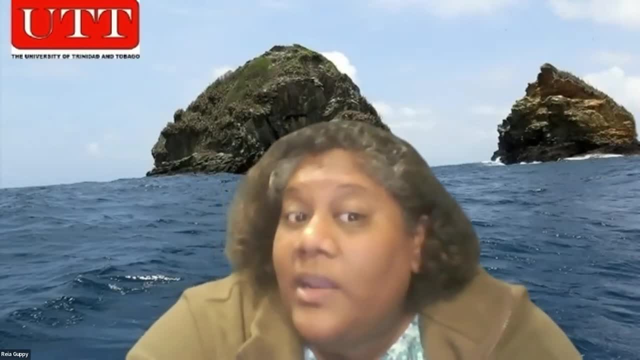 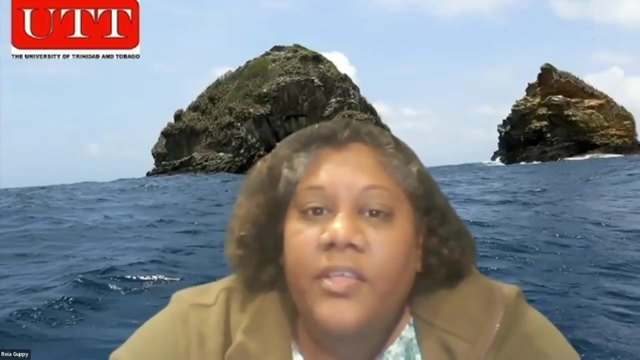 from the abusion um the molinier mpa and um again. they moved urchins from the uh granance area and um into that mpa area and they've actually found the reefs turned around pretty quickly. this uh completely second example, besides urchins, um that is, i'm not sure if the data- 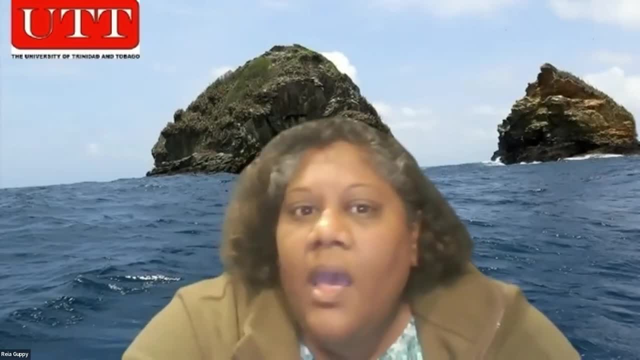 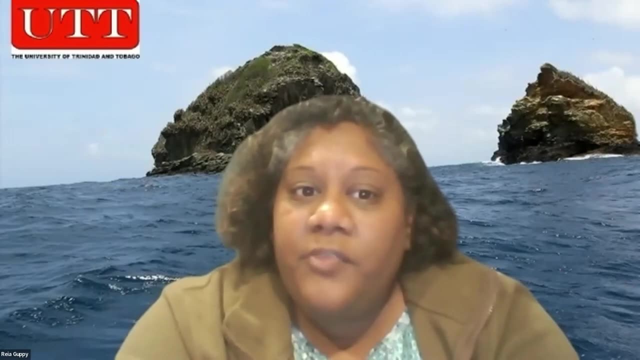 actually supports it. but at least the sentiment is there that the um, their reefs around grenada and those uh on the east coast are generally less affected um from runoff etc. compared to the west coast and given all of the mining activities, the east coast uh is having generally less erosion compared. 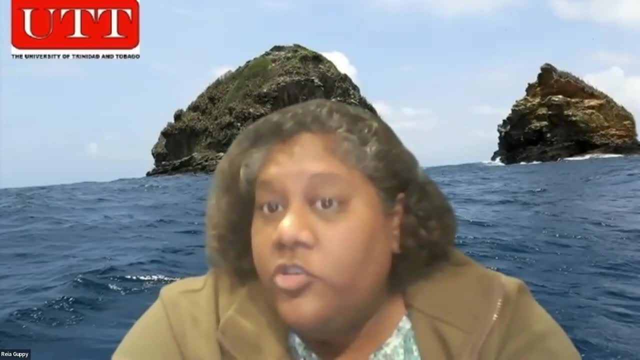 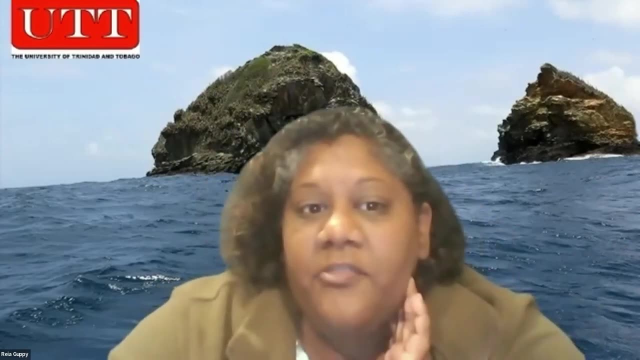 to the west coast, and the group felt that that was attributed to the offshore barrier reefs that are less impacted uh compared to the west coast. and then, finally, uh in terms of specific measures that can be used to measure the risk of erosion and the risk of erosion and the risk of erosion. 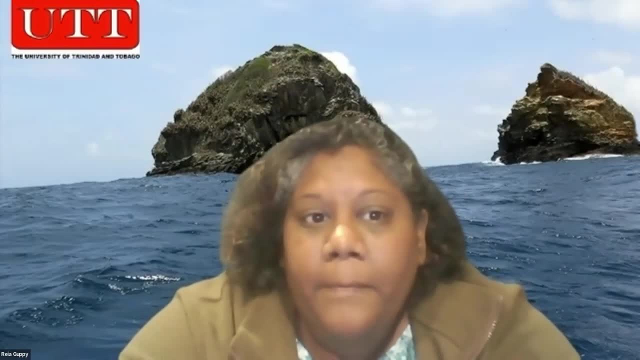 that can be potentially done to increase resilience? um, uh. one specific example was brought up in terms of the plantation of moringa trees, and they have indicated that these specific trees are um have been noted to be at least 20 times better for carbon sequestration, and an estimation of if a 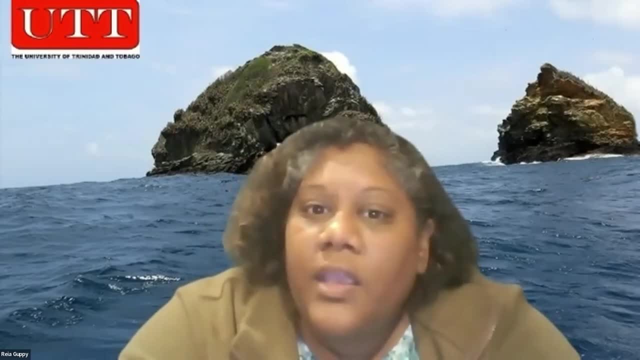 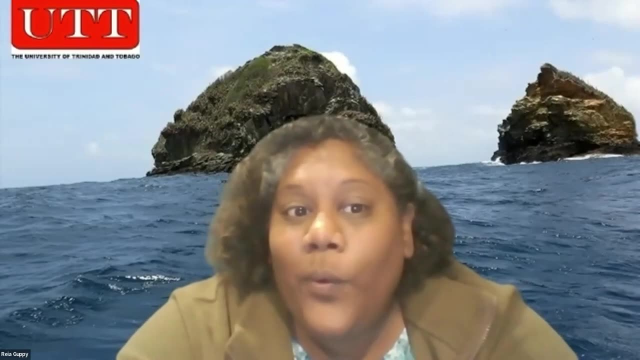 thousand trees were planted on karikou. they can actually make that island carbon neutral, and we ran out of time after that. so i've got the names of persons that can be contacted. uh, for, if any, if that chapter has that um interest in contacting them, and that's it for me, okay. 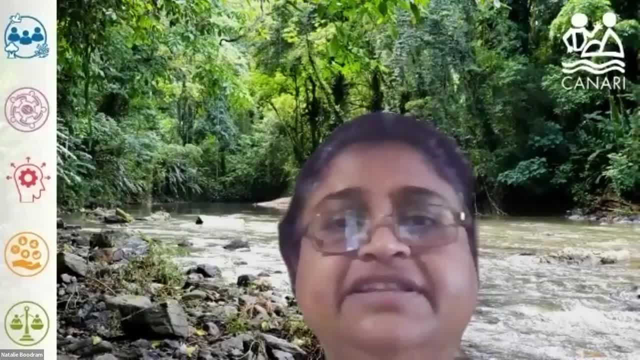 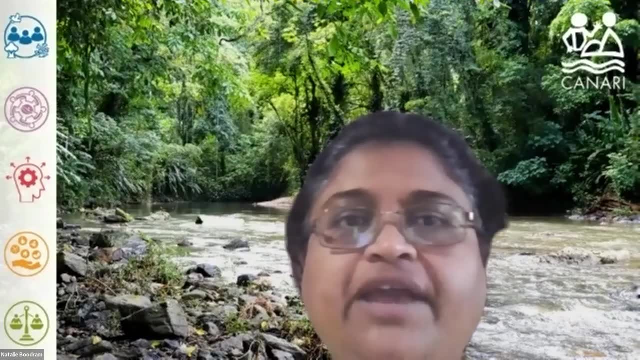 that's some very good info. um the sea urchin thing, the. um the carbon neutral endeavor. um possibly for karikou. that's cool, great, all right. so, guys, um, we are running about 10 minutes behind um, we are running about 10 minutes behind. um, we are running about 10 minutes. 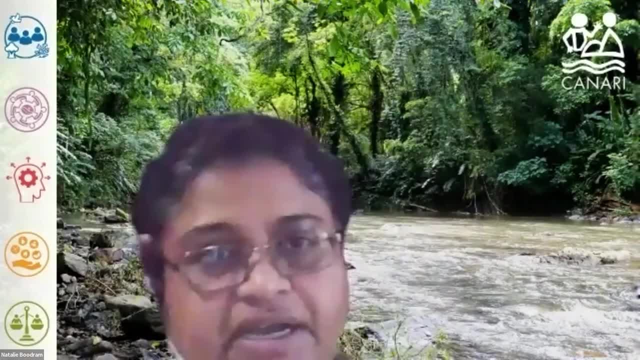 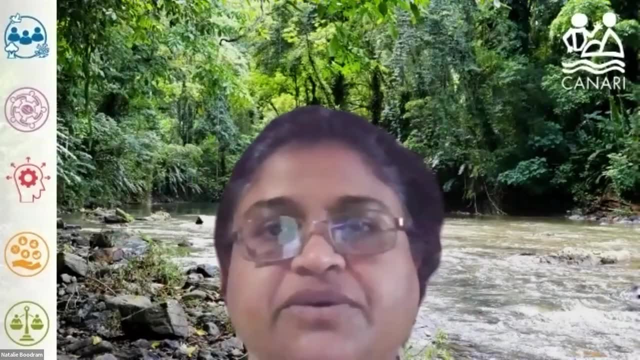 um, so we might run a 10 minutes overall, um over, uh, but i think we do need a break. i think this was a little heavy, um, so i would ask us to go to break now, take a five minutes, go get some coffee etc. and then, when we come back, uh, the evaluation chapter folks will. 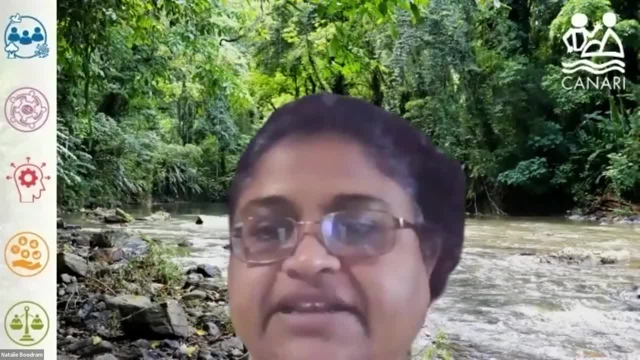 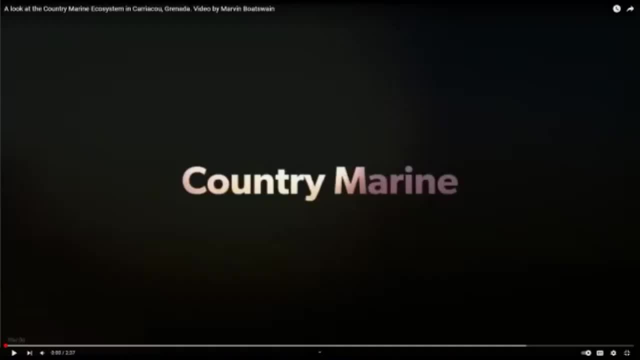 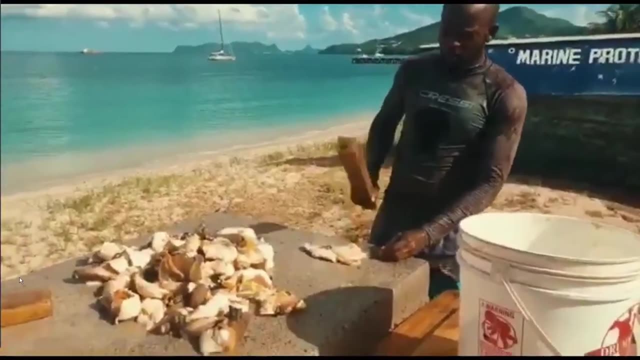 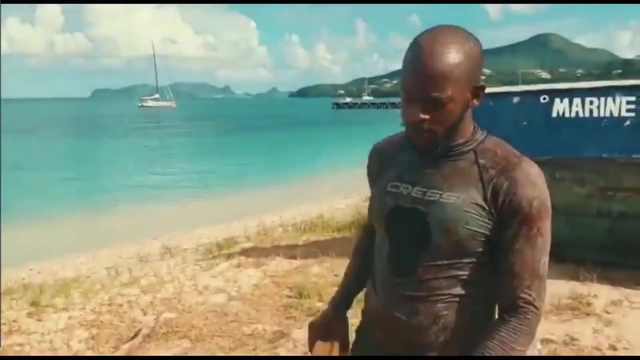 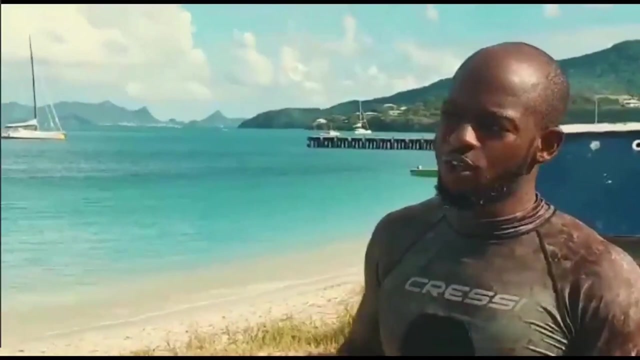 present. yeah, okay, so thanks and see you guys in five minutes. how do you depend on your country ecosystem? well, for me, i really depend on the marine ecosystem in my country because i'm a fisherman and the resources that they, that the marine ecosystem provide, provide me with a livelihood- and not just me, but it provides myself and people on the island. 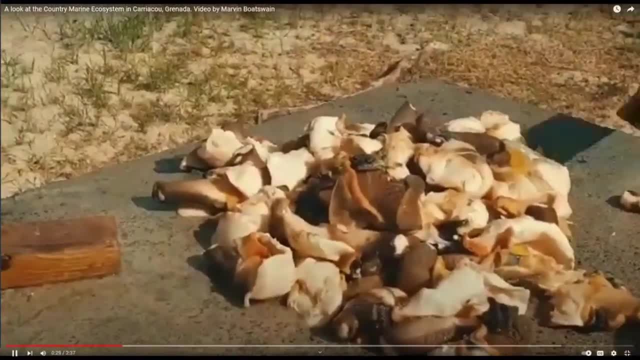 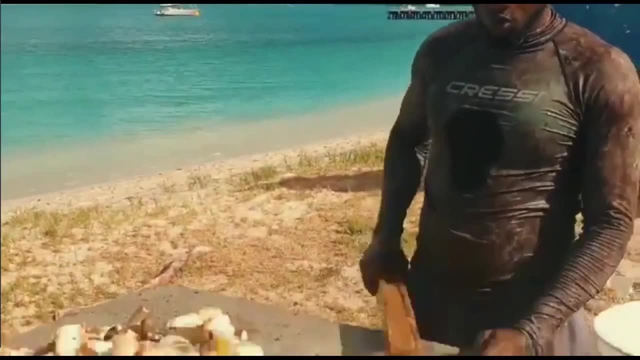 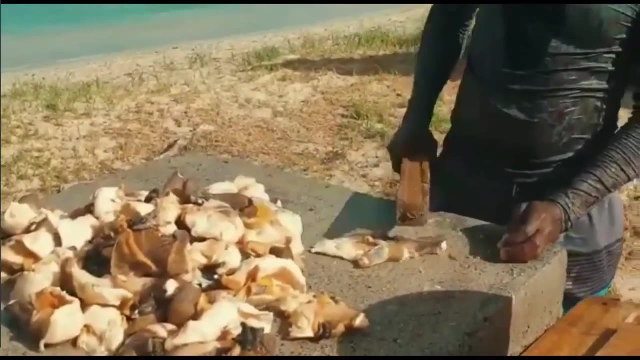 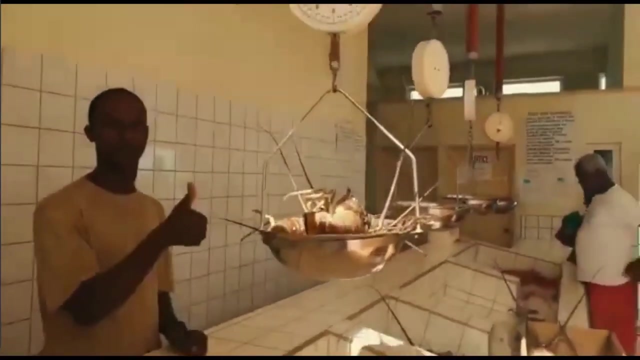 with. you know food security. i could comfortably say that my diet is made up of 75 percent of fish and other marine products. you know. so the ecosystem, the marine ecosystem in particular, for me in our country is paramount to my livelihood, my development and my survival. in the past we would have had more pristine. 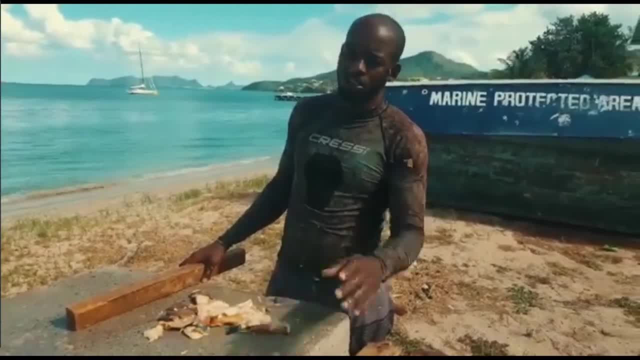 marine ecosystems in and around our waters in veneda, caribou miles, is powering my livelihood, my development and my survival. in the past we would have had more pristine marine ecosystems in and around our waters in veneda, character contributing over the years. you call the my. 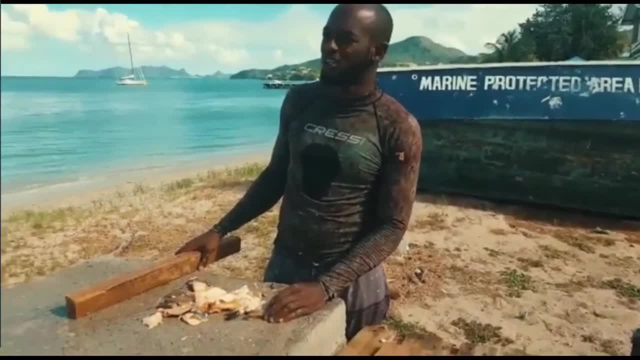 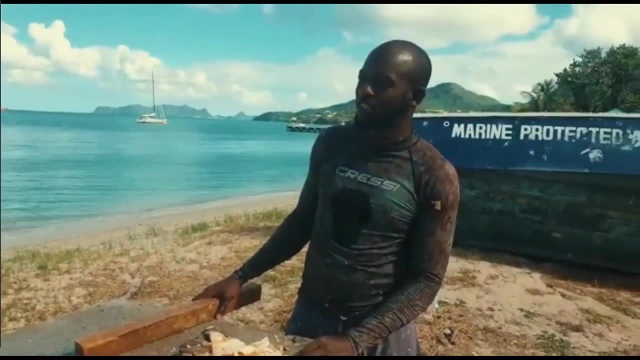 men玦, view the dignity you know To applause ring with the against五, we would have seen a lot of degradation in all of the, in all of the marine and coastal habitats, from our mangroves or seagrass beds even to our coral reefs. 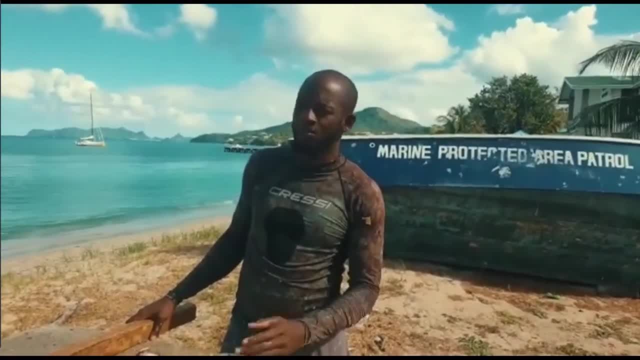 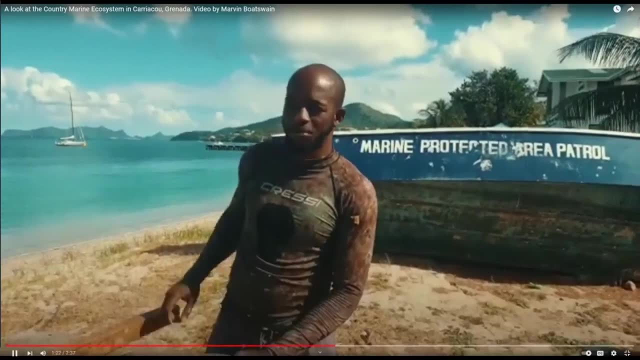 Mangroves would have been more or less damaged, as we have a fair amount of coastal development happening, as we're in the tropics, and tourism is one of our main products. Then our seagrass beds- same thing. we have a lot of yachts, a lot of. 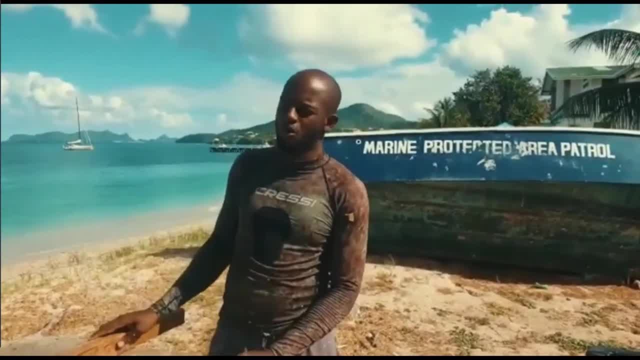 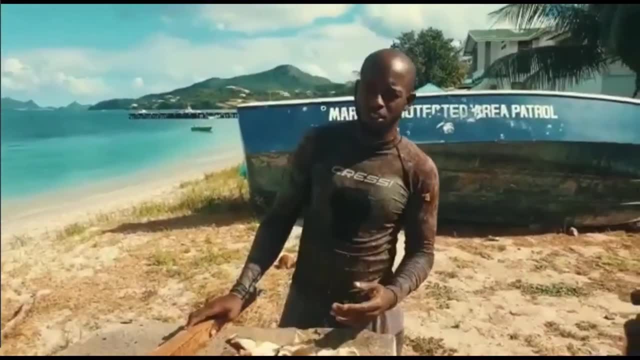 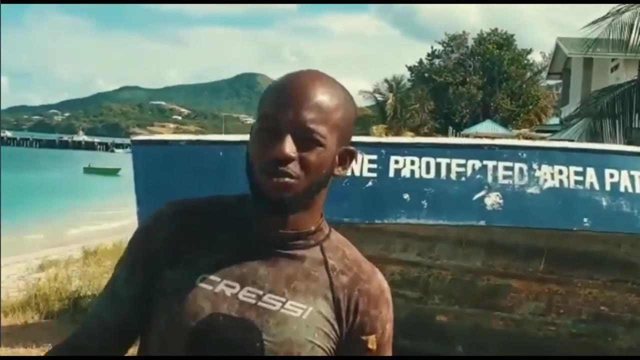 boats anchoring the damage to the seagrass and also on the coral reef. and then our coral reefs have been plagued from since the 70s with not just disease and the emergence of disease with global climate change, but also from physical destruction, not just from the yachts but from one event in particular, the storm surge Lenny. and then 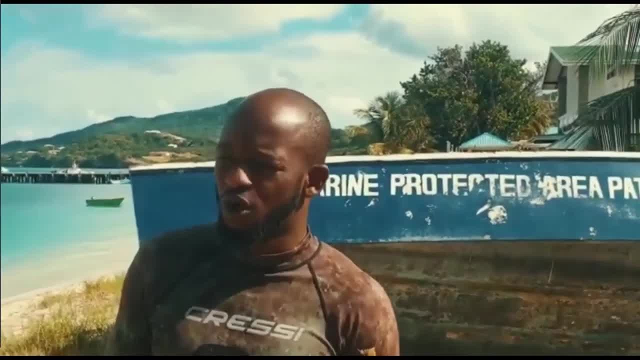 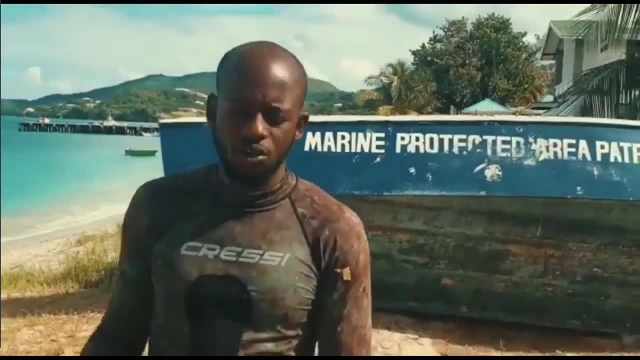 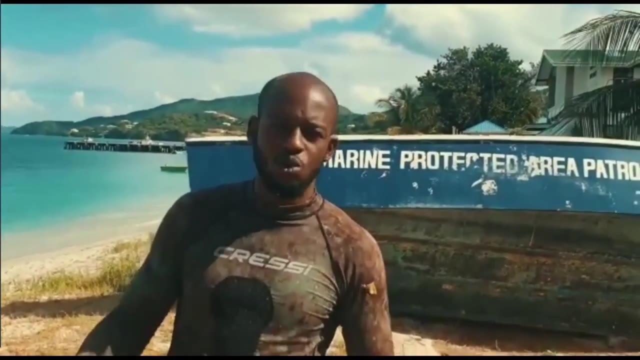 we have other stormy conditions or stormy weather events, such as anguilla, In the future. you know, I really hope that we could see some positive growth and progress where we could be able to restore as much of our coral reefs as possible, you know. 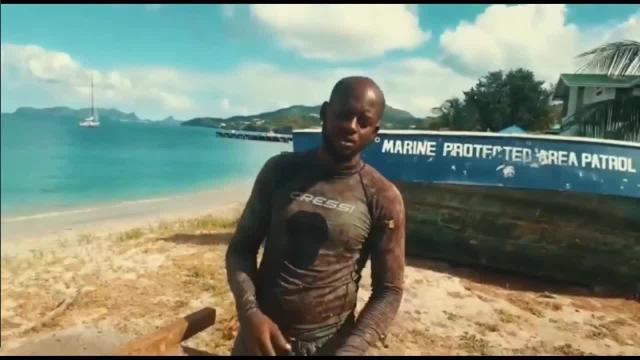 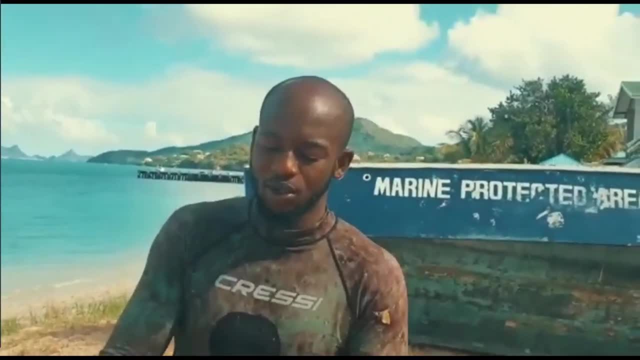 because mangroves, seagrass and coral reef ecosystems. they work in conjunction with each other. for most of the species of fish and other marine life that exist in them, for example your lobsters and your snappers, they hatch in the mangroves and 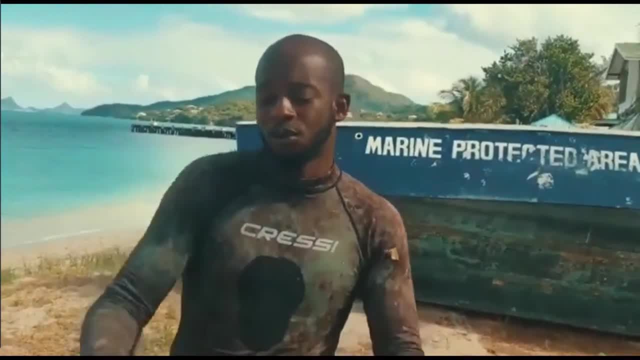 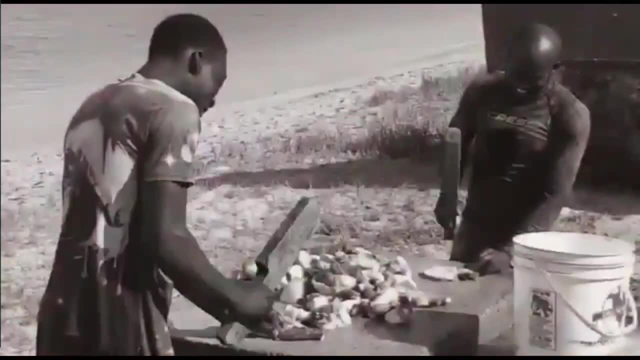 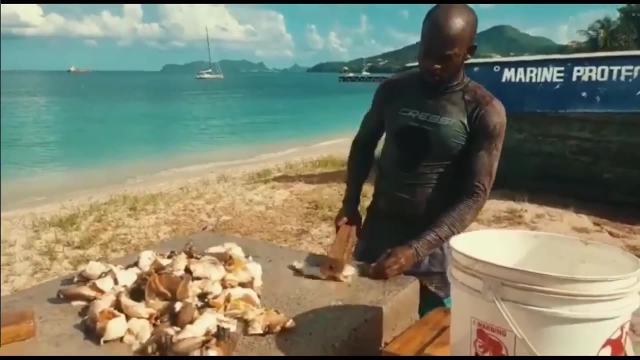 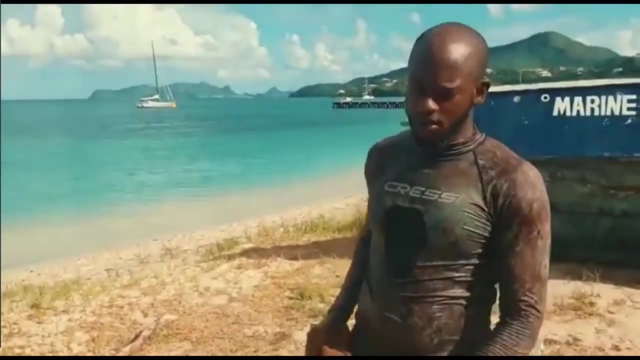 they grow into a super adult and the transition from the mangroves and the moose cook them. How do you depend on the countries eco-system? Well, for me, I mainly depend on the marine ecosystem in my country, because I'm a fisherman, and the resources thatüzh склад the marine ecosystem. 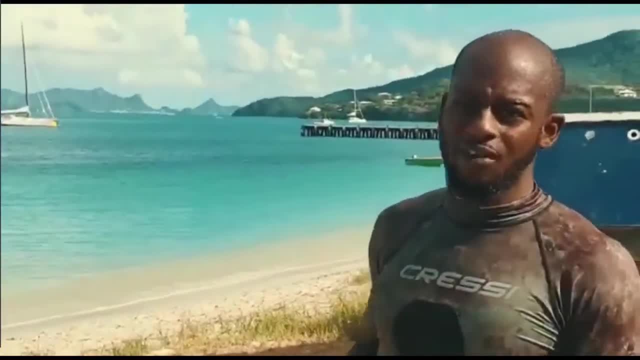 in my country because I'am a fisherman and the resources that usable the marine ecosystem has. with just theogeo, people are spending your savings that you could be interested in and making it more responsible. provide, provide me with a livelihood, and not just me, but it provides myself and 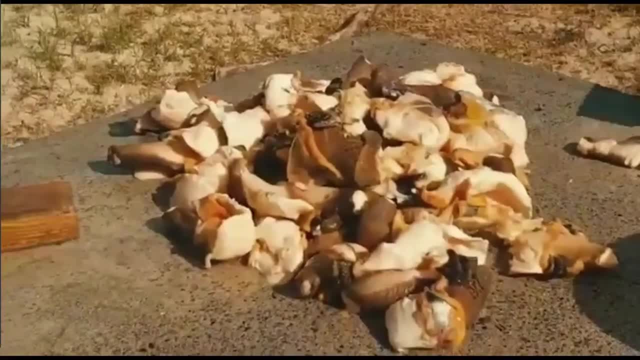 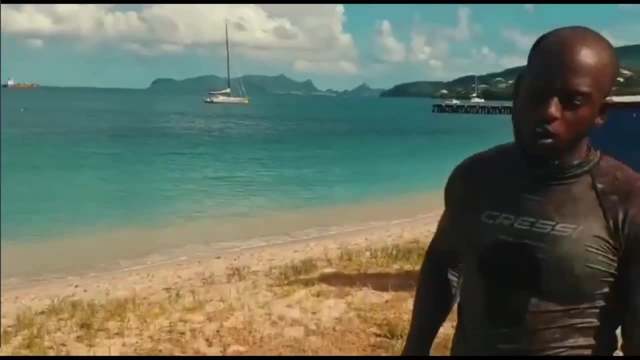 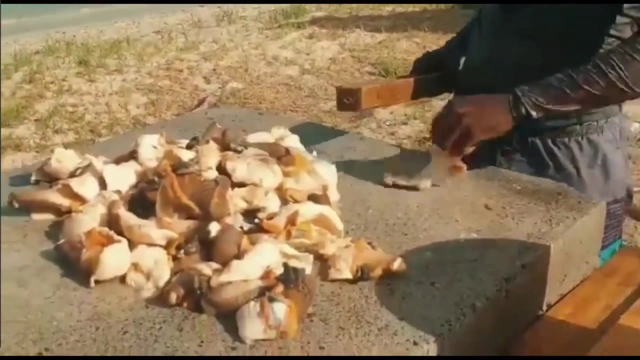 people on the island with you know food security. I could comfortably say that my diet is made up of 75% of fish and other marine products. you know. so the ecosystem, the marine ecosystem in particular, for me in our country is paramount to my livelihood, my development and my survival. 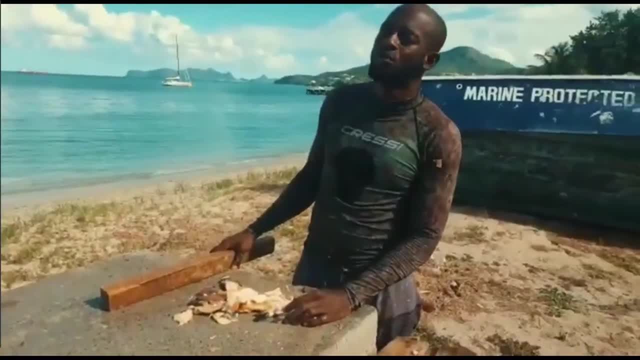 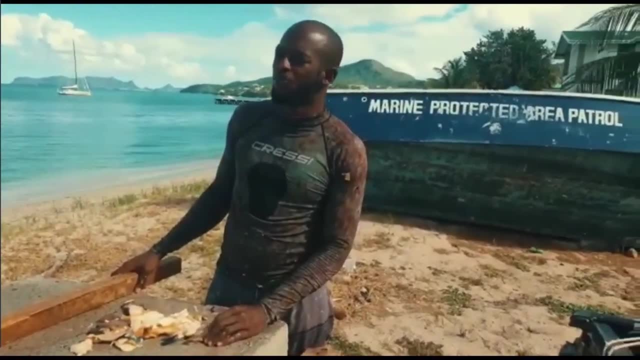 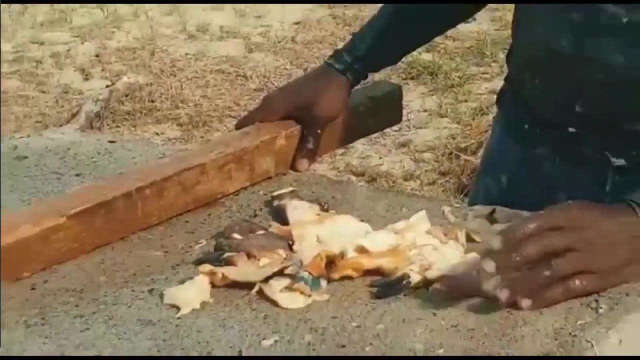 In the past we would have had more pristine marine ecosystems in and around our waters in Grenada, Carriacua and Petit-Marnec. Over the years, we would have seen a lot of degradation in all of the marine and coastal habitats, from our mangroves, our seagrass beds, even to our coral reefs. 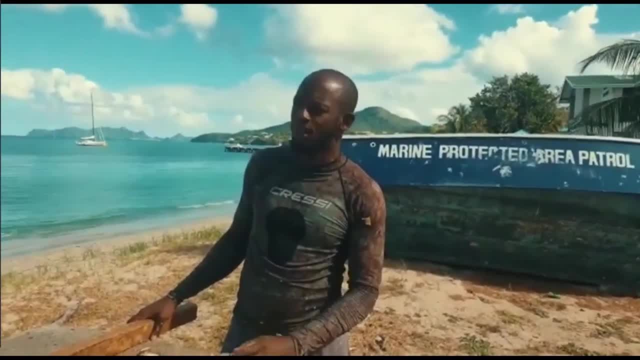 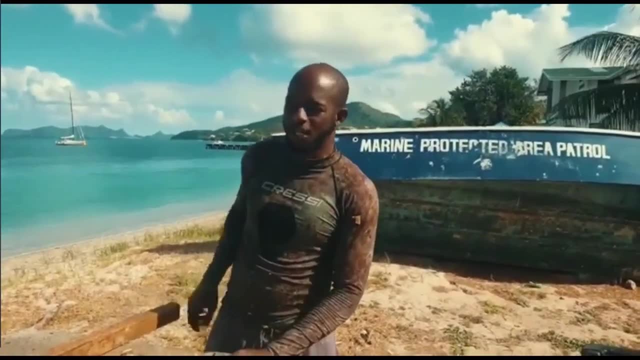 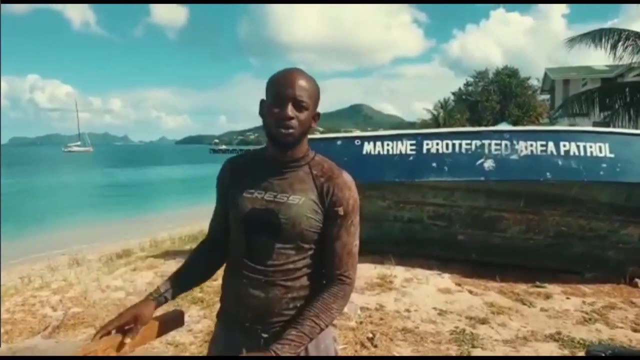 The mangroves would have been more or less damaged, as we have a fair amount of coastal development happening as we're growing, So in the tropics, and tourism is one of our main products. Then our seagrass beds: same thing. We have a lot of yachts, a lot of boats anchoring the damage to the seagrass and also on the coral reef. 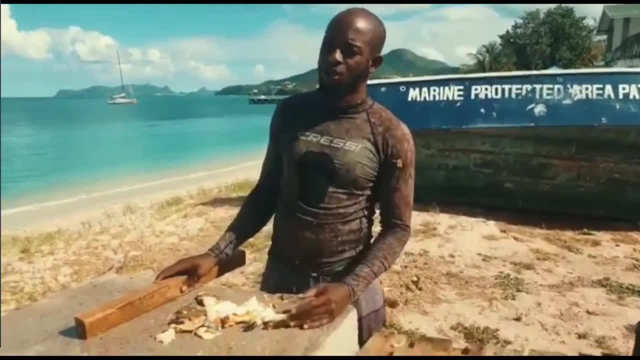 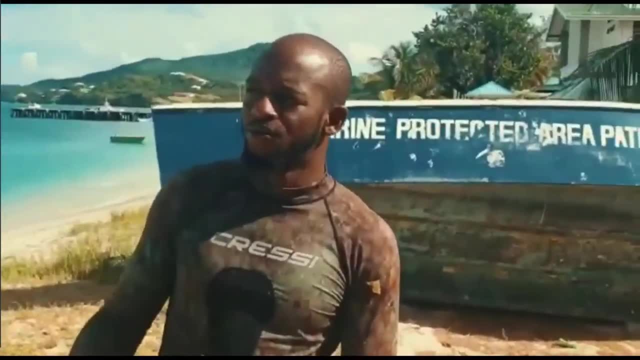 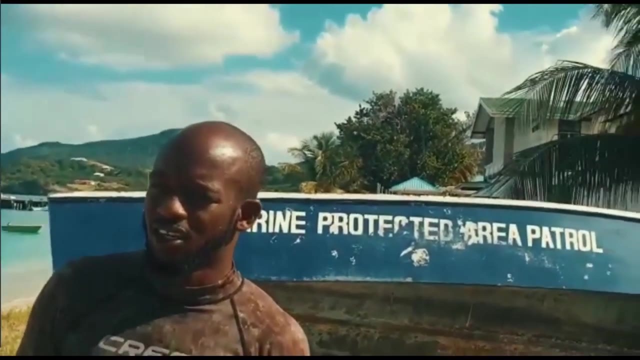 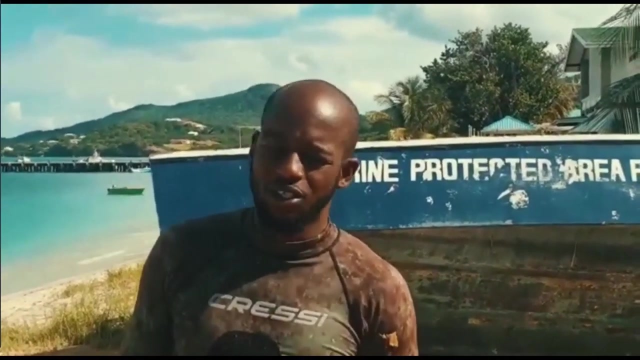 And then our coral reefs have been plagued from since the 70s, with not just disease and the emergence of disease with global climate change, but also from physical destruction, not just from the yachts, but from one event in particular, The storm surge Lenny. and then we have other stormy conditions or stormy weather events, such as ice and anemone, that would have severely impacted our reefs. 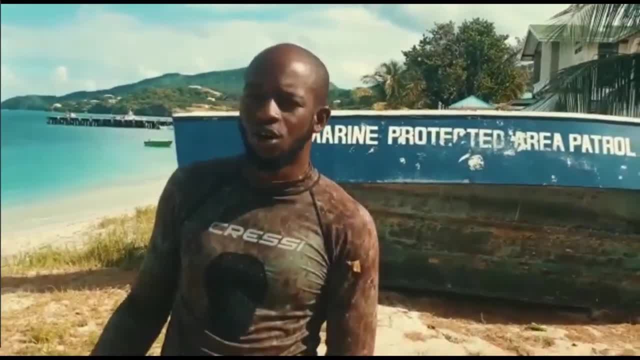 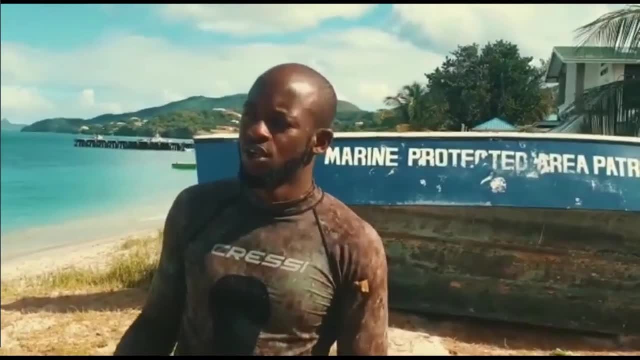 In the future. you know, I really hope that we could see some positive growth and progress where we could be able to restore as much of our coral reefs as possible. You know, because mangroves, seagrass and coral reef ecosystems- they work in conjunction with each other. 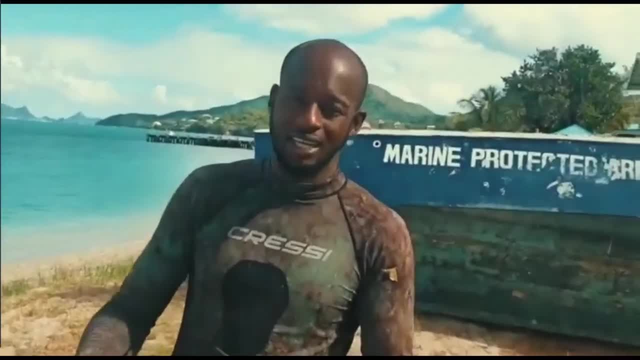 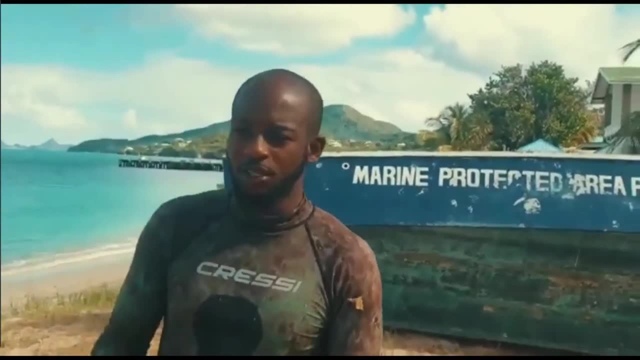 For most of the species of fish and other marine life that exist in them, for example your lobsters and snappers. they hatch in the mangroves And, as they develop into sub-adults, they transition from the mangroves and they move. 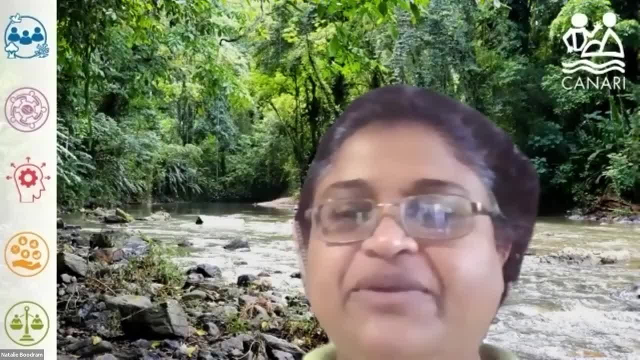 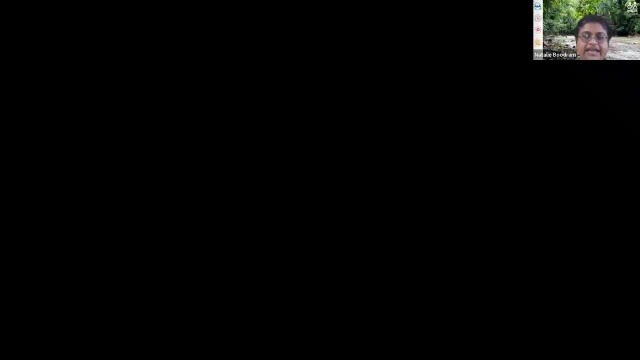 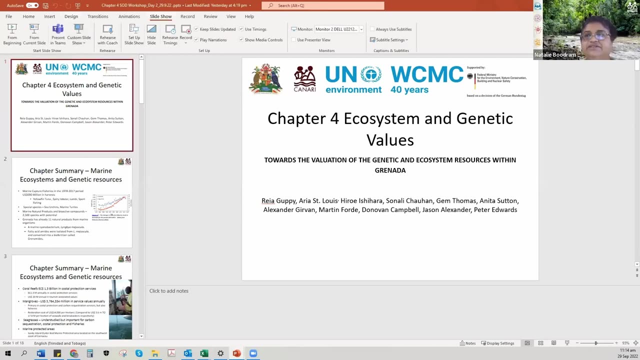 Welcome back And we are going to start right away with the presentation from the evaluation chapter. I believe Aria and Alex are facilitating. Hang on a minute. Let me just do a quick bio of them. I won't bother to share my screen. 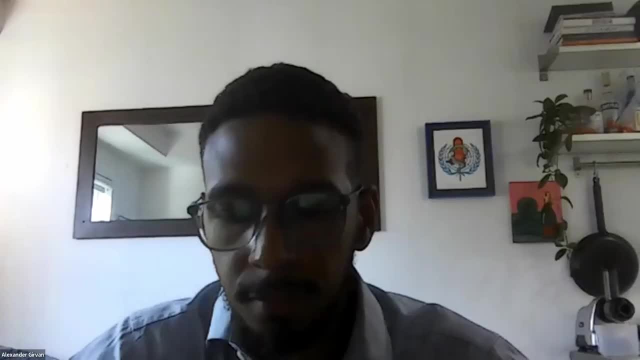 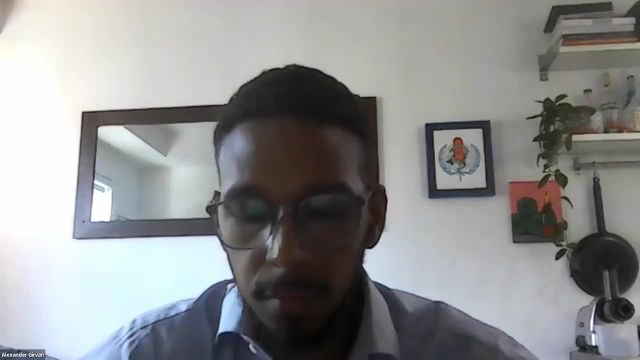 But just to say Aria, of course, who is no stranger to us. she's actually one of our co-chairs as well, And she's the head of the Environment Division within the Government of Grenada. Aria has a key interest on climate change and island biodiversity. 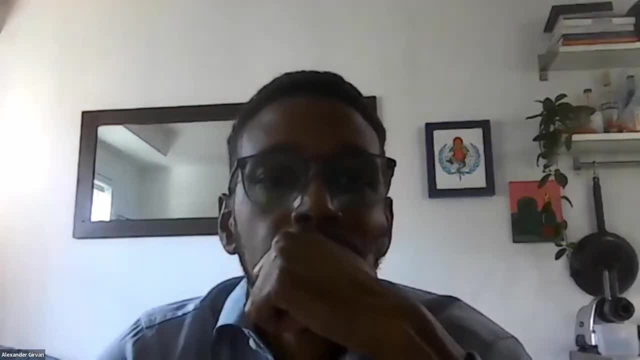 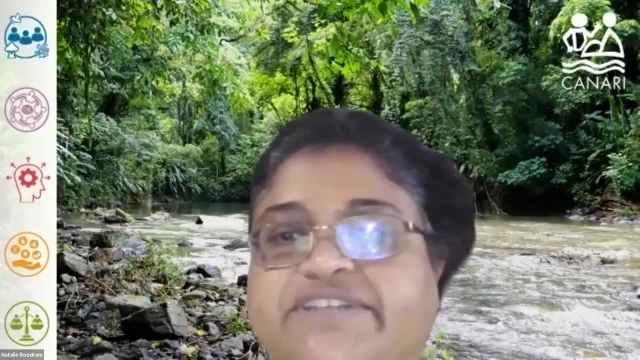 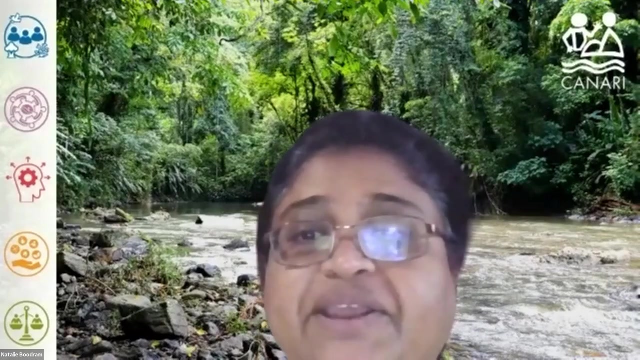 She's done a lot of work with regards to ecology and evolutionary genetics, which is why she's so keen and has played a major role in the genetics aspects. Sorry, a little tongue-tied there. She's actually worked and done research on DNA profiling, different types of molecular DNA work and using molecular markers to address conservation questions. 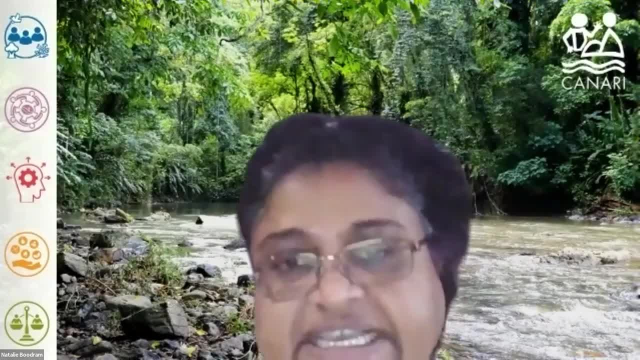 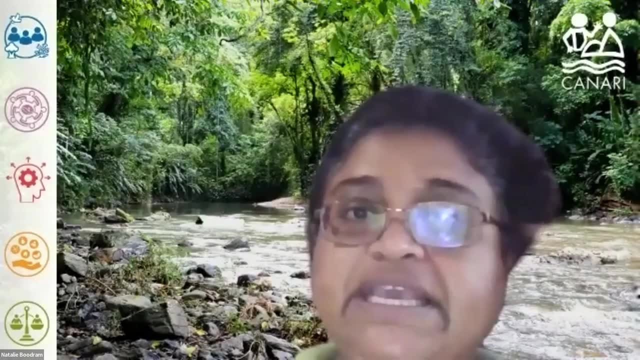 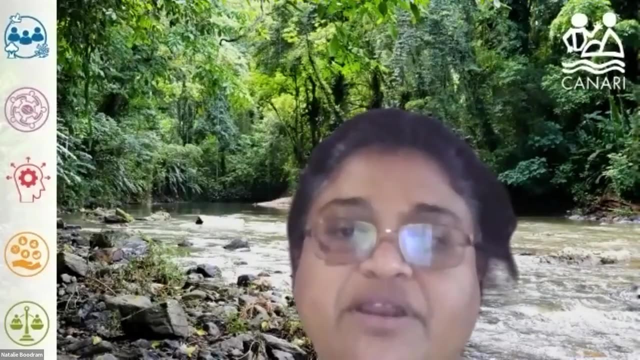 So that's Aria, one of our presenters today and one of the coordinating lead authors for that chapter. Rhea Guppy is another one who is here, but she is not presenting today, And the other presenter is Alexander Gervan, who is an environmental economist and environmental scientist. And he's had a lot of experience doing novel economic work in an attempt to address environmental problems, including in both the NGO, academic and diplomatic areas, And he, for instance, has worked with the UNEP on a project with the US Department of Energy. 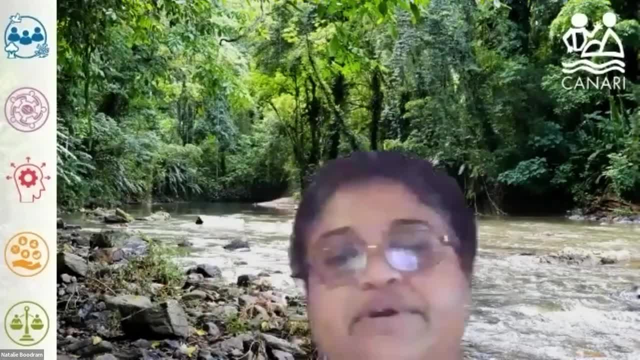 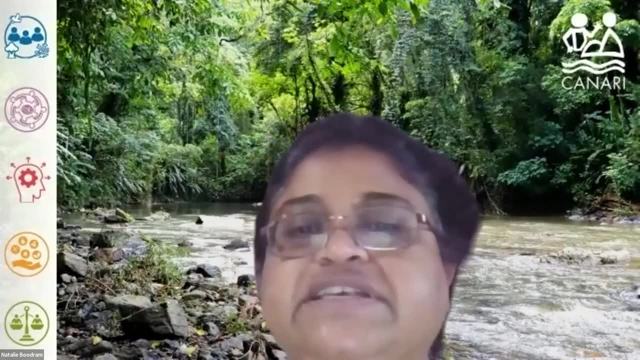 And he's also been involved in a number of other projects. And he's also been involved in a number of other projects. We agree with the UNEP Geoff Project. I think that was the one here in Trinidad which looked at the economic value of ecosystem services, looking at things like flood prevention and pollution. 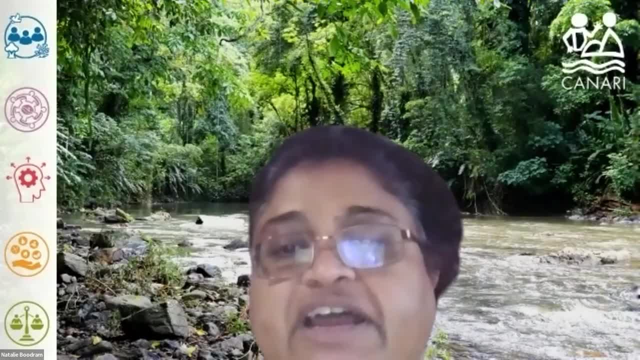 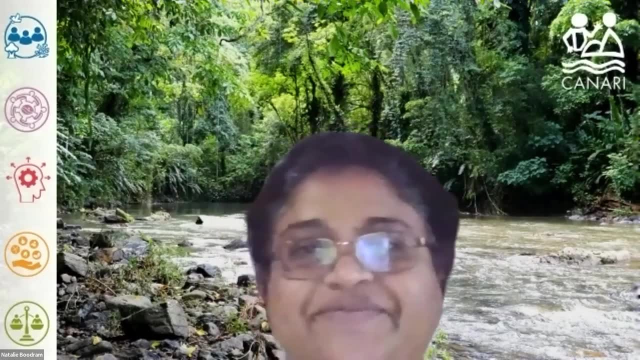 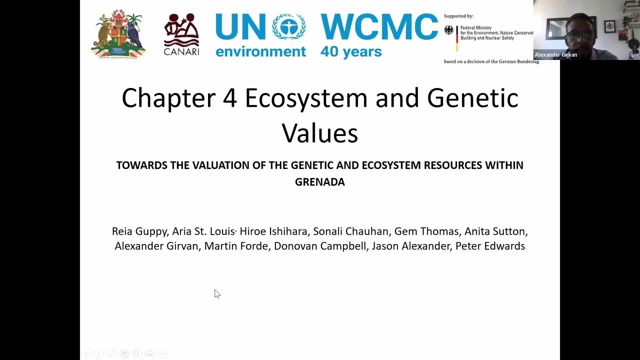 And he's also developed and taught a course on environmental studies and environmental economics at UWE. So with that I will turn over to you, Alex, to start. Thanks so much, Natalie, for that introduction. I'm just going to start by thanking my co, my CLAs, Martin, Ria Aria, but also the lead, 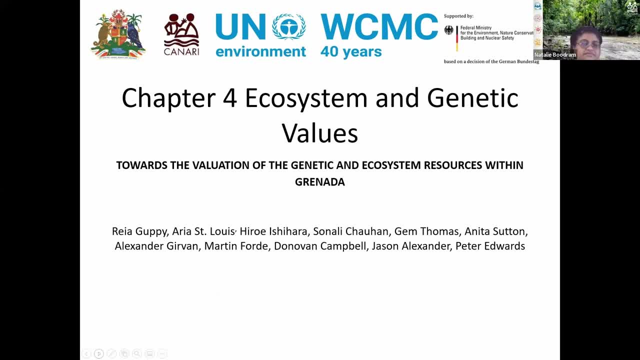 authors on this chapter, who really put a lot of work into it. I also just want to quickly note that we originally started as two separate chapters, but we merged in the end because of a lot of significant work done by both chapters and a recognition that the genetic resources of Grenada, while not all commercially utilized, have a lot. 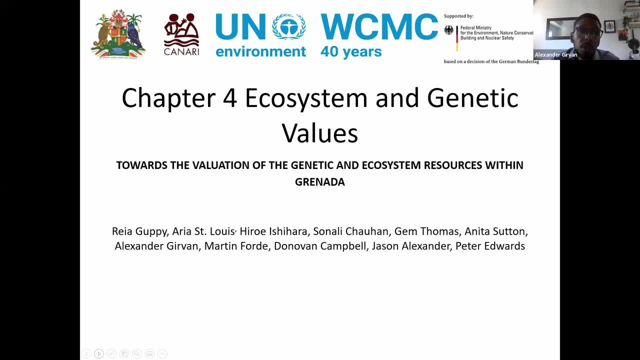 of value right now, but also potentially into the future, because of unique, unique features, unique genes, but also the potential for bioprospecting. So here you'll see all of our authors and CLAs, and I'll just move to the next slide. 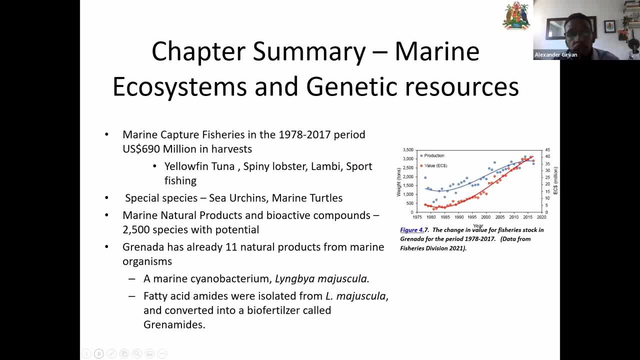 and dive right into it. We broke our section into, broke our chapter into a number of sections which look at primarily economic values, but also instrumental values on a best approach, but also relational values which describe people's relationship with the environment. 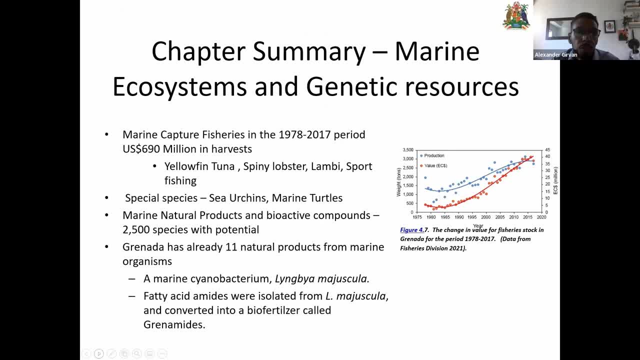 So we tried to expand it beyond a traditional economic valuation or a total economic valuation which just looks at the value of ecosystem services, and tried to expand it a bit to reach or to achieve more of a NCP or nature's contribution to people approach. 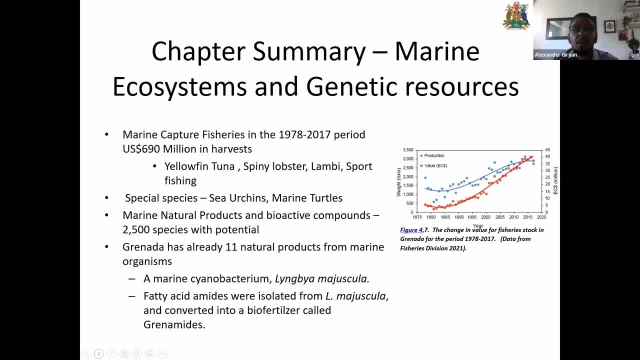 So here you'll see Mr Williams speaking a lot about dollar values, but what I think we really would like to hear from you is stories about people's relationship with nature, which people are finding right now is just as powerful or potentially more important for articulating to influence policymakers. 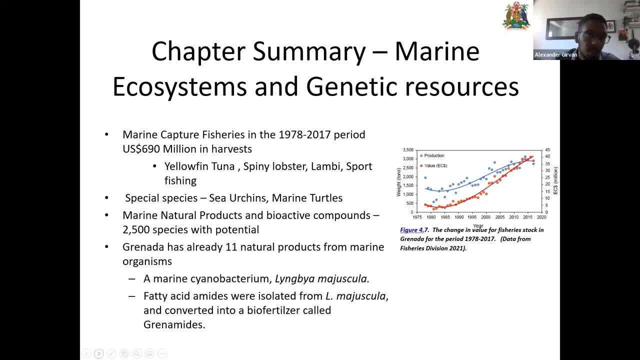 It's great to see that. you know you export X number of dollars in nutmeg every year, but when you really think about nutmeg being essential to Grenada identity, the value may potentially change a little bit. So I'm just going to dive right into marine ecosystems and genetic resources. 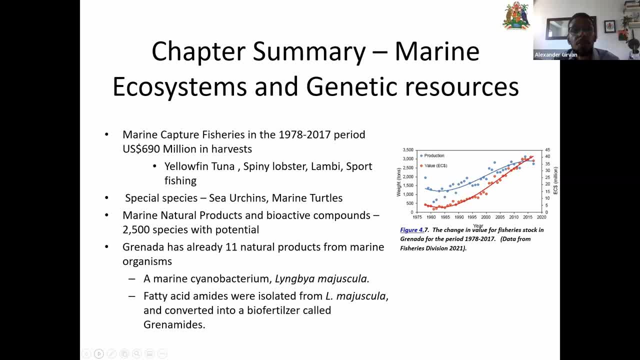 Thank you, Thank you very much for all the. we've got the pleasure to be with you. Thank you, Thank you very much. half a billion dollars US, so $690 million, in harvest from the marine space, Mostly of the commercial species I've noted here. I think there are other commercial species. 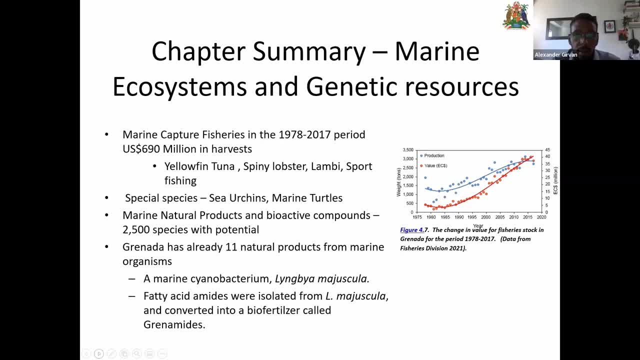 Just give me one second. I want to just pull up my notes Right. So there are about 233 species of marine fish in Grenada, so really quite an extensive genetic diversity, but also 60 species harvested from the marine environment. So these are pelagic, coastal and non-fish species. 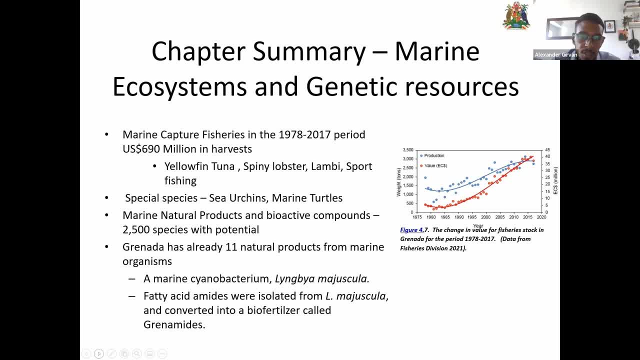 over this 40-year period that we're mentioning here. So I mentioned 233 marine fish, but there are over 2,500 marine species, with each a potential as a future natural harvest, potential for future mariculture agriculture, but also potential for future genetic resources. So 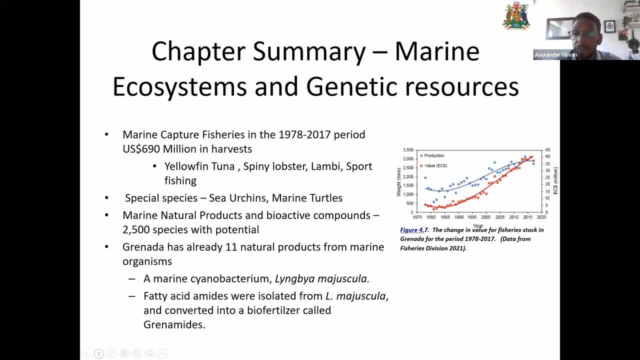 basically what we're seeing here is that fish, but also non-fish species, play a very important role in Grenada's economy but also well-being. There's some special species here that we mentioned: sea urchins, which are eaten kind of as a local delicacy, but also marine. 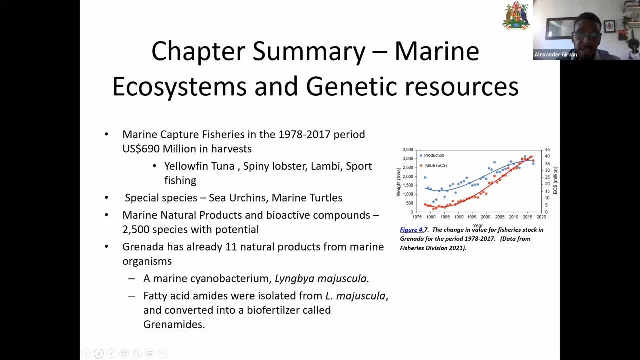 turtles, which have a very important value, not just as a landed product but also really as a support to tourism, because there are lots of tours and income on their own tours to look at marine turtles. Just want to briefly mention this image on the right, which is basically showing: 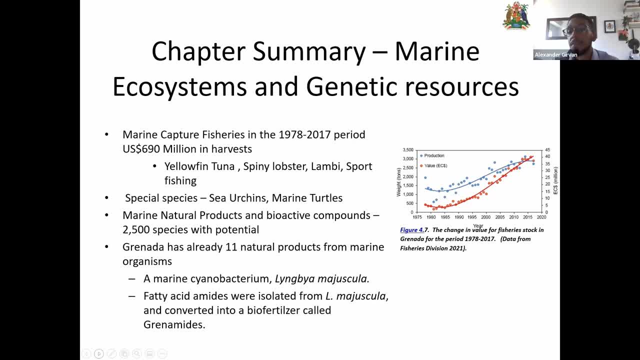 how fishery stock is. the value basically is increasing but production actually we're seeing for some fisheries, while it's increased in the past, may be potentially decreasing right now. So there is a potential or indication of some of these fish species having excessive pressure. 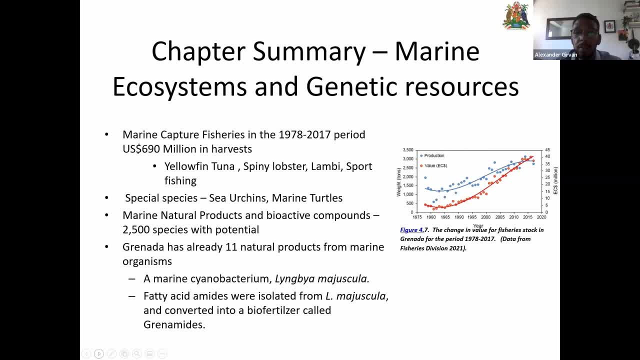 and potentially entering some sort of decline. I mentioned these 2,500 species with potential in the future. I want to already mention that Grenada has 11 natural products from marine organisms. This is not just sea mass, but these are other things that have been extracted from marine 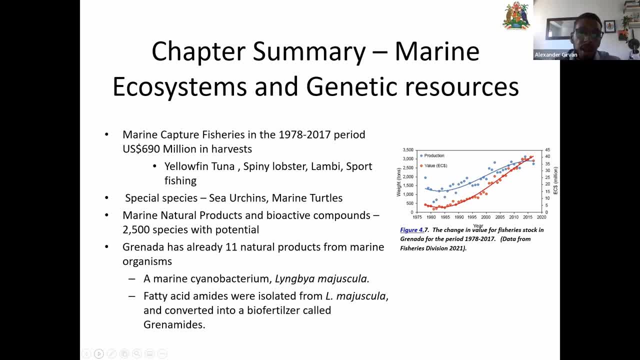 organisms, genetic research- that have been extracted from them. We have here a marine cryobacterium, and also fatty acid amideas, which were isolated from specific marine species to be used into a biofertilizer called grammadines. So these are some of the values that we're getting. 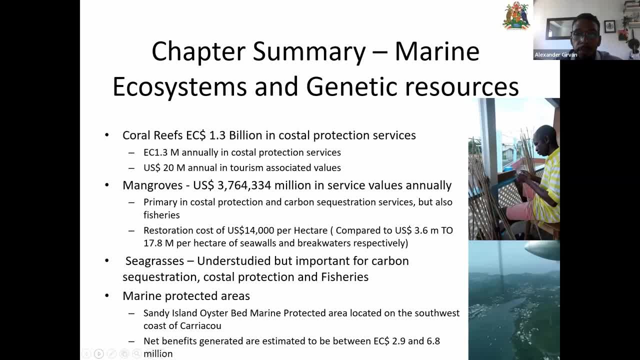 from marine resources. I just want to move to the next slide, Please. So these are some of the genetic resources, marine capture, fisheries, et cetera, and their bodies that they have right now, but also potentially into the future Marine ecosystems. 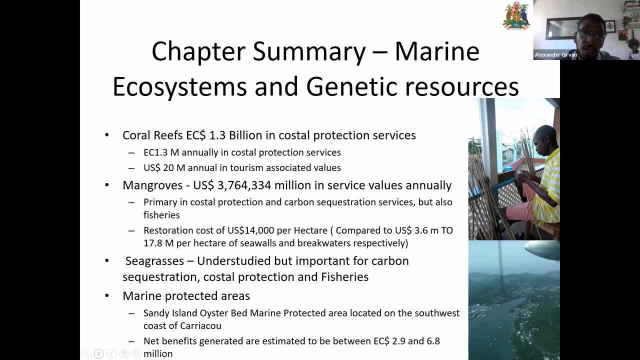 of course we've heard in the last discussion- are very important to Grenadian wellbeing, particularly when it comes to coastal protection. Now, coral reefs, mangroves and seagrass beds offer significant values in terms of coastal protection. every year We see from coral reefs an estimate of EC1.3 million. So that's an estimated estimate, And when you look at the total sea works, we see that it's around 60,000, which is about 15,000, and so we have about 20,000, so we're. 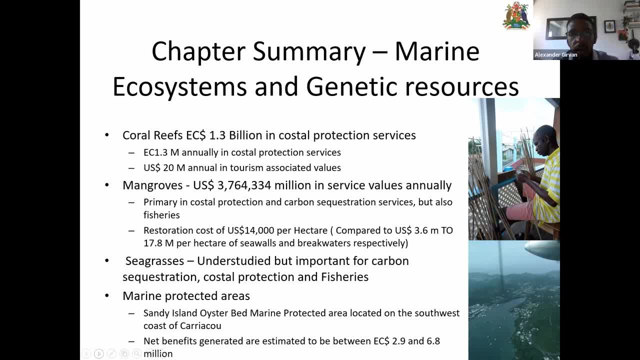 not even looking at 1 million land use, We see that there are 12 million mangroves in area, so million dollars in cost of protection value every year. and typically this is using some sort of replacement cost or damage cost avoided method, which basically means that if the coral reefs 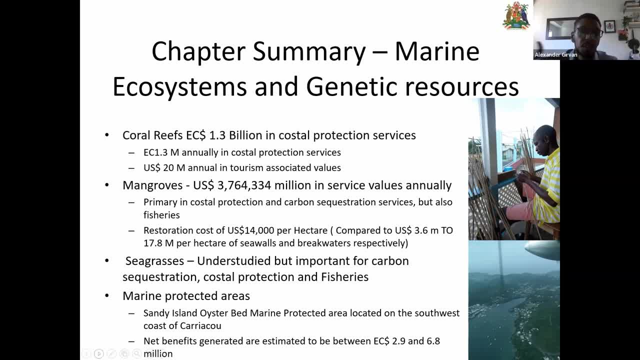 were not there, you'll be suffering 1.3 million dollars in damage every single year. Now these, these coral reefs, also generate significant tourism associated values, and what we're seeing here is, on an annual basis, about US 20 million of tourism values generated in Grenada can be. 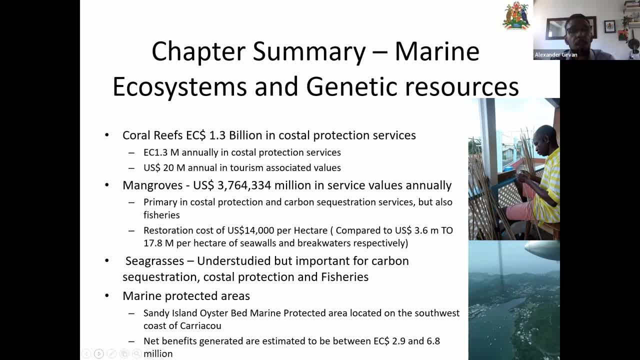 directly attributed or associated to the existence of coral reefs When it comes to mangroves, maybe not a larger number as coral reefs in terms of total value, but they were really also quite significant and they play a very important role, of course, as we mentioned earlier, in coastal 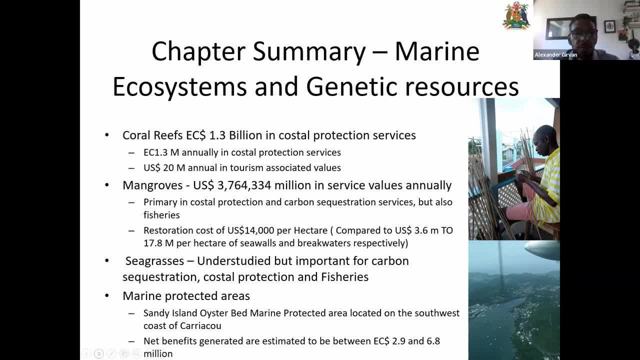 protection and carbon sequestration services, but also fisheries. and what we found is that, you know, when we look at the literature, in Grenada, the restoration cost of replacing one hectare of mangrove was US 20 million dollars. So that's a lot of money and that's a lot of money, and that's. 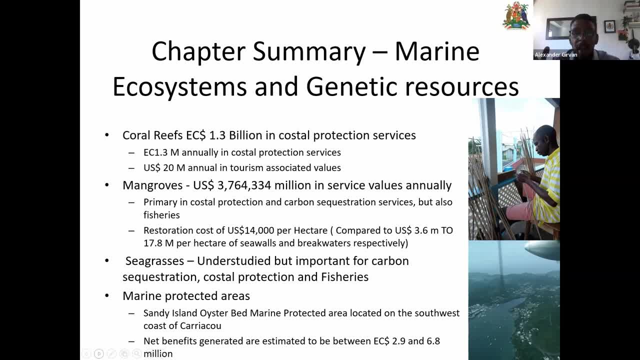 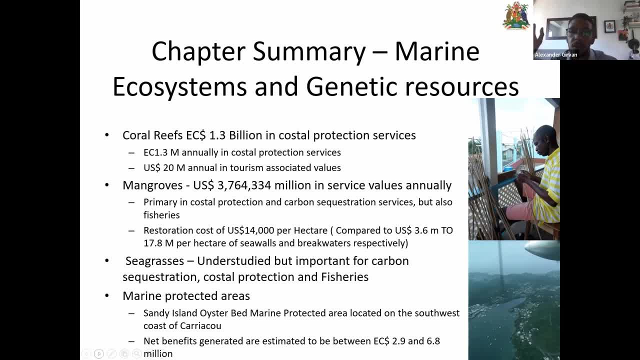 million dollars per hectare respectively, So 3.6 for a seawall and 17.8 for breakwaters. as we know, coastal construction is extremely important, So restoring a mangrove costs 14.. Replacing it with something else costs 3.6 million or 17.8 million, but also mangroves are producing, I think, in excess. 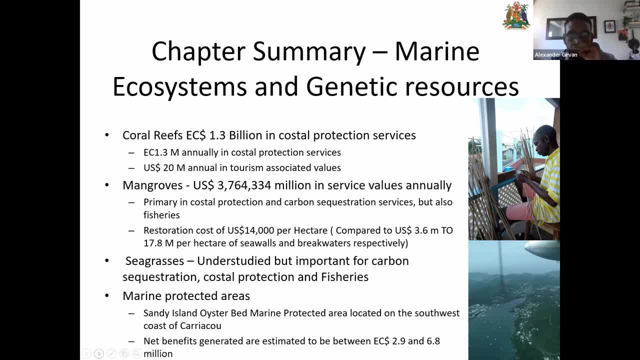 Let me just check my notes in them, because I'm not using the same site. I have to just check my notes in my PowerPoint. But mangroves are worth on average about 20,000 dollars plus per year in terms of service values. So what we're seeing is that if you restored it for 14,000, you're still. 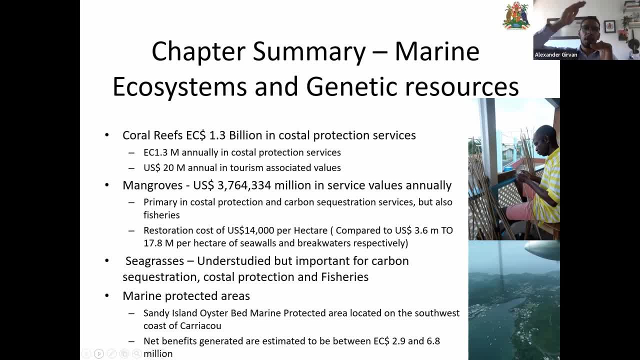 getting 8,000 dollars in terms of additional value provided by those mangroves for the restoration cost. but also, separate and apart, the restoration cost for a mangrove is significantly less. It's only a few thousand compared to millions for seawalls. So mangroves are really important in this coastal protection space and this really looked. 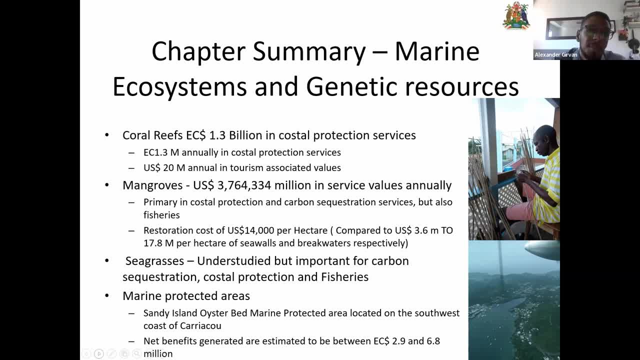 at coastal protection of assets, but this is not even including the benefits provided by the hurricane hole that Nathalie mentioned earlier in terms of protecting boats and other very important marine kind of fares and assets. So if you think about the additional benefits provided by these hurricane holes and by the mangroves, etc. in terms of protecting a tuna boat, 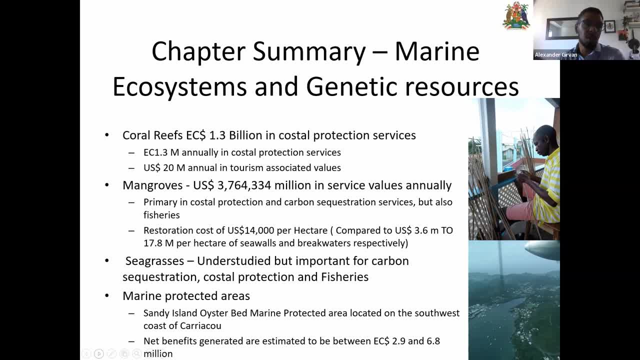 protecting a boat that's important for, let's say, coastal cruises or for some other type of tourism. the value actually is potentially very much more than this. So with seagrass beds, we found that they were understudied in Grenada, understudied globally, but very 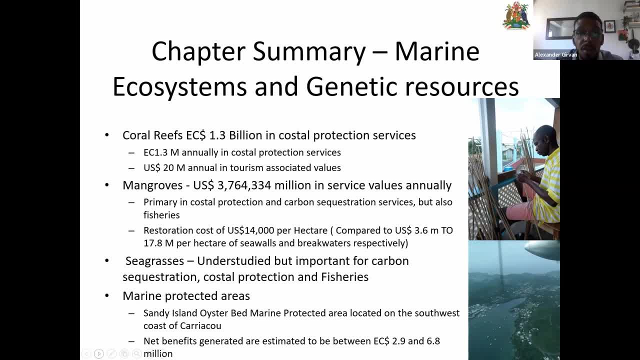 very important for caravan sequestration, coastal protection, fisheries. So, basically, what we're seeing here is this, and I think this is, you know, increasingly recognized in literature: coral reefs, mangroves and seagrasses are a trifecta that work together to provide coastal 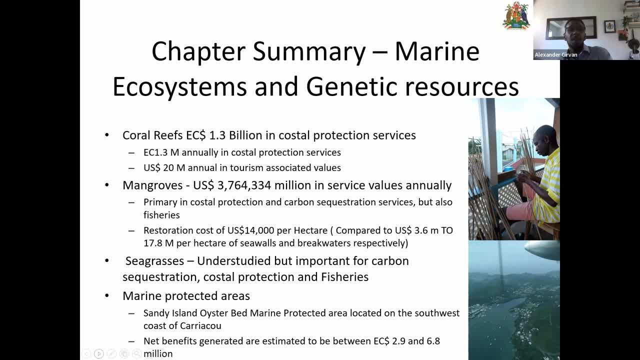 protection, fisheries, but also tourism-related services. I think coral reefs are the prettiest ones and the most charismatic, but I think what we're trying to say here is that seagrass beds are less understood, but potentially almost equally as important, but also part of a complex 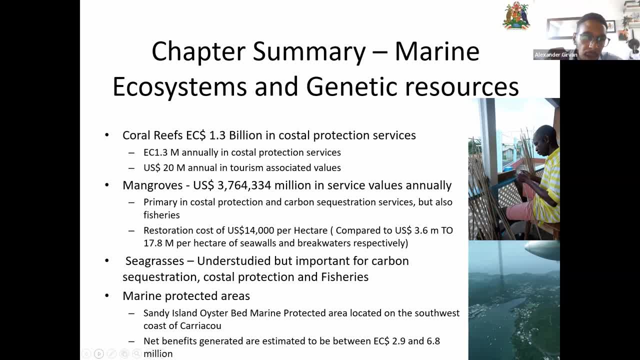 mix that has to exist as a complex mix. So we know that a lot of coral reef restoration is happening in the region. a lot of mangrove restoration is happening in the region, but there needs to be more attention paid to the seagrass beds and they're important In terms of studies on marine. protection. there's a lot of research on marine protection, but there's also a lot of research on marine protection. there's a lot of research on marine protection, so it's hard to tell what's going on, but both studies are definitely showing that there's more and more questions. 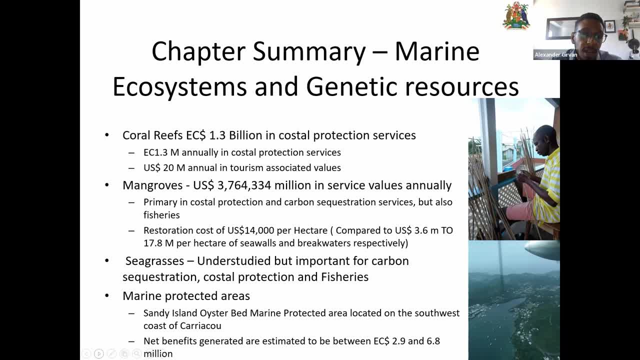 beingatured 2019.. surprisingly, even at the seagrass beds, paraeval baby, everything is in the ocean. tectonic work, I can imagine, here is it. it can be hidden, it can be cut, So we needTINe to provide. we needskin text up, but we don't want. 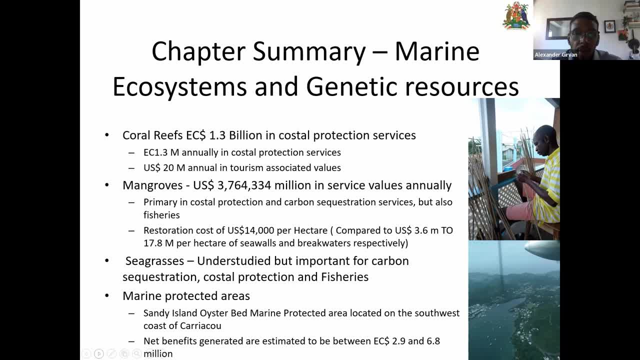 TINIO to get it to be a you know it could be a you know zoned or tIN labs to because to kill any other people. that's a golf We don't want to be. this has been going around and wirdx casa San. 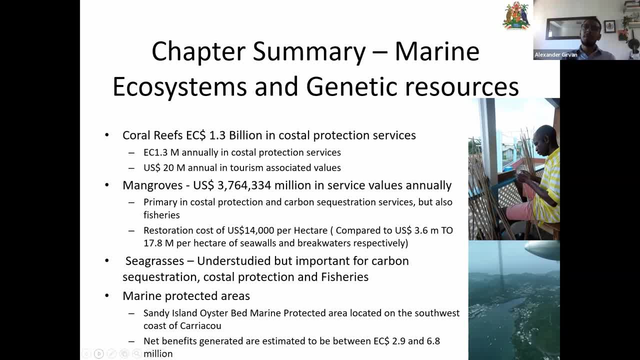 which we'reкольars who say that at the bed it's bob 노 safely downing islands, exactly because they're truthfully, we'll design for the ducks are going to be cut into pieces. money to buy a boat, to buy fuel, to buy ice, to take tourists to that area or to take scuba divers. 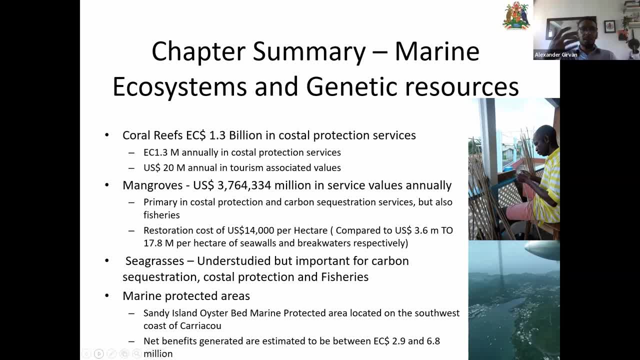 to that area When you account for all of the money they've paid or expended- sorry, the cost of getting to that area- but then you look at the income they've generated, they have generated in excess of the cost: 2.9 to 6.8 million. So that's what it means in terms of net benefits. It's 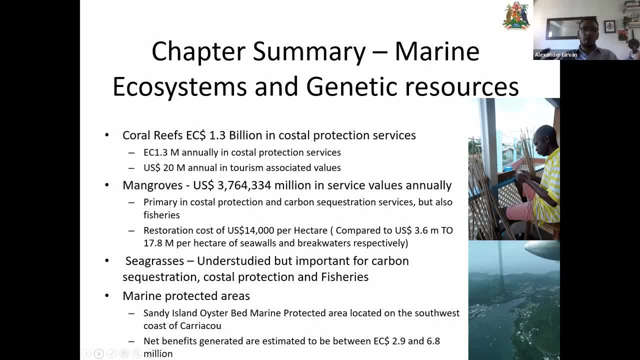 almost like a concept of- I don't want to say this- but profit generated by the marine protected areas. So what we're seeing is that they cost something, but the benefits they're producing are significantly more of these costs Somebody mentioned earlier. I heard you know there are. 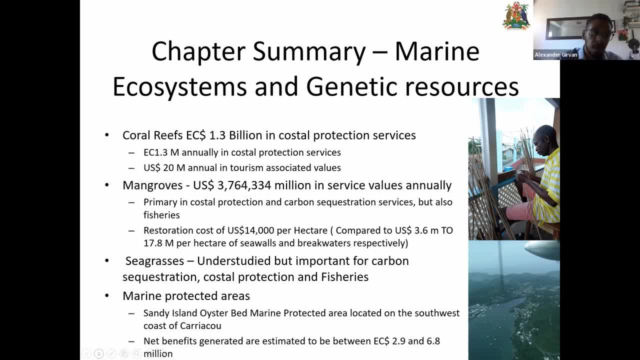 marine protected areas in Carriacou? What about the ones in Grenada? And I think, basically, what this study is indicating to us is that there needs to be a consideration of, you know, marine protected areas on mainland Grenada, particularly because these have spillover benefits for the 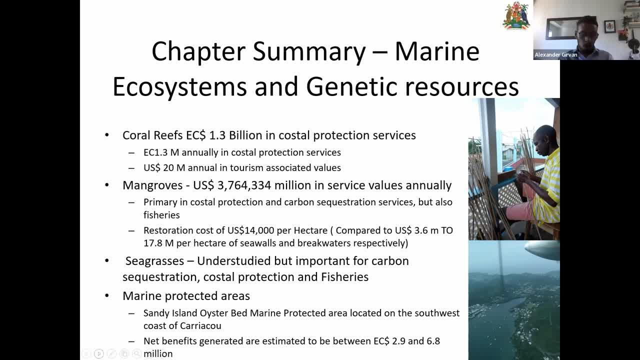 associated fisheries. They can't catch fish in a protected area, but fish can grow up, have a good juvenile life And reach to a good landing size. sorry, if you have these protected areas in operation, producing these net benefits, spillover benefits- Next slide, please. 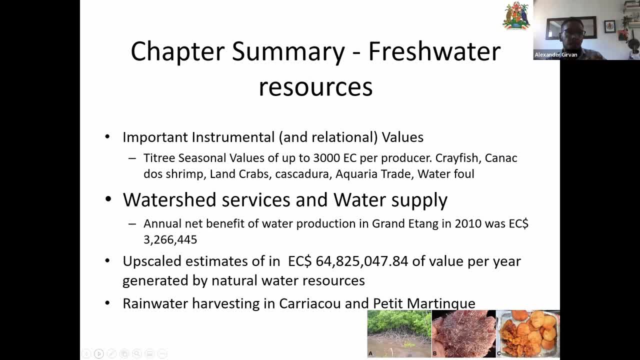 So we looked at marine, then we looked at freshwater, then we looked at terrestrial, recognizing that freshwater resources are a bit in marine but also a bit in terrestrial. They of course run through the forest and they have a watershed kind of relationship. 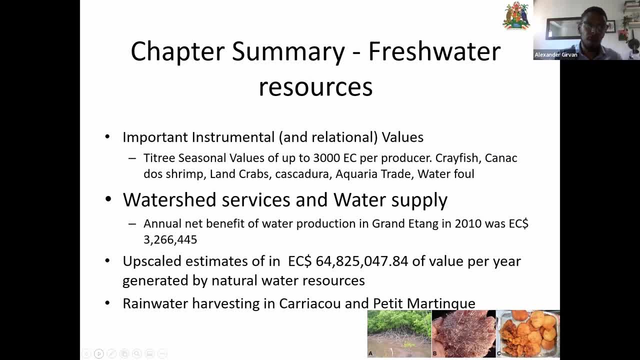 with the forest, but also when they reach the sea, they're definitely going to be able to catch fish. So we found that these were very important, these freshwater ecosystem services for instrumental but also relational values, right? So the instrumental values, of course, would be for the groups of people who are harvesting products from 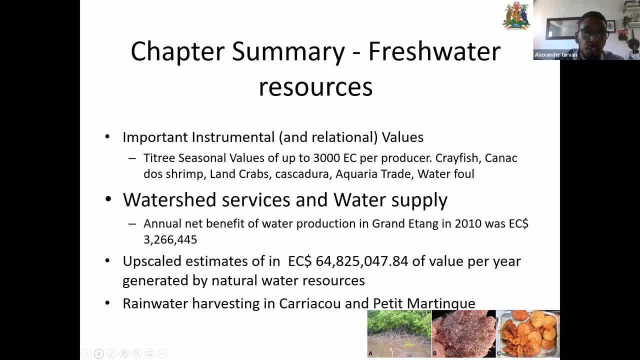 freshwater, And we found that the Thai tree seasonal fishery had values of up to 3000 EC per producer, So a good amount of income for these people. We also saw other things like crayfish, Kanakdos, shrimp, land crabs, Cascadura- some fish from freshwater ecosystems. 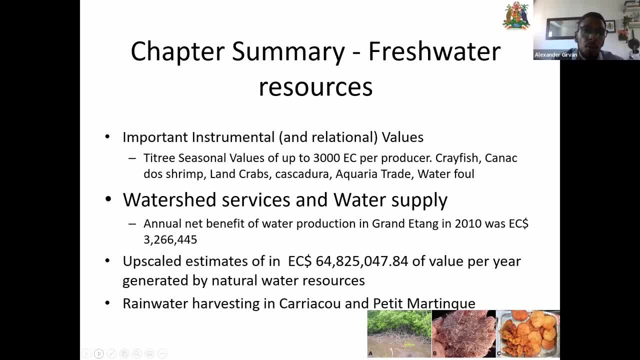 involved in the aquaria trade And, of course, waterfall, also providing some benefits in terms of bird watching, And I don't think there's any hunting of the waterfall, but I could be corrected here. So what we found for these values is, in terms of dollar value, not very important. 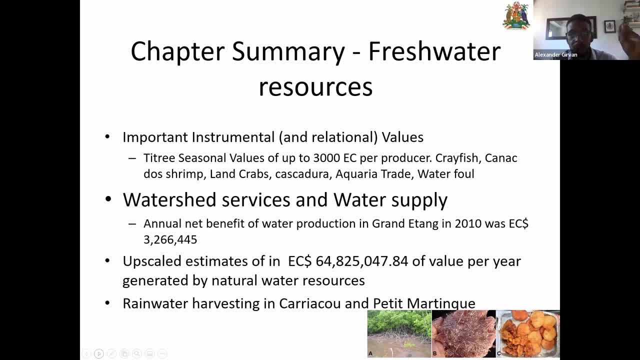 but could they be replaced? Not at all Right. So you know you could compare the cost of harvesting some Thai tree to the cost of a can of tuna, because they're both protein, but they're actually incomparable in terms of the experience. So Cascadura, crayfish, et cetera are not like the things that you can import. 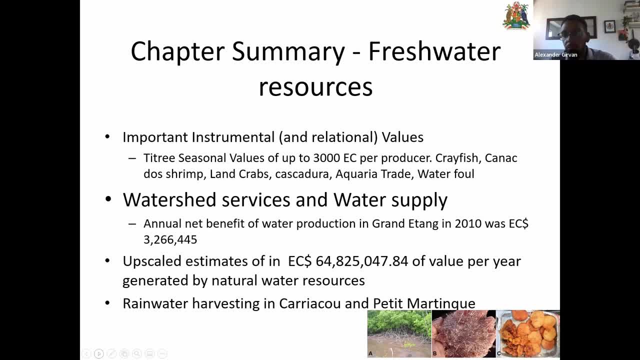 So the relational values in terms of somebody going to catch crayfish or going to catch Thai tree and giving that or transferring that habit to their children and being able to share that meal with somebody- their neighbor- is significant Right, Significantly more than any economic dollar value that we could potentially quote. 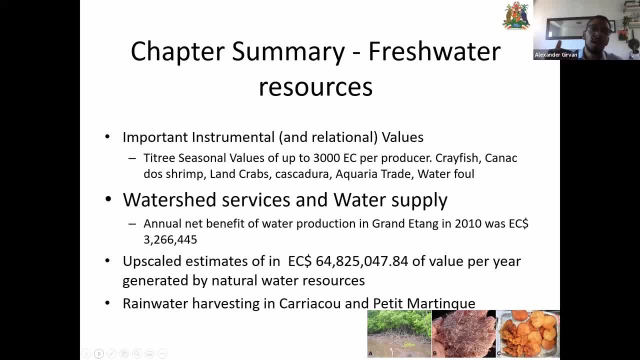 So we wanted to really highlight that here for these values very much relational As well. somebody mentioned as well religious ceremonies which happen in rivers- I think baptisms, but also not religious, but river lines. So this idea of people having relationships with 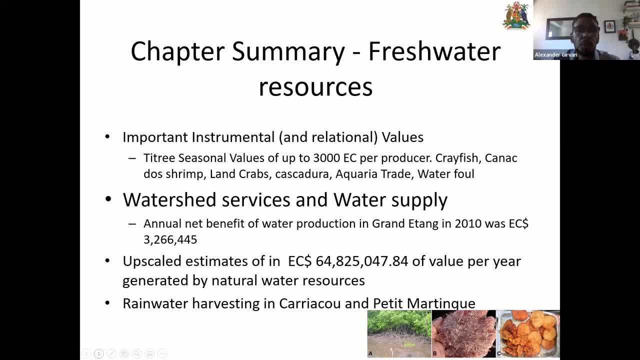 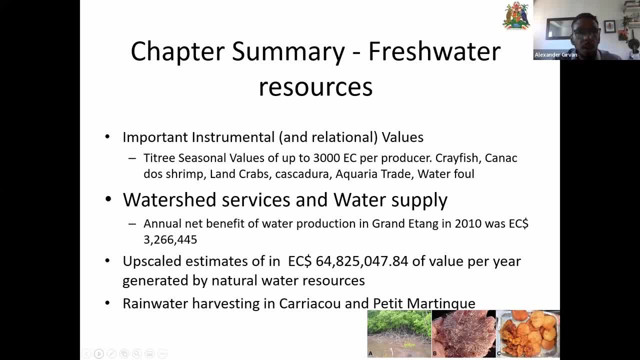 same as the go to a river line, catch some crayfish and carrying it, you know, by the river. In terms of watershed services and water supply, one study found that the net benefit of water production in Granite and Lake in 2010 was worth about EC 3.2 million. 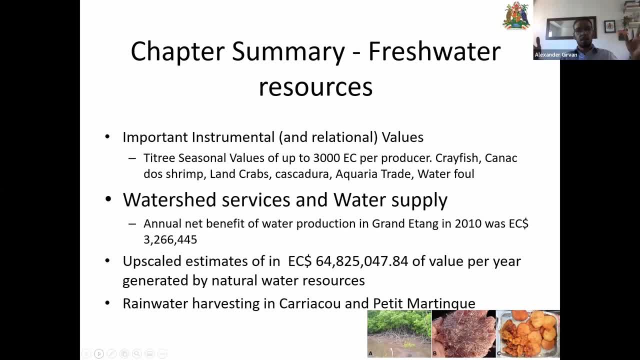 When we took these estimates and upscale them to the entire island, we found that the natural water sources, or watersheds, are producing estimates in excess of $6.4 million of value every year in terms of water provided. Again, with something like water, we can estimate the benefits being 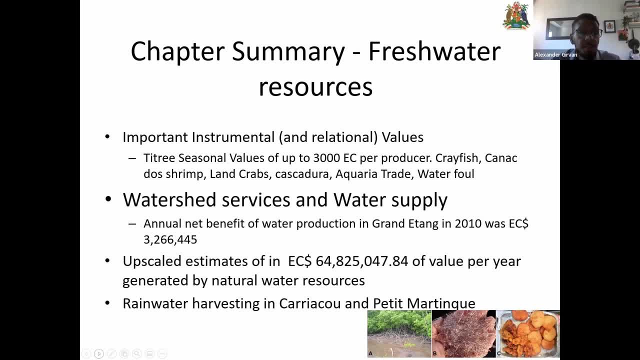 provided by nature but by and large, is the underestimate of the value being provided. You know, for our island, like Grenadier, to have to import water in times of drought is much more expensive than the cost of NAWASA to produce this water. 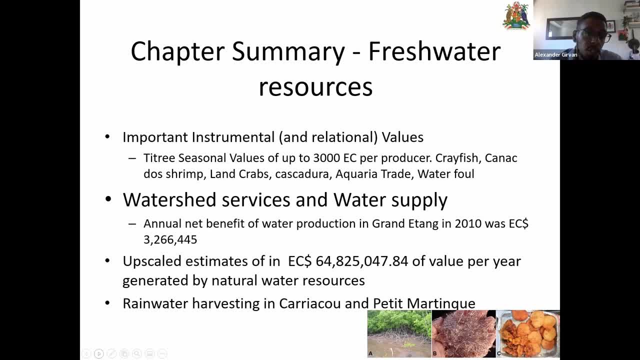 I think we heard a lot about climate change and changing water regimes earlier, so just to push home this point that, yeah, $64 million is a lot of water value being produced by forest every year, but it's actually worth much more than that when you think about replacing it by having to. 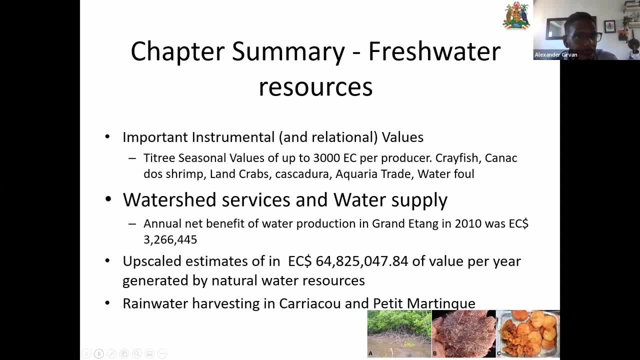 import water with a water boat from someplace like Guyana. It actually would be very expensive And of course, we have to mention that while there are some dry rivers in Karikou and Martinique, some seasonal rivers, there are also some dry rivers in Guam, Guam, Guam, Guam, Guam, Guam, Guam. 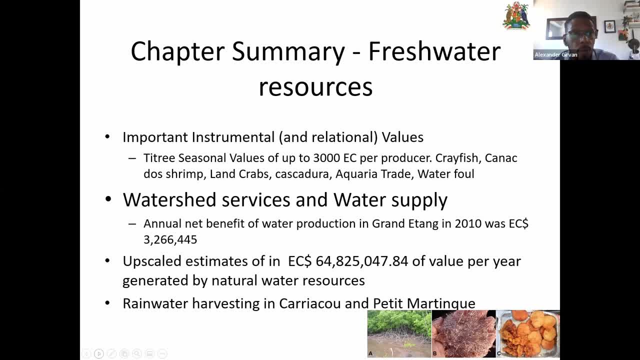 rivers. Water is, by and large, supplied by rainwater harvesting, So of course, the issues of reducing rainfall that we mentioned and climate change are kind of related to this. So I just wanted to note that mainland Grenadier and Karikou and Petit Martinique are not the same. 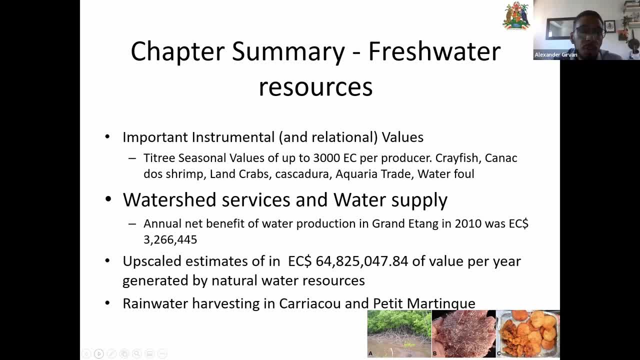 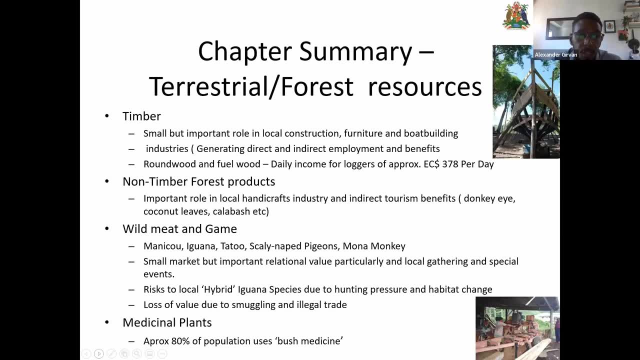 in terms of their relationship with water resources, but also water ecosystem services. Next slide, please. In terms of terrestrial and forest resources, we found that timber played a small but important role in local construction, And we have a picture here of the sawmill. So local construction furniture, but also boat building in Karikou. 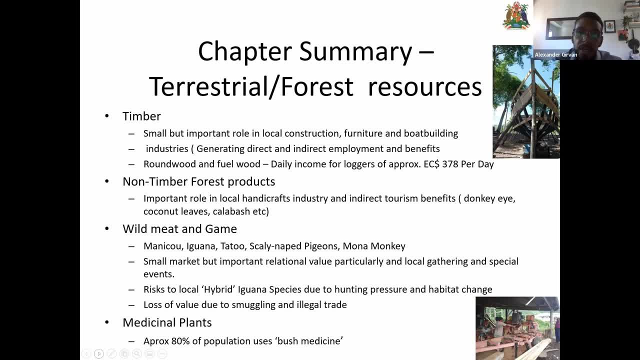 and Petit Martinique. We heard that in Petit Martinique and Karikou they now have to more import wood. But this historic they still harvest wood but they're importing more and more. Of course, boat building is very much a part of the identity. 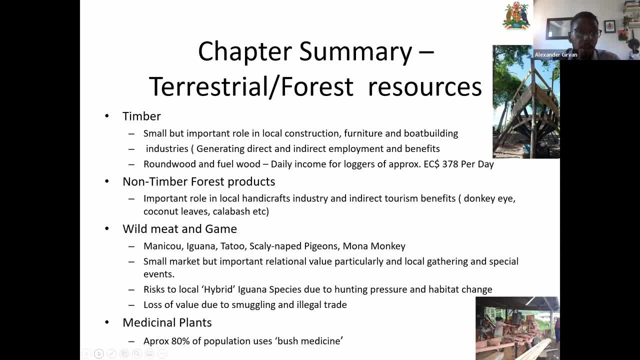 The cultural fabric of Karikou and Petit Martinique, but also a part of the tourism product. So again here you know we're seeing the value may be X and replaceable, but it's actually worth way much, much more because these traditional boat building. 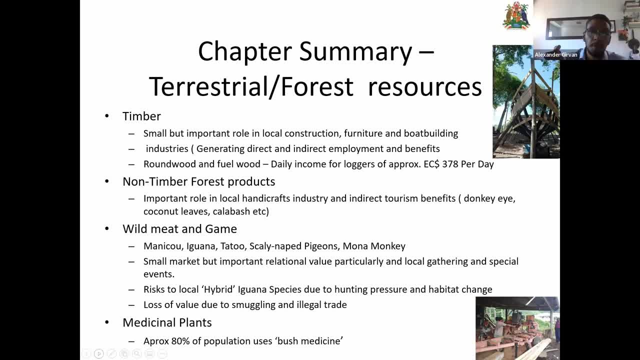 skills can be lost when you're having to import process lumber versus produce lumber on island. So these industries generates, you know, a decent amount of direct but also indirect employment and benefits. We found that for roundwood and fuelwood the daily income for loggers is approximately. 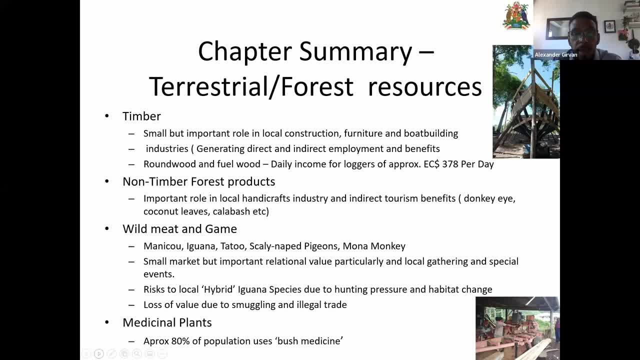 378 EC per day, so almost 400 EC per day. So again here you know, the forest is basically putting money into these people's pockets. But again, you know, what we really want to highlight is these indirect benefits When you make a local furniture. 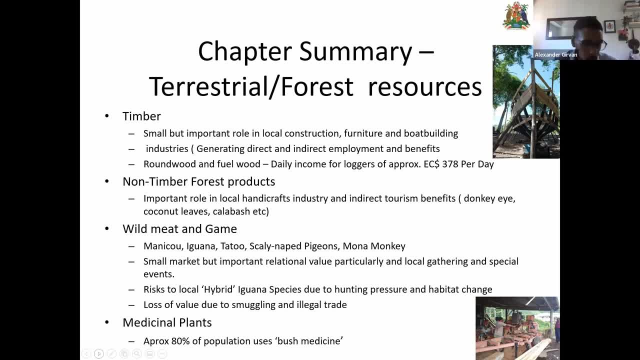 for a small hotel. it, you know, makes that hotel product even better and makes it more attractive And gives you a competitive edge over other Caribbean islands. in theory. You know, when you have a locally built boat, you know people come to Karikou and Petit Martinique. 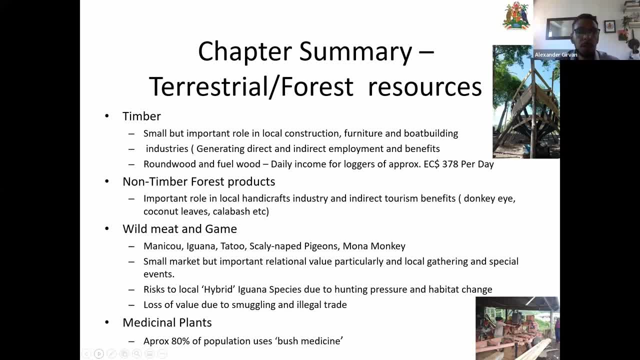 to see these locally built boats, because it's different from a fibergrass boat. So the timber is important, but the add-on benefits and also the relational values in terms of green identity are potentially even more important than the dollar values. In terms of non-timber forest products, we found that these 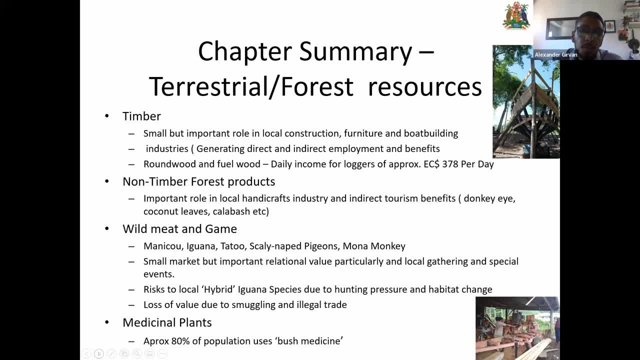 play an important role in the local handicraft industry and indirect tourism benefits. So things like donkey eye, coconut, e-leaves, calabash, you know, reeds for baskets, et cetera. So significant values in terms of the value-added products produced from these things. 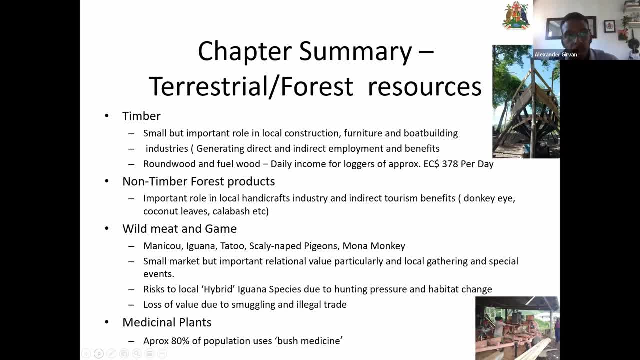 And then, well, wild meat and game. we you know, had you know our values were in the chapter in terms of the values of manikou, iguana tattoo, skanea pigeons and the Mona monkey. 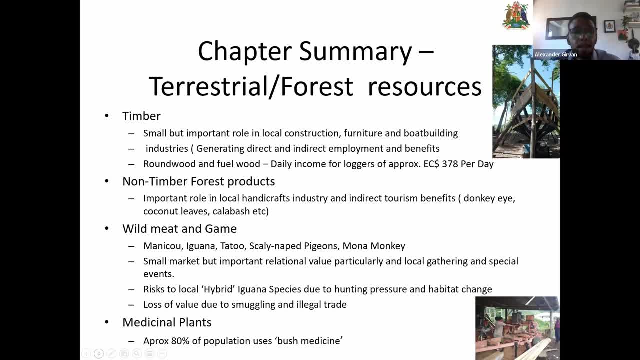 And some of these are actually quite important economically. But again, you know, despite having a kind of relatively small market and not out-competing other protein sources, it's still a very important relational value, particularly to local gatherings and special events. And I'm not so sure if I'm going to use the right word, please. 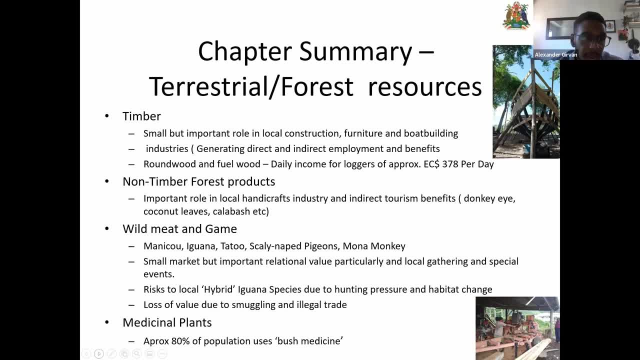 I want a Grenadian to correct me, but basically I think you have, you know, card limes where you play cards, and river limes And these things are very important to these events. I'm assuming also there are big parts of carnival and carnival fets. 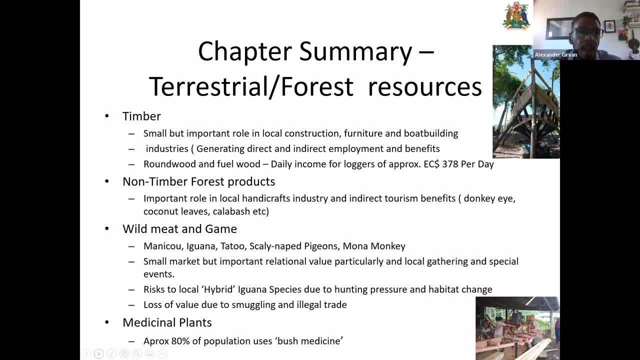 A kind of a wild meat, being very much a part of unitary identity, And the reason that people want those there is because it's not the same as chicken. It's actually quite different and unique. So, despite having a high level of importance, we saw some risks to local iguana species. 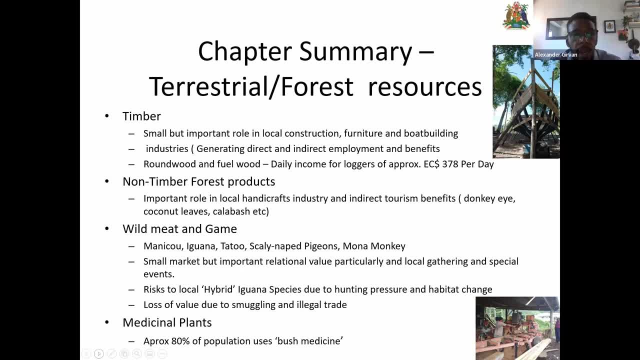 the hybrid species due to hunting pressure and habitat change, And some losses of value due to the smuggling and illegal trade of these products up the islands but also into Grenada. So important, But some serious risks to the continued provision of these services because of 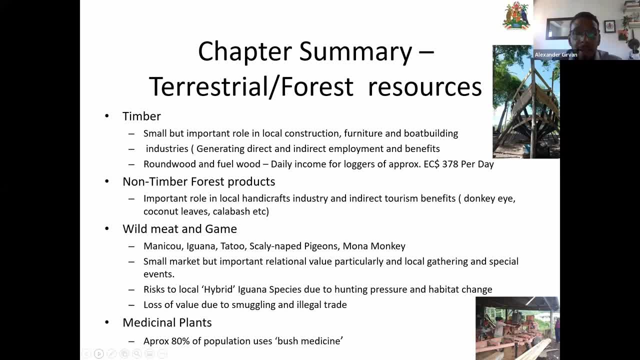 other types of environmental change. Now, medicinal plants. We found that 80% of the population say that they use bush medicine which, again, in terms of, you know, healthcare, but also to treat small ailments or minor ailments. you know, again, that's a lot of significant value or income saved for these. 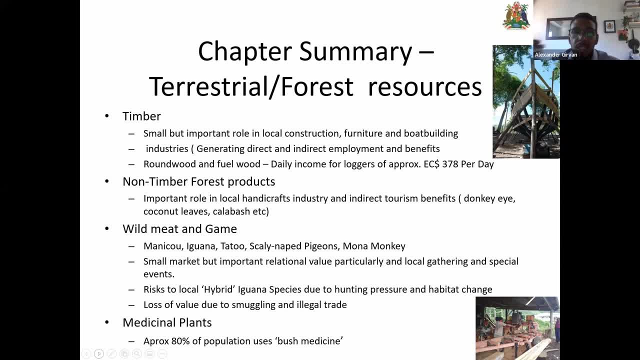 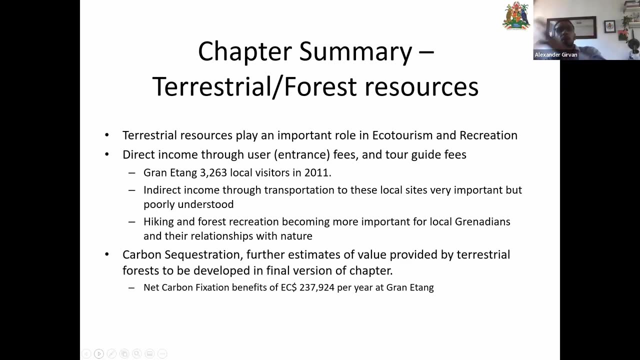 individuals, But also it has significant future potential as a genetic resource and I think that's something that Aria and Rhea can speak to. that, if need be, Next slide please, While people really think about coastal resources and Grenada, you know. 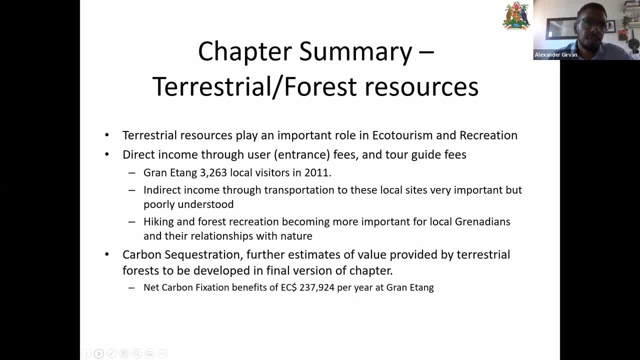 sun sand sea, kind of as a Caribbean tourism product, we found out. terrestrial resources play an important role in ecotourism and recreation nonetheless, right, And there's a lot of direct income earned by the state through entrance fees to national parks. 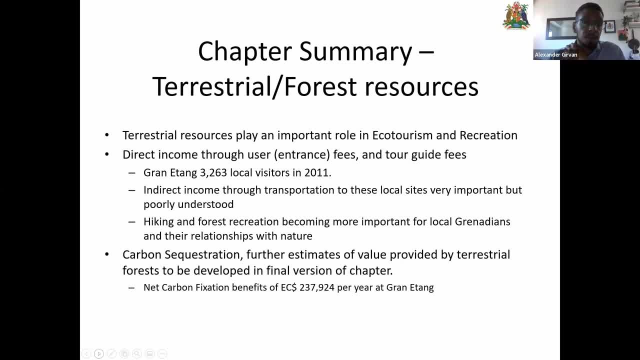 but also to individuals in the private sector through public transport and so on. It's not just about the private sector, It's also about the public sector. It's about the public sector through tour guide fees, right? So we found out. Granite Tang Lake had 3,000 visitors in 2011.. 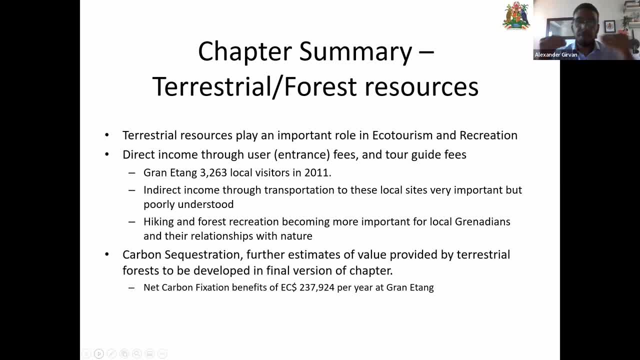 And what we were unable to quantify. we'll be very grateful if people could help us fill these gaps. is sure you know the sun, the sand, the sea is great for the silver sands and the big resorts. but to the local, you know person, taxi driver, person who has 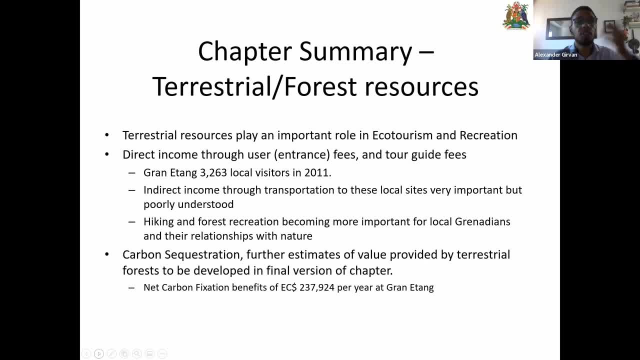 a small cook shop. you know the fees generated from the travel fees. you know the fees generated from the terrestrial tourism. taking somebody to the Granite Tang Lake, driving them there in a minibus and then offering them a tour guide actually is very important for people's individual. 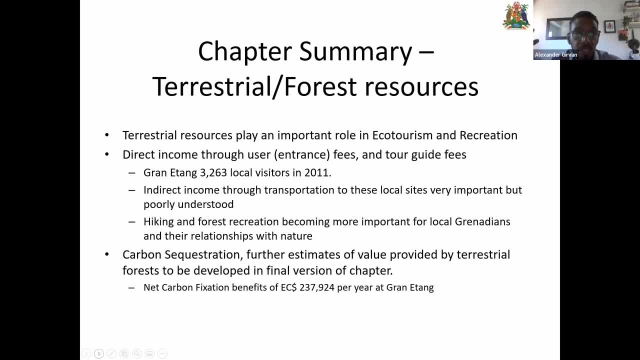 income. So this indirect income from the terrestrial sites is very important but also poorly understood by the chapter. We would love to get more information on this. We also got anecdotal evidence and I'll be very grateful to hear from Grenadians about this. 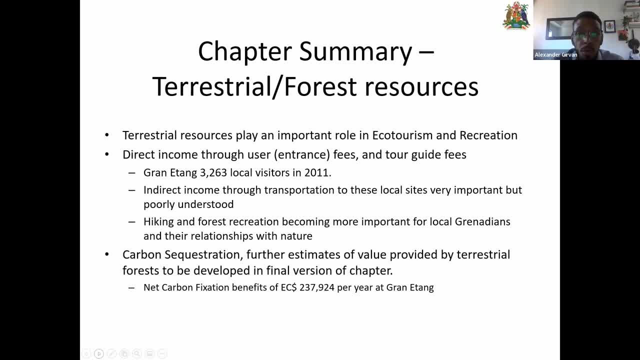 that hiking and forest recreation is becoming more important for local Grenadians And their personal relationships with nature, And I'll be very interested to hear if this you know. people found this was true or untrue, particularly during the pandemic, when people couldn't travel as much, if there was a kind of turning inwards to domestic tourism. 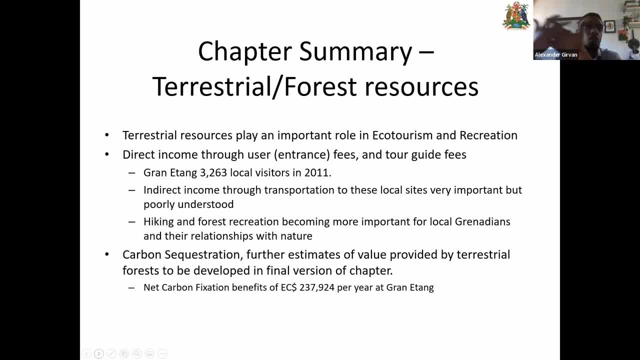 and terrestrial hiking experiences: to go to the river, to go to the waterfall, kind of in hiking groups, because anecdotally we've found that this has increased. Our current iteration of the chapter has some information on caravan sequestration. 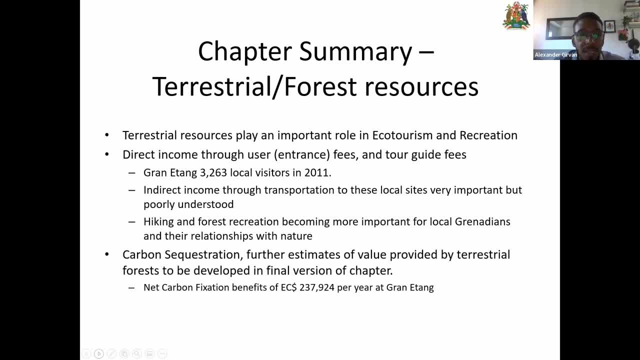 but we would like to develop these further to get more robust estimates. But we already have an estimate of the net carbon fixation benefits provided by the forests around Grenadines Lake as being about quarter million EC per year. So 250, 237,000. So close to a quarter million. So we're assuming that the carbon benefits 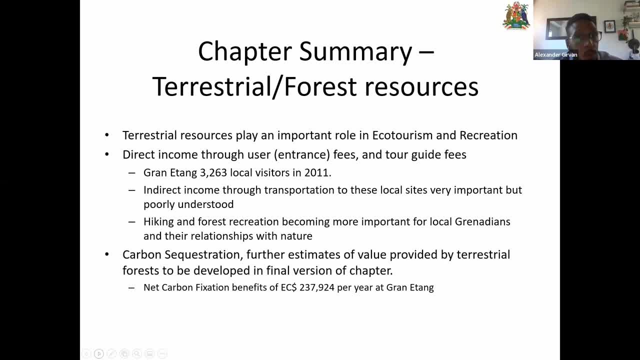 provided by these forests are quite significant And we can definitely put- and we will be putting- a dollar value to those estimates based on whether or not our carbon could be sold in carbon markets. But I think what's important to highlight here is we'll probably get a very big dollar. 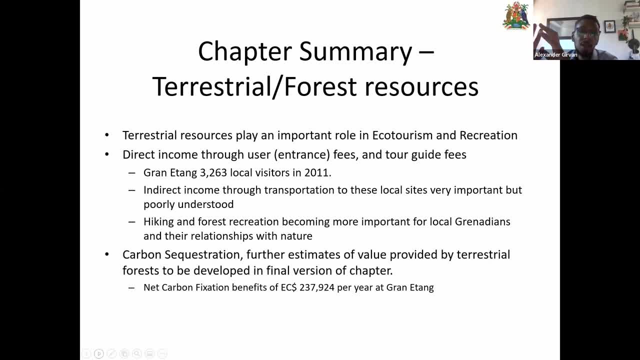 value here for how much this carbon could be sold in markets, But maintaining the ecosystem's ability to store that carbon and the other services provided by those ecosystems are potentially more important to local Grenadians in terms of erosion control, in terms of the water cycle management, as was mentioned earlier, which is one of the 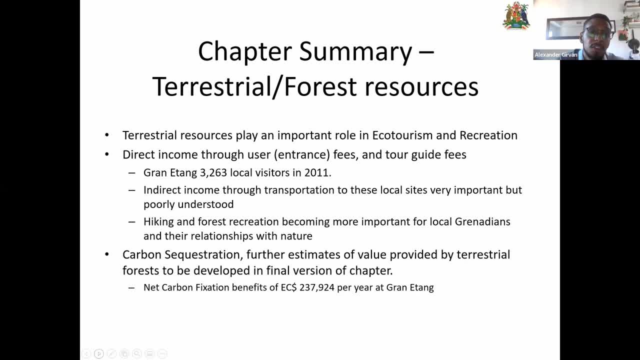 biggest risks from climate change. So we will be providing more detailed estimates of carbon sequestration. I'm grateful for any comments on how you want us to reflect that. But also there are other services provided by IFRS which are equally as important, even. 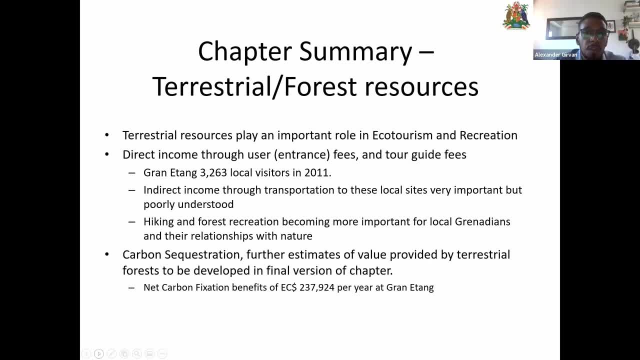 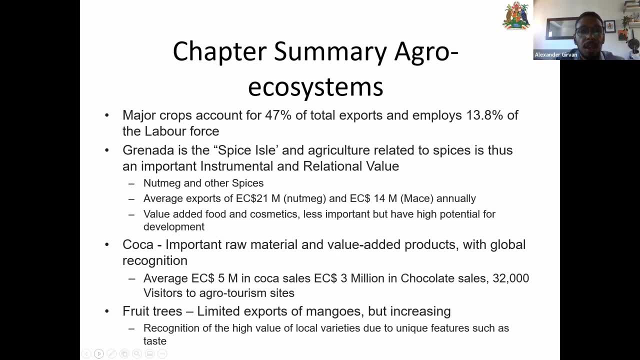 though they may not have as high a dollar value. I think I'm going to pass over here to Aria. if correct, What's the next slide? Yes, So this is. we're going into agro ecosystems and I'm going to pass over to Aria. 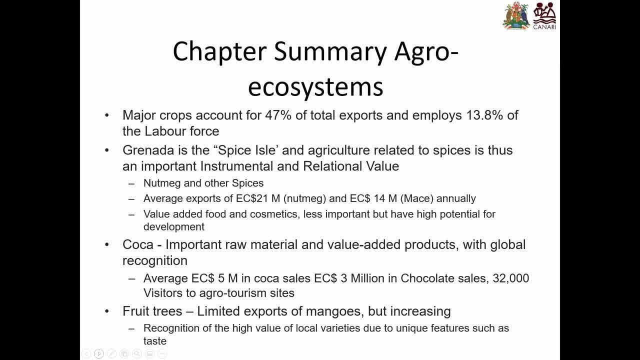 Thanks so very much, Alex, for an excellent start. Well begun is half done, So, just following up, I am going to take us through talking about the values, The value of agriculture and agro ecosystems. a little bit of a touch on the One, Health. 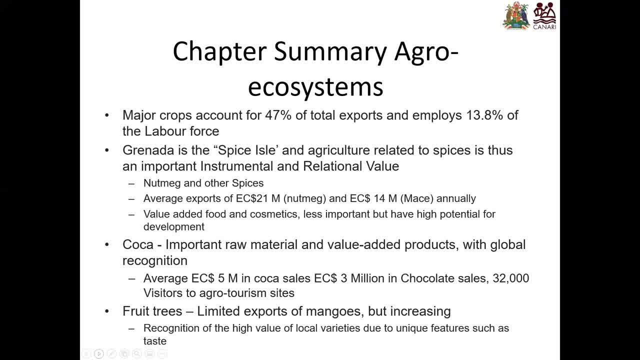 approach a little bit on the summary of emerging issues and recommendations for policy makers. So we don't have too much to do and I'm going to just zoom through it quite quickly. So, in terms of agriculture and agro ecosystems and value there the available literature, 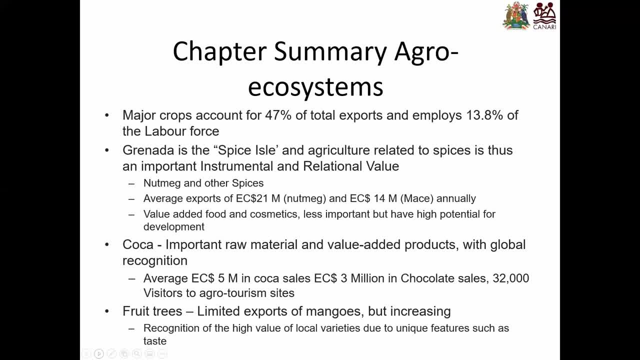 has identified that major crops account for 47% of total excess carbon sequestration. So that's a lot of carbon sequestration. That's a lot of carbon sequestration. That's a lot of carbon sequestration. And then there's church transport, which is particularly important for the economy. 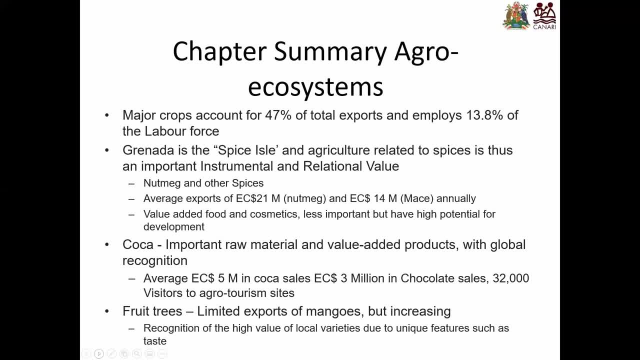 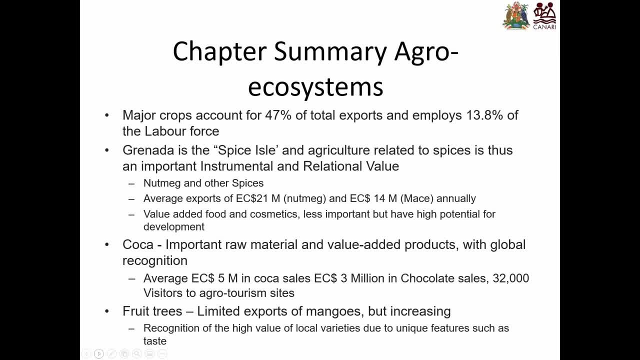 have been identified. An average of 5 million in cocoa sales, as well as 3 million EC in chocolate sales, with approximately 32,000 visitors to agro-tourism sites like the Guav station that we have, Belmont Estate, etc. etc. was also identified. Fruit trees have limited export. 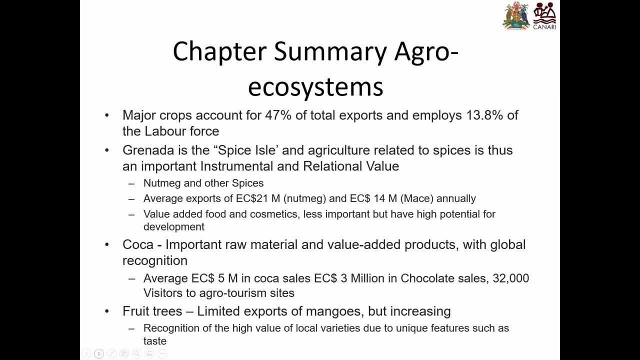 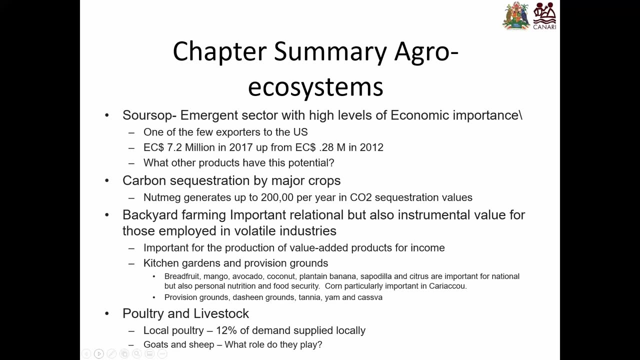 for example, with mangoes, but those seem to be increasing And there was a recognition of the high value of local varieties, particularly of our mangoes, due to unique features such as taste. Next slide For soursop. this is an emergent sector with high levels of economic importance. 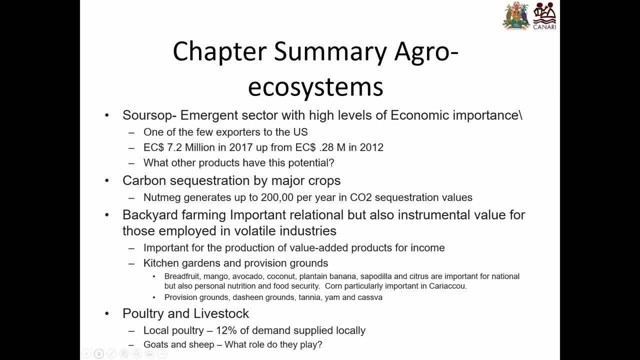 so economic value Grenada enjoys, being one of few exporters to the US of soursop and netted 7.2 million in 2017.. So when we looked at the values we got in 2012,, which was 0.28 million, and again up to 2017,. 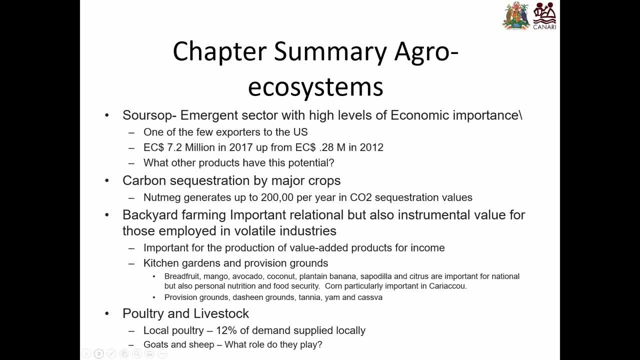 there has been some increase there, considerable increase in the value of soursop, But there are other products that may have this potential and we appreciate having some discussion. I think that we also want to learn about the economic dress code of C, or that is a. 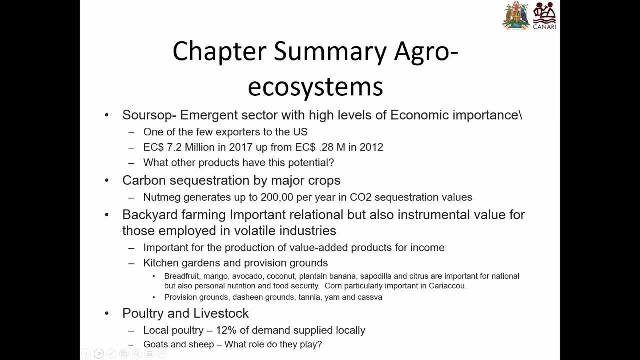 very big coin to have thought before we get into the value of the carbon sequestration. Last slide, please. Next slide, please. carbon nutmeg can sequester as a plant and then when we estimate per hectare whether it's mixed. 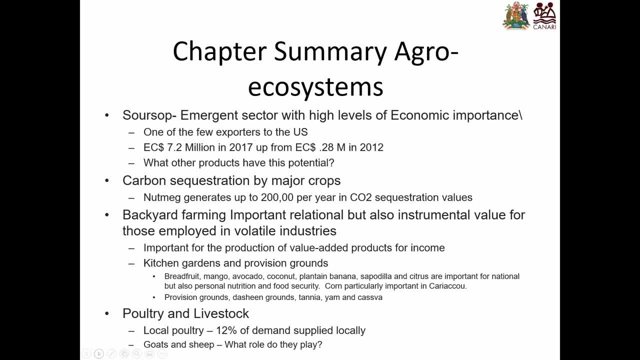 stands with banana and cocoa or whether we have less stands and with appropriate spacing and a conservative estimate is 200 000 in carbon pricing per year in terms of its carbon sequestration potential. and that's really important to us because it says not only do we have the value within watersheds and agro ecosystem, but now in the context of climate, 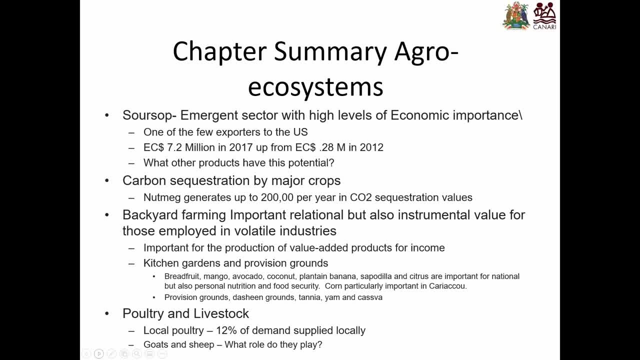 change and our fight to capture and store carbon. we recognize that there are, that our agricultural lands can also give us support for that. backyard farming was also identified as important for both relational and instrumental value for those employed in more seasonal or more volatile industries, and it's important for the production of value-added. 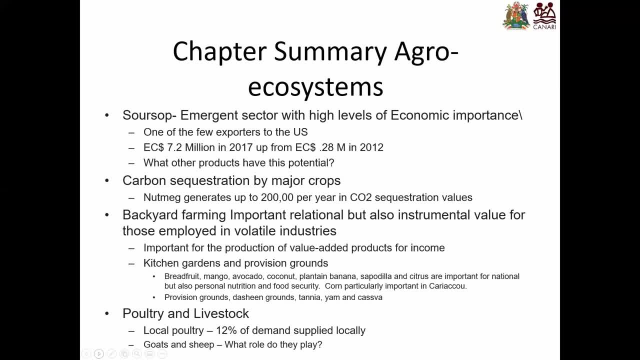 products for income and kitchen garden gardens and provision grounds including breadfruit, mango, avocado, coconut and provision like dasheen tanya yam, were also really important, both instrumentally but also relationally culturally, for the poultry and livestock and the value from poultry and livestock on island. local poultry was 12 of the demand. was supplied locally goats and sheep. we still are not. 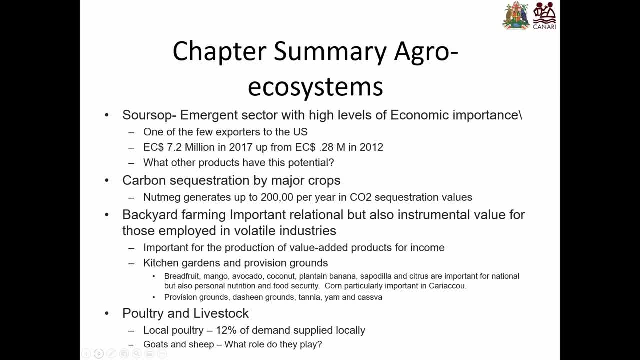 understanding fully and would appreciate some more information, um as a chapter, on what role do they play in terms of their value, both locally and if exported, and we're talking about both the economic value, the cultural value and the, the value in a, in a bigger picture, intrinsic cells. 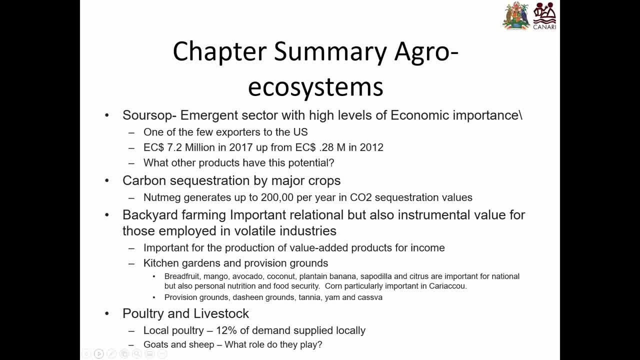 as part of bigger ecosystems and again, as as indicated by alex, we are looking at an um nature's contribution to people, which is a little bit more wider and more flexible than the, the more traditional ecosystem services, and is very, very much supported by the apes methodology. next slide, please, for poultry and livestock. 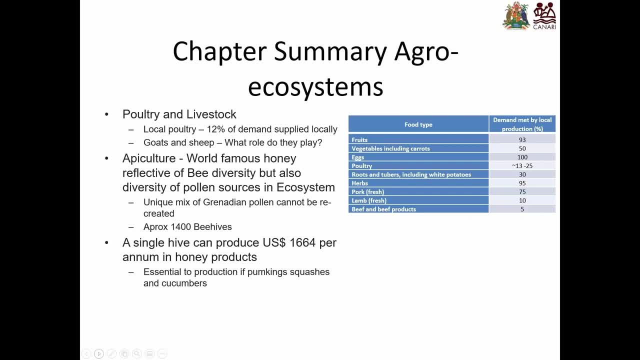 as i indicated, 12 of the demand is being supplied locally and we need to know a little bit more about goats and sheep. for bees and apiculture, grenada produces world-famous honey, reflective of the bee diversity, but also the diversity of pollen sources within ecosystems, and that unique. 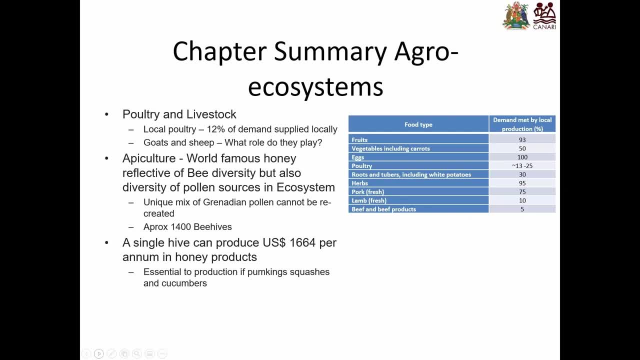 mix of grenadian pollen cannot readily be recreated and you can see there that we're starting to. to tease out the value of that, and approximately on island um suggested that there are 1400 beehives where a single hive can produce us 1 664 dollars per hectum per per annum. sorry. 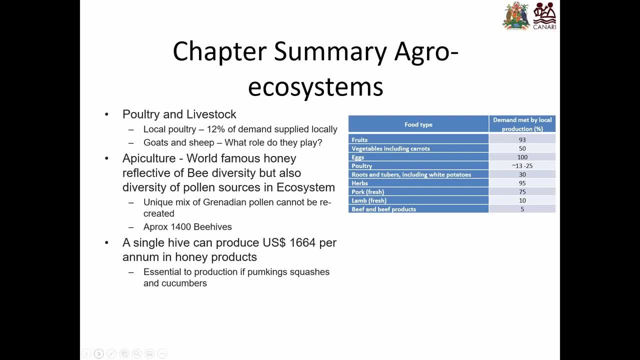 in honey products and these are essential to production of pumpkin, squash, cucumber and other species that rely on bees as pollinators and indeed all pollinators in general. and you see a lovely table there. i don't want to go into too much detail. that looks at the, the food type and 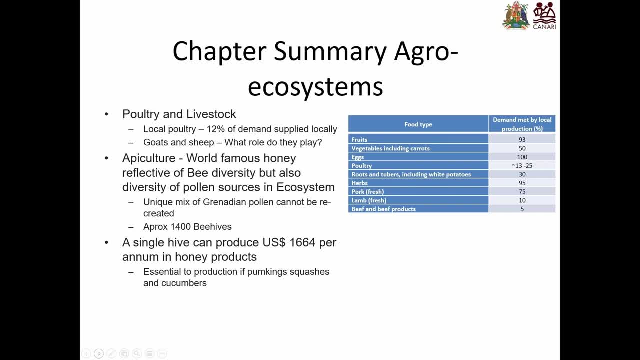 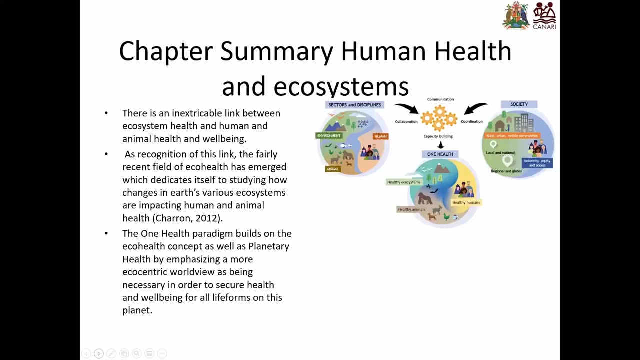 then the demand that currently is being met locally, which speaks to the value of these species, both economic as well as intrinsic and cultural. next slide, a little touch on human health and again, having come through the pandemic, we're really aware, and even before the pandemic, of the inextricable link between ecosystem health. 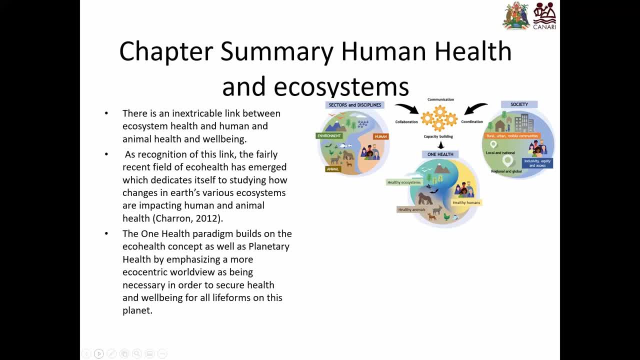 human health and plant and animal health and well-being, and this has been well encapsulated in the, in this section in the, the chapter which speaks to the one health paradigm and it's against. this link has spawned a relatively recent field of eco-health which has emerged and which is 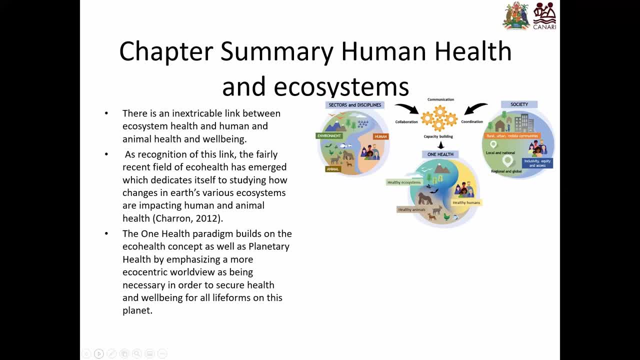 dedicated to studying how the changes in the environment are going to affect the environment in the earth's various ecosystems are impacting human and animal and plant health. the one health paradigm builds on the eco-health concept, as well as planetary health, by emphasizing a more eco-centric world view as being necessary in order to secure health and well-being for all. 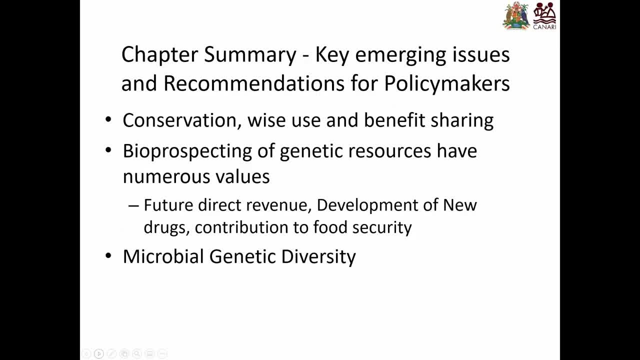 life forms. next slide just a few emerging issues and recommendations as we move into our small discussion. the first is to make sure that, as part of the recommendations for management of our biodiversity, we include conservation, wise use, as well as benefit sharing, both monetary benefit as well as non-monetary benefit sharing. a second key recommendation that 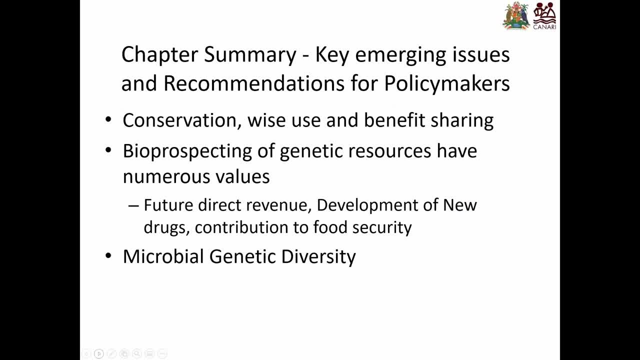 came up in prior discussions and listed was bioprospecting and the opportunities of bioprospecting of genetic resources, which have numerous values. they can provide future direct revenue. they can also be involved in the development of new drugs and contribute to food security. we in our small group discussion this morning heard a 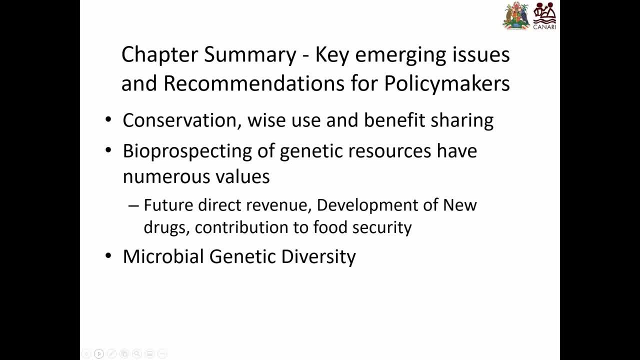 little bit already about microbial diversity and the importance of soil health, but this speaks to not just soil health on land but in general, the effort that needs to be focused on microbial genetic diversity: myofauna borax in the marine environment, in the freshwater environment, as well as the terrestrial myofauna. 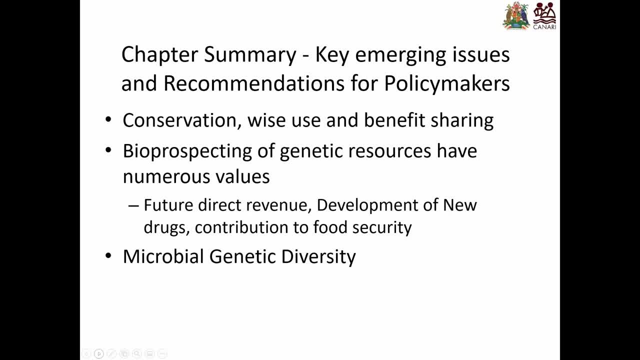 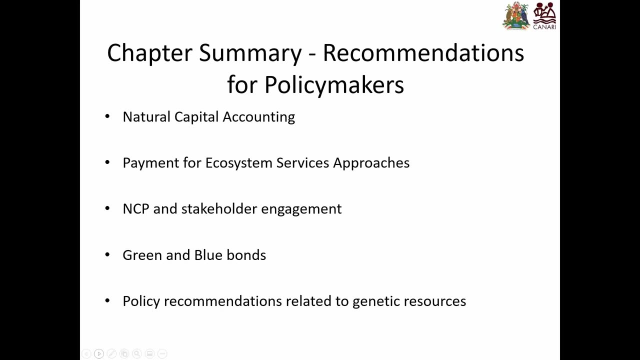 which exists between the grains of soil and sand but are really key in carbon capture and storage and maintaining healthy soils. next slide, thank you. finally, just to touch on the, the final part of the recommendations. the chapter touches a little bit about natural capital accounting and here i think we've had some already um rich discussion. that looks a little bit different. 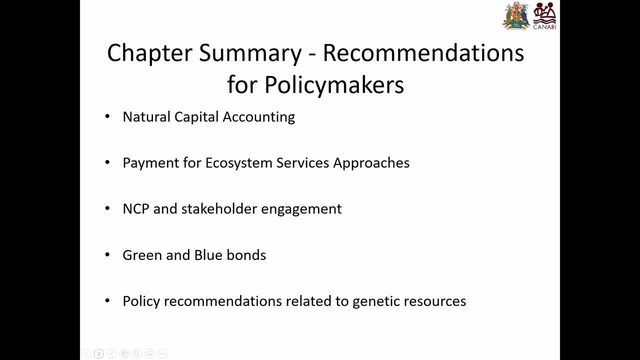 from what we've had in the past, but i think it's really important to look at making the linkages between the value of species and the value of ecosystems and how that is balanced in the equation for decision making being done by policy makers- and in the past i don't think that these 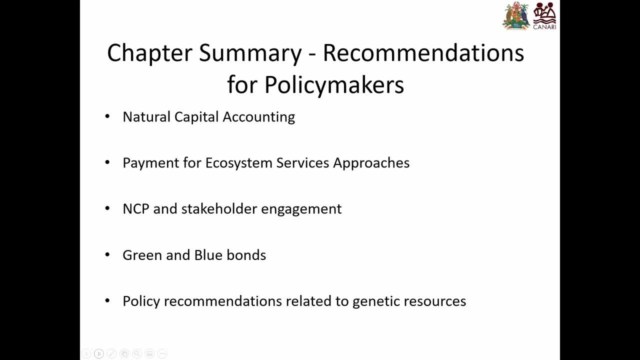 values may have well been captured in that equation, or indeed they may have been missing from that equation. so now, through this chapter and through the near, we get that opportunity to really place in text island what kinds of values we are placing on, and not just economic value, but also cultural value. 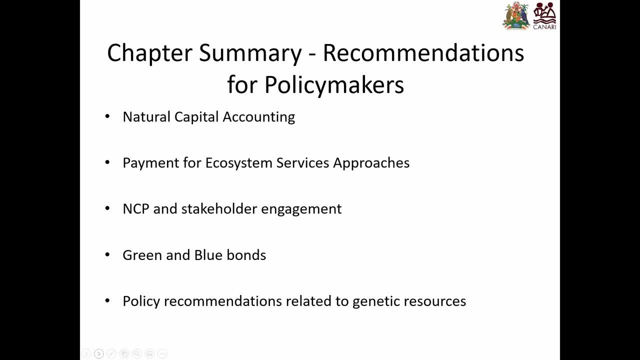 to us and, as highlighted by alex, the cultural value is being found, particularly for local communities, to be as important, if not more important, than the typical economic values that we are accustomed to using um in the development decisions, etc. etc. touching upon payment for ecosystem services approaches talking about nature's contribution to people and the need 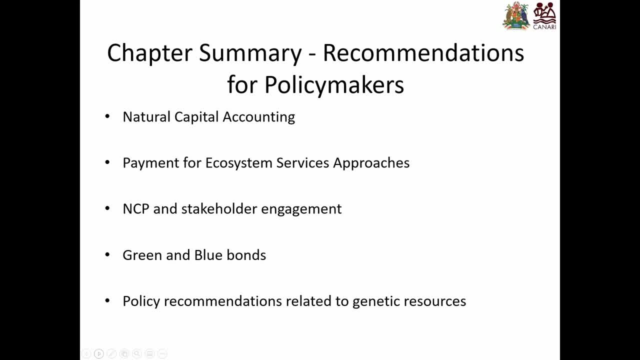 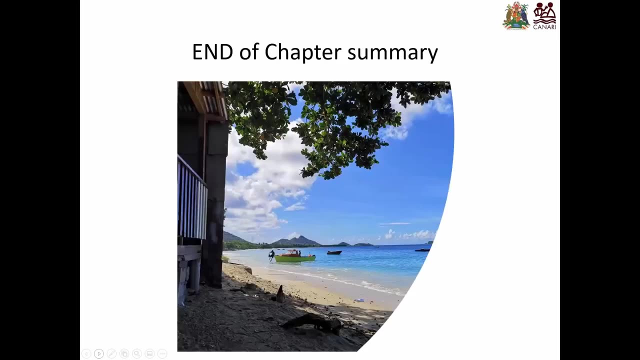 to make sure that we have robust stakeholder engagement, touching on green and blue bonds and policy recommendations related to genetic resources. on that note, i want to close and invite us all to move quickly to the breakout sessions, where we will be addressing specific questions looking at coastal and marine ecosystems, freshwater resources, terrestrial 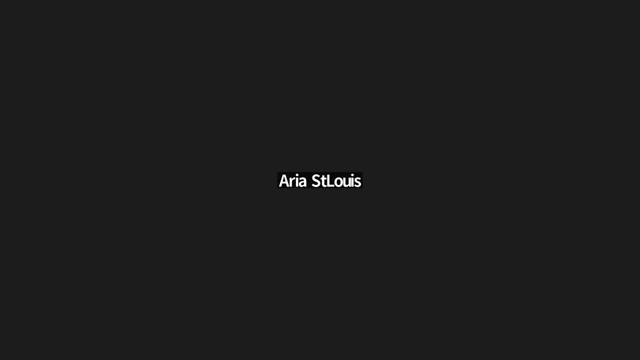 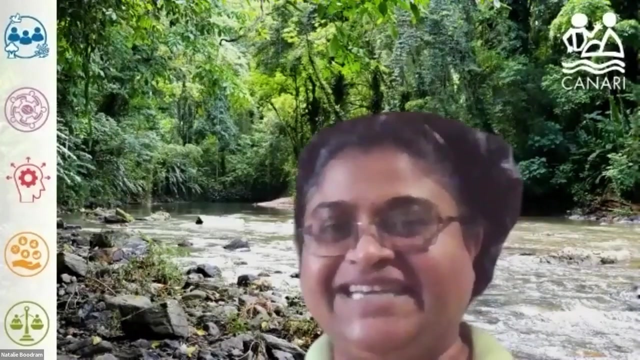 forest resources, and then the agriculture and agro ecosystems, and then some other questions that we have for you to to look at and give us some feedback. thank you, and over to the chair, aria. okay, so i know you're concerned about time. um, i will open the floor for two comments before. 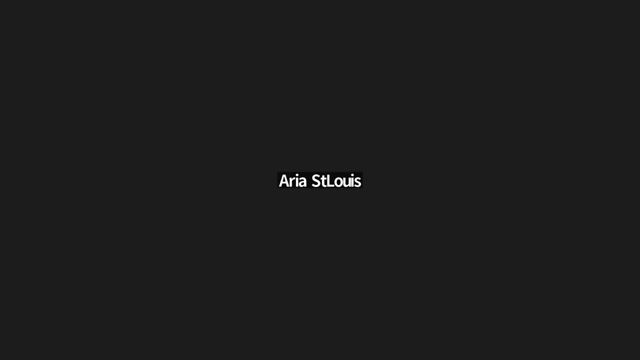 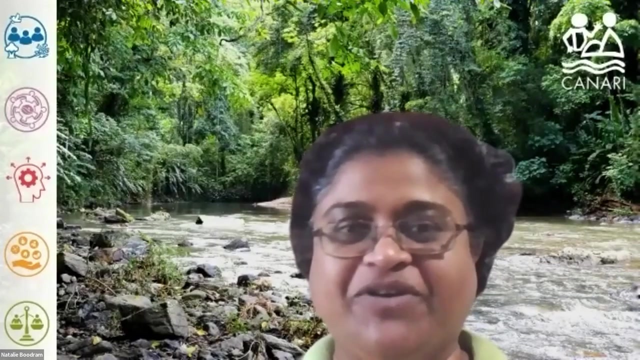 we go today. oh, i beg your pardon. yes, sorry about that one. if anybody has anything they would like to say in plenary before we go to um, the breakout groups, just to say that was an excellent presentation, guys, joyce go ahead. joyce, you're on mute. yes, thank you very much. um, i hope i don't. 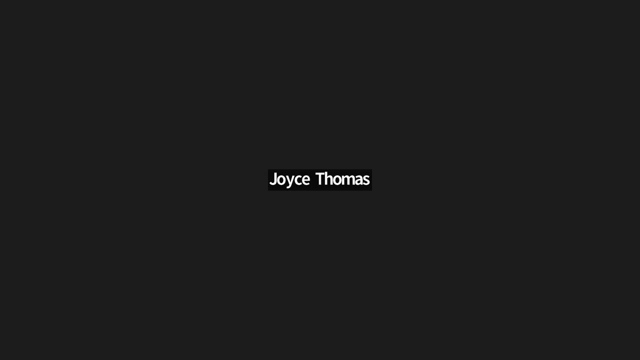 want to stay too long, but, um, okay, um, i have a number of things i wanted to raise. uh, one of the presentations, um, just for correction. um, i think it's important that when we- because you're speaking to grenadians- that we try to use our language, um, i know, teacher, is is vincentian, but they didn't. 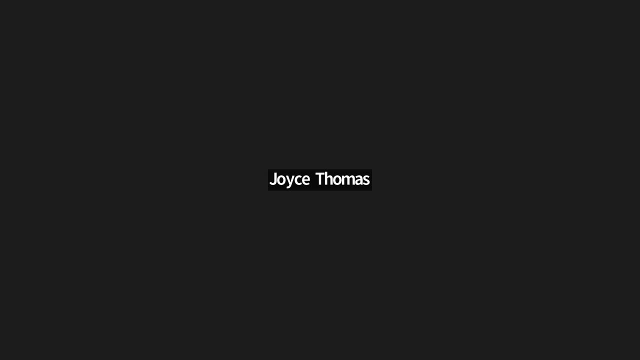 secondly, um, please, please you, um, what we do by the river is that they would make our waters with the crayfish. so please note that. um. one of the issues i wanted to mention is the issue of the drying up of the rivers, the loss of the rivers, um, while there will not be any water in the channel. 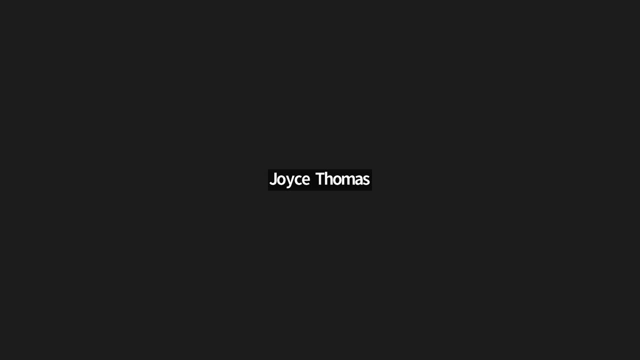 we have to remember that we have to note them as water courses, or else they will be used as for filling whatever put houses, development, and whenever it drains, the water will flow in the channel again. so this is something that that has to be emphasized: that even though there is no water in the channel, it will- it will rain. 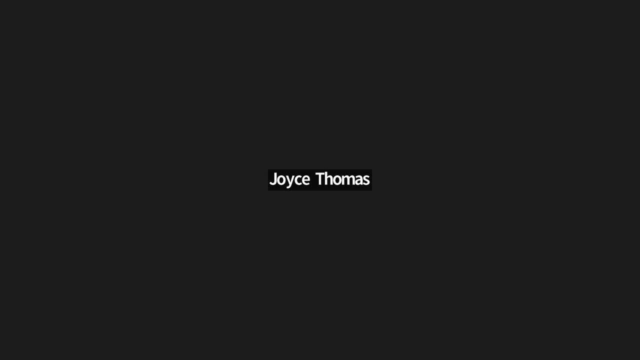 again just a little bit of concern about well for me personally, because I've been been involved in this business for so long. I mean I've not heard anything new out of it and I've told Natalie that already. but the good thing is that we are actually documenting it again and the valuation part is a 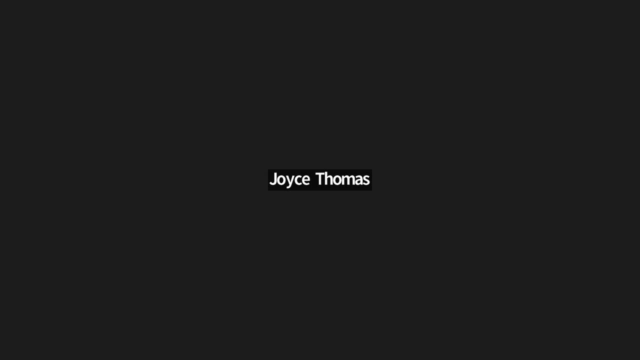 is a is is very useful, but in going forward in terms of getting- I know the intention is Natalie's intention- is to go past that and and to get to the, to the, to the policy makers and to to get action on the ground while the policy makers- I do think that they're not- 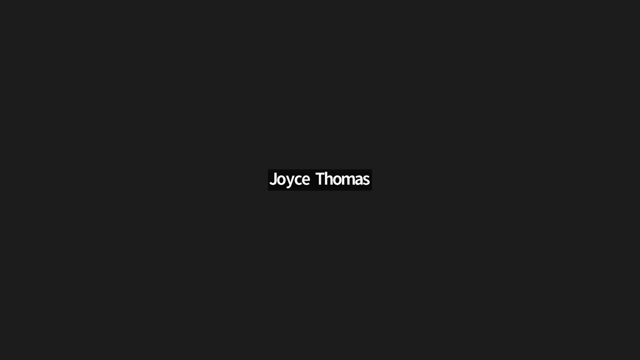 aware, you know from my experience, they are all aware. the question is whether they feel it feel motivated to do something about. it's a different story and and I don't want us to forget the- the important role that public officers play in holding the government ministries together. 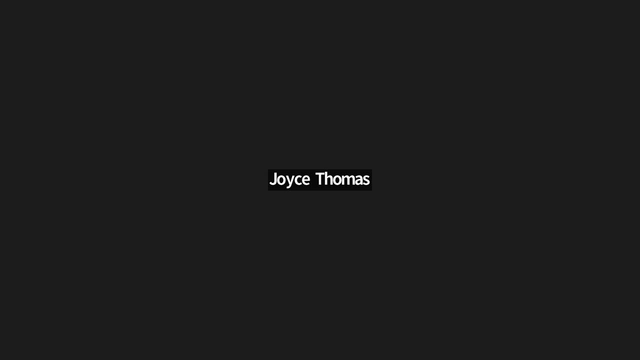 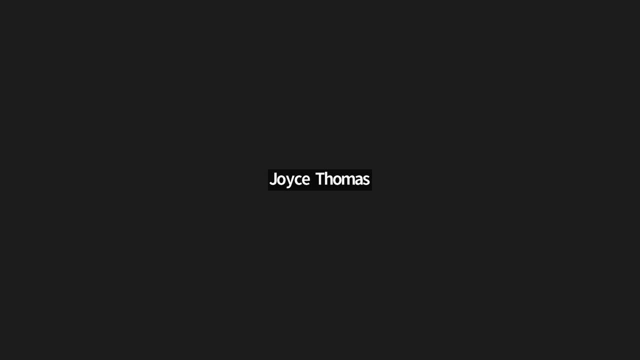 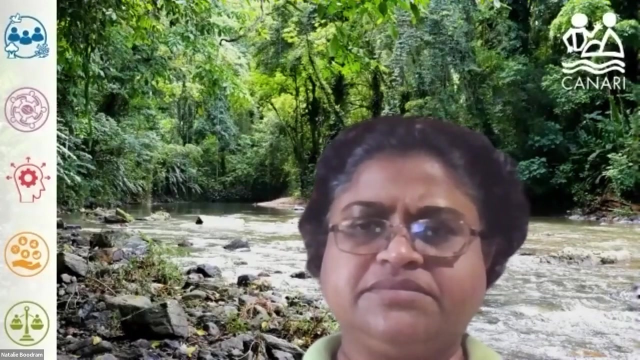 of the government ministers. I want us to think about the senior government officers and the technical officers in the various ministries. They are very important stakeholders. That's all I want to say, Natalie. Thanks, Joyce. Anybody else All right, so let's go. 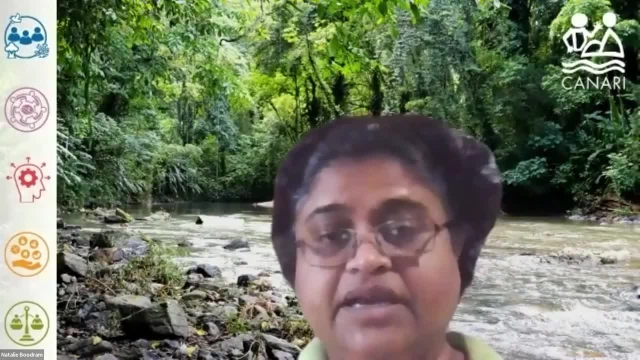 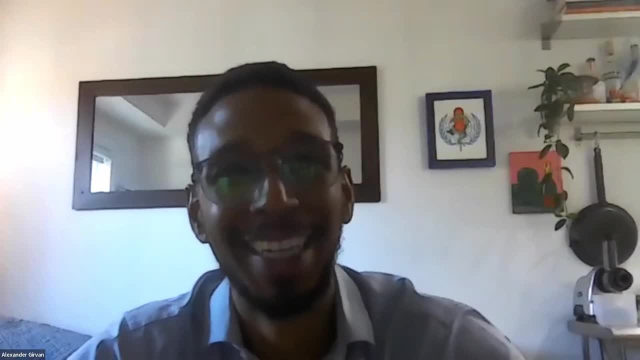 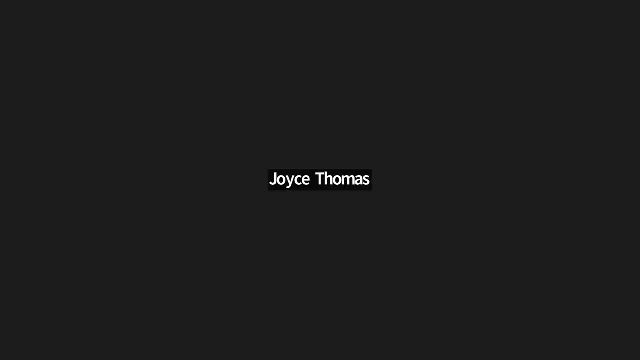 I'm not seeing anybody else. Let's go straight to the breakout groups, Joyce. I had one question. Joyce, you personally know how to make crayfish waters. Well, I don't know if they would enjoy it. My husband, he doesn't like the way I do it. 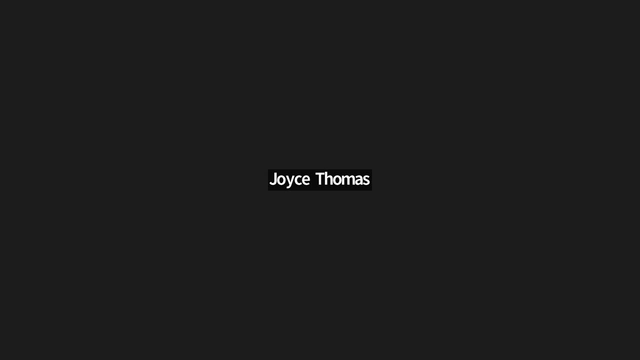 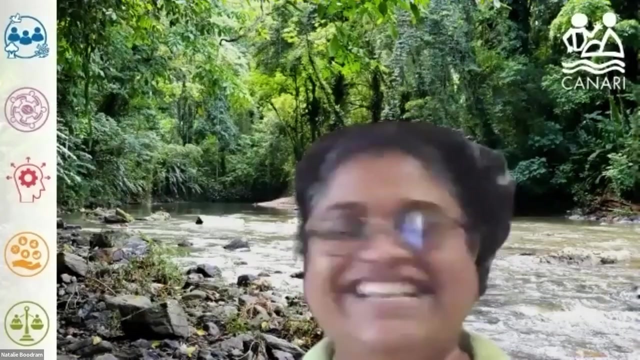 but the men have a particular way that the women can do it, so the men know better. All right, that works out Next time, next time. All right, okay, guys. So let's go to the breakout groups. Apologies, I know we may have. 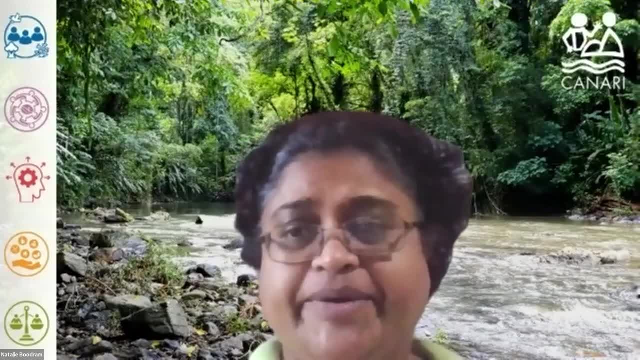 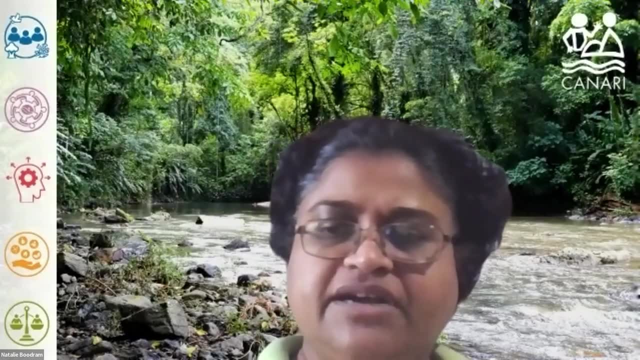 cut some of you short, but we're going a little too over, So I will ask the rapporteurs to please summarize and try and keep it as brief as possible. I want to finish no more than 10, 15 minutes from now. 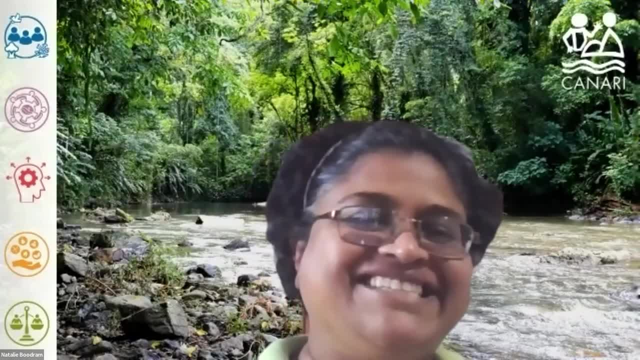 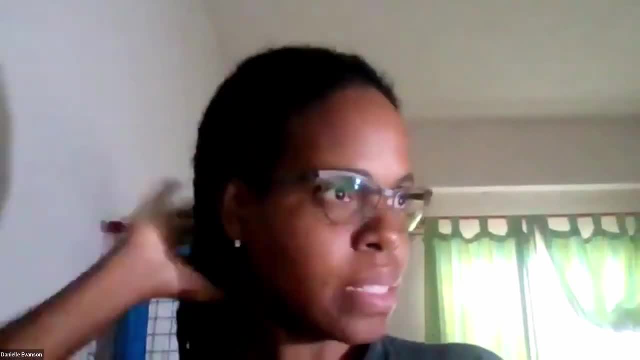 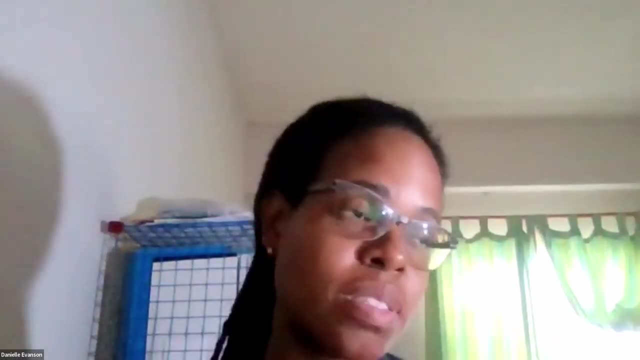 So, Danielle, I'll put you on the spot again, please, if you can start. Thanks, No problem, All right. so in relation to the valuable, the valuable ecosystems, we talked a lot about fresh water. Without water, there's nothing. 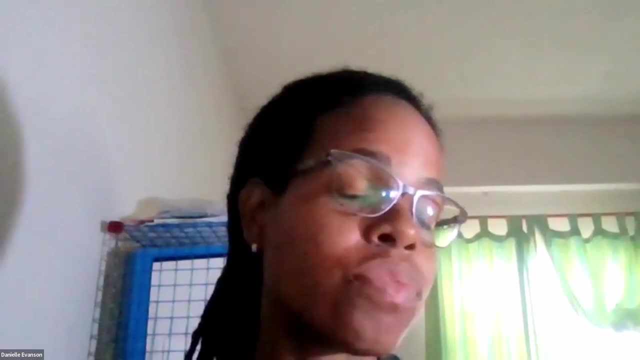 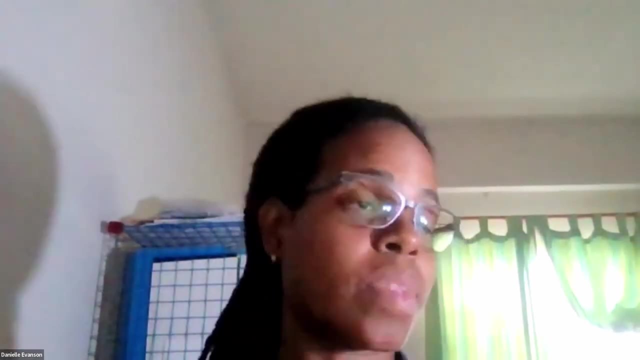 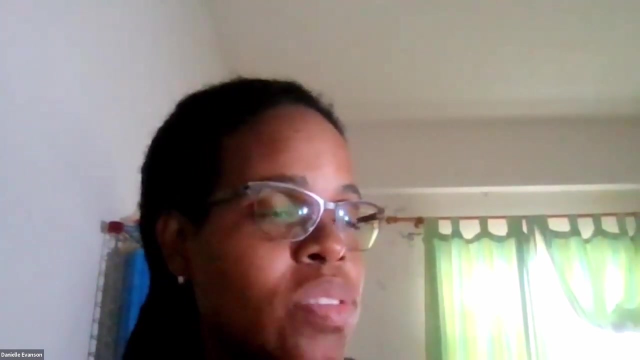 was one of the comments that was made. The reuse or recycling of waste water is an emerging topic, an emerging practice which is used for as a adaptation measure in water stress areas. It's limited. it's used in hotels to a limited degree. 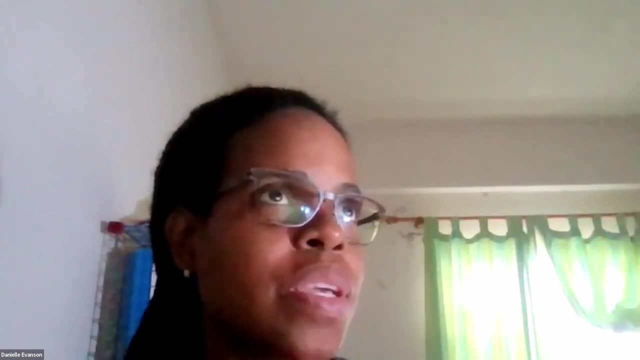 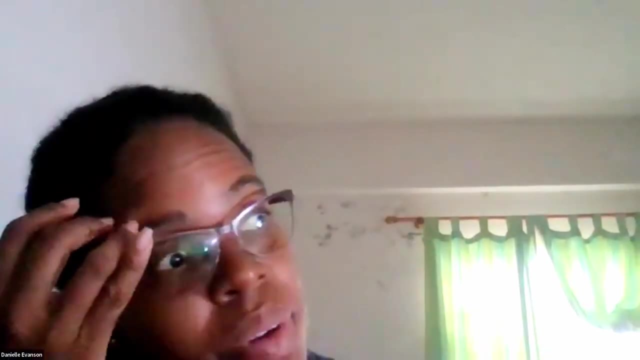 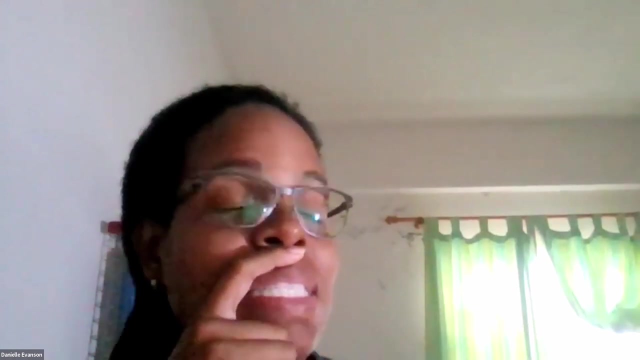 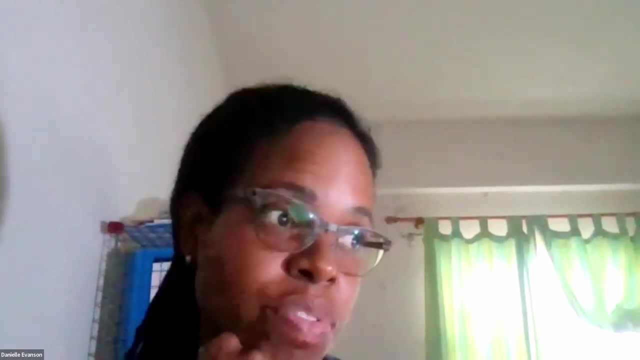 And it was also mentioned that the quantum of water reuse can be an indirect measure of fresh water value. There was mention of rivers and lakes being used for rinsing and dumping by cement trucks, which is quite disturbing, And you can see crayfish floating down river dead. 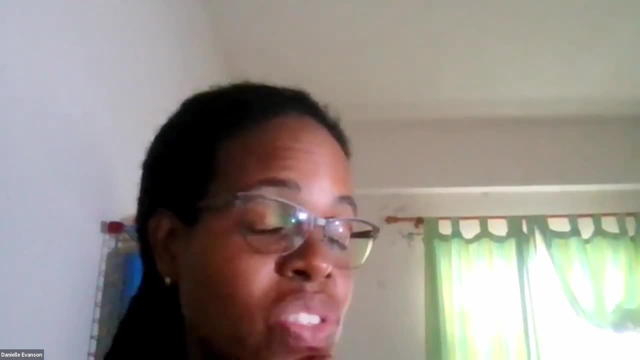 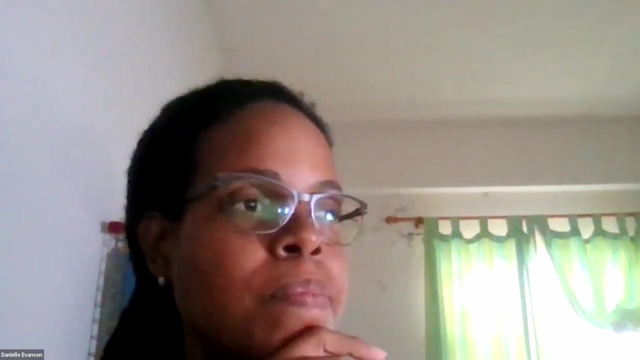 and it doesn't seem as though the people are understanding the effects of their actions or they don't care really. Litter, particularly plastics, was also mentioned as a threat to marine and terrestrial ecosystems. Terrestrial specifically because it's been. 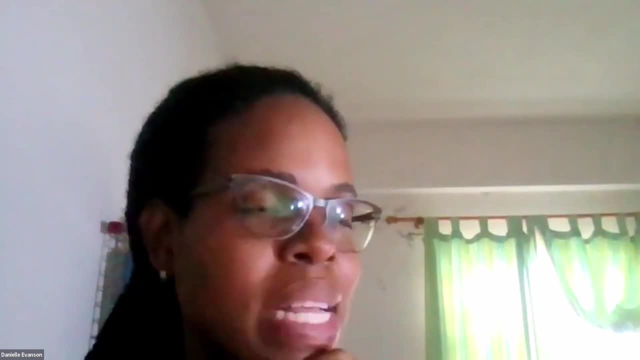 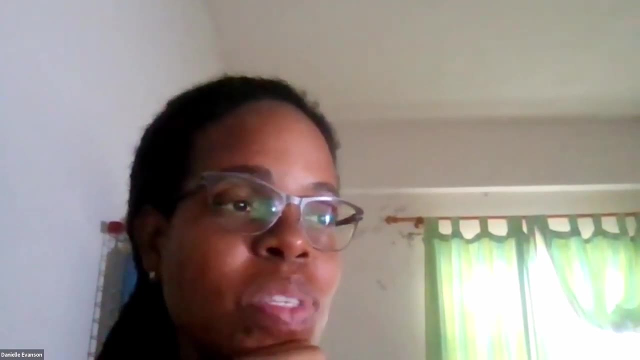 they've been shown as they break down to aid absorption of heavy metals in terrestrial plants. And one discussion that Ian had with some students- and I think it's a good one, but it's a good one- is that there's a lot of you know. there's a lot of you know. 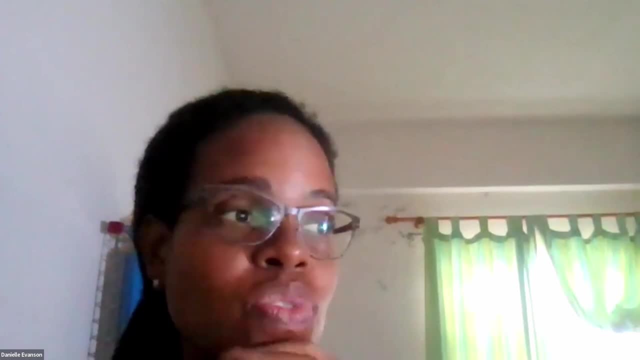 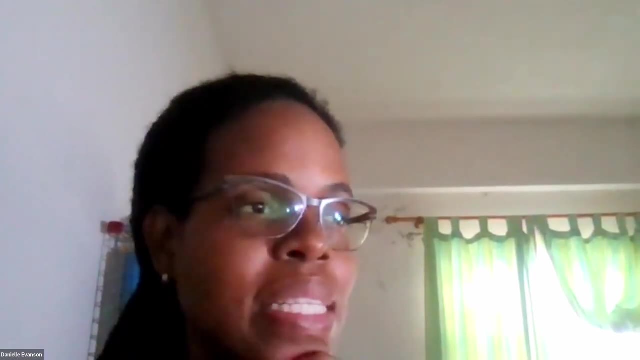 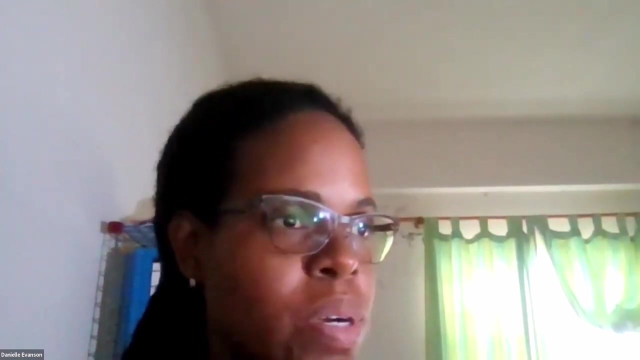 Swiss Chocolatier said that they are going to refuse to source from some South American countries because of the heavy metal contamination in their cocoa plants. So that has implications for that industry And we also talked about in terms of additional plants and animals. 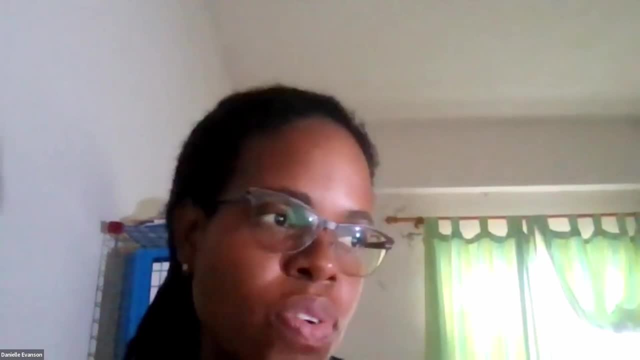 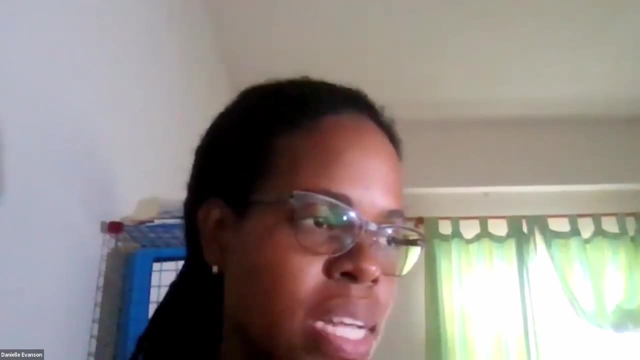 talked about bay leaf or boarden misuse for bay leaf. So all of those things are things that are going to be used in their collage. But it was also noted that you know we bought some of our chamado bay leaf at a local brewery in the Bay of bears. 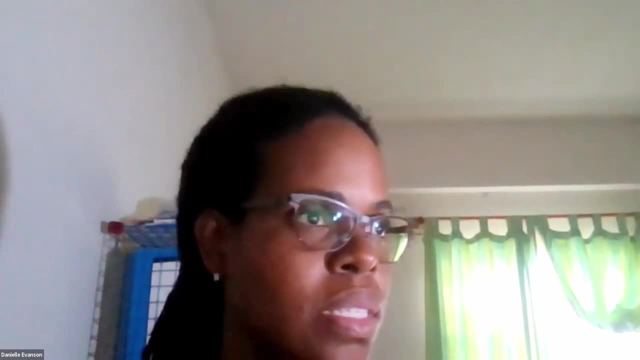 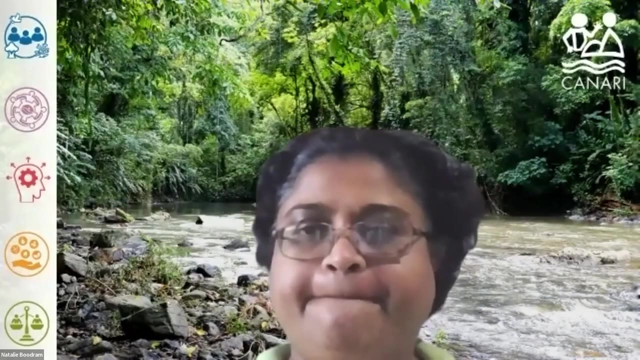 And we bought them some bay leaf. and we bought some bay leaf And I think that's an example of you know, we bought Bay leaf and I'm thinking about why we're going to do that. We also talked about the disgusting methods. 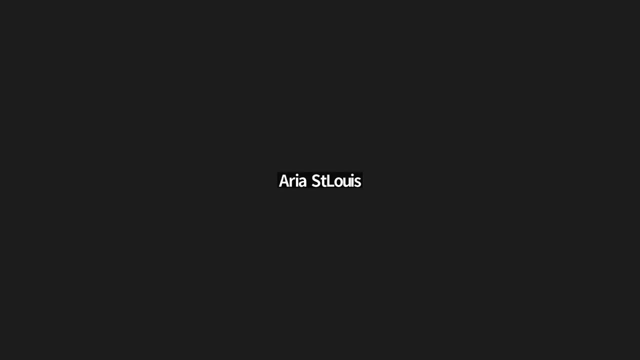 of growing bay leaf, which is it's one of the most difficult of crops to grow, And it has a very big effect actually, in fact ecosystems, And here we spoke a little bit under freshwater, about crayfish waters and cultural activities related to that, about the river still being an important resource for domestic chores. 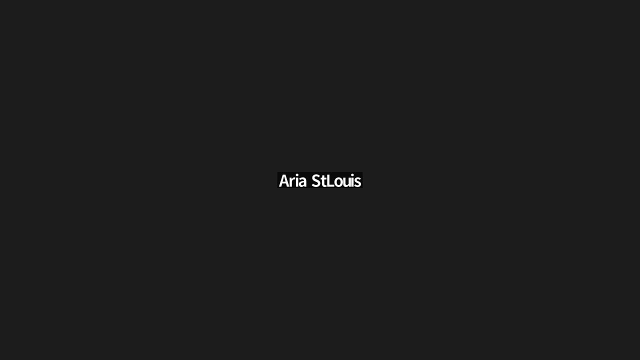 and that was raised by Joyce. Brian raised on bottling of water and the bottling water plants and the value attached to their businesses, as well, as he also raised not having piped water and having to use bottled water and boiling of rainwater and the cost that would be attached to. 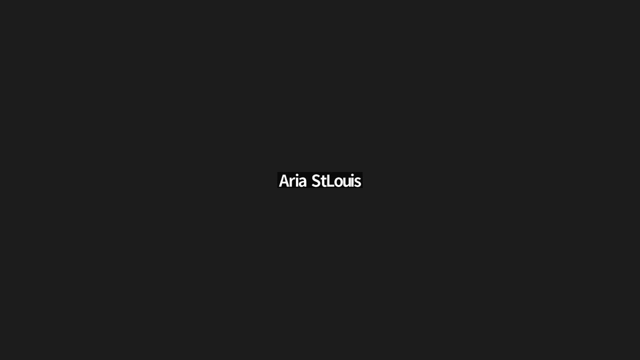 that For the marine environment. Brian also raised a question about the economic value of our ports and the vulnerability to sea level rise. but just speaking about the economic value of our ports And then when we move to the terrestrial environment- now we did move around a little bit- 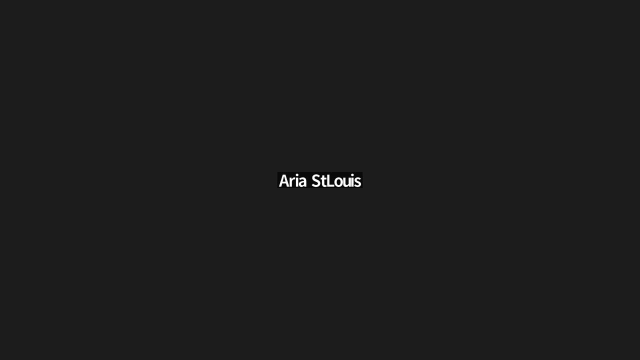 but I've covered freshwater, I've covered a little on marine and for the terrestrial environment. we spoke a little bit about sulfur springs, for example in Kleboni and the Shambo area, where they accommodate both locals and visitors, and it can be used for skin problems. We spoke also about backyard gardens and those. 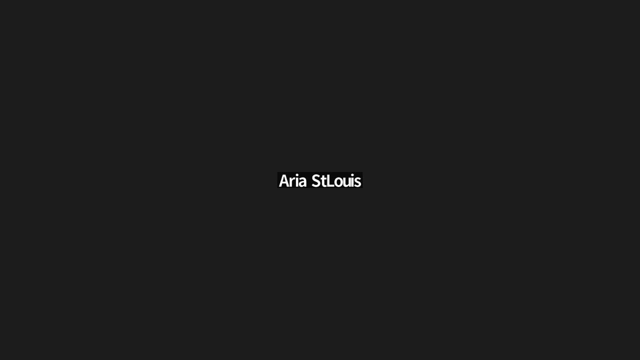 being really medicine cabinets. We spoke a little bit again about the importance of soil, and here Karim spoke a little bit about the importance of soil and the uniqueness of soil and how that helps with the flavoring that we see coming out in our cocoa. 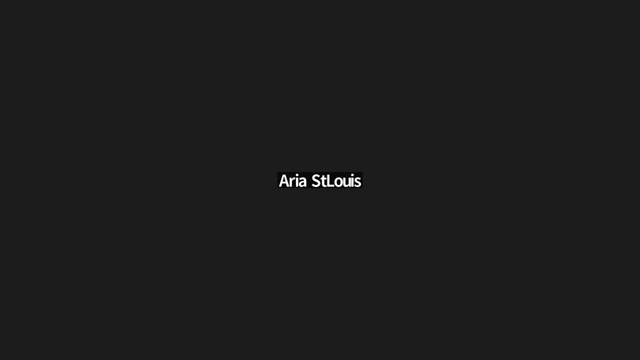 And the flavoring in our fruits. Karim also supported the idea of having a seed back in Grenada and an emphasis on understanding and documenting the diverse wild stock that we have and the value of that wild stock. He spoke a little bit more again about soil fertility, soil health and how. 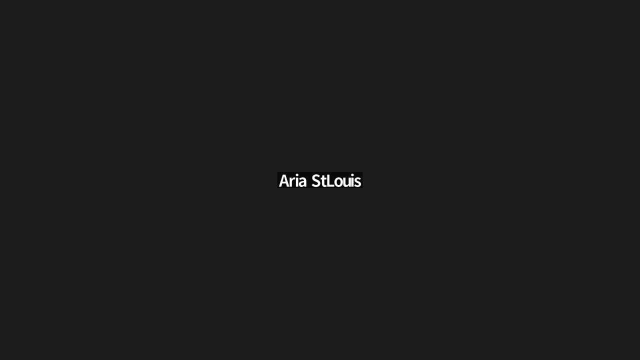 it is being managed, because the soils are vital to overall production and to feeding livestock, and the key emphasis being on how soils are being managed and the treatment. We heard a little bit more about use of already existing databases for fruits that needed to be updated and, from that, assessments done. 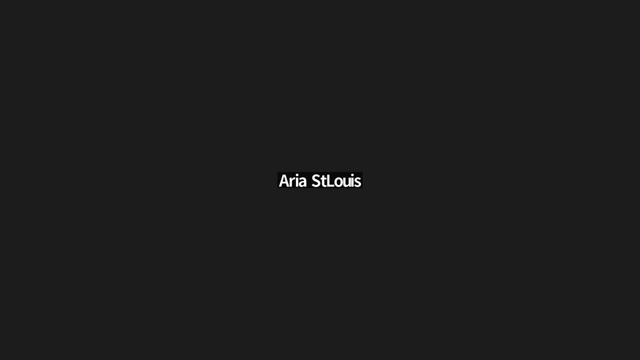 to understand what we are losing and the value of what we are using for fruits, for crops, as well as for medicinal plants. Kenia just lastly spoke a little bit under opportunities about the ecotourism opportunities that can be developed, and instead of having a focus on 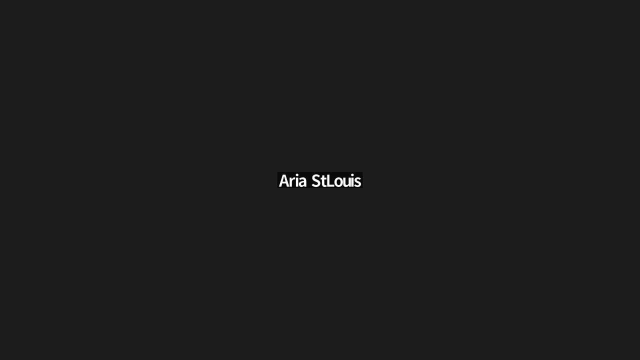 building big hotels have a focus in an ecotourism context, on smaller hotels, supporting hashing, hiking and that specific niche within tourism, the ecotourism niche For emerging issues. Brian's highlighted a little bit about things that help us with managing. 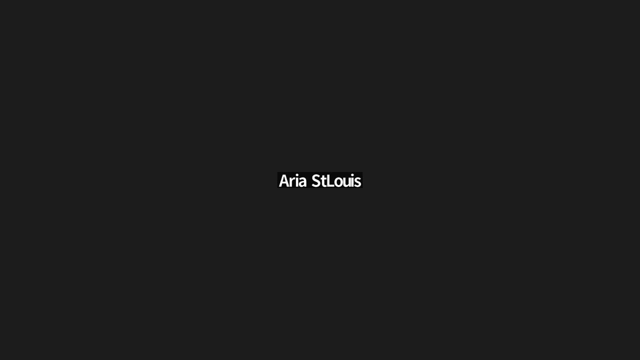 mosquitoes, not just because they're pests but because of the limiting of vector for diseases. So he spoke a little bit about that angle and the value of managing mosquitoes And we did have one or two things addressing not having stagnant water and improving water quality, water management, Again under emerging issues. Kenia actually spoke a little. 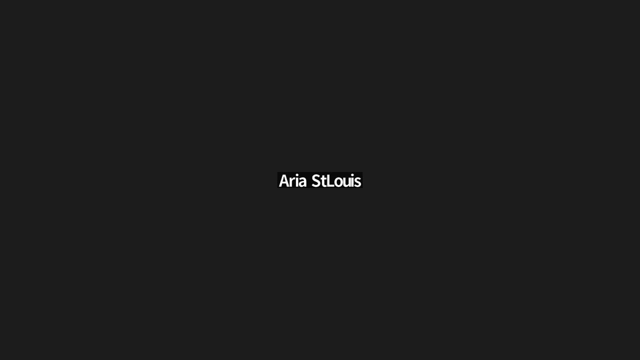 bit about exploring and looking at the One Health and the links to medicinal research, increasing research on medications. Right now we have a lot. we know that we have an increased risk of cancer, diabetes, hypertension, and there are local foods available that can reverse sometimes or else at the very least regulate. She spoke about 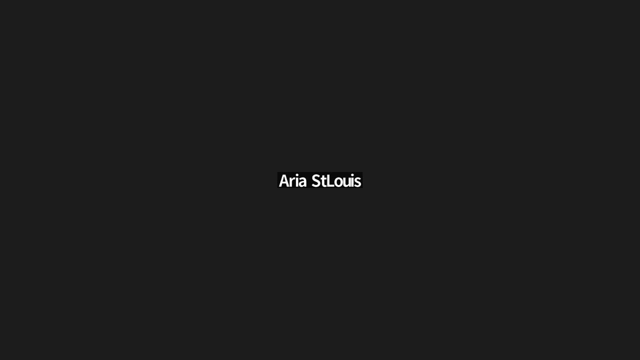 sorosap. we spoke about turmeric, ginger and other natural products and there the relationship to opportunities to get value from these. She also said that it would be really important to list the value and the benefits of the various fruits we have. So we've seen this for apples and sodas and so on. 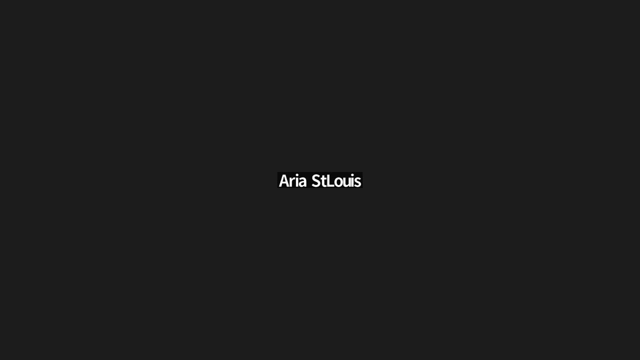 so on. I know that the Food and Nutrition Council does work to look at what our local fruits produce in comparison to when you hear about blueberries and so forth. So she spoke a little bit more about saying we need to have that kind of information well documented. That knowledge must be on paper. 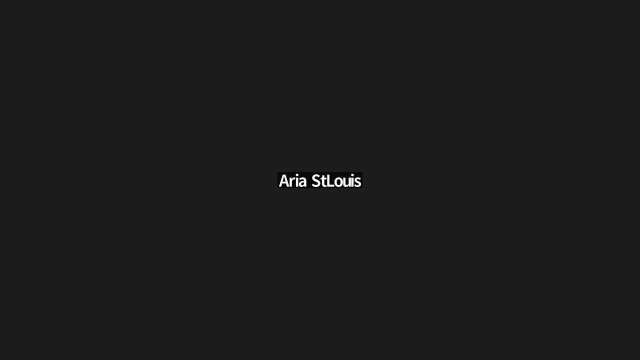 about. here's what we know. Another thing that came up related to that was, as part of emerging issues, that it's a two-sided coin, because we know that other countries can access these resources and, with that knowledge, go on to do research, patent and then benefit in monetary and non-monetary. 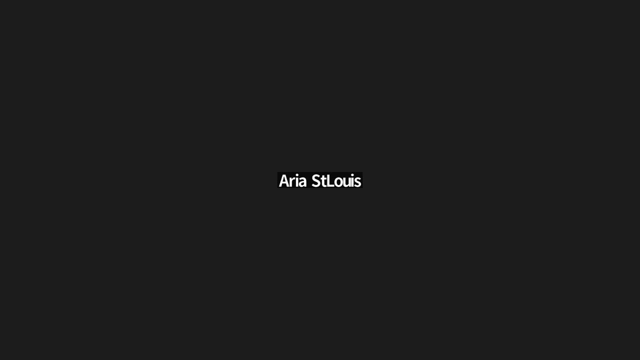 ways from all resources without us getting anything back, and therefore documenting this and also joining things like access and benefit sharing protocols and setting these up to help welcome that partnership. but recognizing that benefit sharing must happen was also part of the discussion- was important. The chapter was identified basically as 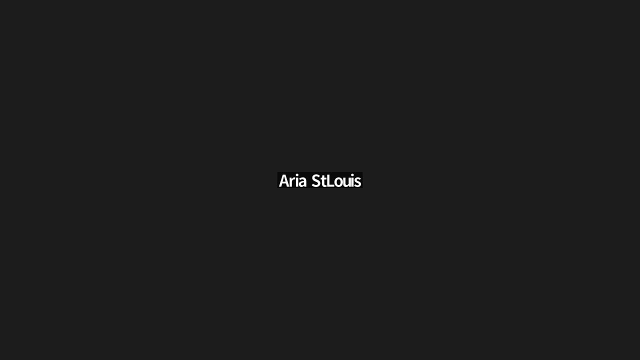 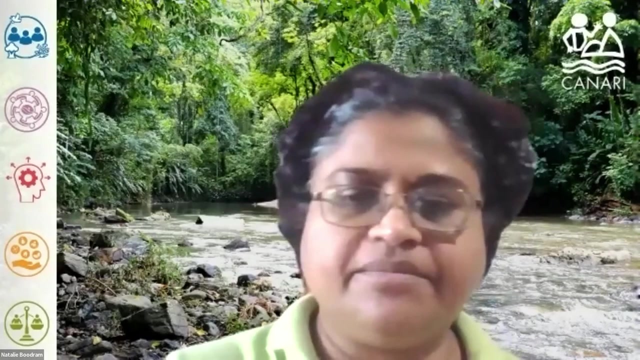 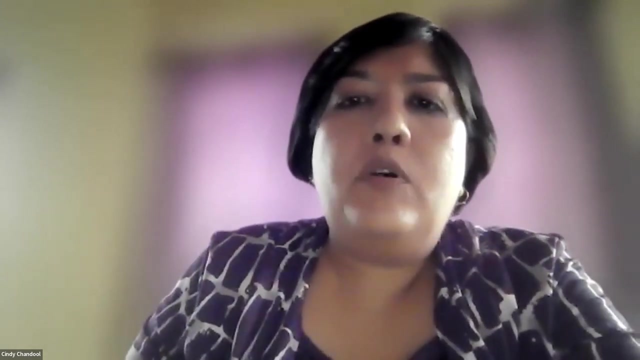 being a part of the discussion on how to access and benefit sharing. So I'm very excited to be here and thank you very much for taking time out of your time and being a part of this. Haha, thank you very much. Great thank you. Thanks, Natalie. So, in terms of coastal ecosystems, our group mentioned that. 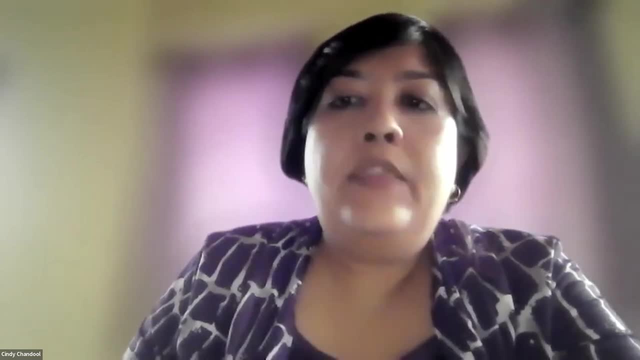 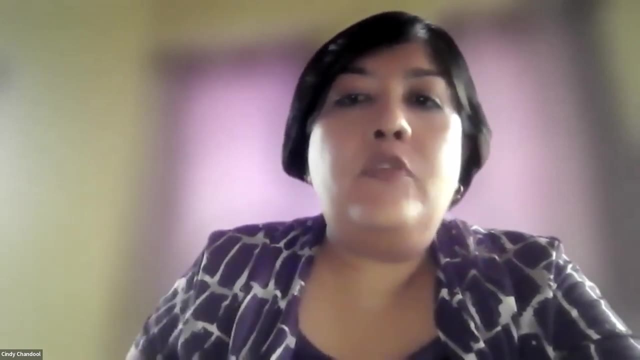 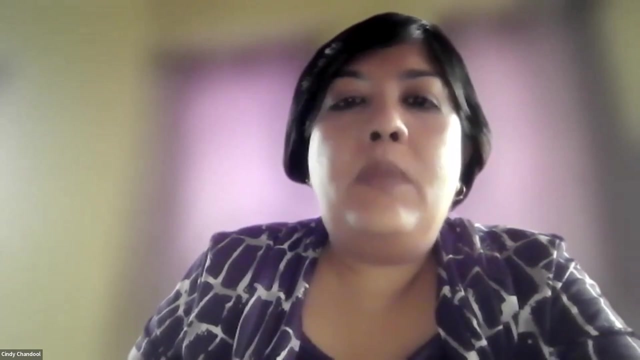 resources. species are getting scarcer or disappearing that many times. they may not be commercially important but are an important part of the food chain. So if you, if these are lost of, of course there will be issues with commercially utilized species also disappearing. So the mention was made of species like sardines and fry, which are bait fish for larger coastal pelagics. 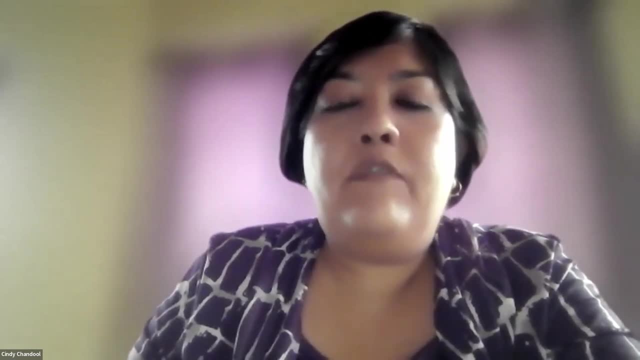 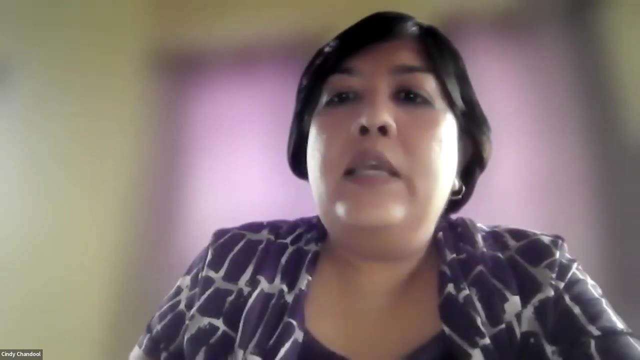 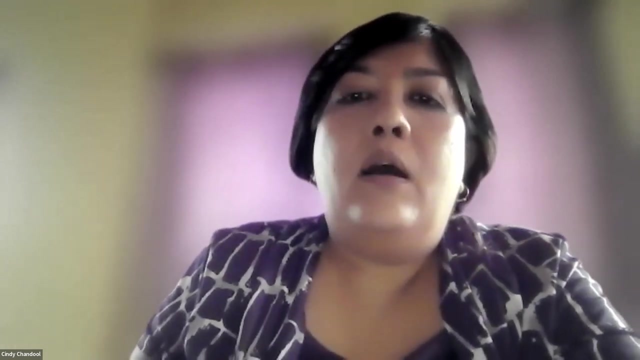 And these are disappearing because of pollution going into the marine environment and other issues. So it's important to look at terrestrial ecosystems when we're addressing issues of the marine and coastal environment. needing to clean up our agricultural, domestic dangerous chemicals, those kinds of waste that get into our marine ecosystems. 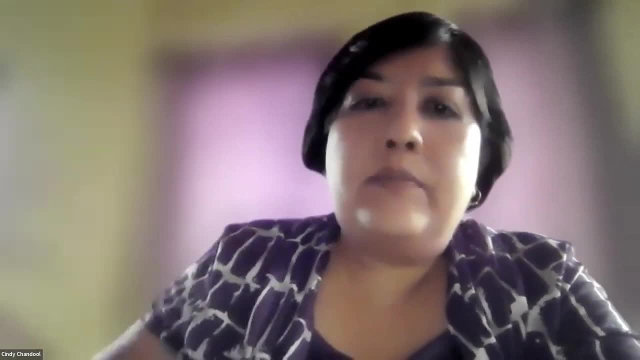 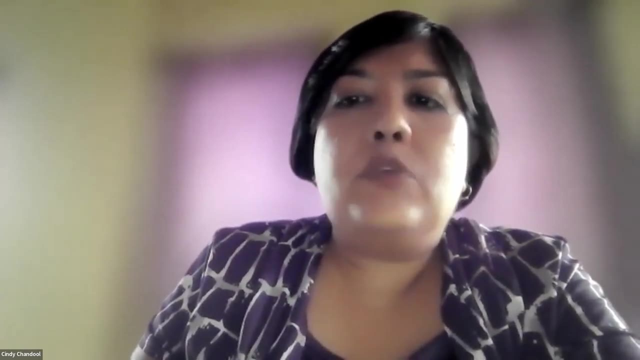 So the point was made that you know we have to protect our terrestrial ecosystems to have add-on effects of protecting our marine ecosystems. One of the issues again was overfishing, where the fishers are using beach sands which have small net sizes. 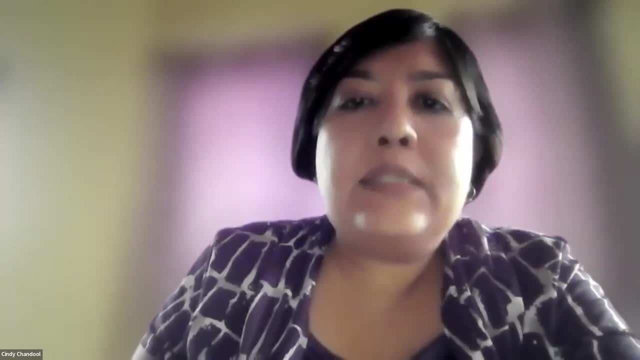 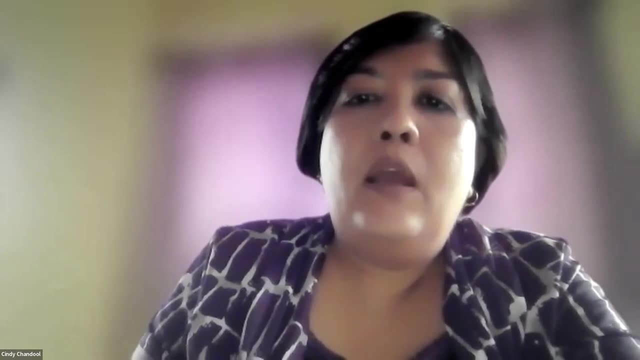 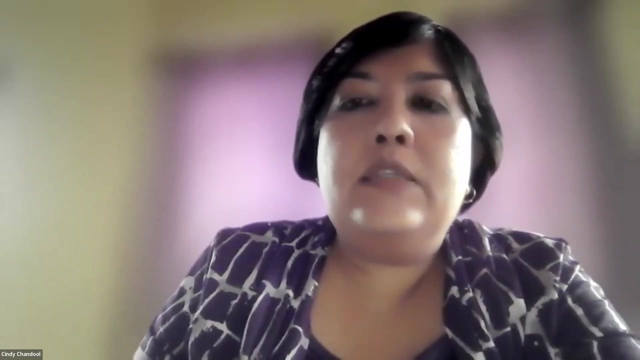 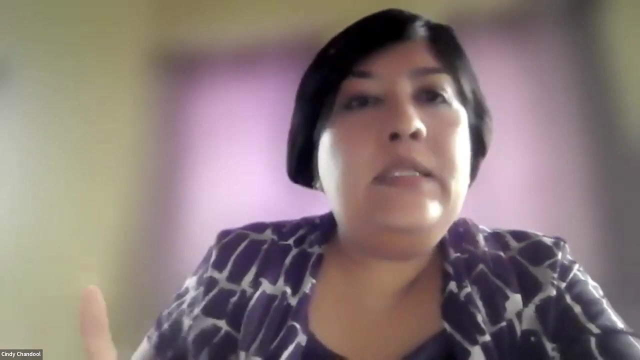 So we're having an issue of smaller Sizes of fish being caught that are also not thrown back or anything, so they're still affecting the fish species and the coastal environment. The issue of solid waste and plastics was raised in terms of, you know, values on human health, negative environmental activities affecting human health and hence you know there's a price attached to that in dealing with health issues. 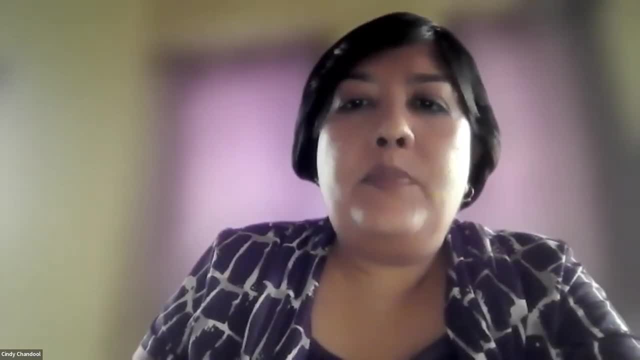 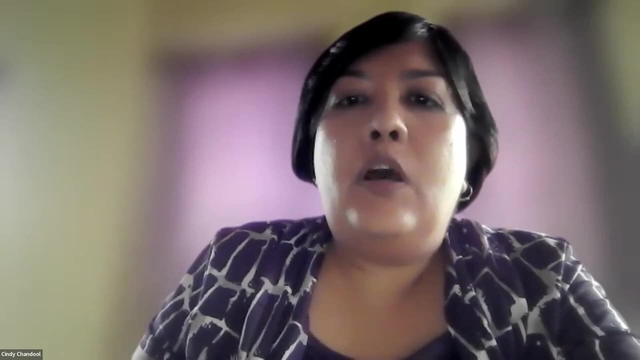 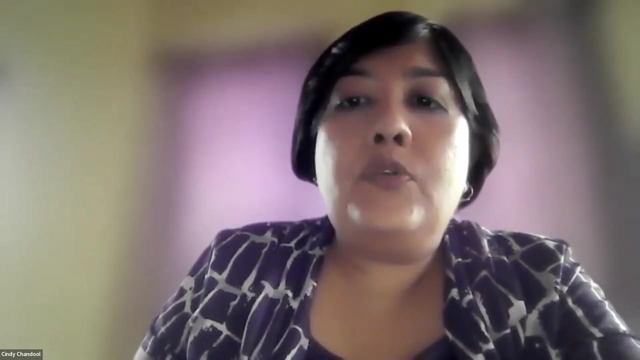 A reminder was made to look at endemic species overall and there was mentioned that there were a number of them mentioned in the chapter already. In terms of agricultural systems, the mention was made of a lot of discussion was done on the backyard farming issue, which Arya just mentioned as well. 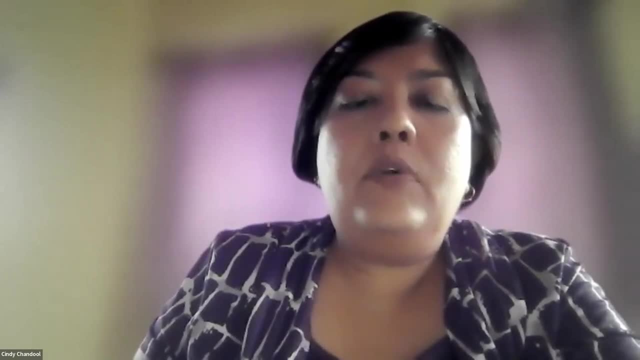 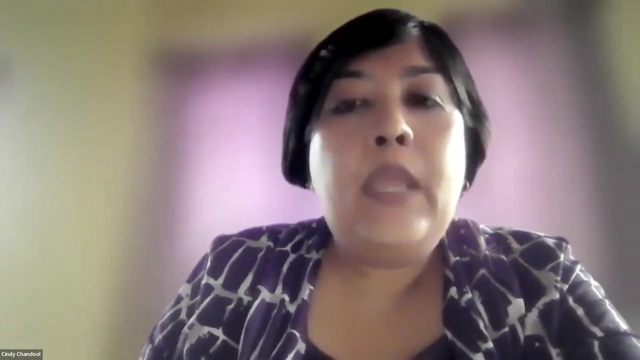 Apart from economic values, it's seen as a cultural value. There are a number of people engaged in rearing goats, sheep, cows, etc. And it's seen as a cultural value, As I said, not just an economic value, because a lot of householders use this type of agriculture as a source of income. 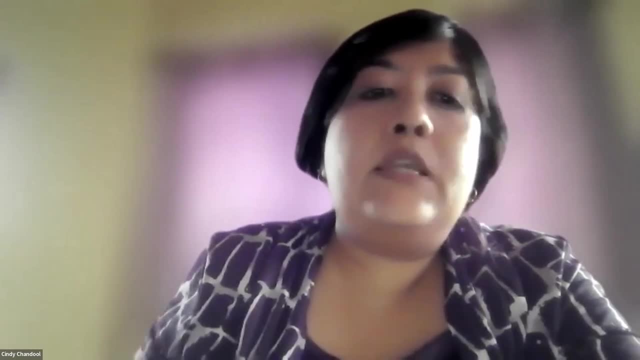 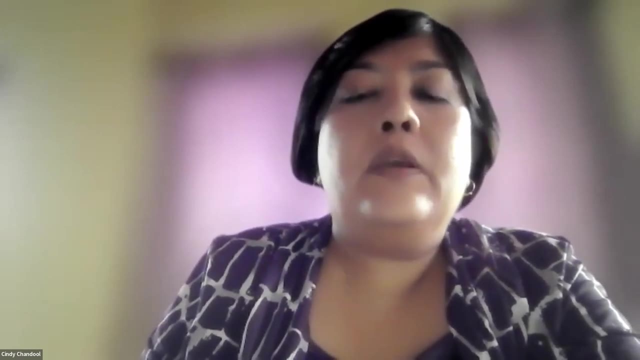 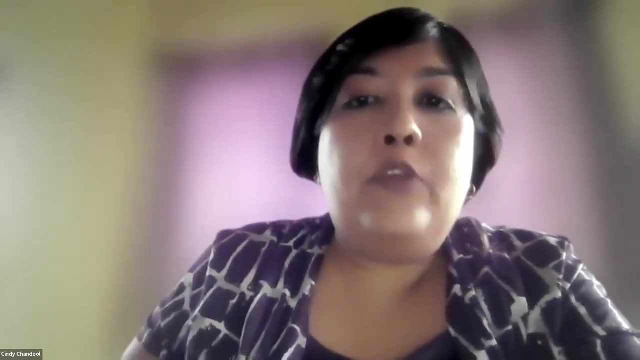 There's anecdotal evidence that it's used to even send their children to school. so they do depend on these backyard farming, but it's also an issue of imbuing the aspects of discipline and responsibility in youth. So, besides, you know it may not be a great economic value, but there's also, you know, there's a subsistence, subsistence value to be seen there. 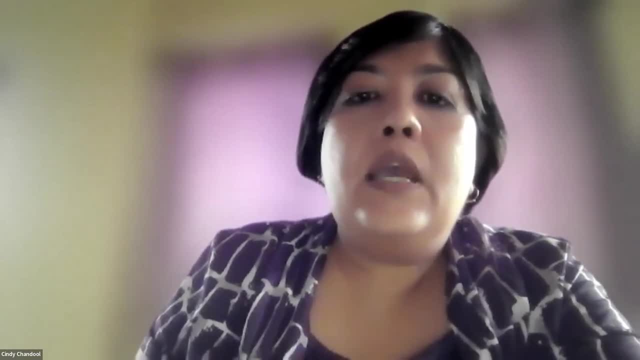 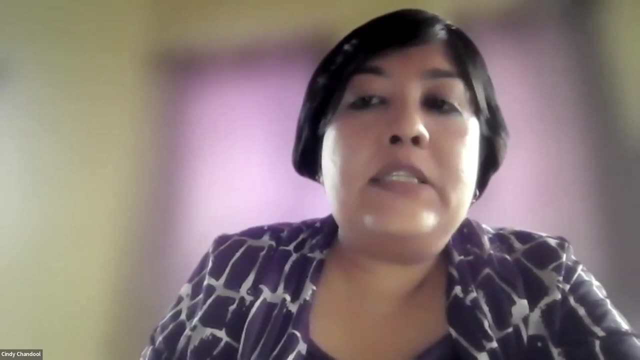 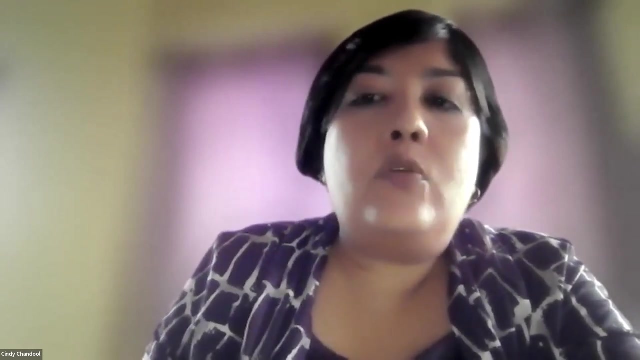 The freshwater. when we talked about freshwater resources, there's the need to look at, of course, where these agricultural activities are taking place. you do need the water resources near watercourses, and there's small waterfalls and watercourses have been seen disappearing. In some cases they may disappear for several years- dry seasons- and then reappear, and in some cases they've disappeared completely. Even small ravines that feed into larger systems, larger river ecosystems. So the value of these smaller ecosystems need to be understood as well. small ravines where you find crayfish, etc. 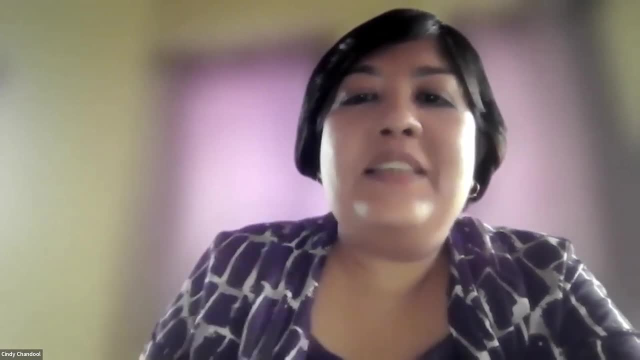 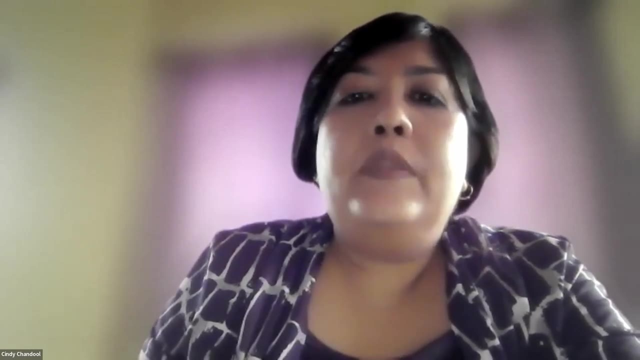 We ended a little abruptly, as you said, because we were cut off. We talked a little bit about bush medicine. we addressed that issue. we talked about zebra pick. Mention was made that other protein sources need to be explored and used rather than those that may continue. 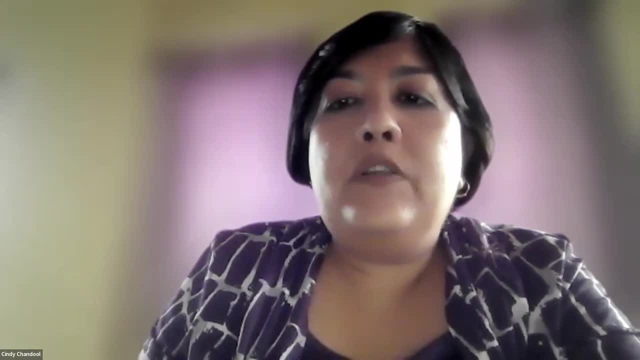 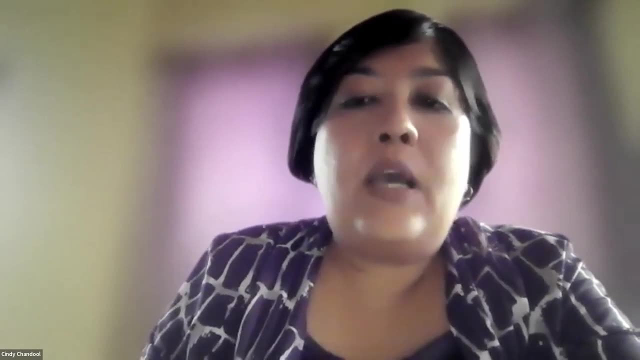 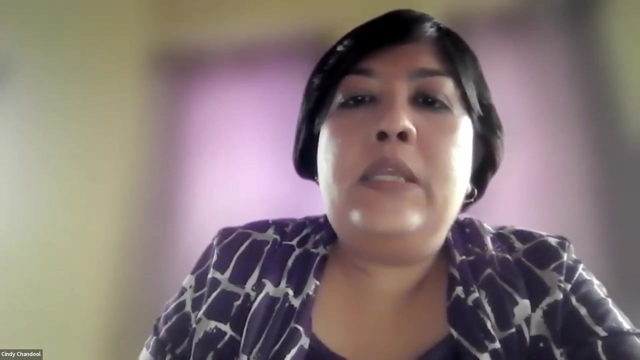 We talked a little bit about greenhouse gases and we started talking about development projects and the need to consider ecosystems when these projects are developed, That their consultations are done and then, well, that's what we got, cut off a little bit, and just one caveat that you know: they need to stop doing studies and start acting, making decisions and acting. 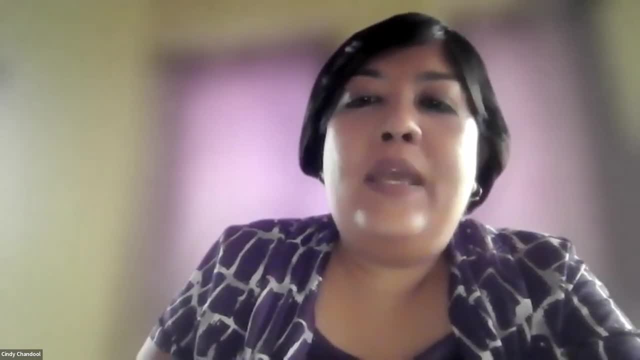 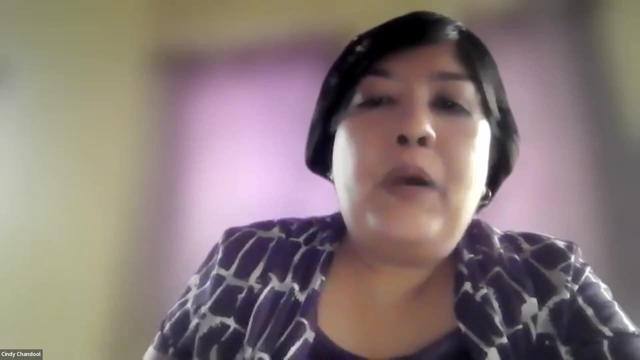 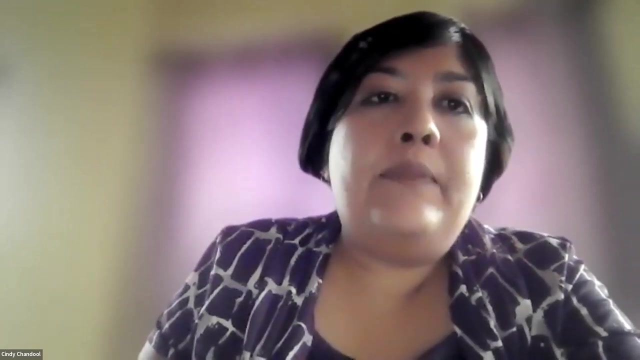 And, of course, they need to build the capacity, awareness and advocacy skills of, You know, the public at large, which I know is part of this project, so that they can participate when these consultations and development projects are done and they can effectively, you know, contribute and make their representation at such consultations. 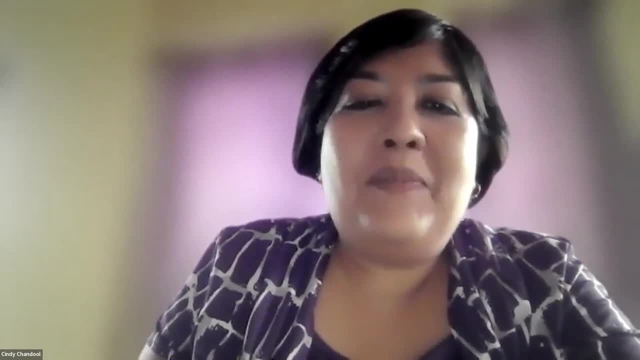 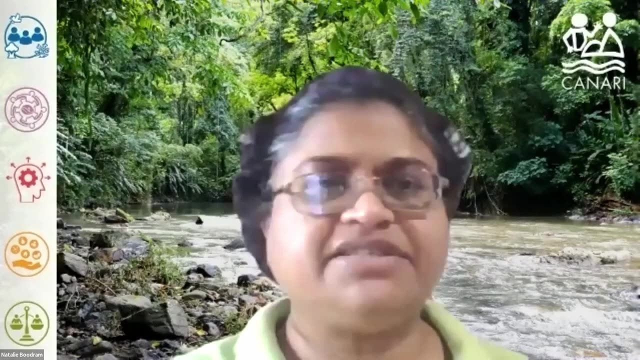 So that's all we had time for, so I'm sure there would have been a lot more coming on stream, But that's it for our group. Thank you Great, and I apologize for cutting us, cutting everybody off. We are running significantly. 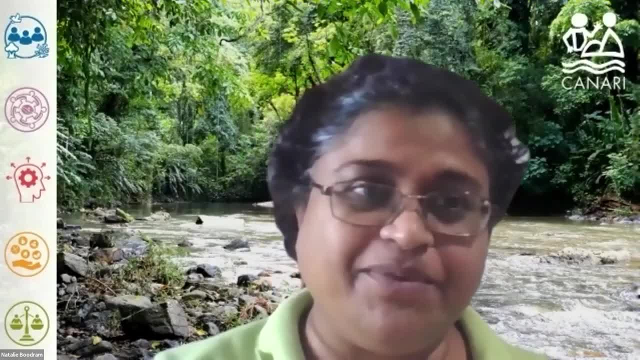 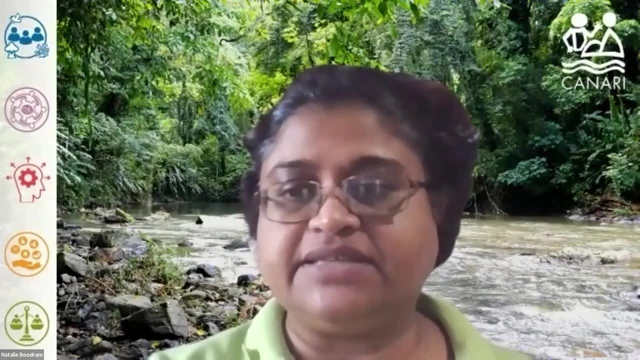 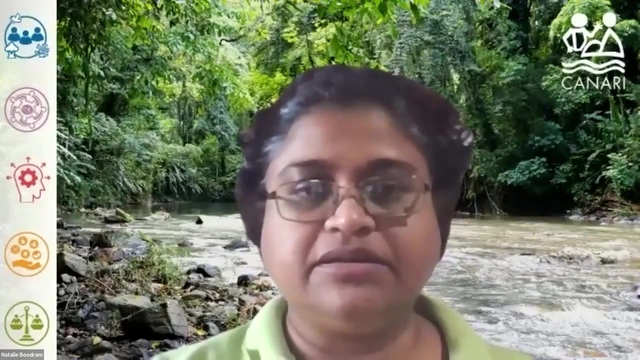 We are running significantly, We are behind time And I didn't want to keep you guys too much longer. I will take two very quick comments, if anybody has, and then I'll just say: talk about next steps. Richard, Richard, Yes. 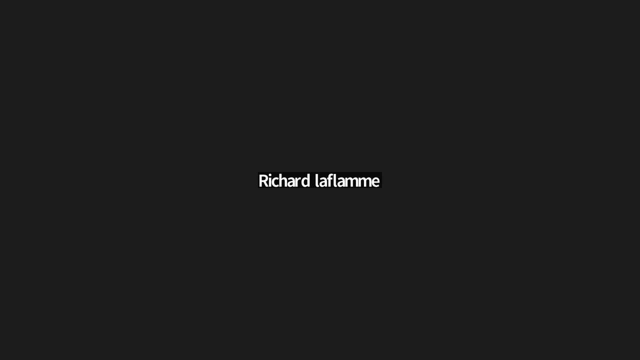 I just want to mention that, since I'm in Korea cool for the last 12 years, This is the most impressive. I had zoom meeting Very, very well organized And I think your document is really easy to understand. I ever You're missing a chapter. 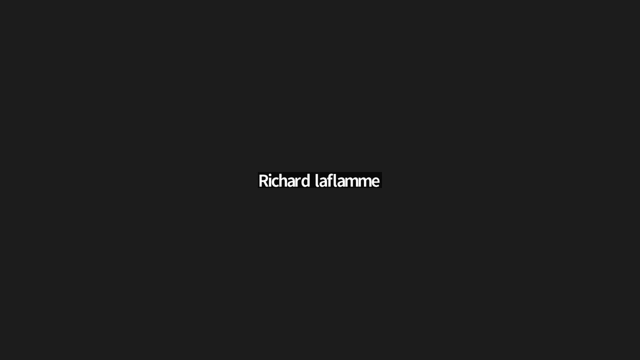 And the chapter you're missing is the action plan. You need to identify who, what, where, how much it would cost to to with the priority and then decide: Okay, Attack all. the priority number one, because there is so much to do that we need to prioritize. 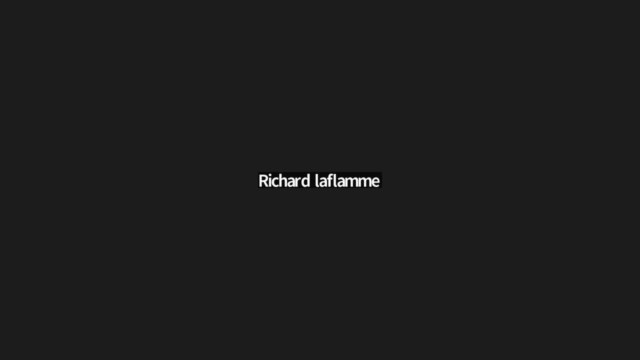 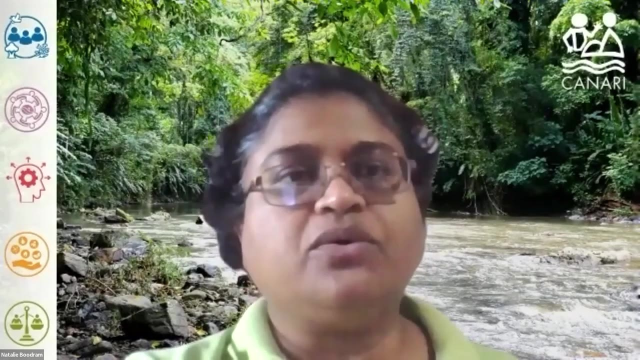 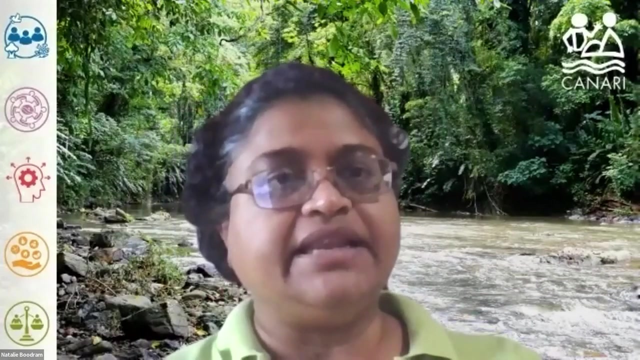 But it was very, very good Presentation Right, So to say. we do have a chapter on policy and recommendations which will go some level into that. I'm not sure if we're going to get as concrete as an action plan, but certainly there will be action suggested under that chapter as well. so there is. 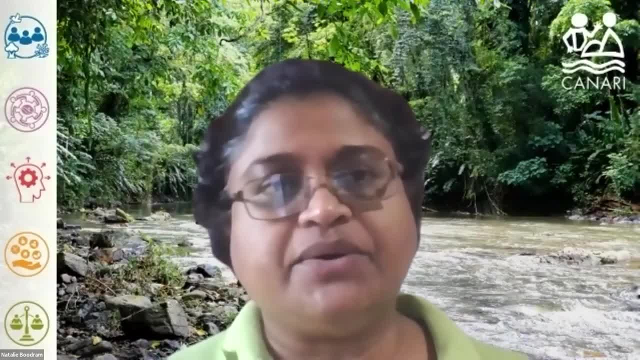 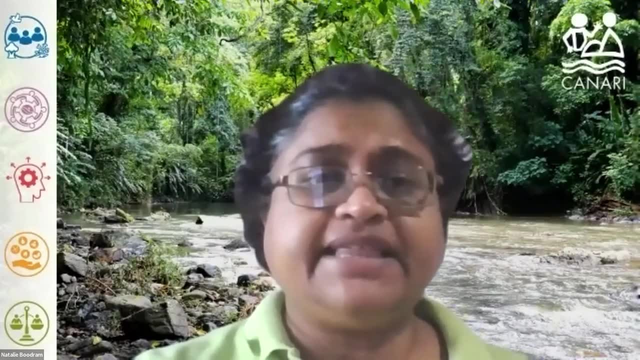 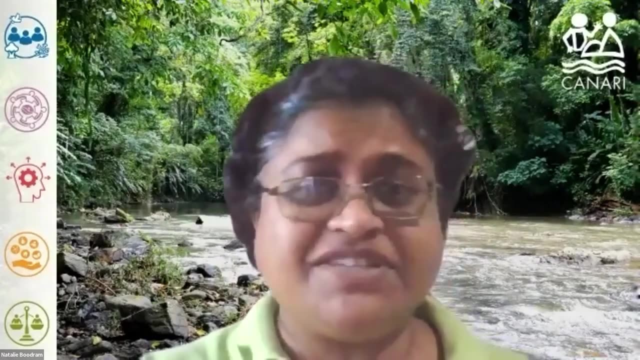 We'll be doing a review of that chapter Later on this year or early next year. Okay, I'm not seeing any other hands up, So just to say thank you to everybody. thank you all for allowing us more time. We don't normally run this late on meetings, but thank you for sticking it out. 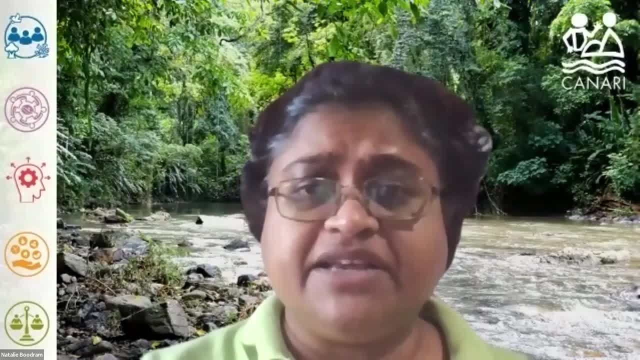 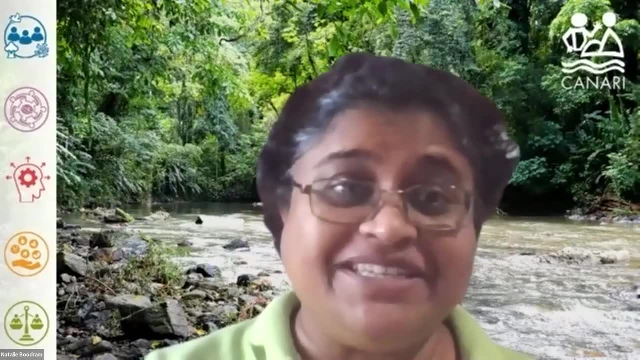 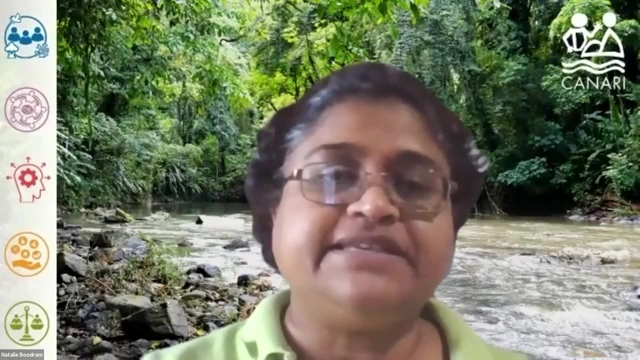 Thanks to all the presenters. I think you all did an excellent job. Thank you so much, Cindy, Alex, area or reporters, especially Daniel, who did that double duty. Thank you, Thank you. Thank you very much, Daniel, to proper during sessions and a reminder to you all to send us in the word document summarizing that we can forward to the chapter authors as well. 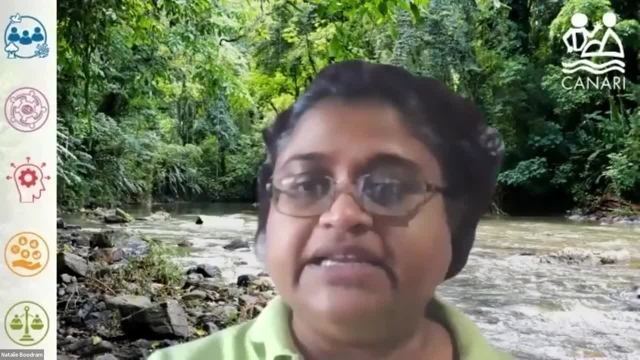 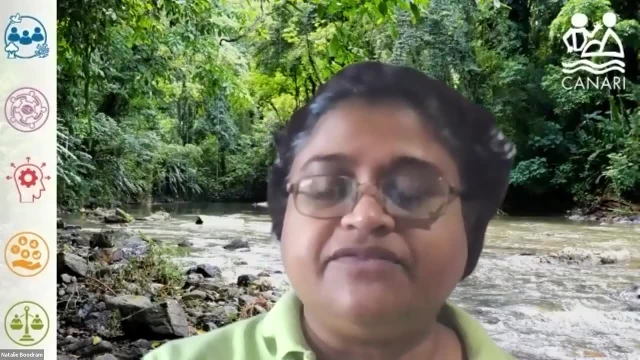 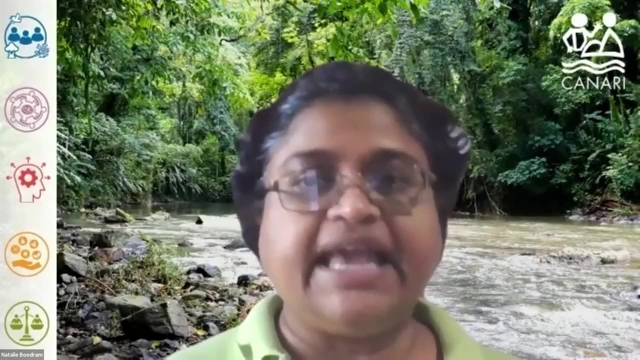 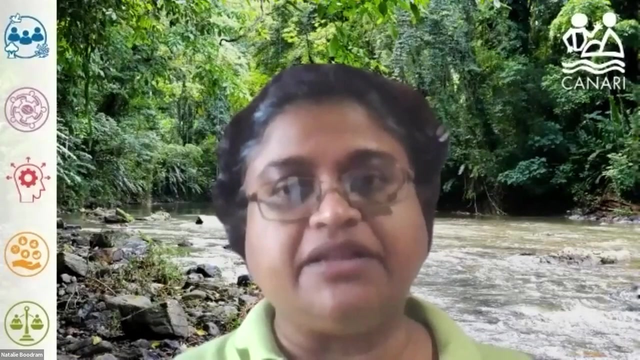 Thanks to the Canary team very hard at work behind the scenes. so Iran at DT and Anastasia, Thank you very much. In terms of next steps, So we will be making a final call for comments on: we'll send out the chapter, We'll send out the chapter summaries again and you break out group questions. So if you didn't get a chance to comment Now, you can send us comments via email. 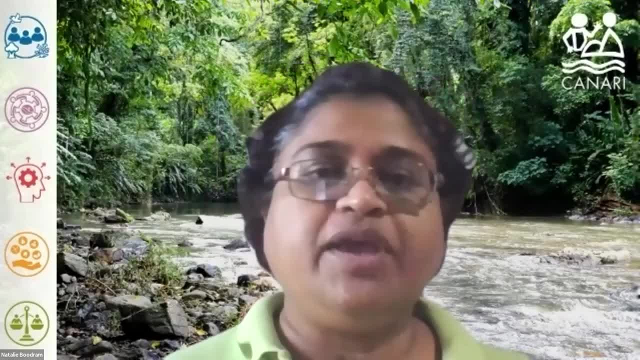 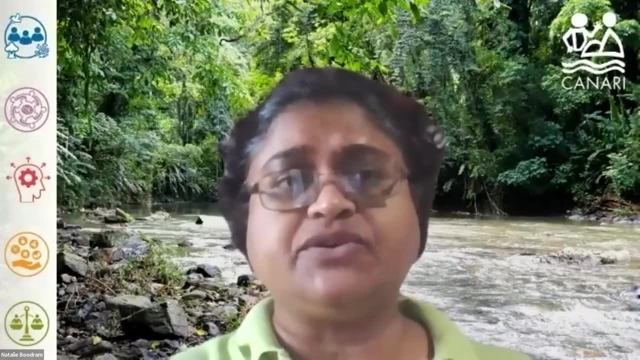 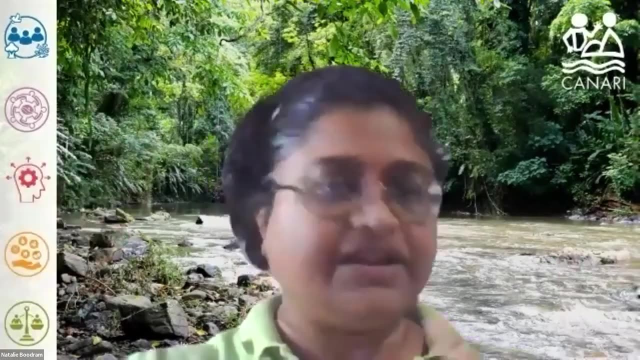 As per the first session we had a couple weeks ago, we are looking for official chapter reviewers, people who will review the actual document. So if you are interested in doing that, you'll have to let us know. you'll have to sign a little confidentiality agreement before we actually publish the document. 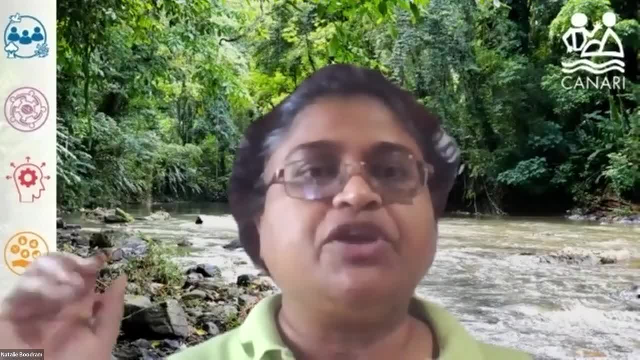 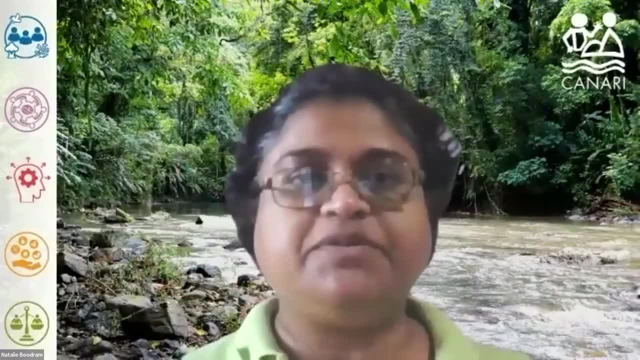 And then we'll send it to you if you're reviewing the draft material and you will be credited as a reviewer on the chapter as well. so, And it doesn't have to be the whole chapter or more than one chapters- whatever you're comfortable and are interested in. 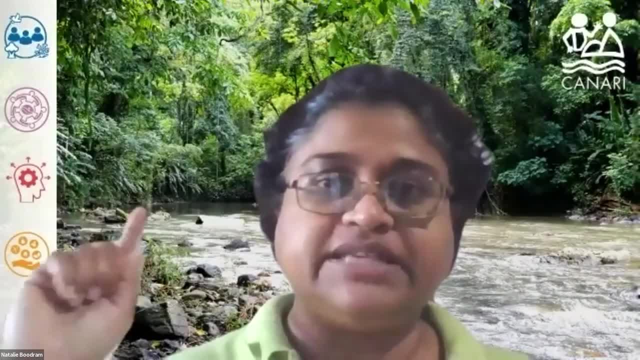 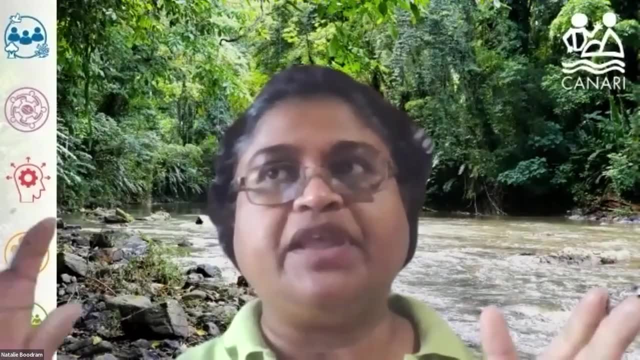 The next step. we are actually going straight in a couple weeks into that advocacy slash: communication of info, environmental information. we'll be using the some of the material in the NAA as the basis for this, But overall it's about how to do it. 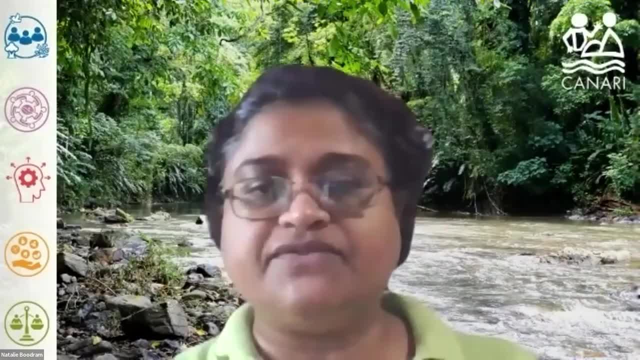 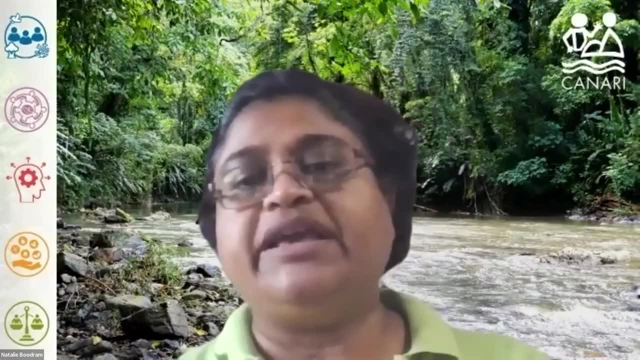 But overall it's about how to communicate, how to advocate. so our colleagues, for instance from the Grenada Green group, you are more than welcome to attend. you might get some ideas how to do your own campaigns as it pertains to littering, etc. So look out for notices for that. 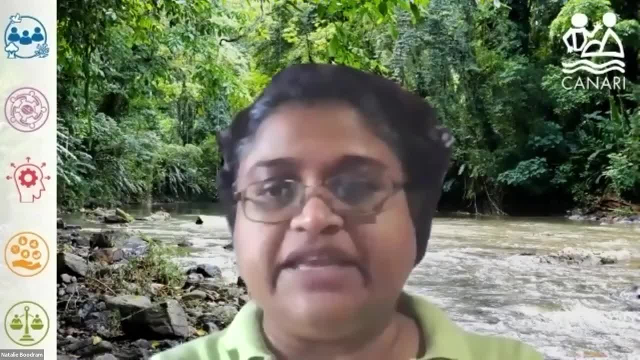 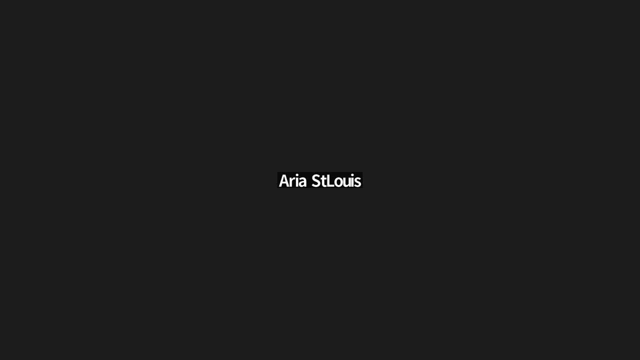 And with that, Aria, do you want one minute to give some closing remarks as a co-chair, as you didn't speak the first meeting and then we can close. Sure, I just want to say thank you so very much for the response. 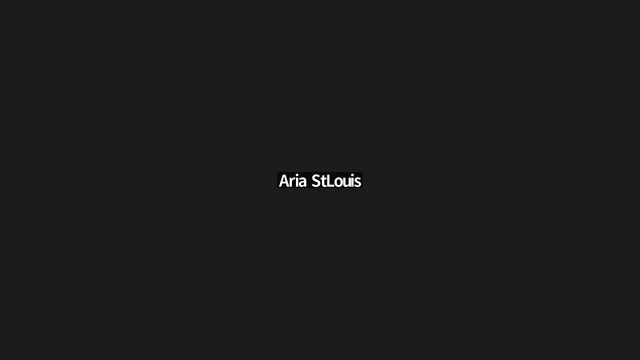 And I just want to say thank you for the effectiveness of those who have attended. I really feel that I like to echo Mr Laflamme's comments. We have seen a tremendous effort to coordinate by Canary 72 different authors. we have seen a tremendous effort by the lead authors, some of whom presented today, and the contributing authors to work with Grenada. I think that it's really clear that we have a rich opportunity.